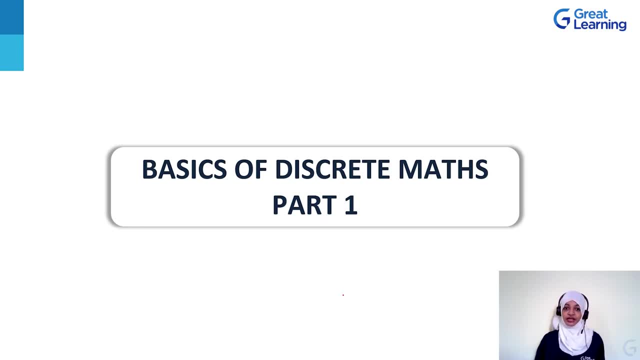 you're pursuing, if your field is computer science, various other higher level subjects such as networking, operating, system-based scheduling, AI, ML and various other fields such as graphics, are all dependent upon the basic discrete mathematics concept. Understanding the basic concepts of discrete mathematics will often help you better. 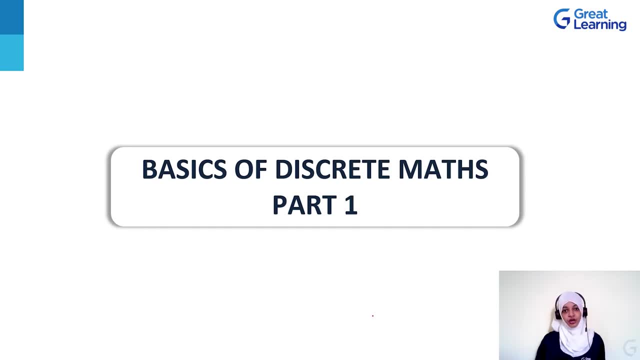 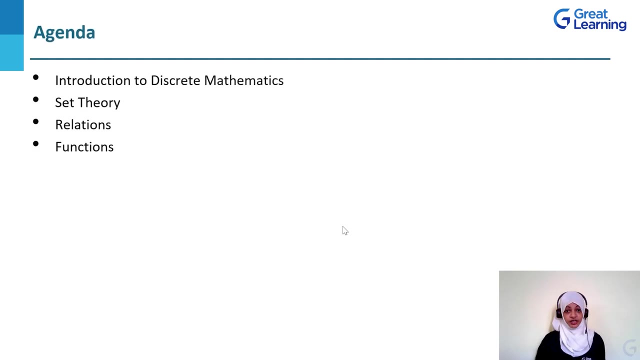 understand the hows and whys of the advanced topics that you might learn later in your degree. Thus, discrete mathematics is an important part of any computer science degree. Let us now look at what we're going to study in discrete mathematics. First, we'll be looking at what discrete mathematics actually is and a few of their. 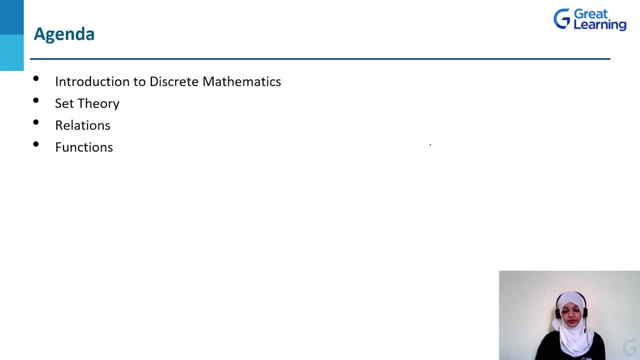 applications in solving real-life problems. Next, we're going to look at set theory, which is often helpful in resolving scheduling problems and is also used in software engineering, often in order to resolve any kind of resource problems. Next we'll be looking at relations because, of course, if any two sets would be related to each. 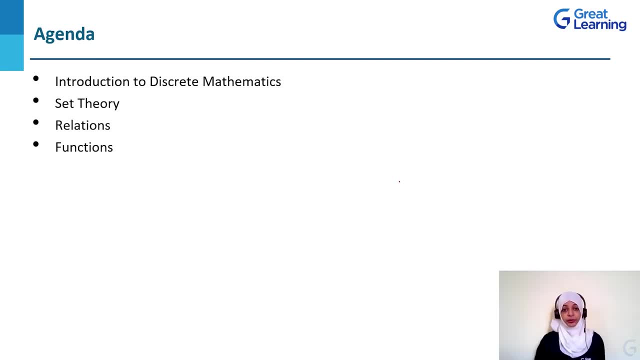 other or are in working with, continuing with one another, there would be a relation between them. So what are those relations and how can they be resolved? Lastly, we'll be looking at functions, because relations between any two sets are obviously based upon some functionality or the 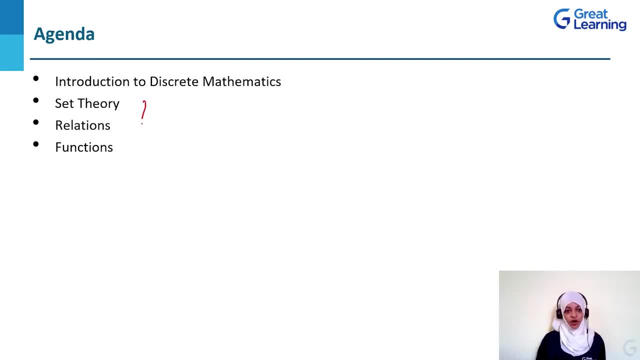 other. Thus, we'll be looking at all of these three components in tandem with one another, so that we may better understand these concepts and how they're related to one another. So let's get started. So let's get started with the introduction to discrete mathematics. 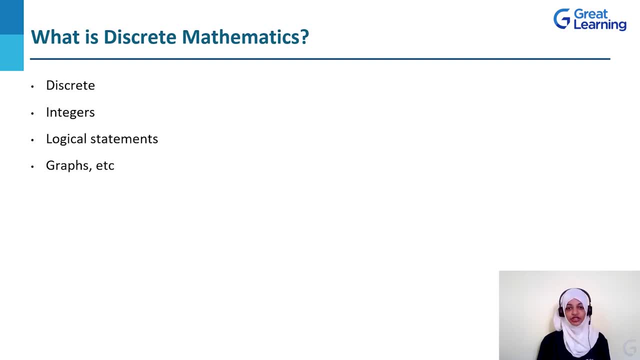 Let us first look into what discrete mathematics actually is. Discrete mathematics is the branch of mathematics which is concerned with discrete or non-continuous values. In order to understand the difference between continuous and non-continuous values, let us take an example of two separate sets. Let the first set be a set of natural numbers. 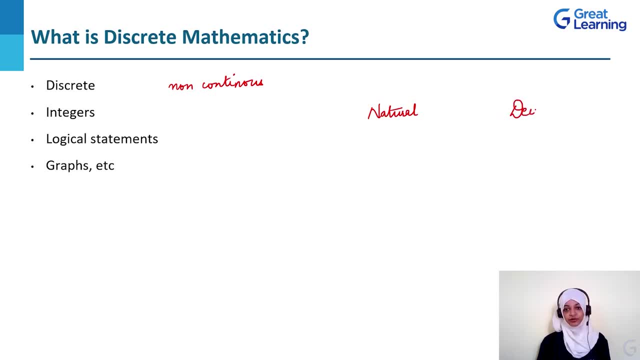 and let the second set be a set of decimal values. Consider any two adjacent values in natural numbers On a number line 3 and 1. and 4 are adjacent values. Similarly, let us consider two adjacent values for decimals. Say, on a number line 1.4 and 1.5 are two adjacent decimals. 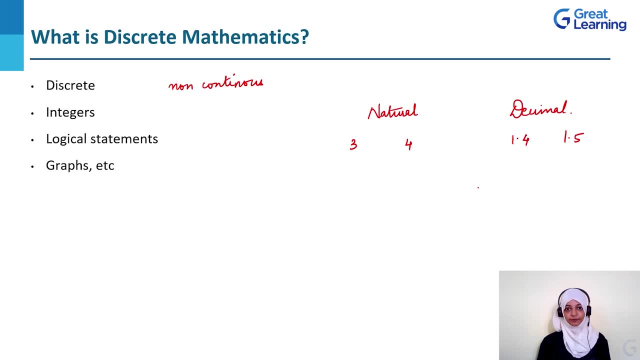 Observe these two and look at the difference between them, You will find that on the number line between any two adjacent values in natural numbers there are no other values available. This means that between two adjacent values there are no intermediate values. when we look at the set of natural numbers, 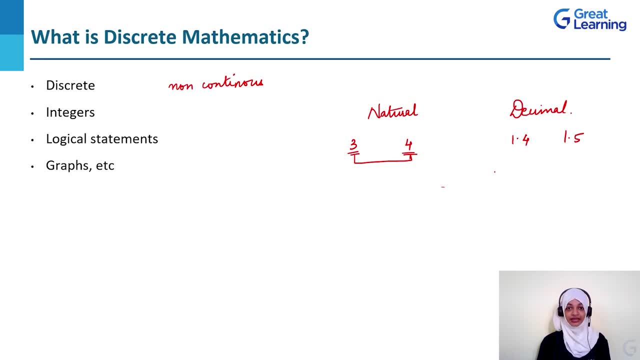 Let us observe decimals. on the other hand, In a number line between two adjacent decimals, we would ideally have a set of infinite number of intermediate decimals, For example 1.41,, 1.42,, 1.423, and so on and so forth. Thus, between two adjacent values in decimals, 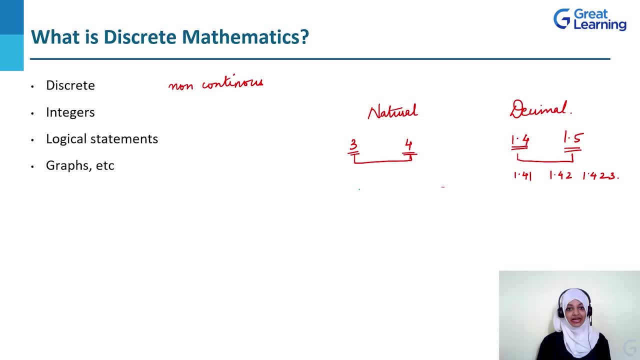 we will find a number of continuous values. Thus, a set of natural numbers is known to be discrete in nature, whereas the set of decimals are known to be continuous in nature. Other examples of discrete components are integers, logical statements and graphs. 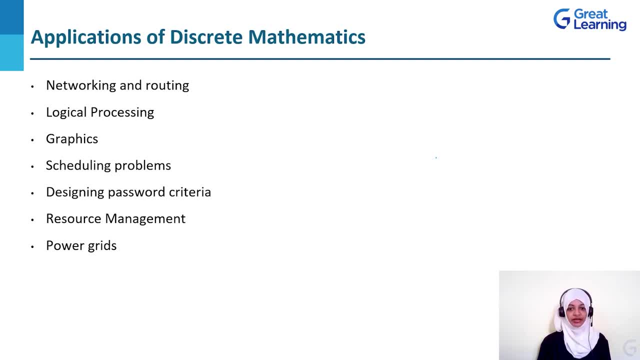 Next, let us look at some of the real-life applications of discrete mathematics. Discrete mathematics, or DM as it's called many a times, consists of various branches. Many of these branches, in basic or advanced forms, help us in actually resolving real-life issues. 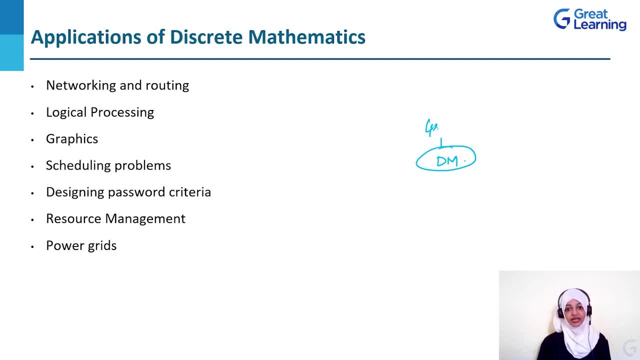 For example, a branch of discrete mathematics known as graph theory helps us in resolving all kinds of networking and routing problems. It also helps us resolve power-grid issues. The basic components are very simple, because the questions in both of these problems are similar to each other: How is a particular route supposed to be chosen? 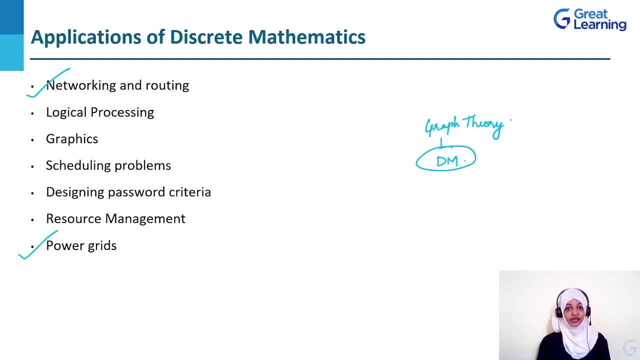 If there is a traffic line in one particular route, what about this traffic line? How to we reroute our cars in such a manner that we can get off of a traffic-laden area scot-free? How many units are supposed to be supplied in any power grid? 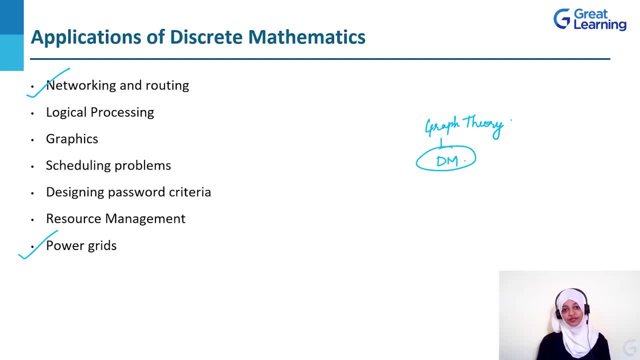 How many towers or lines have to be constructed in order to successfully supply sufficient amounts of power to various areas that are a part of the grid? All such issues can be resolved using graph theory. Next, logical processing can be resolved by using the concept of logic. 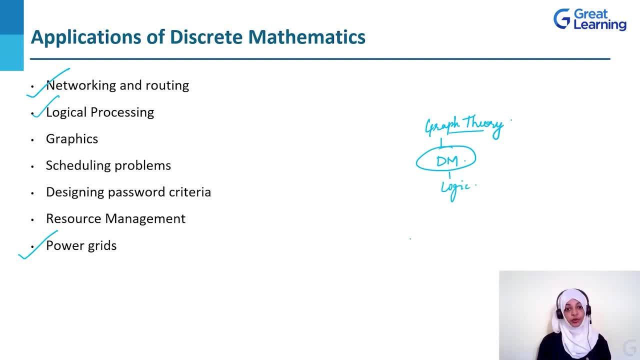 Logical statements that provide us with yes or no answers, or zero and one answers or, as we can call them, true or false answers, often help with logical processing in computers. Now, these computers are any device that can compute or process, So they may be laptops, they may be desktops, they may be mobile devices. 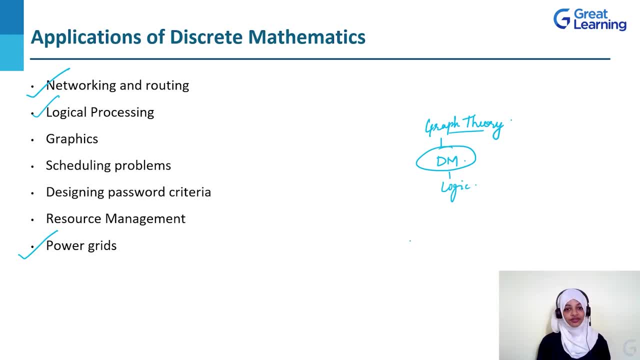 All of these have logical processing And therefore all of these devices have the basic component of logical statement processing, which helps with higher-level logical processing in them. Next, we've got graphics. In various graphics we've seen objects move from one place on the screen to another distinct 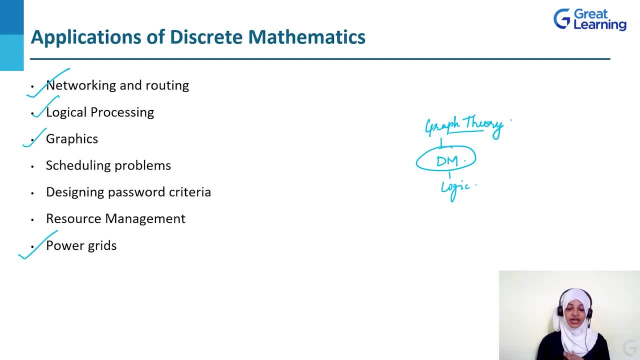 place on the screen. These transformations are carried out by using a branch of discrete maths known as linear algebra- LA for short, Linear algebra- L-A for short- Linear algebra is a branch of discrete mathematics that actually helps us in producing transformations such as translation, which is movement of one object from one place to the other, scaling. 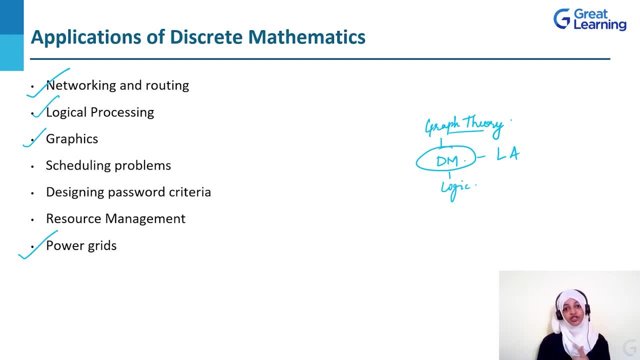 which is enlargement or shrinking of an object, and rotation of an object around one or multiple of its axis. There may even be transformations which are a combination of all of these various transformations. These can be implemented by using the concepts of linear algebra. Scheduling problems can often be resolved using graph shading or graph colouring. as 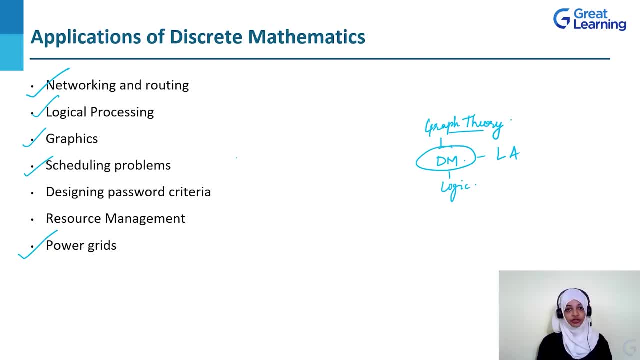 it's called, which is an advanced part of graph theory. Next, we've got password criteria designing, which uses components such as permutations and combinations, which is NCR. All of these components actually help in doing so, So let's take a look. 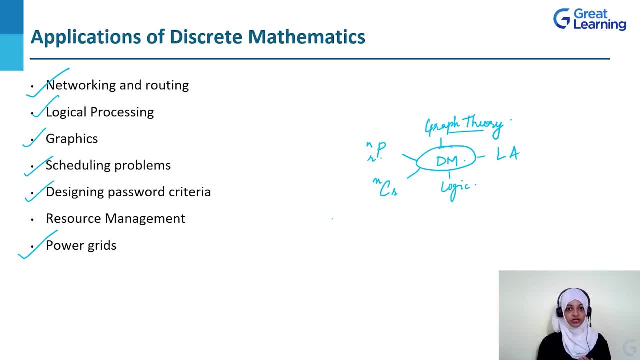 Let's take a look. Let's start off with determining how a certain set of characters should be arranged. These characters could be alphanumeric in nature or specialised. The arrangement and number of components in any of the price password, the number and arrangements of these characters in any password, will determine the strength or the weakness. 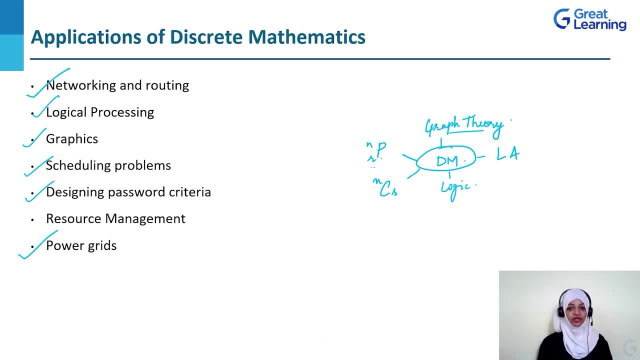 of the password, And this can be calculated by using permutations and combinations- another part of discrete maths. Lastly, we've got resource management management. Resource management, or any apportionment problems for that matter, can easily be resolved by using a component of discrete maths known as counting. There are various counting rules. 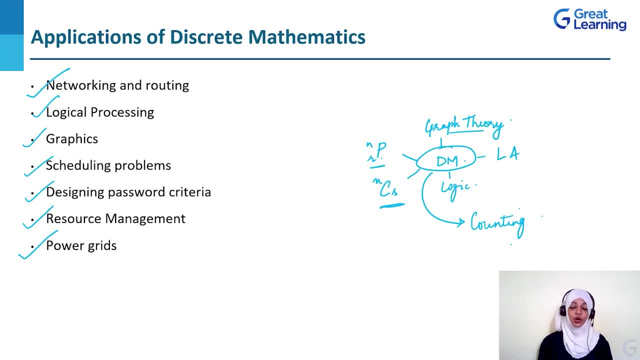 and algorithms that are present within discrete maths, which help us exactly determine how much should be allocated to what. Now, what? the resource that needs to be allocated can be food, it can be stationary, it can be space, So any kind of resource that needs to be allocated. 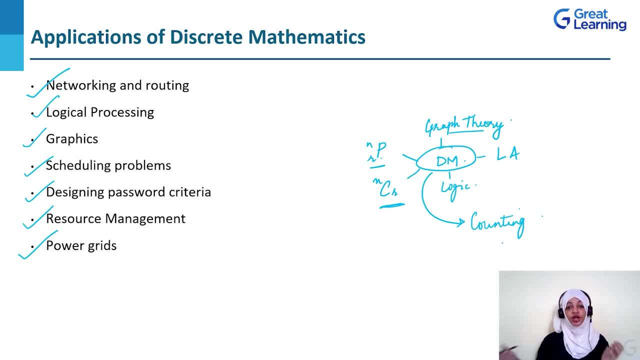 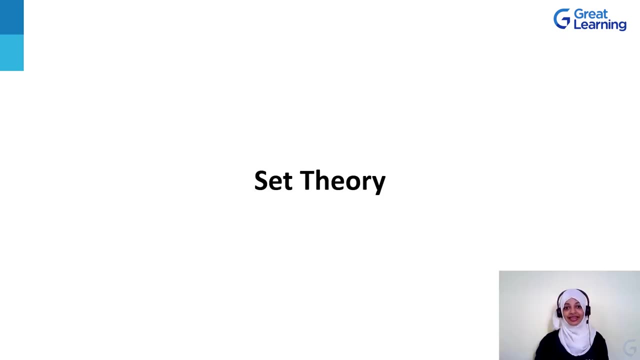 can be distributed between a certain set of people using our counting principles. Thus we've seen how a lot of the real life problems can also be resolved using discrete mathematics. So let's now get started with the basic components of discrete mathematics. Let us start with our first basic. 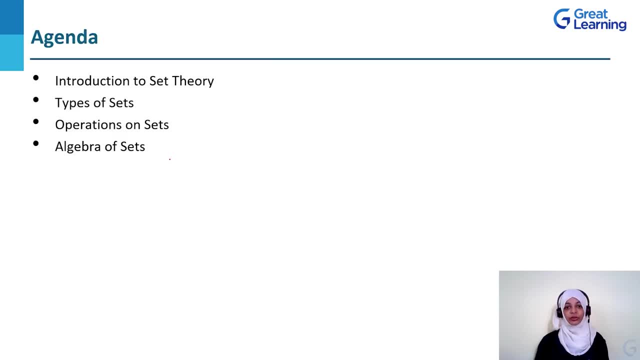 concept in discrete maths, which is set theory. We'll start off with understanding what set theory actually is. Next, we'll look at the various types of set that are a part of set theory. We'll also look at some of the operations that can be performed between or on a single set And, lastly, we'll look at some of the laws that form the basis of the algebra of sets. Apart from these, we'll also be looking at some 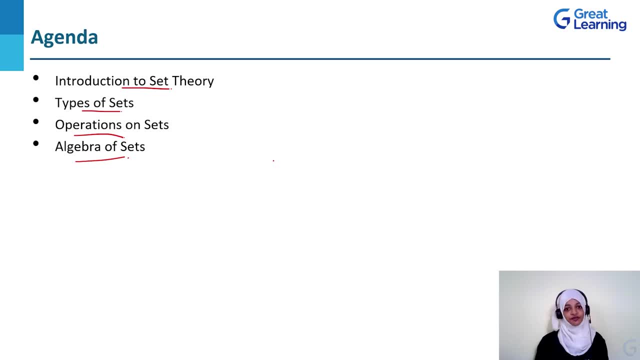 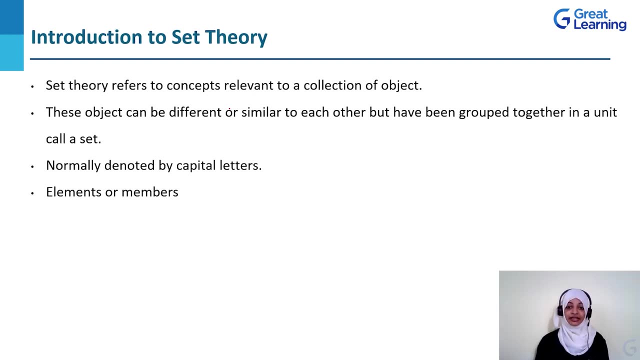 algebraic sums based upon the algebra of sets. So let's get started. So what exactly is set theory? Set theory refers to all of the concepts that are related to a collection of objects. Any collection of objects are known as set, and any concepts related to those set will be referred to as set theory. The objects that we have clubbed together may either be similar to each other or they may be different from each other. The basis of formation of a set is a particular logic, which we'll be looking at in this video. So let's get started. 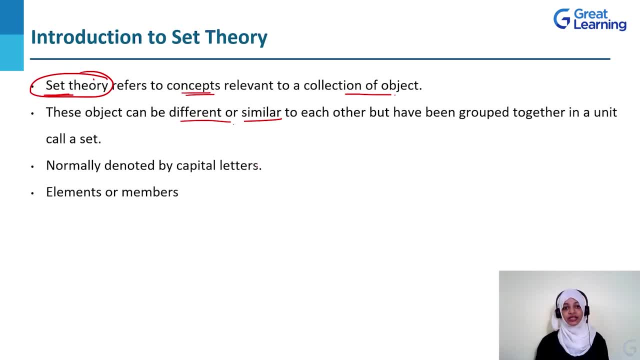 Let's try to find out what all those objects are. So two sets of sets capture different threw poorer Dia, who are most commonly used capital alphabets, Not toering with the ideas or including the concepts. We've also learned that all sets have a common сем: specialist. 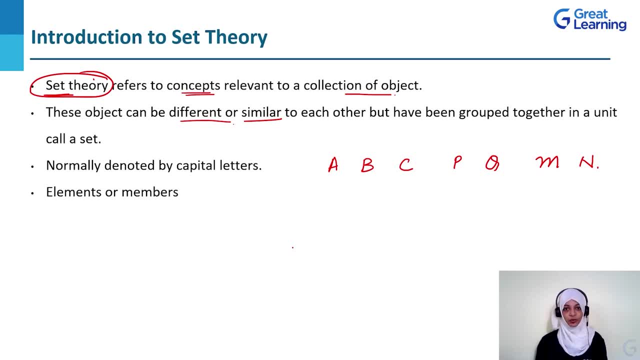 namely theippessimist for the form of the words. We know that is not their fathom in the word. stacks is not a normal UST, It is reference superior, such as considering name or part of a continuous string vs examining the fixed form of things. 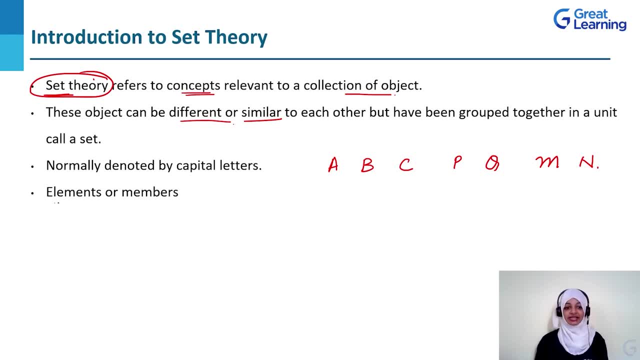 The common semantac writing model is They write a mort, C, D, P, X. These models get architecturally a set, are often known as elements of a set or members of a set. Members of various sets interact with one another based upon the algebraic rules that we'll be seeing later on. 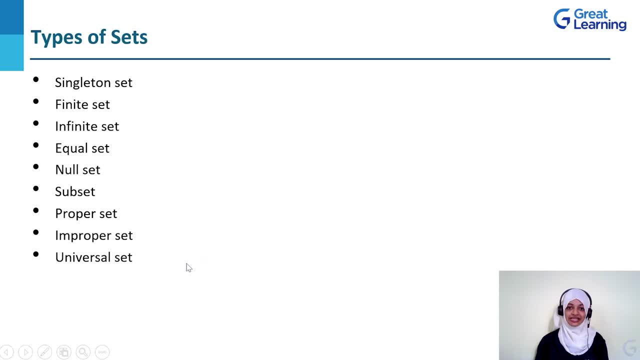 Now let's look at the various types of sets which are commonly seen in set theory. The first type of set is known as the singleton set. As a definition, it's very easy: Any set that contains only one element is known as a singleton set. So a set, say A, would be a singleton set, since it has 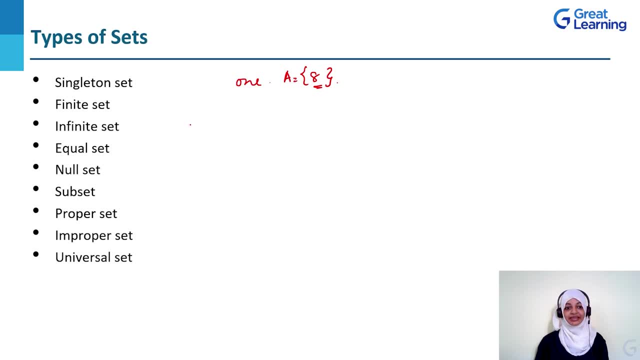 just one single element in it. Next, we've got finite sets. As the name suggests, if we have a set that has a finite number of elements within them, it'll be known as a finite set. On the other hand, if a set has infinite number of elements within it, then it will. 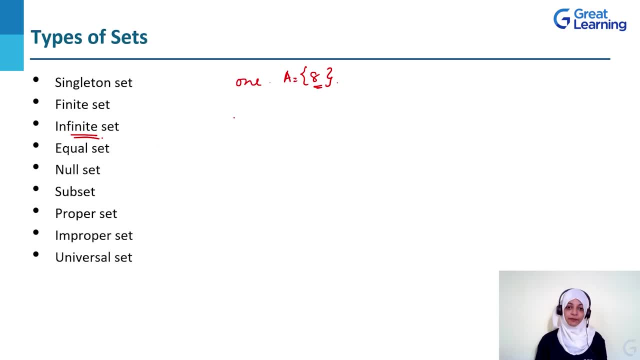 be known as infinite. In order to illustrate this with an example, let us take two sets. Let one set be the set of even numbers between 2 and 10, inclusive of both the values given here. Thus, the set would be say 2,, 4,, 6,, 8, and 10.. Five values, right. 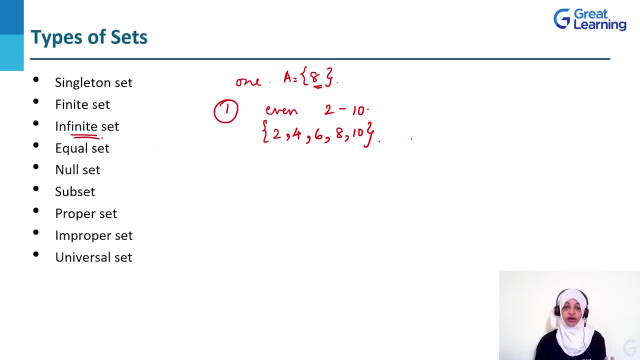 So a definitive, countable number of values which are a part of the set. This set is a finite set. Let us look at an example of an infinite set. So examples of infinite set are infinite in themselves: Set of natural numbers, set of integers, set of real numbers, set of whole numbers. 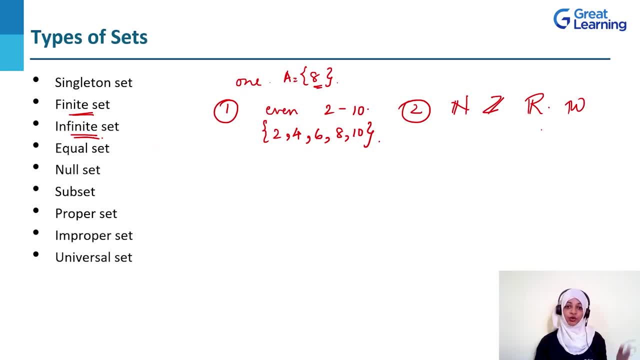 All of these are infinite sets because they can go from a lower limit to a no upper limit or, in some cases, no lower limit. So a finite set is a set of even numbers between 2 and 10, inclusive of both the values given here. 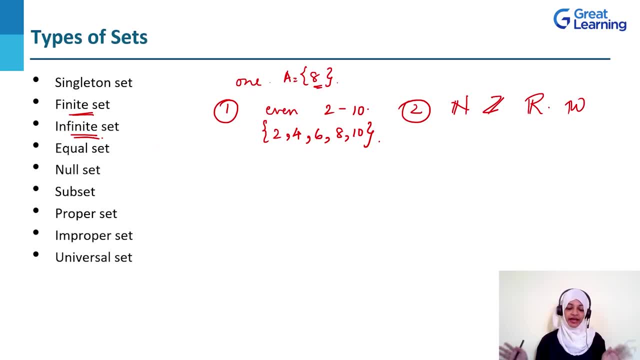 Thus the set of even numbers between 2 and 10, inclusive of both the values given here. Such sets, which have uncountable number of elements and ever-growing number of elements within them, are known as infinite sets. Next, let us look at equal sets. 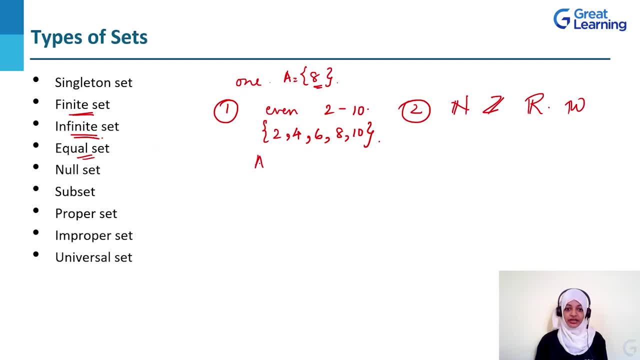 Equal sets are those sets wherein, on comparison, we've got the exact same element in both sets. Please note: the key word here is exact same elements. So the number of elements, as well as the elements themselves, have to be the exact same in both sets. 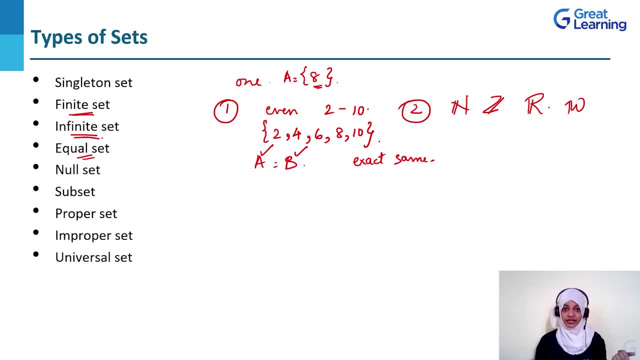 The reason I'm saying this is because often equal sets are confused with equivalent sets. Please note that these two are not the same. Null set is often denoted by the value phi. A phi implies that there are no elements within this set. Another denotation of a null set would be: 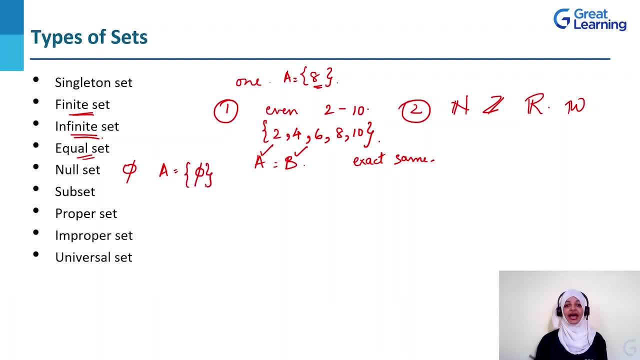 the writing of a set followed by the writing of phi as an element within that set. This again means that there are no elements within the set. So the number of elements here basically would be zero. Next, let us look at subsets. Subsets refer to sets which are a part of another set. 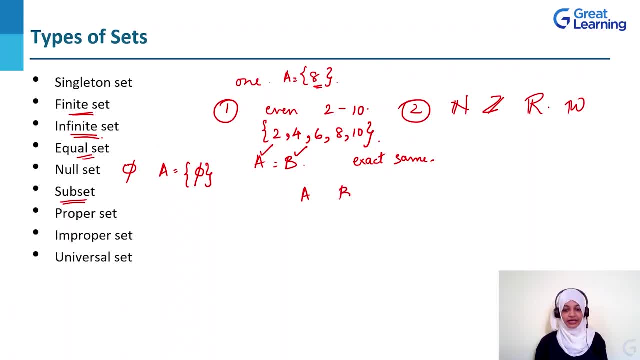 For example, if we have a set A and a set B, A is a subset of B. if A contains some or all the elements of B. Let us take an example. for the same Say: set A is equal to 2, 4, whereas set B is equal to 2, 4 and 6.. 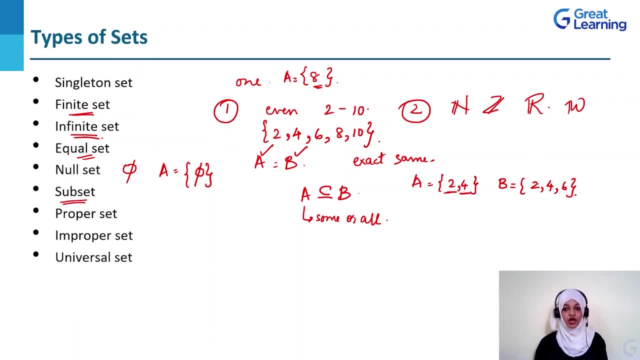 Observe that set A contains elements of set B. They might not be all the elements, they might be only some of them. They do contain A- I'll repeat this- But A does contain some elements of B. Thus we can say that A is a subset of B. Based upon subsets, we now have two. 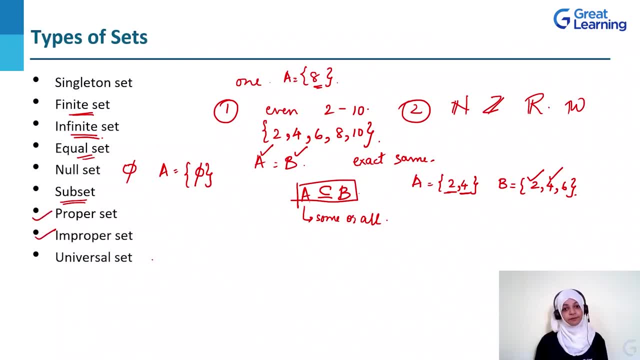 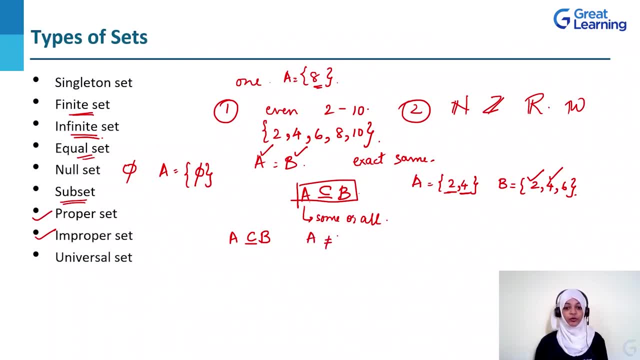 B, then A is never going to be equal to B, So any subset that is never equal to its superset would be known as a proper set. An improper set, on the other hand, is a subset of any set, such that the subset may be equal to the set. Thus we've got proper and improper sets. 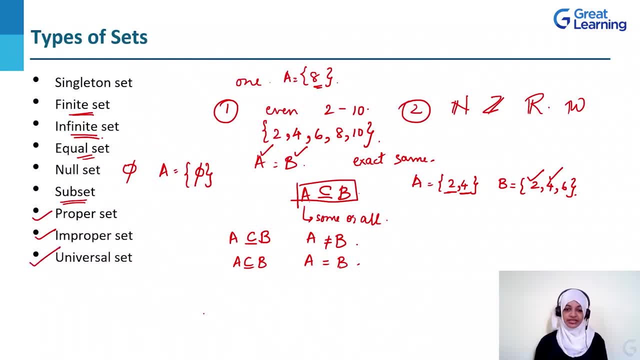 The last set we have is the universal set. The universal set is a parent set consisting of all the relevant subsets. Another way of defining this is that universal set is the parent set containing all of the subsets under consideration. Please make a note of this. The reason I'm emphasizing on this is because 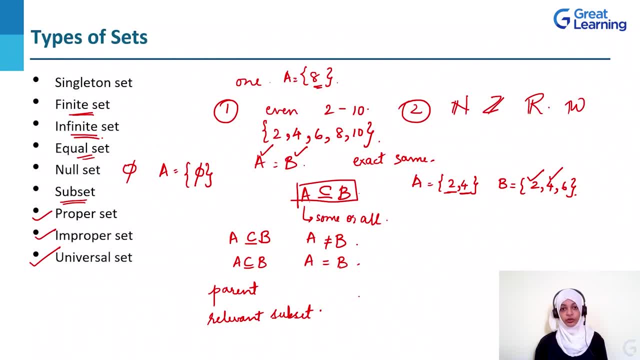 the universal set is different from what is normally known as a power set. We'll look at the difference now. A power set refers to the parent set of any and all sets that we might use in set theory. A universal set, on the other hand, is just: the parent set of all of the subsets. The user can use the universal set to say that C is equal to B. If I take this set of N and Z between officers C and E, they will all be equal to 8 and 5.. So any set of N and Z is equal to 12.. If I take this set of Y and Z, they will all be equal. 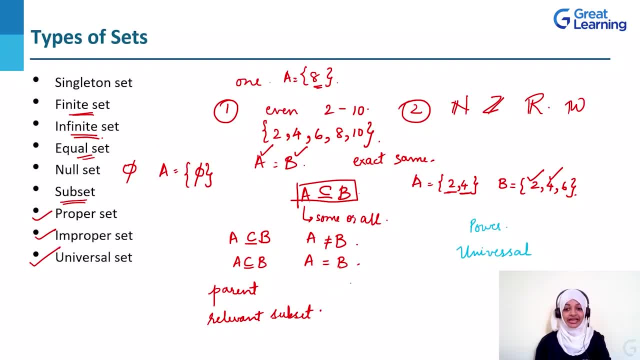 to 0.. We are also able to compare our total set of N and Z. So the universal set of N and Z comes out as the set of N and Z, So we get the difference in use here. We thank you for your sets currently under consideration. Let's take an example of set A and B. 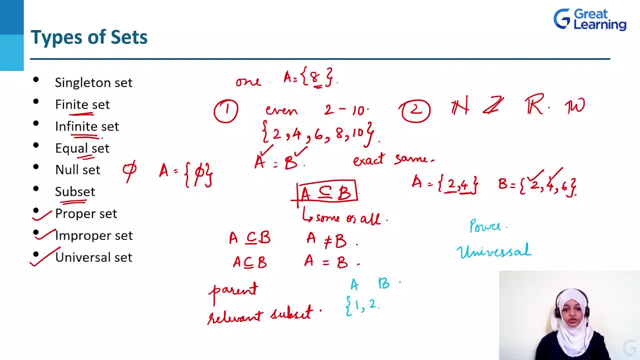 Say, set A is equal to 1,, 2 and 5, whereas set B is equal to 3 and 4.. The universal set would be the set of numbers between 1 to 5, because that is what the complete parent set of A and B would be. 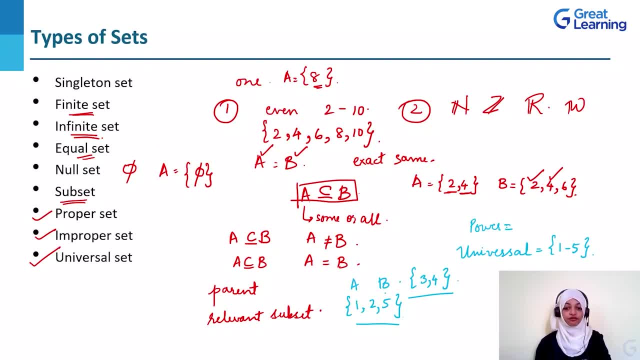 On the other hand, the power set of A and B would be the set of all natural numbers. This power set does not necessarily only contain A and B sets within them. It might contain other sets too. On the other hand, the universal set contains only the set A and B. 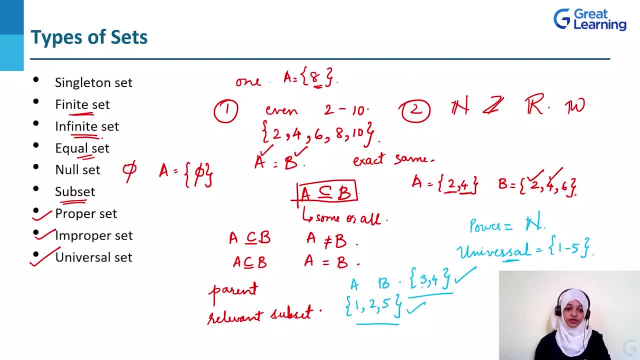 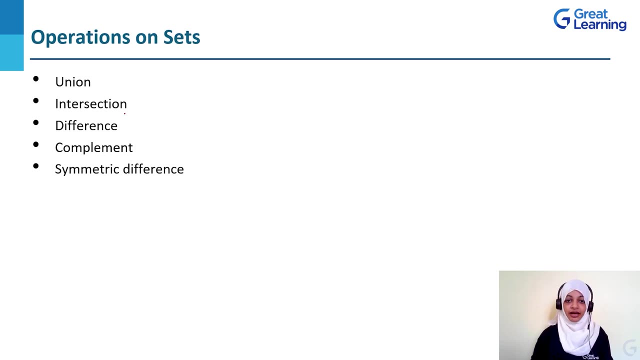 which are the two sets under consideration. That's the difference between universal and power set. So These are some of the various types of sets that are commonly used in set theory. Next let's look at some operations on set Given. here are the five basic operations that are often performed between any two given. 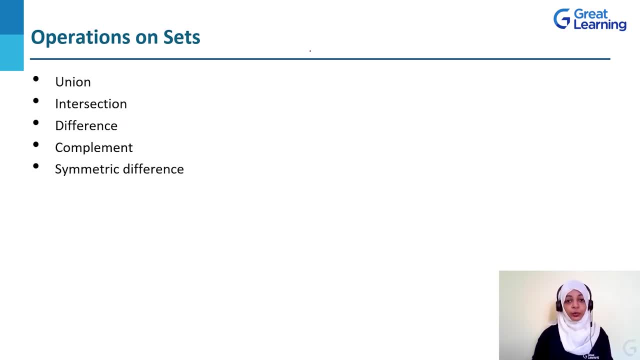 sets. In order to understand these operations, we'll be using a concept known as Venn diagram. A Venn diagram is a very simple concept where each and every set is denoted using a circle and any interaction between these sets are denoted using intersecting circles. in this, 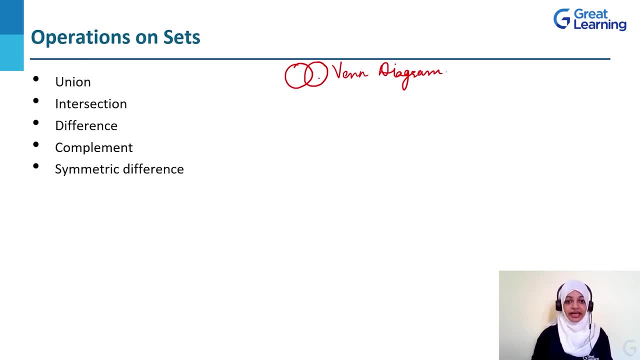 manner, The number of set define the number of intersecting circles. Thus, here in this example, there are three intersecting circles. as shown, therefore, there are three sets. Using the Venn diagram, any area apart from the sets involved is known as not a part of. 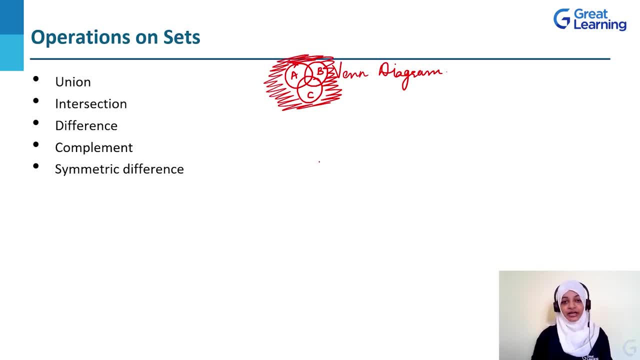 the set. Thus Venn diagrams help us in actually visualizing sets as concrete elements instead of abstract concepts. So now, using Venn diagrams, let's understand the various interactions that occur between any two given sets. For the purpose of this particular topic, let us take two sets as an example, say set 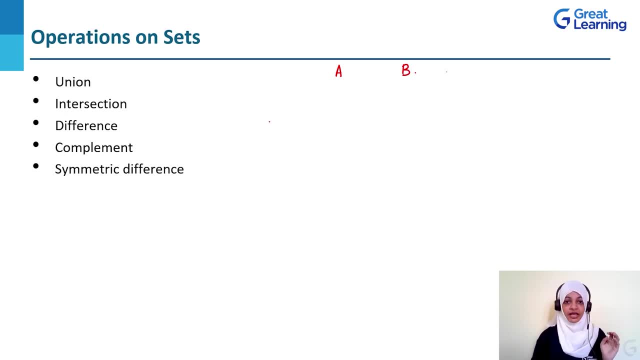 A and set B. As per Venn diagram, the two sets are interacting with each other. Thus we'll have two intersecting circles shown on them. So the two sets here are A and B. Let's take the first operation given here. 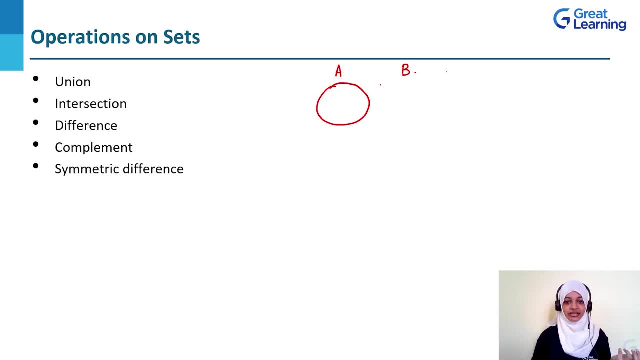 Here is an intersection of these sets, and this is the point of the Venn diagram. It uses the highest and lowest potassium due to the same altimeter. For this reason, it is SUN license here, which is union. Union is an operation that is denoted by a symbol that looks like: 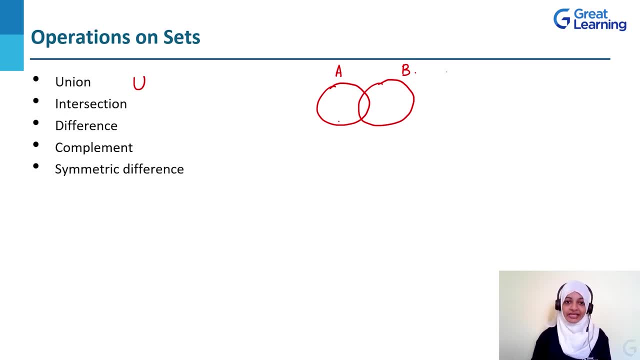 U. A union implies that all the elements of the two sets have to be combined together under one singular set. Thus, if a union operation is performed on A and B, it is denoted by A union B And, as per our Venn diagram, all the components of A will be combined with. 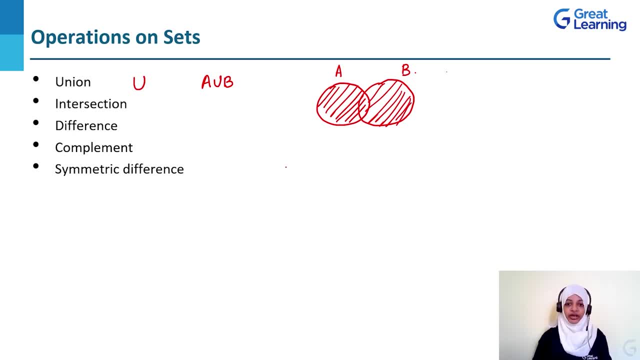 all the components of B in order to give a new set, which is a combination of the elements of A and B. Next, let us look at intersection. Intersection is again an operation that is denoted by a symbol that looks like U, A. union implies that all the elements of the two sets have to be combined under one singular set. Thus, if a union operation is performed on A and B, it is denoted by a symbol that looks like U And, as per our Venn diagram, all the components of A and B- it is denoted by a symbol that 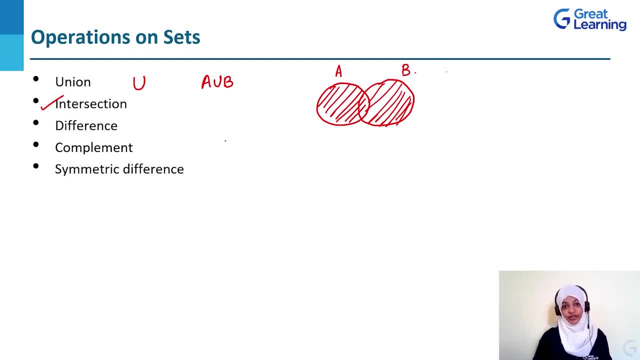 looks like U. Intersection is again an operation that is performed on two sets interacting with each other. The symbol for intersection is an inverted U. Intersection between two sets is denoted as A intersection B. Let us look at the Venn diagram representation of the same. Let us consider two sets, A and B, As per intersection, the intersection operator. 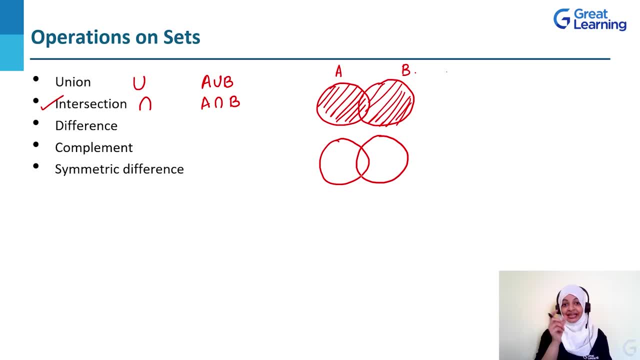 works in such a manner that it extracts the commonalities that are present between any two given sets. As we can see here, there is a certain section between the set A and B, which are present in both set A as well as set B. That is what the intersection operation. 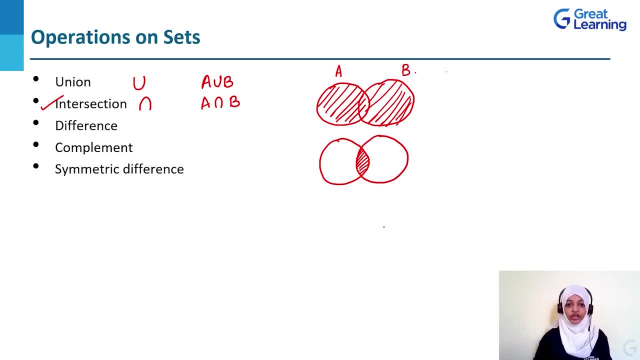 will give as a result. So union operation actually helps us combine all the sets under operation in order to give a new set. Now let us look at the intersection operation. The intersection operator is concerned with extracting the commonalities between all of the sets that are under operation. Next let us look at the difference operator, The. 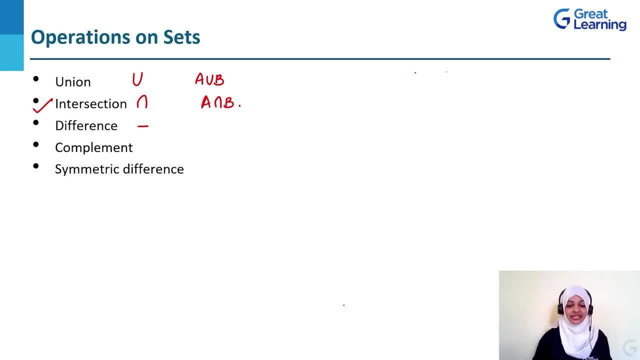 difference operator is denoted with a minus sign. Difference operator is non-commutative in nature. This means that the order of the set matters here. It is denoted as this: set A minus set B, As an example, to understand exactly how the 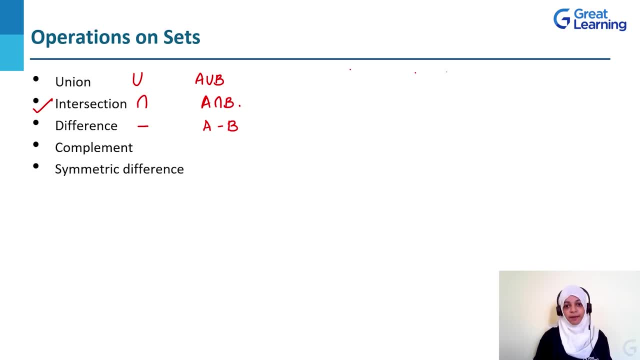 difference operator works. let us create a Venn diagram for the same Suppose. we have two sets, A and B, such that they are interacting with one another. A minus B denotes that we are supposed to take all the components of A, but none of the sets that are under operation. 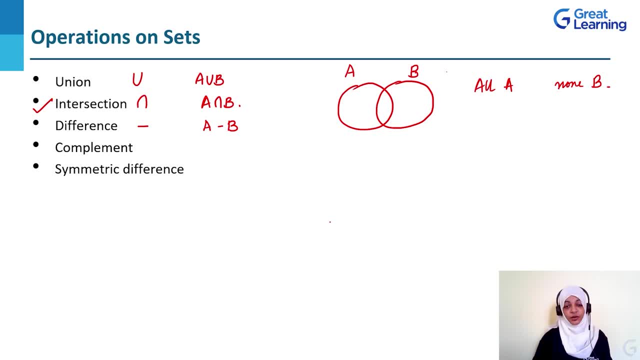 What does this mean? It is actually pretty simple. It means we take all the components of A, but none of the components of B. So, as you can see, the intersecting area between A and B have been excluded. Why is that? Because that section is also a part of B, So that has been completely excluded because we take none of the sets that are under operation. This means that we have taken all the components of A, but none of the components of B. So, as you can see, the intersecting area between A and B have been excluded. Why is? 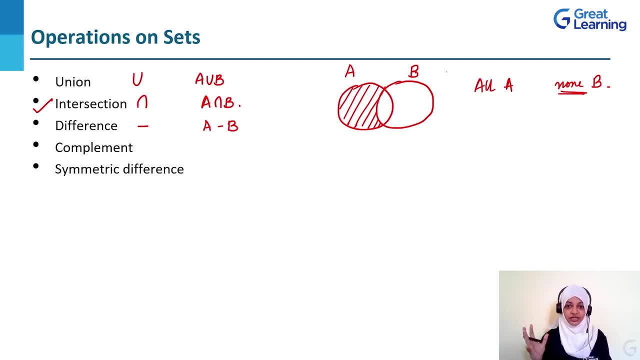 that Because none of the components of A and B have been excluded. So this is how the difference operation works. If we take a look at union and intersection, they are actually commutative in nature, such that A union B would be the same as B union A. Similarly, 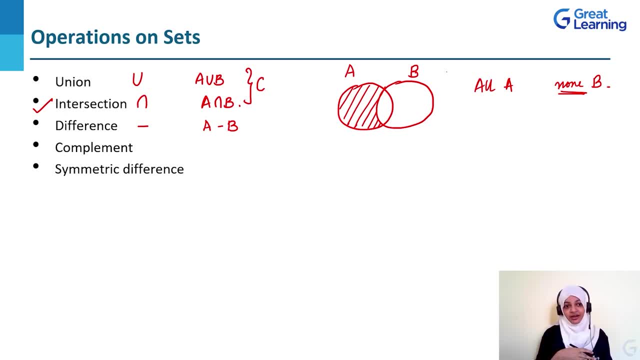 A intersection B would be the same as B intersection A. On the other hand, difference is non-commutative, Meaning that A minus B would have a different answer than B minus A. We can also assume that B is equal to A and A is equal to B. 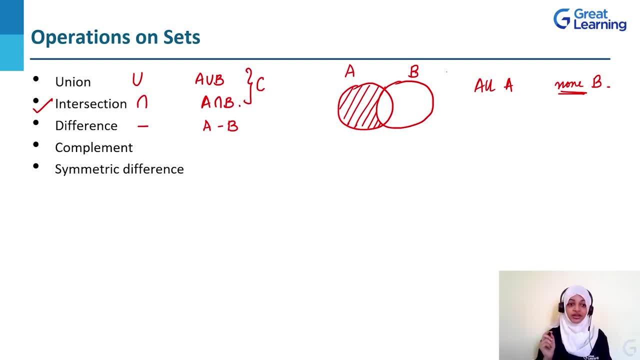 So, in the same way, we take a look at the definition of the recent behavior in this example. For example, if we have a reference of a group of A, let us compare A with a group of A minus a. So be very careful while using the difference operator. Next, let us look at the 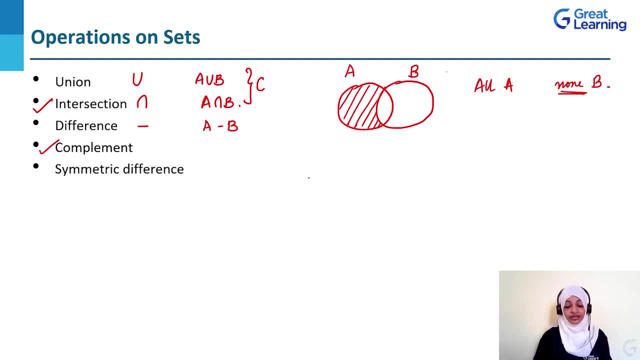 complement operator. The complement operator or the negation operator is actually pretty simple and it's one of those operators that work on a single set only. It is denoted in various ways. At times it is denoted as an asterisk, a simple single asterisk, or in other cases, 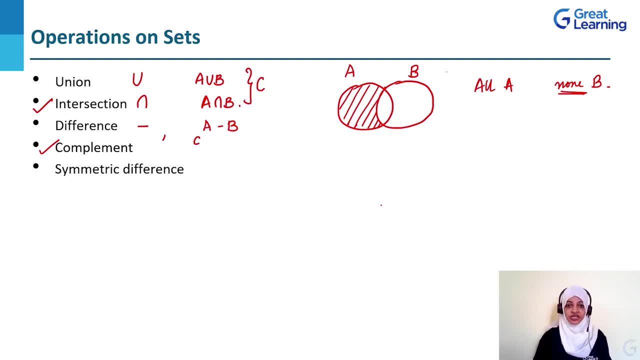 it could also be denoted by a tiny superscript of c. In any case, it means the same thing. Any element which is not a part of the set becomes a part of the complement of the set. For example, let us take a set c. Let c be contained in some superset p. 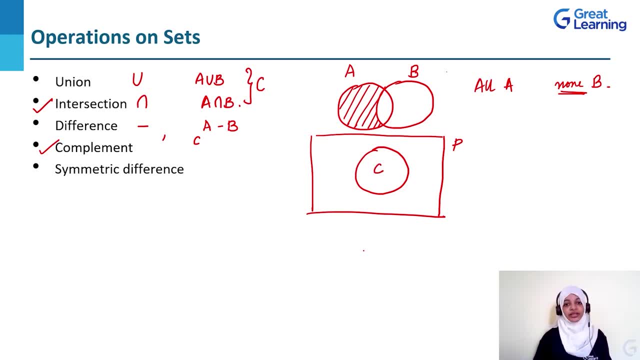 So we've got a superset p and a set within it, c. If we take the operator c, dash or c raised to small c, both of these stand for the complement. Performing this operation will actually give us all of the values that are not a part of c. 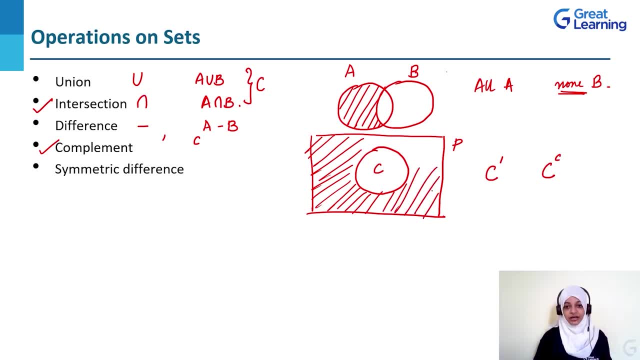 So any value not within the set c will be counted as a part of our complement of c. Lastly, let us look at symmetric difference. Symmetric difference is denoted in various ways. It could be denoted as a delta. it can be denoted as a minus symbol inside a circle. 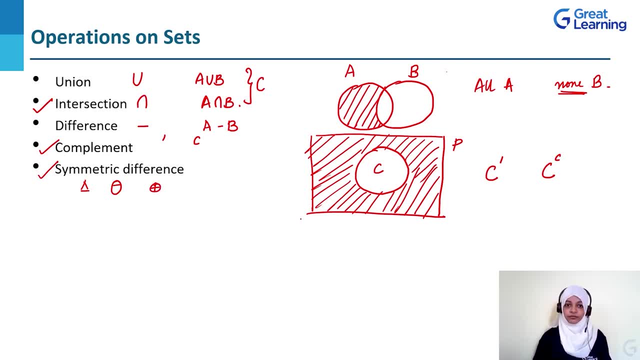 or it can be denoted as a plus symbol inside a circle. All of these mean the same thing: the symmetric difference. Again, symmetric difference is a binary operator, which means that it requires two sets in order to work. The symmetric difference is a binary operator, which means that it requires two sets in order to work. 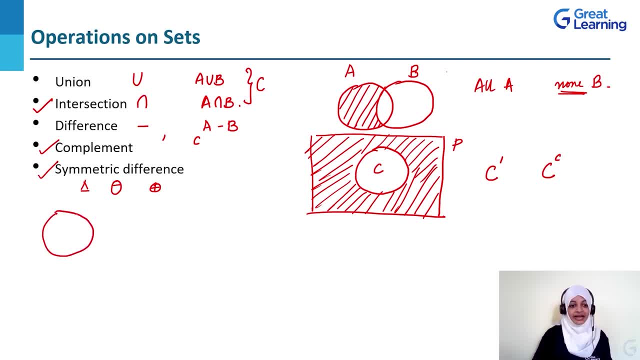 Let's take an example of set a and set b, our favorite two sets. So what is symmetric difference? In order to understand symmetric difference, let us take two sets, a and b, which are interacting with each other. One of the simplest ways of 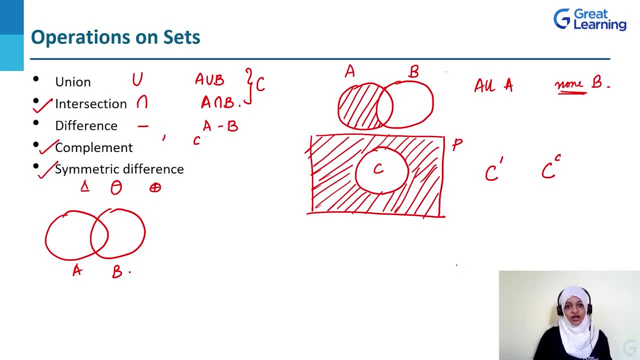 explaining symmetric difference is that it is a combination of union, intersection and difference. As I write down this formula here, you might better understand it. Symmetric difference can be written as a union b minus a intersection b. This means that we are creating a union of a and b and then subtracting the commonalities between. 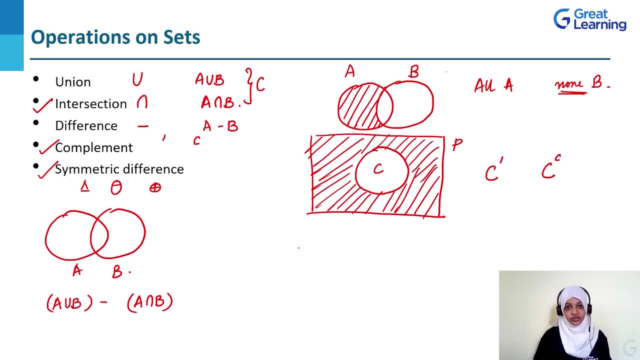 them. Whatever, the result will be the symmetric difference. Let us look at it with different colors. Suppose a union b is the area which I am shading currently with dark green. Now let us take a intersection b. A intersection b would be the area that I am coloring with blue. 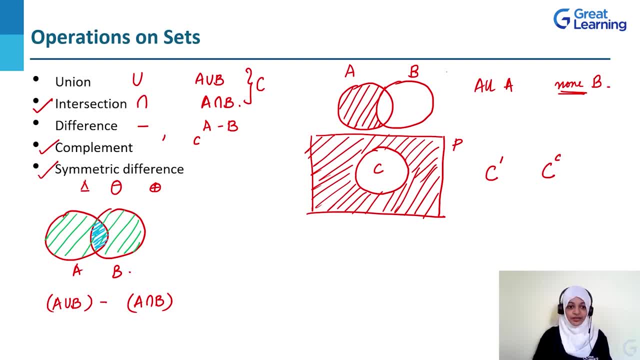 As you can see, the blue area has to be subtracted from the green area. As such, what we will have is something like this: We will have the two sets, a and b, such that all of the elements of a will be considered and all of the elements of b would be considered, but all the elements which 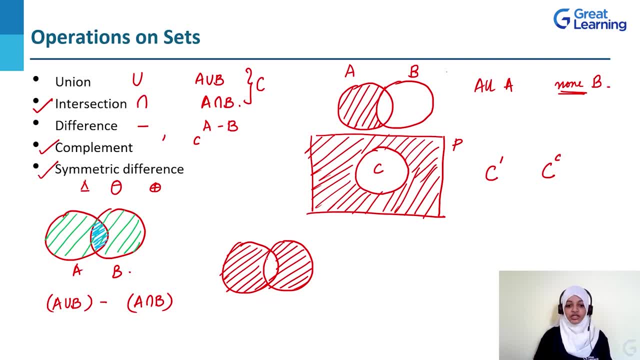 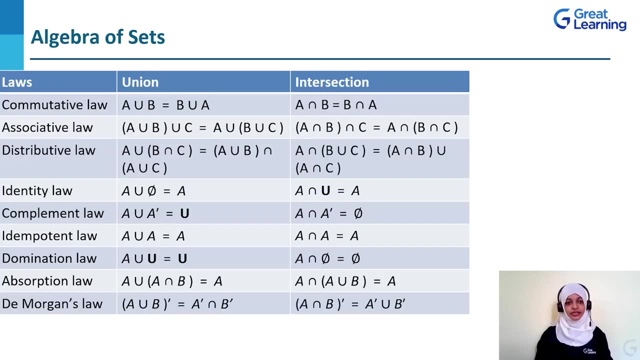 are there in both a and b would be excluded. This is what symmetric difference does. Thus we have seen all of the various operations. Now let us look at the algebra of sets. The algebra of sets is actually a certain number of laws that are formulated by using the various 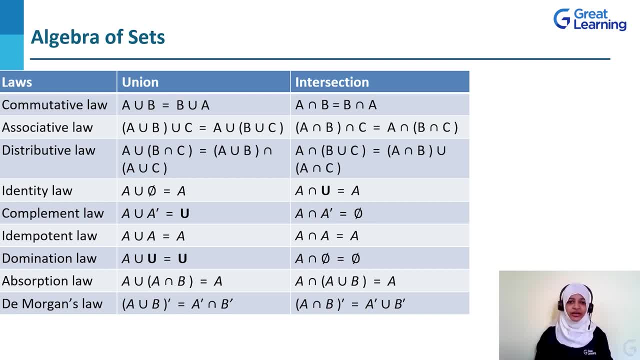 operators that we have seen previously. These are quite logical in nature, meaning that if you use a Venn diagram, it's easy enough to understand how these are working. Some of them we've already seen. Actually, one of them we've already seen, which is the commutative law. 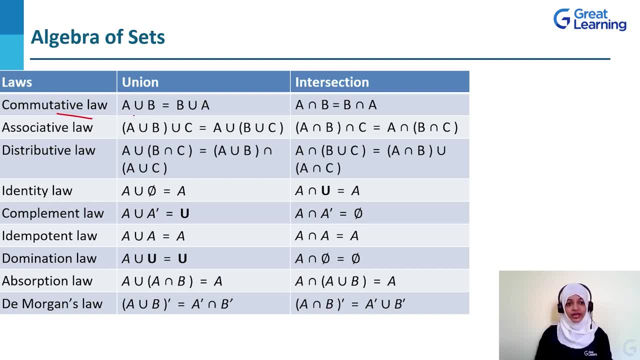 The commutative law is extremely, very simple: A union B is equal to B union A. Similarly, on intersection A, intersection B would be the same as B intersection A. The logic behind it is pretty simple: Any two sets would give you one set, irrespective of how you combine all of the elements within. 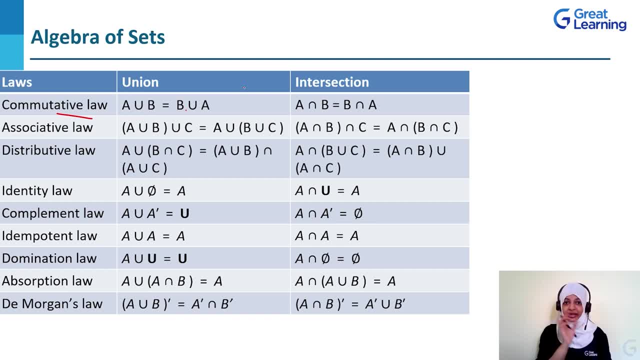 them. Similarly, while taking the commonalities between any two sets, you would always have the same commonalities, irrespective of whether the set A is first or the set B is first. The next law we have here is the associative law. How do we associate any two or three sets based upon the union, as well as the intersection? 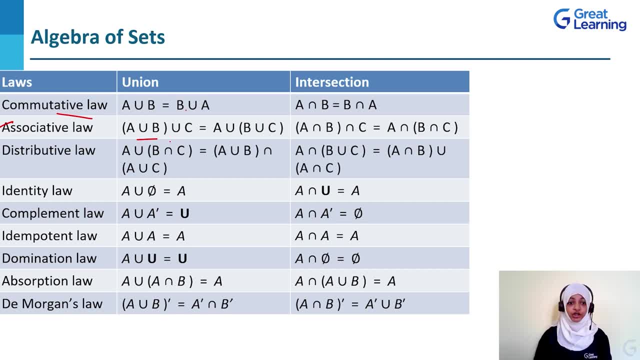 operator. So A union B, union C would be the same as B union C, A union B, union C. Similarly for intersection A, intersection B, intersection C will be the same as A intersection B, intersection C. Next we've got distributive law. 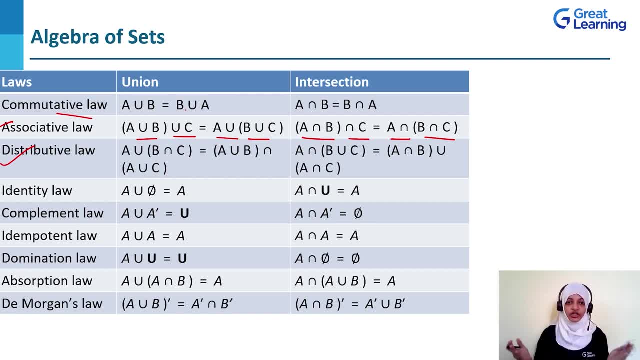 How do we actually split up a certain equation on the basis of the operators within that equation? The distributive law is often given as a combination of union and intersection. So here we have a combination of union and intersection. So here A- union, B, intersection C will be written as A union, B, intersection A union. 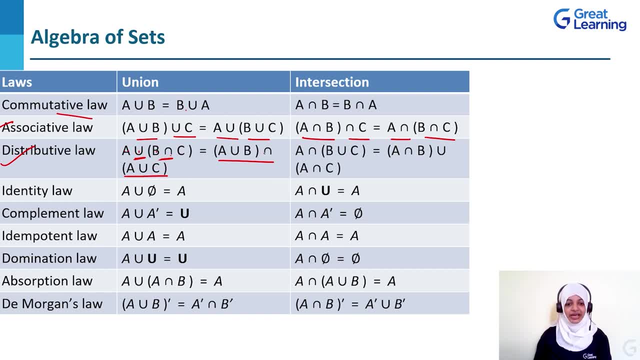 C. as we can see here, A union B, intersection A union C. Similarly, for our intersection the distributive law follows the same pattern. A intersection of B union C will be equal to the union between A intersection B and A intersection C. 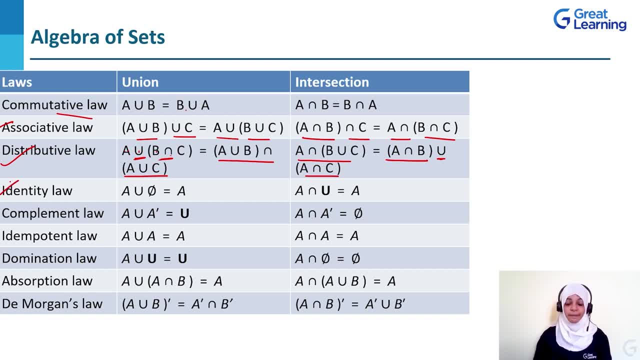 Next we've got the identity law, which is based upon the union and intersection of any set with the union and intersection identity sets. Now, what is an identity set? From basic mathematics, we already know what identity values are. Identity values are all of those values that maintain the integrity of whichever other. 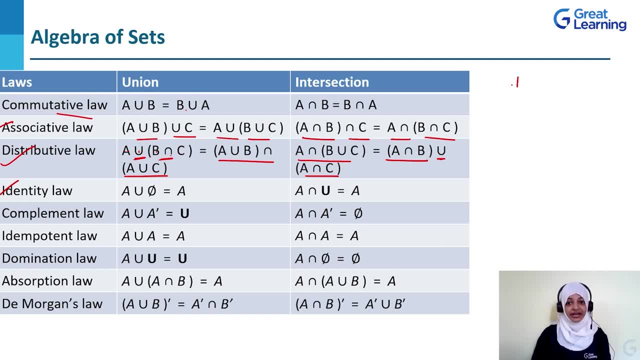 operand interacts with them. So, for example, for addition, the identity values are like this: So, for example, for addition, the identity values are like this: the identity value is 0.. Whereas for multiplication the identity value is 1.. 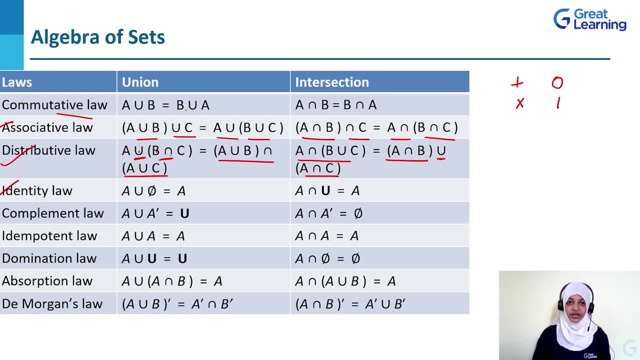 Adding anything with 0 will give back the same element. Similarly, multiplying anything with 1 would give us the same element. Similarly, the identity element for union is the null set. Union of anything with the null set will give back the initial value, And for intersection, 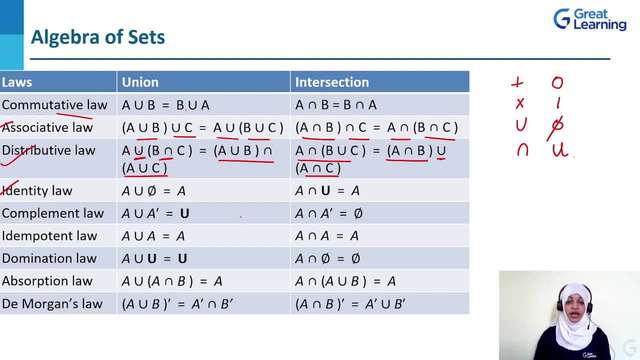 we've got the set, which is our universal set, Because the commonalities between a set and its universal set will be the set itself. Right? Thus we have two separate identities here, Namely A union phi gives us A and A intersection U gives us A. 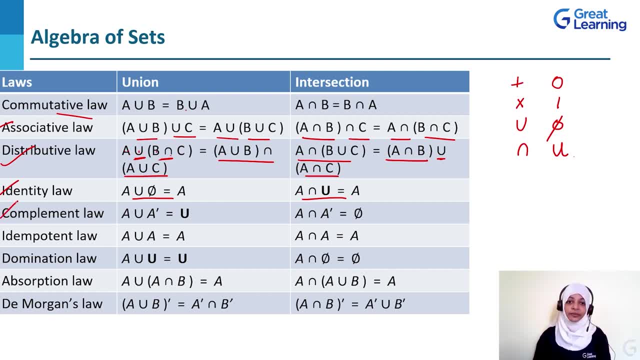 Next, let's look at the complement law. The complement law is based upon. what will the result be If a union of a set is performed with its complement or the intersection of a set is performed with its complement? Union of a set with its complement will give us the universal set. 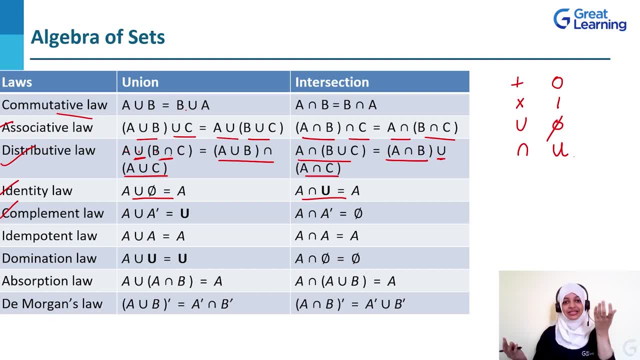 And why is that? Because if you take the set A and you add it or you union it with all of the values that are not a part of A, we would actually get the whole set That was under consideration. Thus, the complement law, in terms of union, gives us U as the final. 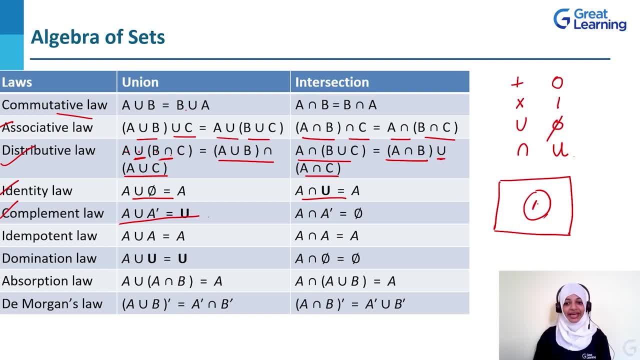 answer, which is the universal set. On the other hand, if you take a set and you perform an intersection with the complement of the set, there are no commonalities between them. That means there would be a set which is empty. Basically it would be a null set. Thus, intersection of A with 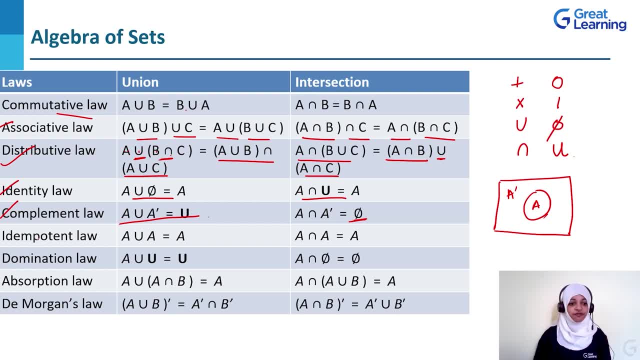 its complement will give us the set. And if you take a set and you perform an intersection with the complement of the set, that gives us U as the final answer, which is I Here we have. the Idempotent Law states that the union of a set with itself gives. 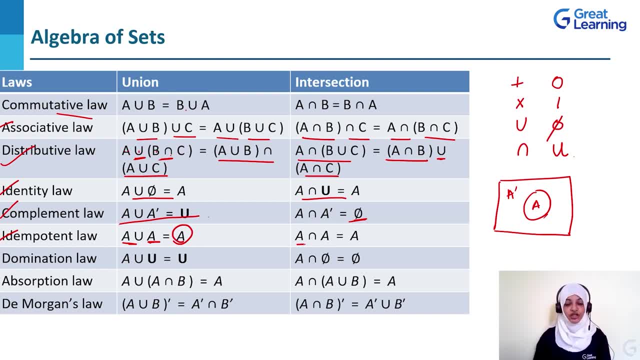 us the set back. Similarly, the intersection of a set with itself will give us the set back. The Domination Law states that two sets that are in union or intersection with each other would have aathlonation of one set over the other due to some property quality. Therefore, 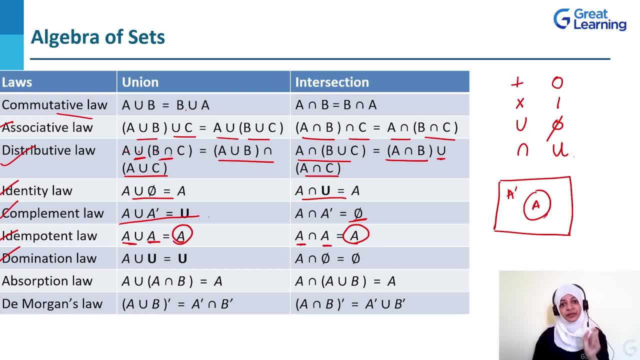 soberness would benumbered by 1 over 0.. to some properties of this dominant set, For example, here we've got the union of A with its universal set. Union of A with its universal set would give us back the universal set itself. 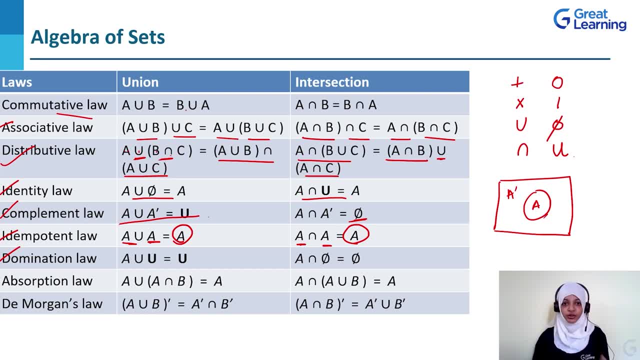 because A is, after all, a part or a subset of its universal set. Similarly, intersection of A with a null set would again be null, As we can see here. in both cases A has disappeared from the final result. That is because, in the case of union, the universal set is dominant. 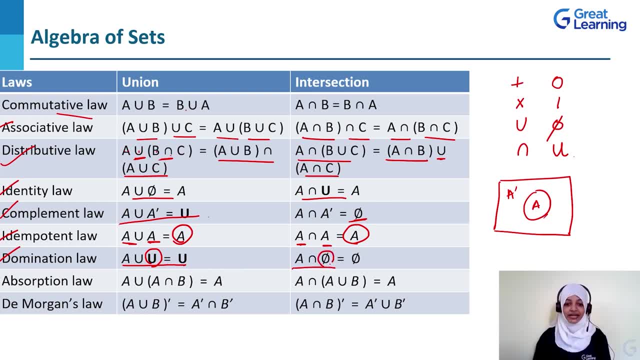 and in the case of intersection, the phi set has become dominant because of their intrinsic properties. Next we've got the absorption law. The absorption law is pretty simple: When two sets interact with each other in a certain manner, one of the set completely. 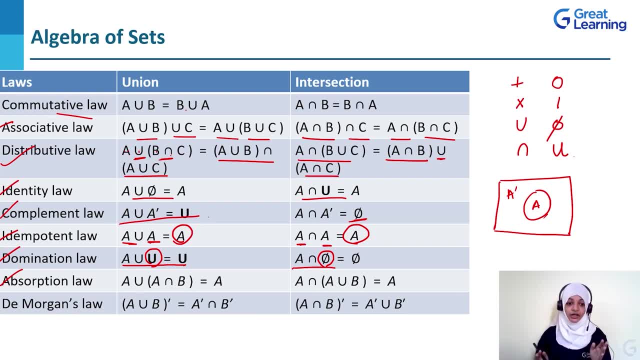 disappears from the resultant set. Here we've got an example of two sets, A and D, which are actually interacting with each other. Let us understand the absorption law with an example. Let's create a Venn diagram such that we've got A intersection B, The Venn diagram of. 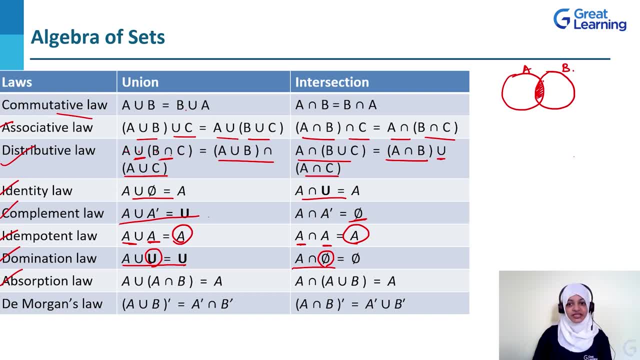 A intersection B would give us A intersection B. We've got A intersection B. We've got us this specific value between A and B. Next, let that particular set be unioned with A. If we union this particular set with A, we'll get back A. Why is that? Because that intersection. 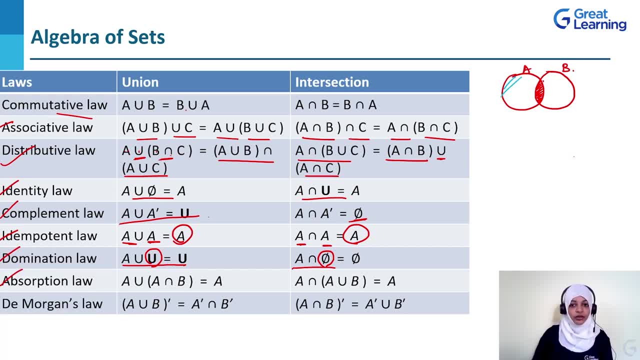 is already a part of A. Unioning it with A will actually lead to complete disappearance of that part, and what will be left with us would be the whole set A. As you can see, we've got no components of B here involved. We've got a whole A set. That means the set B, which 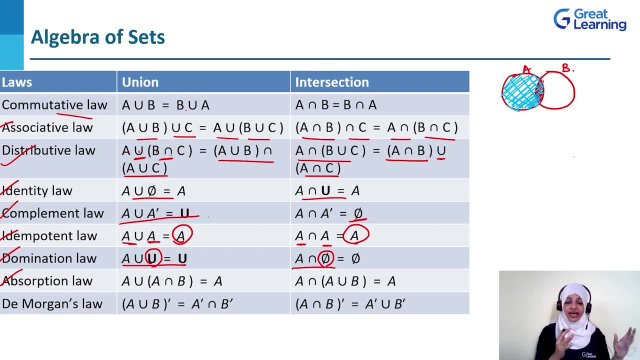 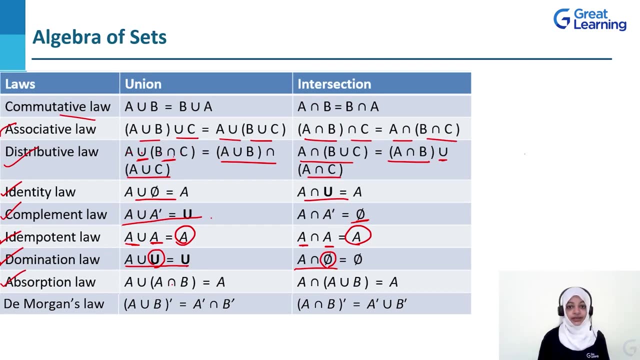 was initially there as a part of the equation, has now disappeared completely or has been absorbed into the equation itself, thereby giving the resultant set as only A. A similar Venn diagram can be created for the intersection of A and B. Thank you. Lastly, let's look at the De Morgan's law. The De Morgan's law is actually a combination. 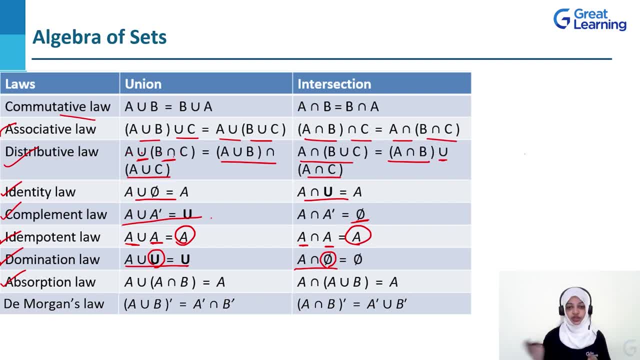 of union with complement or intersection with complement. Let us understand the union identity of De Morgan's law with the Venn diagram. Consider a universal set U with two sets, A and B, inside it which are interacting with each other. If we perform the operation A union B, this operation actually provides us with this particular 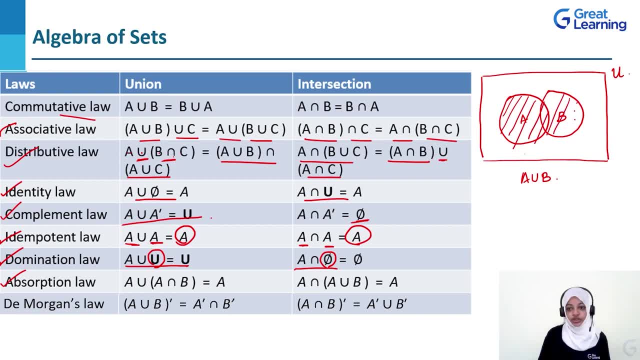 area, As a normal union operation would do. negation of A union B would provide us all of the rest of the elements that would be a part of U but are not part of A union B. That is shown as the blue shaded area. So now we'll look at the De Morgan's law. We'll 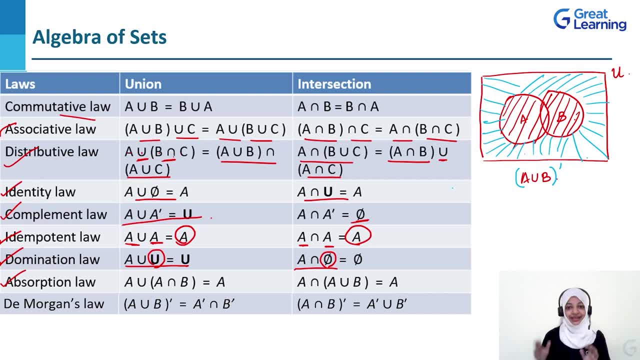 take a look at it in a minute. Let's take a look at it in a minute. This is a normal union operation. This is a general union operation. This is a union operation. This is a normal. So now we've seen the exact area that is supposed to be the output of the De Morgan's. 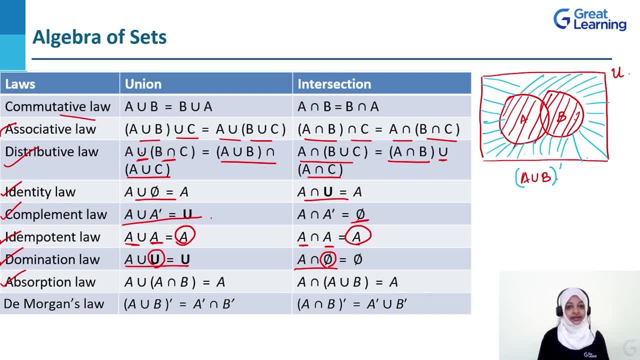 law. Let us see if the union identity of the De Morgan's law's right hand side also provides us with the exact same output. Let us consider A dash. A dash will be shaded in orange, As you can see. A dash is all of the elements which are not a part of A. 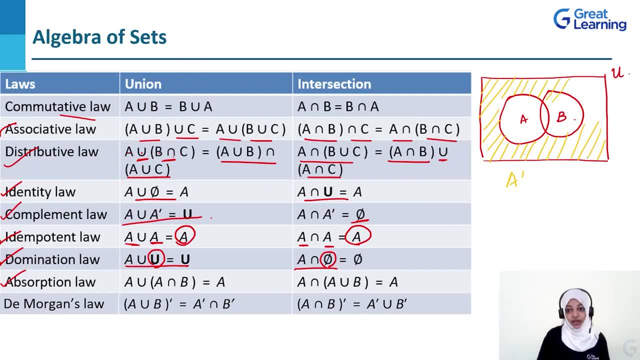 So any element which is not a part of A, including the set B, would be included within this A dash section. Similarly, the B dash section will contain all the elements which are not a part of B. This implies that the set A is also going to be a part of this particular B dash set. 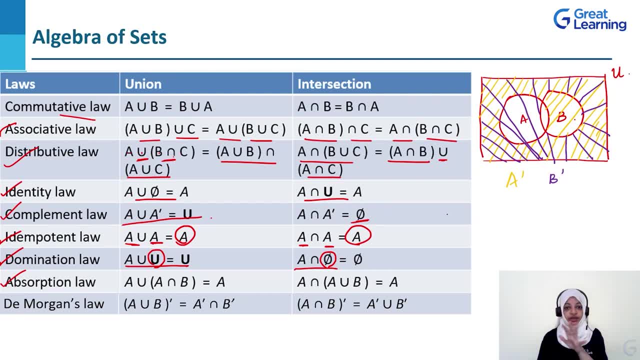 So, As you can see, we've got two shaded colors here. We've got the purple lines and we've got the orange lines. Taking an intersection of A dash and B dash will actually give us the common area where we have both the orange as well as the purple lines. 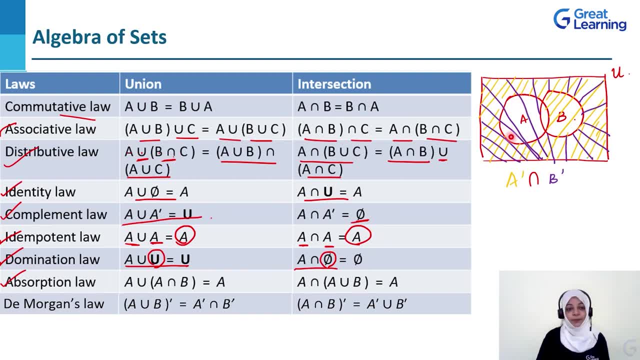 As you can see, the set A has only purple lines, whereas set B has only orange lines, And all of the area within U apart from the set A and B has a combination of both purple as well as orange lines. If you remember the previous diagram properly, you will note that this is actually the area which was shaded as blue previously, denoting A union B complement. 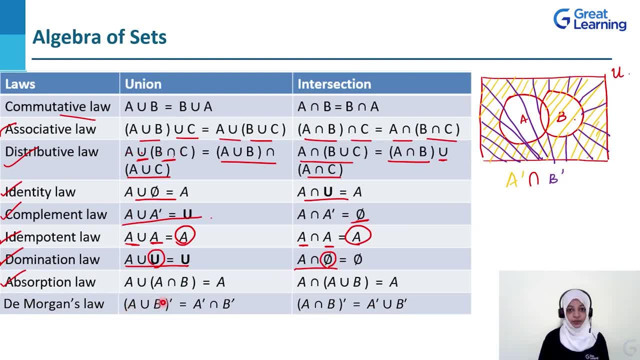 Thus we've seen that A union, B complement is equal to A complement, intersection, B complement. Thus we've proven, using the Venn diagram, that the De Morgan's law for union holds. In a similar manner, you can also prove the intersection identity for De Morgan's law. 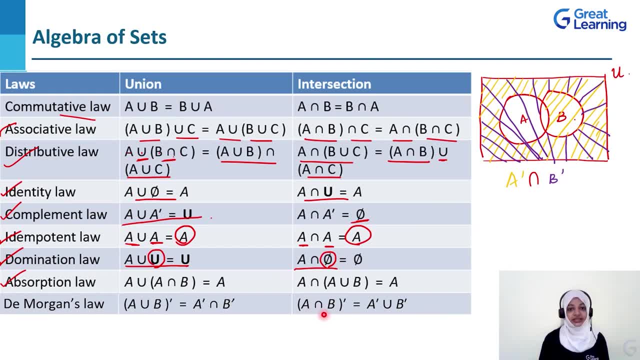 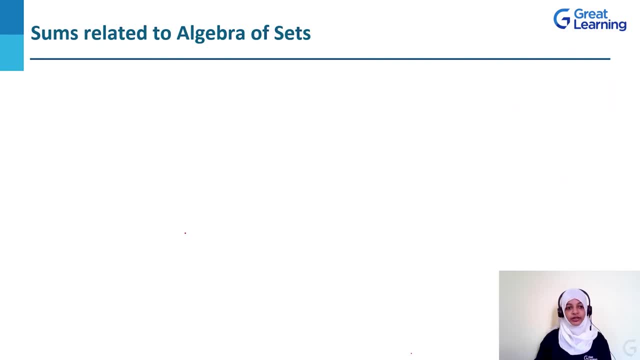 The intersection identity states that A intersection, B complement is equal to A complement, union, B complement. Let us now look at some of the sums which are related to algebra of sets. So suppose this is our first question. The question here is very simply stated. 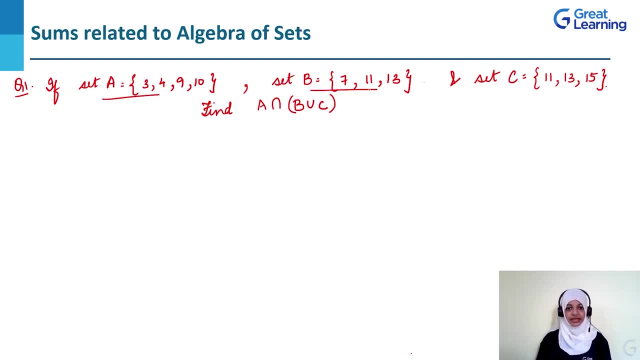 We've got three sets- set A, set B and set C- And we need to find out what the value of A, intersection B, union C is. Let us first understand how we can resolve this question. It's a pretty direct question based completely upon the distributive property. 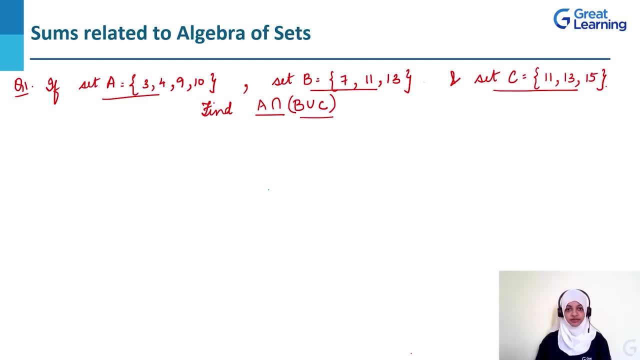 The distributive intersection intersection property, to be specific, as per the distributive intersection property, A intersection B, union C can be resolved by distributing based upon the operators here. As a result, it will give us A intersection B, union A, intersection C. 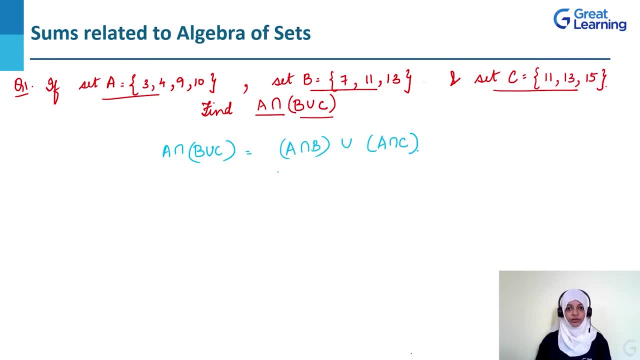 Using this formula, we can resolve this particular problem Very easily. First, consider the first part of the equation here: A: intersection B. Considering the two sets A and B, when we try to find out what the intersection between them is, we find that the intersection between A and B is null. 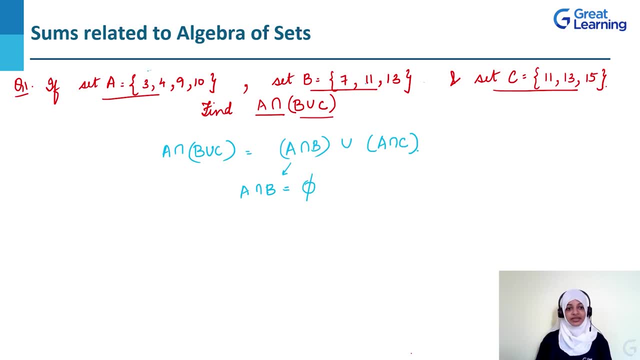 Why is it so? Because there are no common elements between the set A and the set C. When we try to find out the commonalities between A and C, we find that again, A intersection C is equal to null, Because there are no commonalities within the elements of the set A and C. 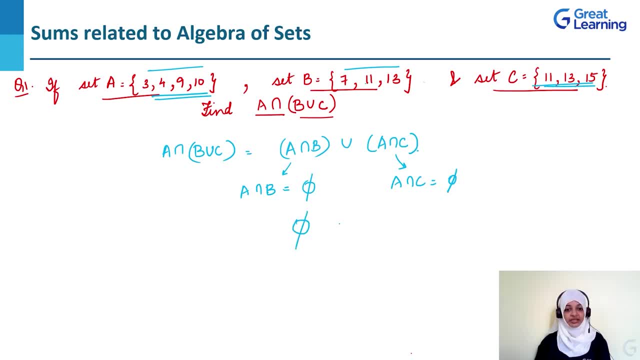 As a result, unioning the two elements given here, we get the final answer as NULL. As a result, we can say that A intersection B union C, for this particular example, is equal to an empty set. Next let us look at the second question. as stated here, 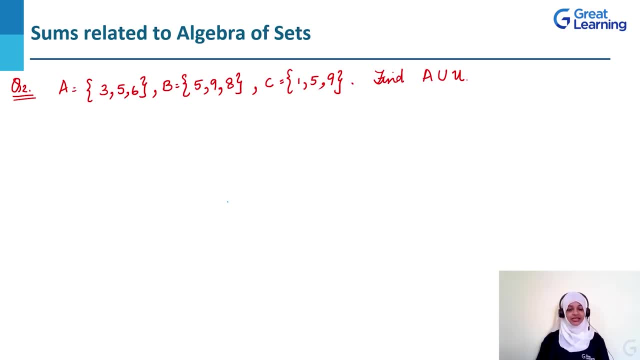 Let there be three sets: Set A, Set B and Set C. Using these three, we need to find out the union of A with its universal set. Now, as per this equation, we can say that For our laws in algebra of set, we know that A union U is going to give us U itself. 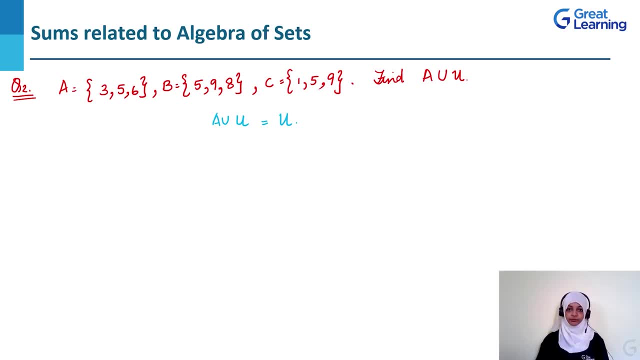 This is due to the domination law under union. The issue here is not how to resolve this. The issue would be: how do we find the universal set? Finding out the universal set is very simple if we remember the definition of universal set. As we already know, universal set is the set containing all of the sets that are currently under consideration. 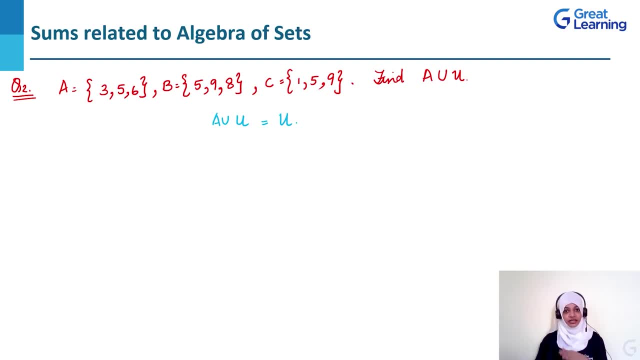 So the pairing set of the sets currently under consideration would give us our universal set. So let us see what U actually is. Consider the three sets given here: set A, B and C. Put all of the elements of set A, B and C into one single set. 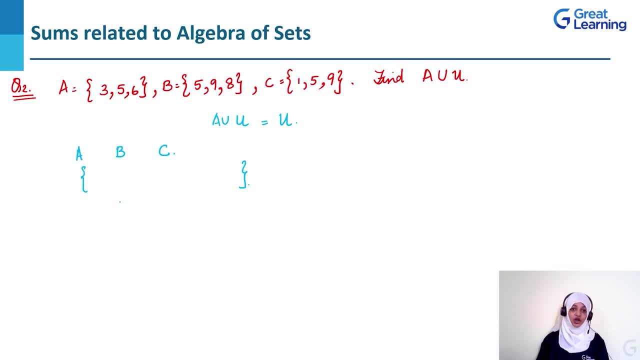 Please make sure that you do not repeat elements. If they have occurred once, leave them in as is and do not repeat them. Consider set A. 3,, 5, and 6 have never been repeated, So we have included them into the new set as is. 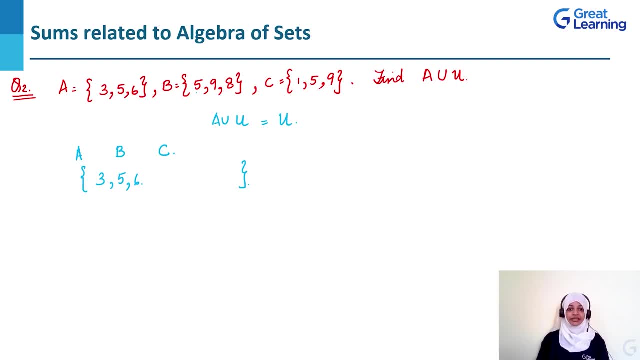 Next consider set B. The first element in set B, 5, has already been included in set A. Ignore it for now. Next we have got elements 9 and 8, which have not previously been included in the set. 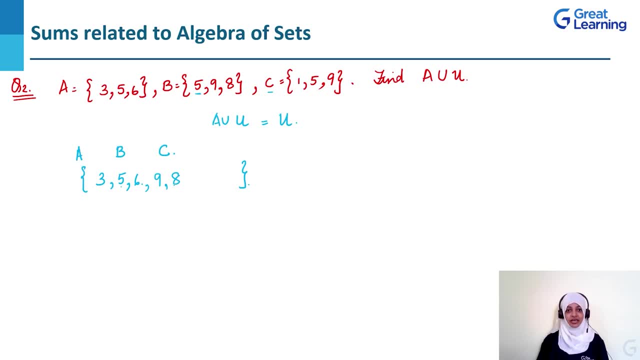 Do so. Lastly, we have got set C, which has three elements: 1,, 5, and 9.. The first element, 1,, has not previously been included in the set Included. 5 and 9 already exist in this set. 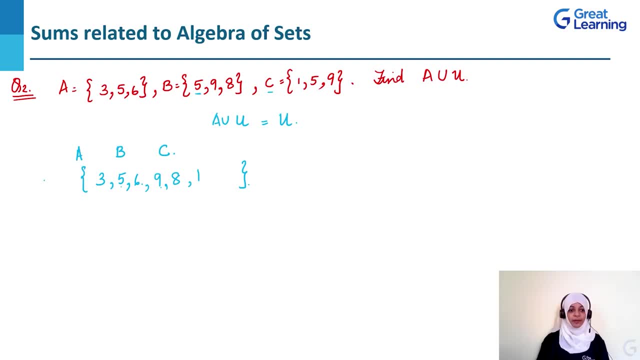 Included. As a result, we are ignoring them. This becomes our universal set. As a result, while carrying out the operation A union U. our answer would be 3,, 5,, 6,, 9,, 8, and 1,. 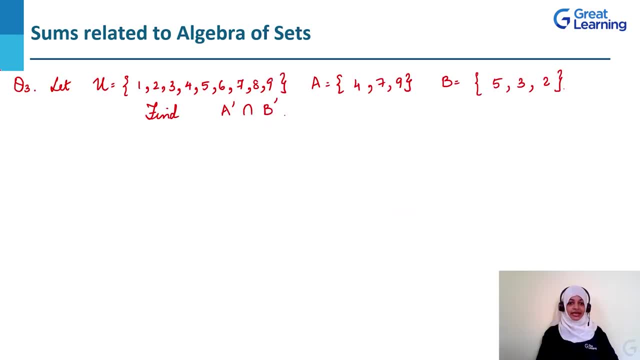 which is actually the universal set. Lastly, let's look at this third example for algebra of sets. Let there be a universal set. Let there be a universal set which contains elements from 1 to 9.. Let A be a subset of this universal set containing 4,, 7, and 9.. 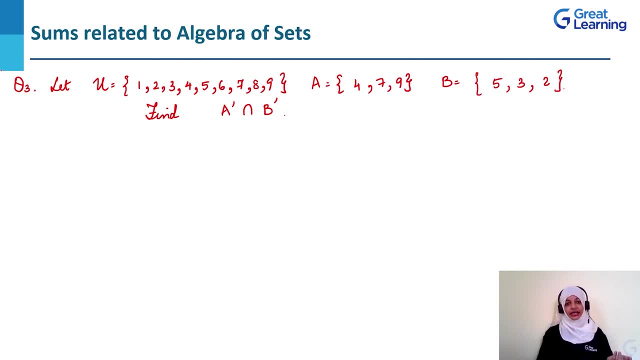 And let B be an other subset of the universal set containing 5,, 3, and 2 as its elements. What we need to find out is: A complement intersection, B- complement. This actually looks pretty familiar to one of the formulae or laws that we've already seen in algebra of sets. 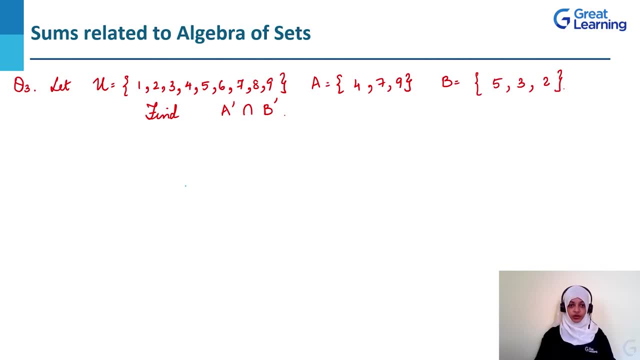 That is the De Morgan's law. As per De Morgan's law, A union B's complement is equal to A complement intersection B complement. So a simple way to find out A complement intersection B complement is to find out A union B and complement it. 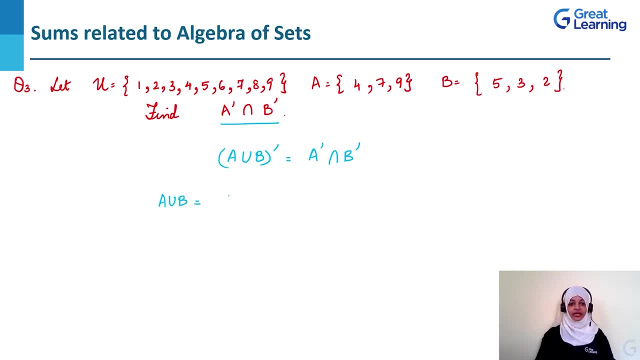 Let's find out what A union B is. A union B is equal to all the elements of A with all the elements of B in a non-repeating manner. Complementing this would actually give us all of the elements that are a part of U. 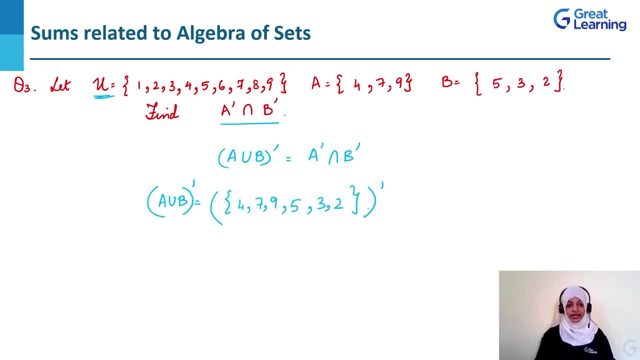 but are not a part of A union B. Therefore, A union B complement is equal to 1,. 2 and 3 are a part of A union B. 4 is also a part of A union B. 5 is a part of A union B. 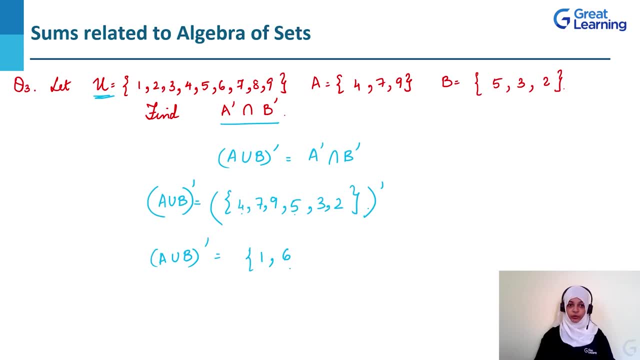 6 is not a part of A union B, thus it will be included into the set. 7 is again a part of A union B, 8 is not a part of A union B and 9 is also a part of A union B. 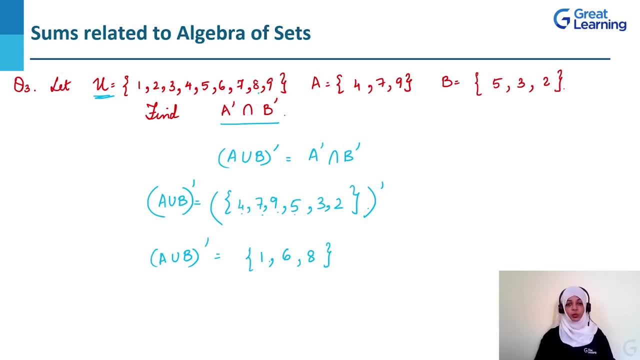 Thus our complement of A union B becomes 1,, 6,, 8, and that is what A dash or A complement, intersection, B complement actually is. Thus we've seen three examples of how algebra of sets. I'll repeat this. Thus we've seen three examples of how laws within algebra of sets. 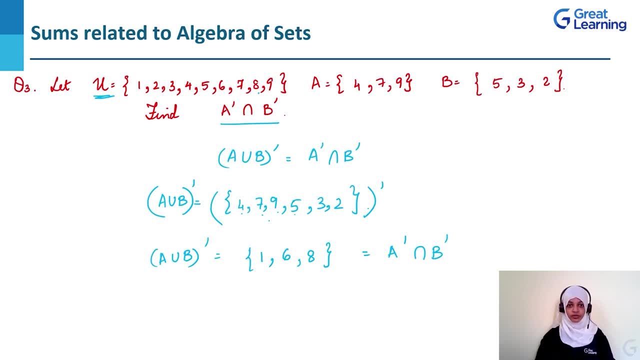 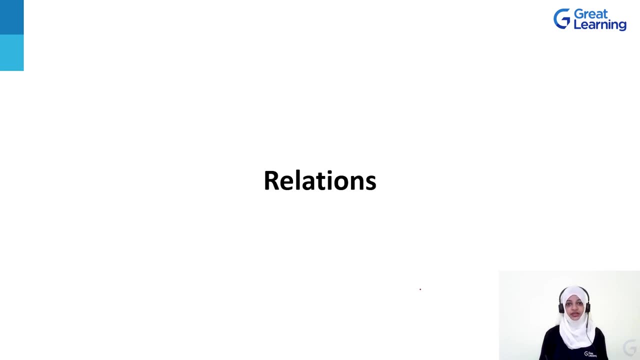 can be used to resolve set-based problems. Thank you, Hello everyone. Let's start with the second concept in our series for basics in discrete mathematics with the topic of relations. Relations are an important concept of discrete maths because its applications are often seen in subjects such as functional analysis. 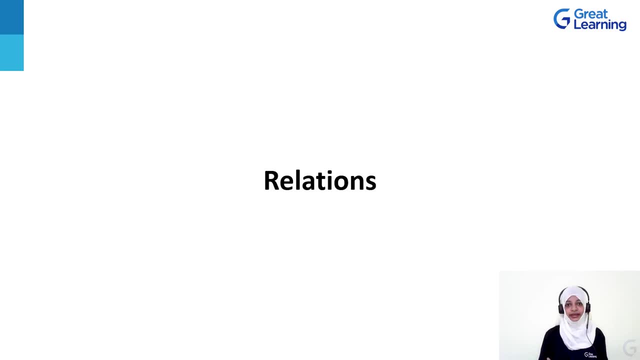 which is a very important part of any kind of environment building. Functional analysis is actually a pretty simple way of trying to understand how a certain variable works in a microenvironment and then extrapolating and predicting its behavior in a macroenvironment. Thus, relations in coordination with sets. 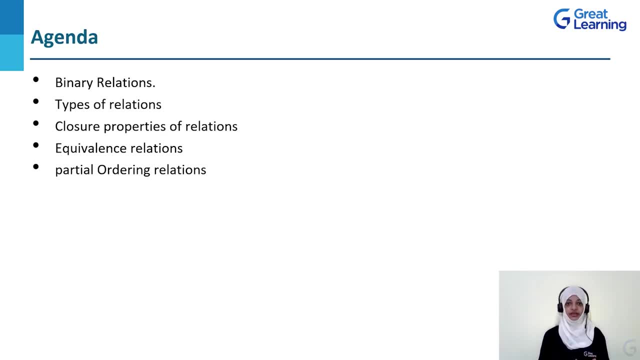 in this particular session, we're going to understand what binary relations are, what are the components of binary relations and how do they work with one another. We're also going to look at the different types of relations that are commonly utilized within set theory. 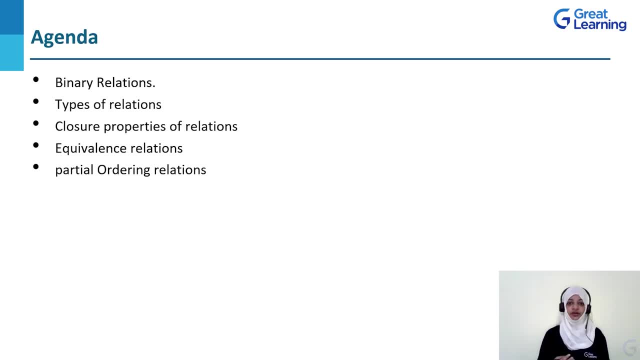 Next, we're going to look at the closure properties that are a part of relations, wherein we'll see how a relation can actually be closed on three different levels. Next, we've got a specialized type of relation known as equivalence relation and partial ordering relation. 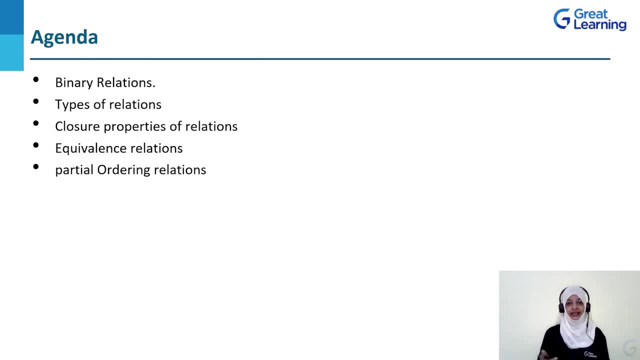 Why they're special and how they're special will be seen and illustrated with the help of some examples. So let's get started. A binary relation, often known just as relation, is actually just a connection between any two elements of two separate or the same set. 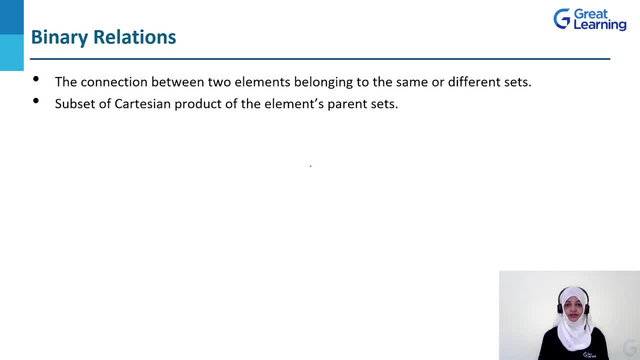 Now what do we mean by separate or the same set? The reason behind this term separate or same set is actually because relations can either exist between two different sets or they can exist within the set itself. So that means the relation would be from the set to itself. 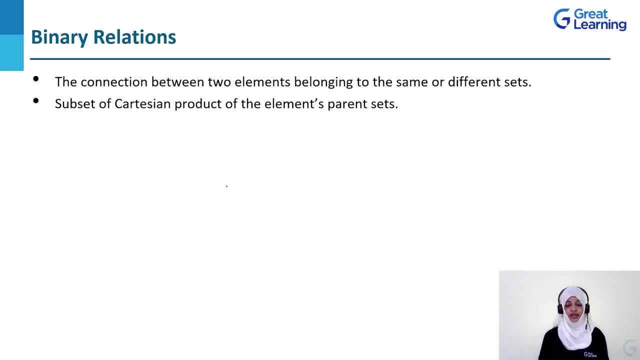 Let us understand this with an example. A relation, often known as R, is defined by some functionality passing from one set to another, such that one element of set A is in relation with one element of set B. Thus we say that there is a relation. 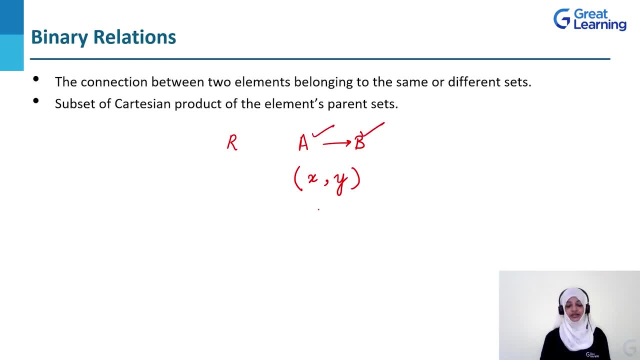 between two separate sets. Similarly, a relation R can be defined as going from set A to itself, such that both x and y are part of the exact same set. Thus you can see how the relation can exist between two different sets or the same set. 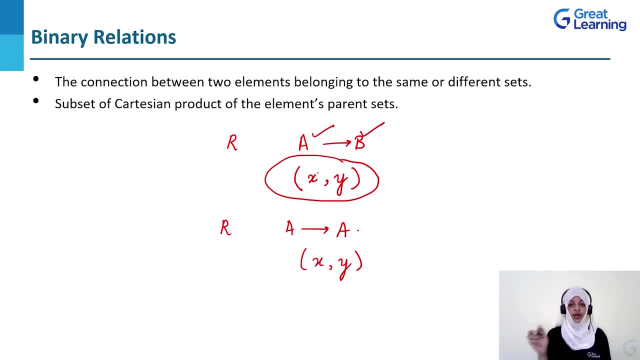 Now the pair given here is actually a relational pair. One element of A has been related to another element of B. This type of clubbing between the two elements of the sets which are related to each other is known as an ordered pair. In any relation, there could be multiple. 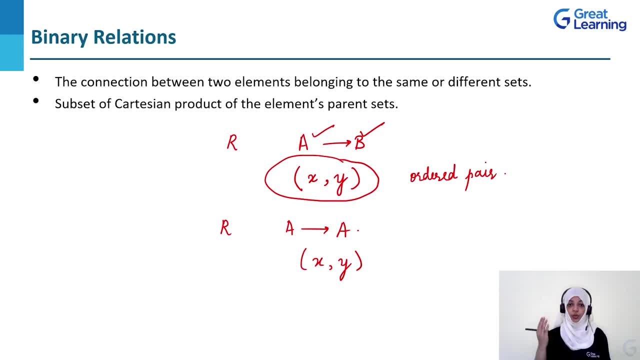 or no ordered pairs, depending upon what sets the relation are set upon and what defines the actual relation. At the end of the calculation, the answer for any relation that we obtain is going to be a series of ordered pairs. This series of ordered pairs- 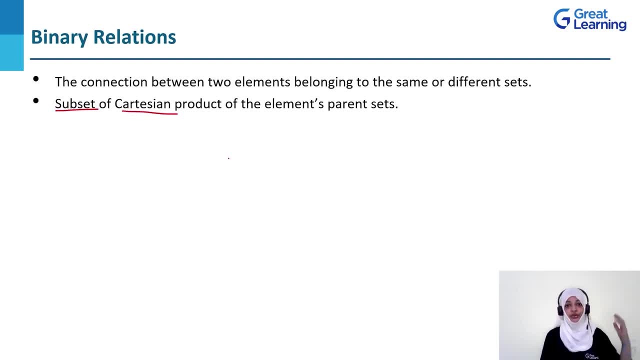 would be a subset of the Cartesian product of the two actual sets on which the relation is acting. Let us understand this with an example. Let there be a set A such that A contains the elements A, B, C and D. Let there exist another set B such that 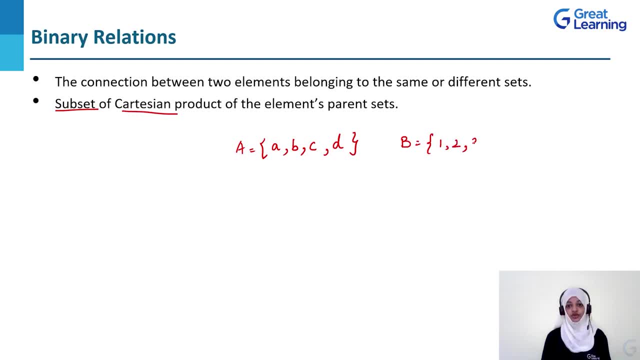 B contains the elements 1, 2 and 3.. Let there exist a relation between A and B such that each and every element of A has to be matched up with a similar positioned element on B, What we are essentially going to do here. 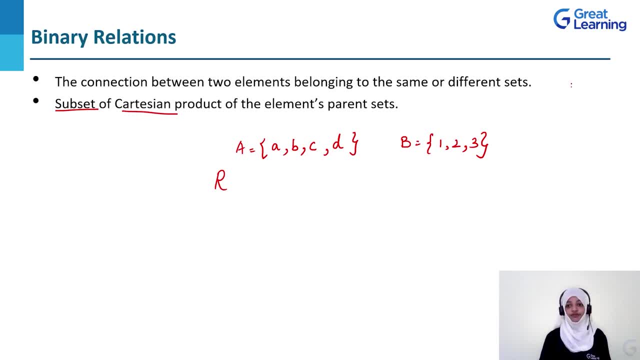 is that we are trying to match up all of the A's with the 1's, the B's with the 2's, the C's with the 3's, and so on and so forth. Why is that? Because the relation that we have defined. 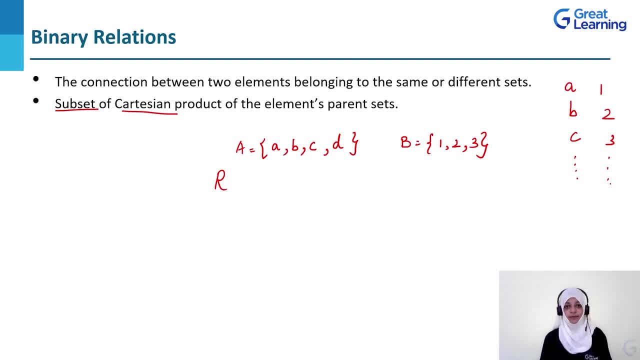 is actually saying that the positions of the elements must be the same, not that the values must be the same, So in their own set of alphabets or numbers, if the position of that element is the same in relation to the other elements, 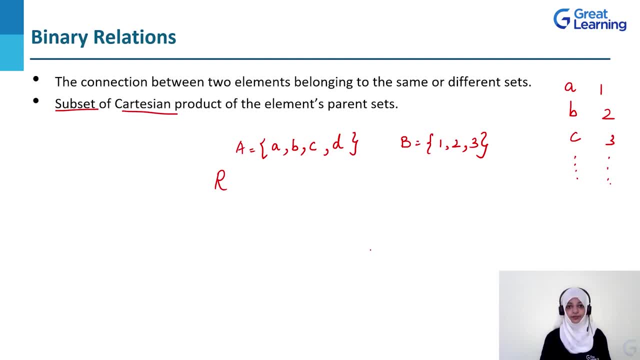 then we are simply going to match them up and put them in the relation. In order to understand this, let us first take the Cartesian product of set A and set B. Now, what is a Cartesian product? Cartesian product is just a pairing of every element of one set. 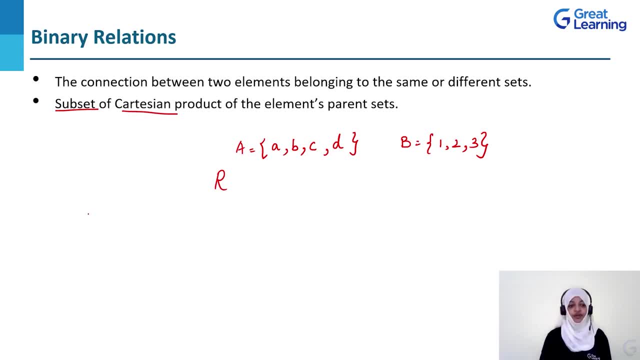 with every element of the other. In this example, we've got element A, B, C and D, and we are supposed to pair them up with 1,, 2, and 3. This would provide us with a Cartesian product. 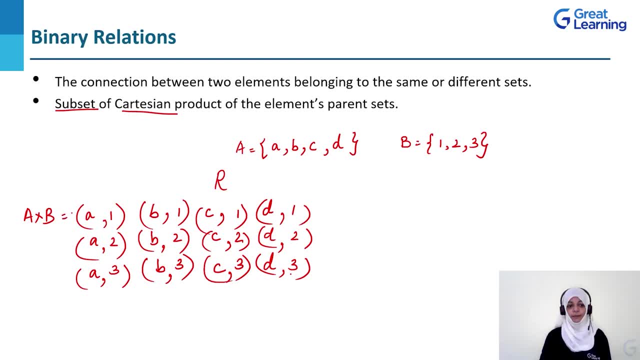 Does? the Cartesian product of set A and B, denoted by the cross symbol, would look something like this, wherein each element of set A has been related to each element of set B. There is no discrimination here. Every element of set A has to be linked. 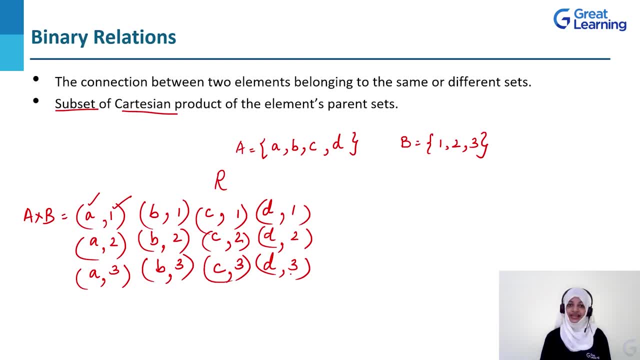 with every element of set B, But in a relation that is not possible because there are certain guidelines that have to be followed while we are actually setting up the relation. Now let us look at what would possibly be the answer. when we look at the relation. 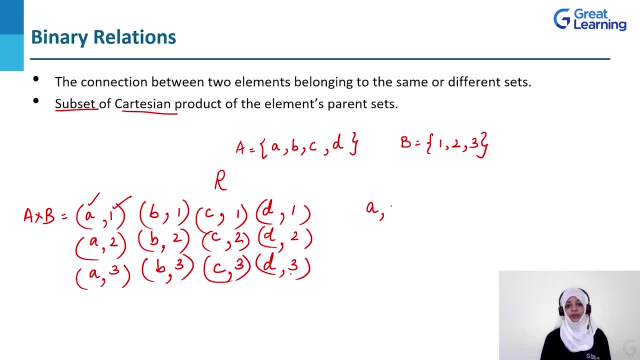 We can see that A can only be clubbed with 1.. The reason behind that is because A and 1 are similar to each other, such that the position of A in alphabets is the same as the position of 1 in natural numbers. 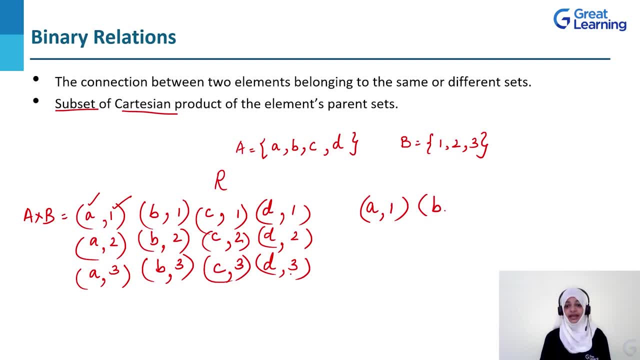 Next, if we take element B, B will be related to 2.. Next, taking element C, C would be related to 3.. Next, element D does not have any corresponding elements in set B because there is no 4 in B. 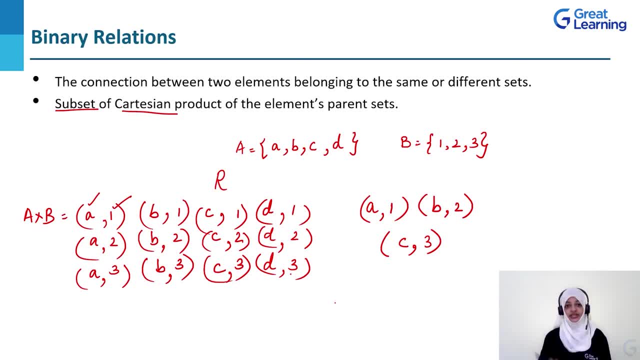 Thus there are no similar positioned objects in the other set and thus D will not be included in the relation. Thus we find that our relation R is actually equal to A 1, B 2 and C 3 ordered pairs, If you observe closely. 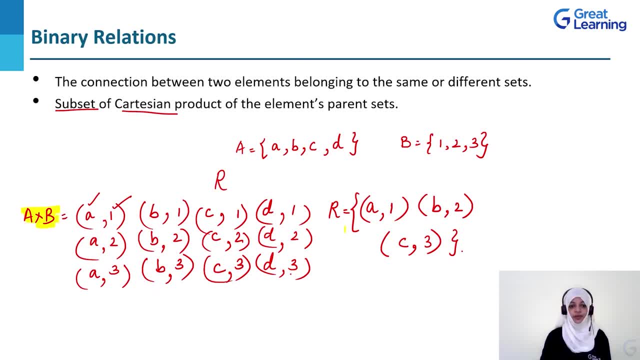 there is a difference between A cross B and R. Obviously, the most obvious difference here is the number of elements within them. But observe closely: every ordered pair that is a part of R is actually also a part of A cross B. We've got A comma 1,. 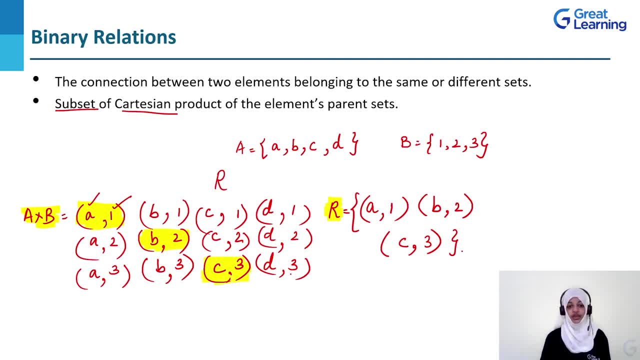 we've got B comma 2 and we've got C comma 3, all which are a part of A cross B. Thus we can say that every relation is actually a subset of the Cartesian product of its pairing set. Let us now look at the next topic. 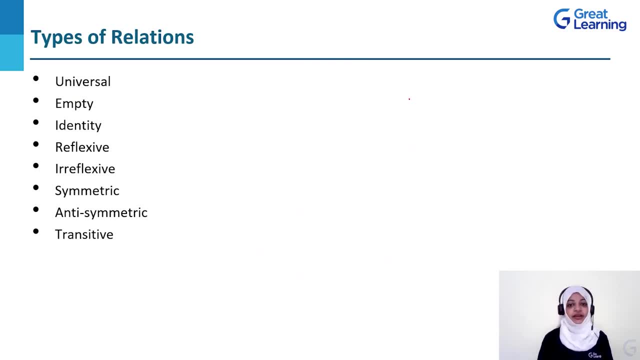 which is types of relations. There are multiple types of relations in relation theory. We'll be looking at the examples of some of these later on in the course. First, let us understand exactly what these relations are. First we have the universal relation. 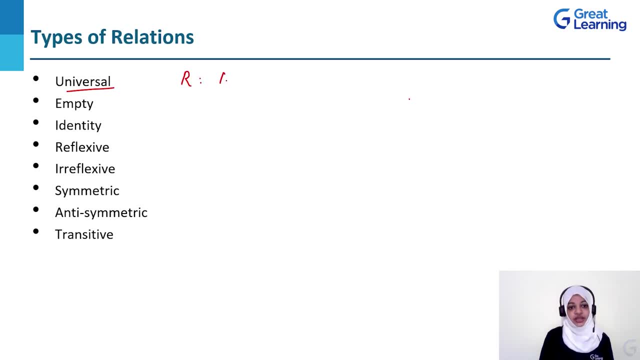 The universal relation is such that if the relation is defined on set A to B, then the relation will actually contain the Cartesian product of A and B, So all of the ordered pairs that would be a part of A cross B would actually be a part of the relation. 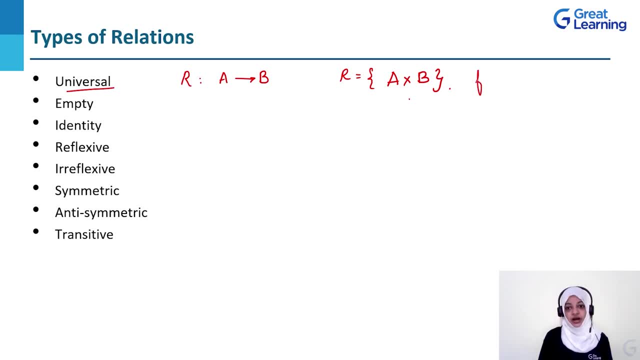 As a result, this relation is also known as a full relation. Next we've got the empty relation. The empty relation, say R going from a set A to B, is actually a type of relation that has no ordered pair within it. 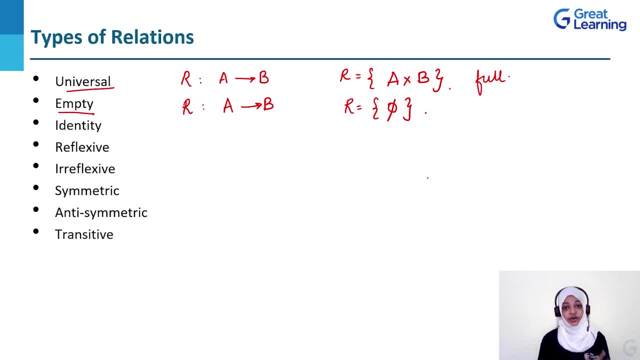 Since the ordered pair given inside is phi, and we already know that phi stands for null, we can actually denote it as this: that the relation has null number of ordered pair within them. This means that there are zero ordered pairs. This is what an empty relation is. 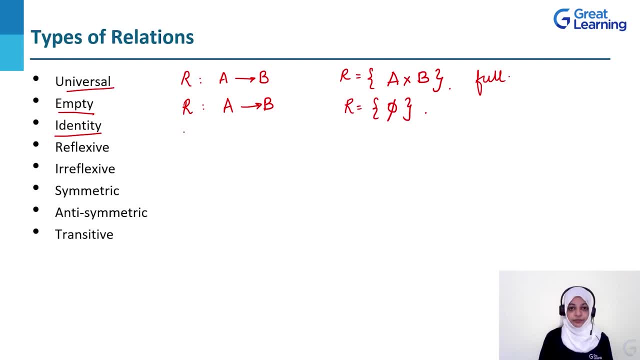 Next we've got the identity relation. An identity relation is one in which one set is related to itself, So R, which is an identity set, is defined from A to A itself. So the actual relation would contain ordered pairs of the type: 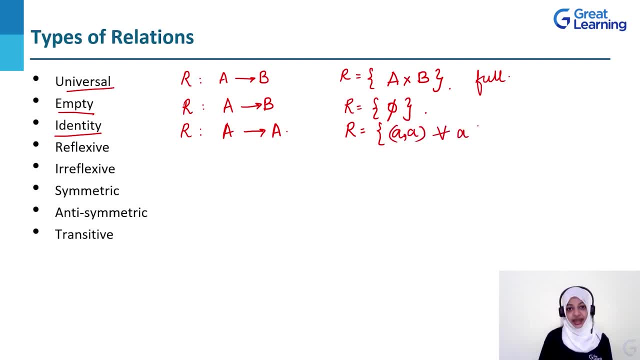 for every small a that belongs to the set given here. Next we've got the reflexive relation. A reflexive relation is a specialized type of relation wherein we've got the relation defined from A to another set B, But in order to be a reflexive relation, 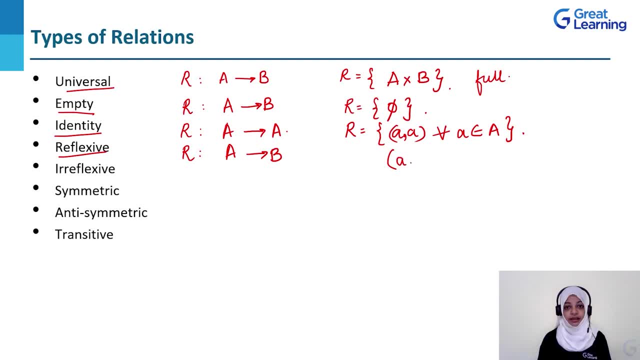 the relation should contain ordered pairs of the type wherein each and every value of A belongs to the set A itself. What is the difference between the identity relation and the reflexive relation, then? There is only one very small difference. Note that here the identity relation. 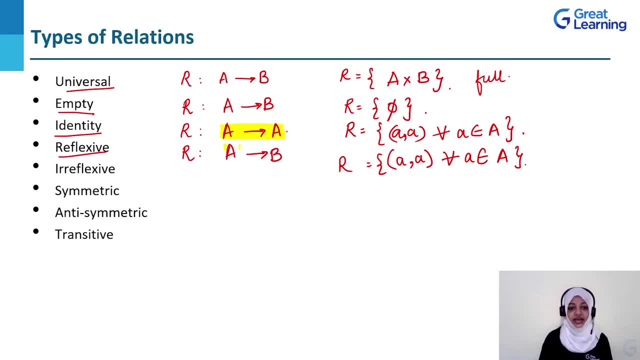 is going from A to itself, whereas the reflective relation is going from A to B. Moreover, in an identity relation, there would be no other ordered pairs apart from the A-A pairs. On the other hand, in the reflexive relation, there would be other ordered pairs. 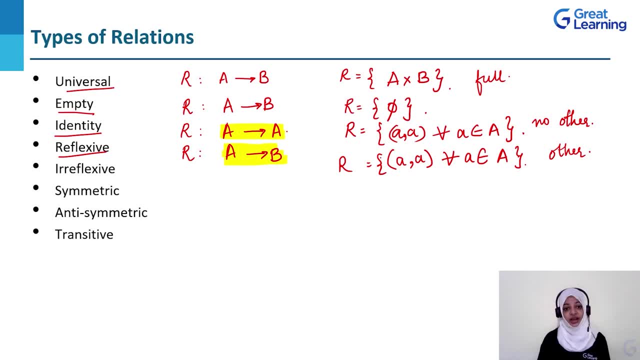 apart from the A-A pairs given because, after all, we need to account for the set B also. So that is the difference between the identity and the reflexive relation. Next, let's look at irreflexive relation. An irreflexive relation. 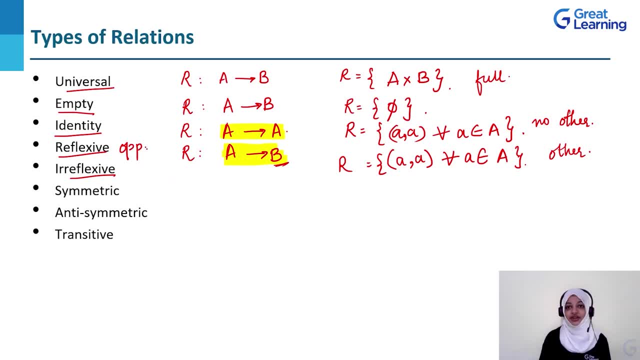 is actually the opposite of the reflexive relation. The reflexive relation says that there has to be ordered pairs of the type. The irreflexive relation, on the other hand, says there should be no ordered pairs of this type in the relation. There could be other ordered pairs. 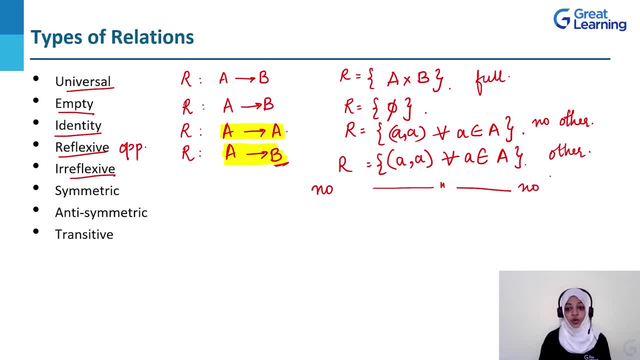 as we have in reflexive, but there should be no A-A ordered pairs. Again, this relation is also defined from A to set B. Next we've got the symmetric relation. A symmetric relation again is defined as a relation passing from set A to set B. 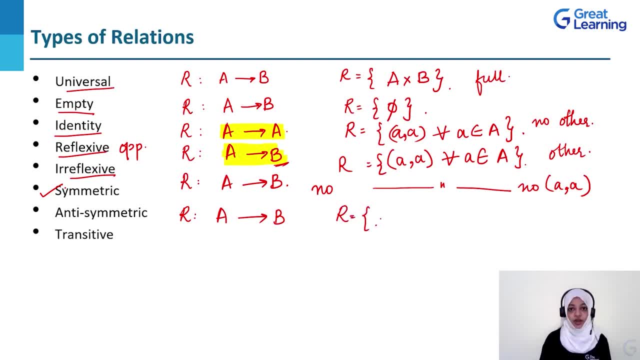 such that the relation would contain ordered pairs of the type, And if such an ordered pair exists in the relation, then it stands to reason, as per symmetric relations, that an ordered pair of the type would also belong to the relation. Please make a note of this. 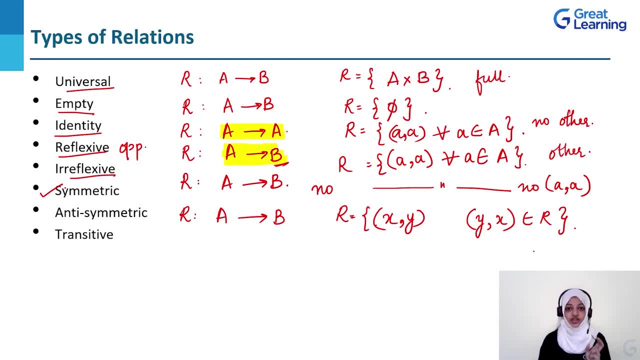 This is important in understanding exactly what symmetric relations are. If ordered pair exists in the relation, then ordered pair should also exist within the relation. Next, let's look at the anti-symmetric relation, As we've seen, with a reflexive relation, 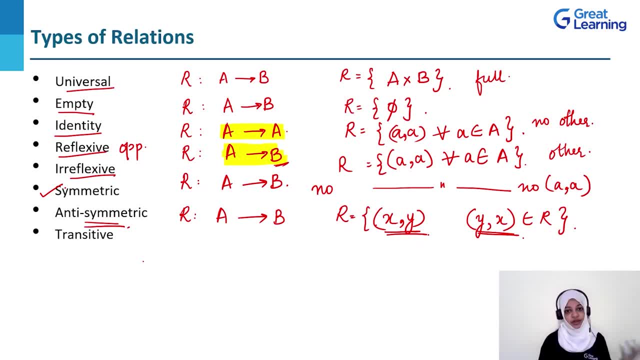 we've got an irreflexive relation. Similarly, with a symmetric relation, we've got an anti-symmetric relation. The definition of anti-symmetric relation, however, is slightly different. There are two conditions for any relation to be anti-symmetric in nature. 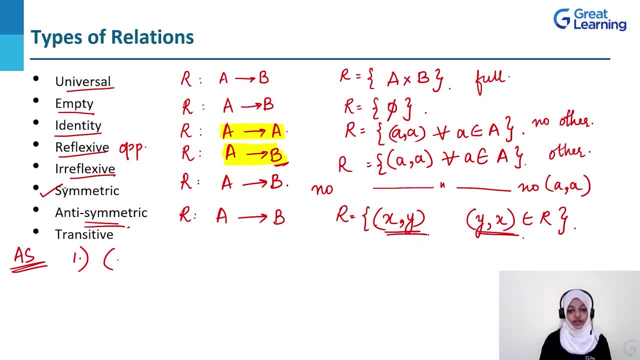 The first condition is that if we have an ordered pair of the type, then there should exist an ordered pair of the type such that x and y are equal to each other. This is the first condition. Secondly, if, in case, y and x are not equal to each other, 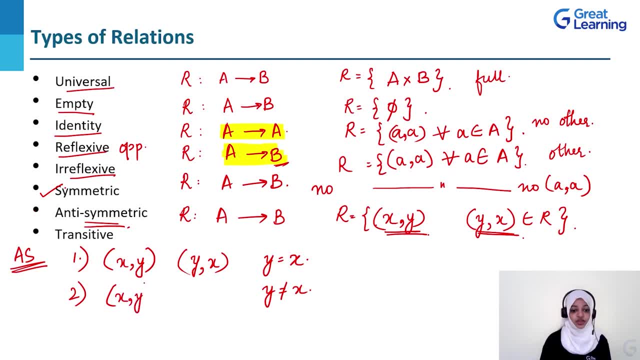 then we should only have y and y and x should ideally not belong to the relation. Please be very careful while remembering these two conditions of anti-symmetric. We're going to see an example of anti-symmetric relations later on in the course. Lastly, we've got transitive relations. 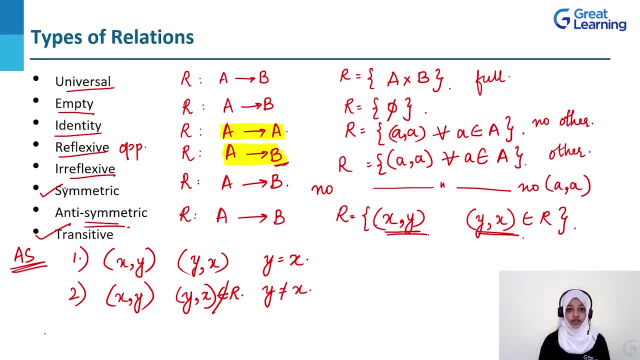 Again, in transitive relations we've got two conditions which we need to take care of. A transitive relation is one where if we have an ordered pair of the type and we've got an ordered pair of the type, then it stands to reason. 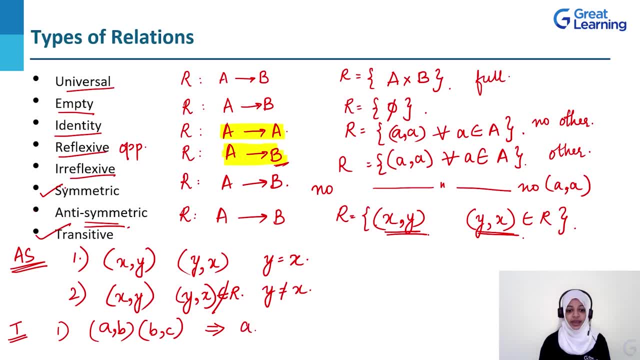 that we should have an ordered pair of the type. It actually sounds a lot similar to our transitivity relation, wherein if a is equal to b and b is equal to c, then it stands to reason that a is equal to c. The transitivity relation. 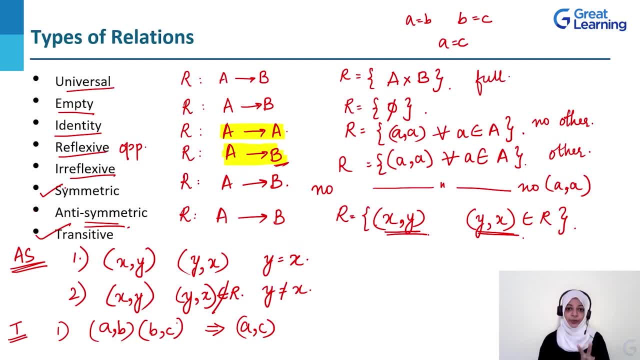 is actually stating something like this. So if the two ordered pairs belong to the relation, then also belongs to the relation. The second condition is slightly different. The second condition says that if exists in a particular relation and there is no given in the relation, 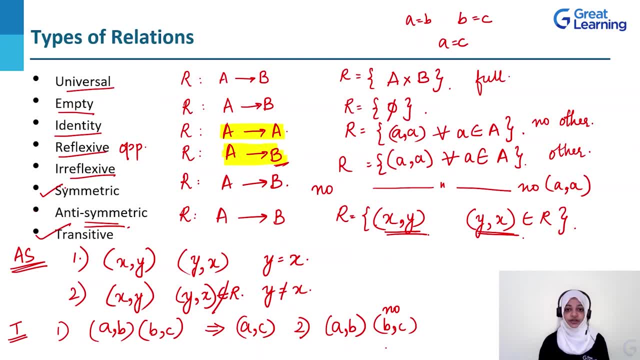 then the relation is still termed to be a transitive relation. So please make a note of these two conditions. Firstly, if we have two ordered pairs of the type and then we need to have an ordered pair of the type, Then the relation is said to be transitive. 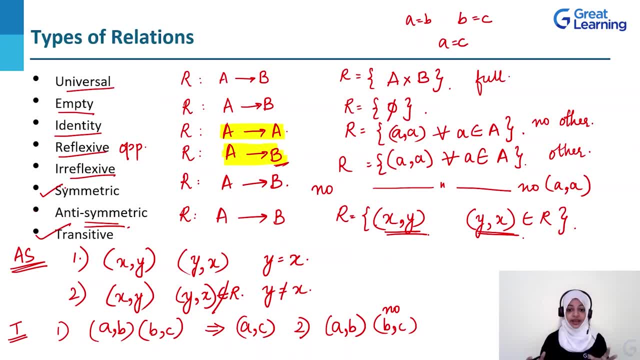 On the other hand, if we have an ordered pair of the type but no ordered pair of the type, thereby giving no ordered pair of the type, then this particular relation is still said to be a transitive relation. A doubt some of you might have is: 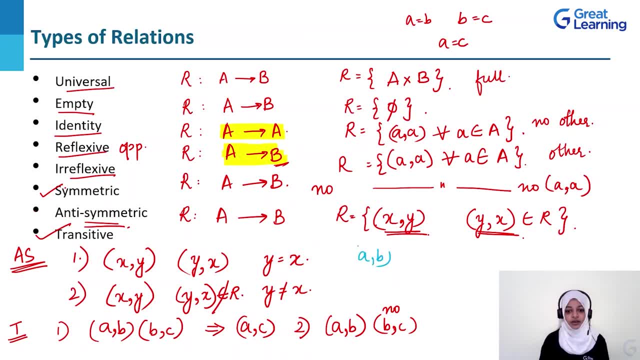 what happens if you've got and but no, Since there is no relation between and, we will consider as a part of the second condition and consider it as transitive in nature. Thus we've seen the different types of relation and their definitions. 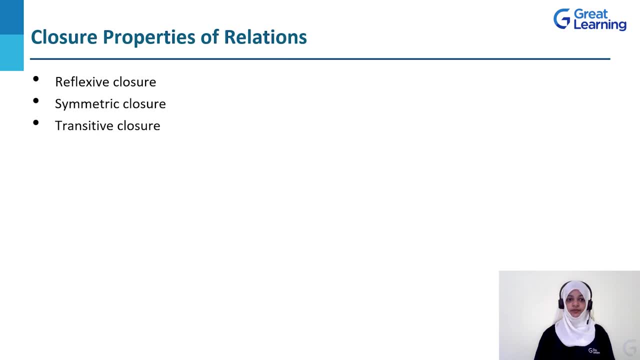 Let us now look into the closure properties of relations. What are closure properties? So it's a concept wherein, if a relation is not something, we make it into that. There are three actual types of closures that we often see within relations. We've got the reflexive closure. 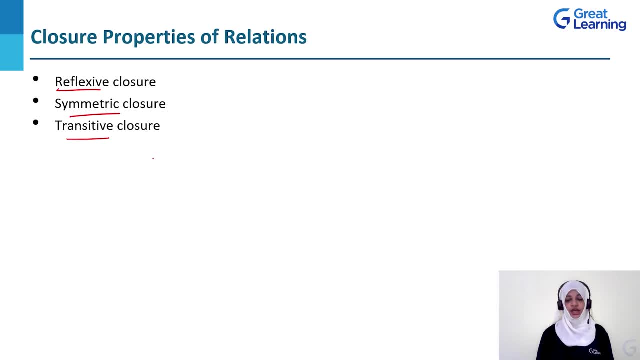 the symmetric closure and the transitive closure. So what this basically means is that if a relation is not reflexive, we will try to make it reflexive. Similarly, if a relation is not symmetric or not transitive, we will try to make them symmetric or transitive. 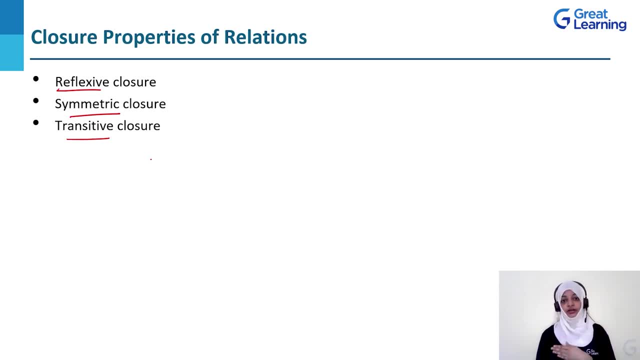 Now how do we make them into what they aren't? It's very simple. We simply attach an ordered pair. Attaching an ordered pair of a certain value will obviously make the relation reflexive or symmetric or transitive, based upon what kind of ordered pairs. 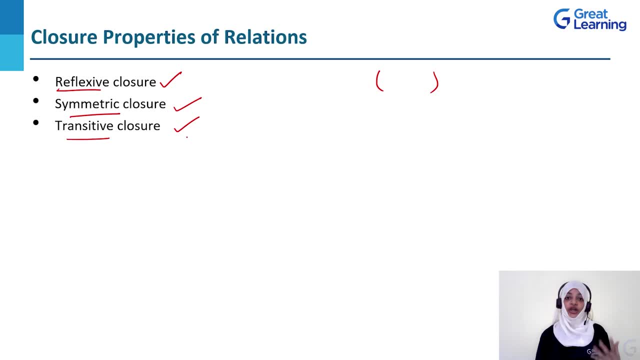 are added to the relation. The ordered pairs that have to be added should be minimal in number. This is very important to remember. They should be the most minimum number of ordered pairs that can be attached in order to convert a relation from non-reflexive to reflexive. 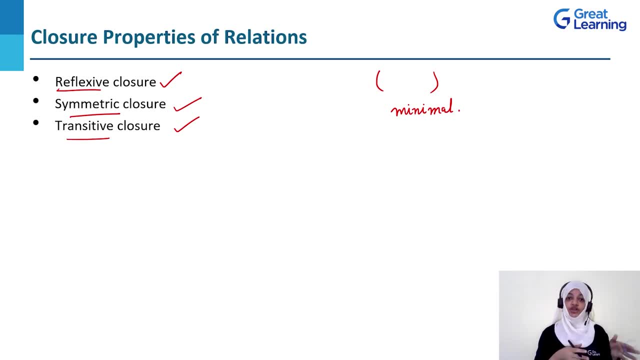 or from non-symmetric to symmetric, or from non-transitive to transitive. Let us first define these closures. If a relation R is such that it is non-reflexive in nature, then how do we provide reflexive closure? It's very simple. 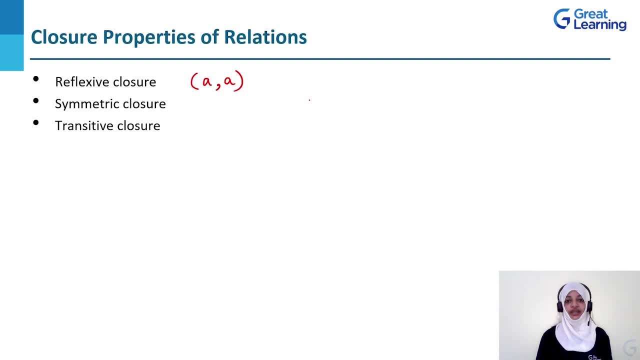 Simply attach an ordered pair of the type where a belongs to the set which is a part of the relation. Similarly, how do we change a relation which is currently non-symmetric into a symmetric relation? If there are any ordered pairs of the type, attach corresponding ordered pairs. 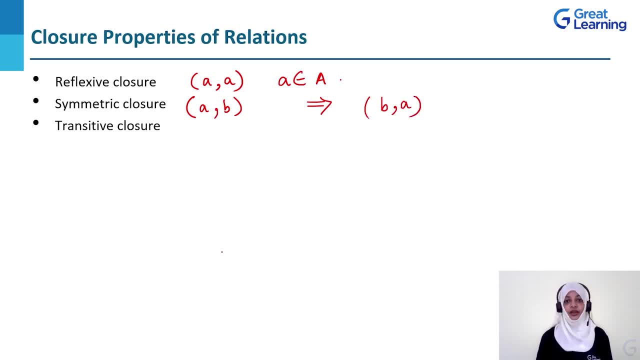 of the type wherein a belongs to the set and b belongs to the set of the relation itself. Lastly, how do we convert a relation which is not transitive in nature into a transitive relation, For every ordered pair and attach a corresponding ordered pair? 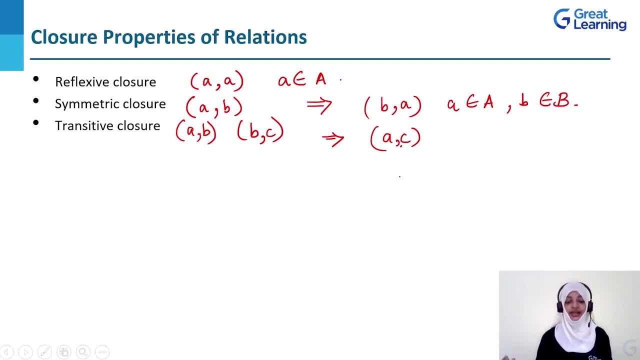 This needs to be carried out iteratively till we don't have all of the ordered pairs in this form. As a result, any relation which is currently non-reflexive, non-symmetric and non-transitive can be converted into reflexive, symmetric and transitive. 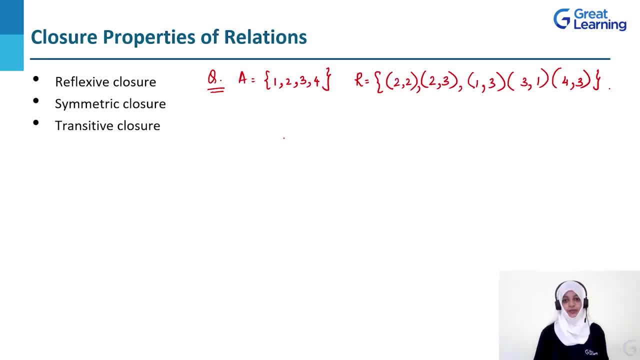 Let us look at this with an example. Let this be our example under consideration. It's a simple example. We have a set A and a relation R, such that we've got the relation going from the set to itself. The relation R has a set of ordered pairs within them. 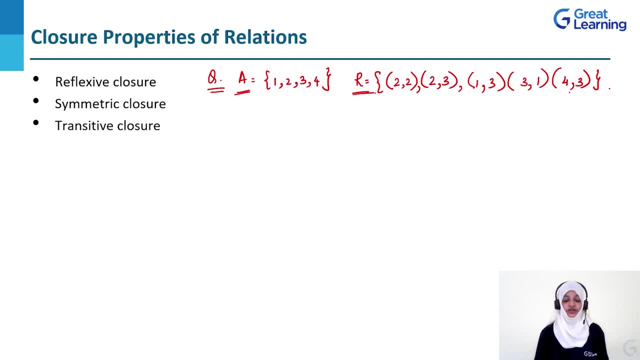 As we can see from the definition of reflexive, symmetric and transitive sets, this set is neither reflexive, nor symmetric, nor transitive at the moment. First, let us try to make this set into a reflexive set. It's very easy to convert any set into reflexive. 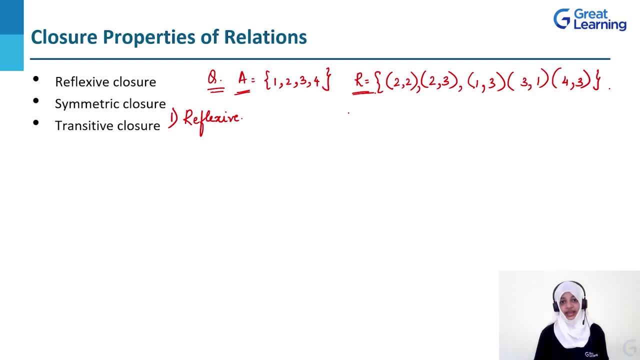 Just add ordered pairs of the type. This means that if relation R has to be made into a reflexive set, we are going to attach ordered pairs of the type. and Some of you might have a doubt: why did I not add here? 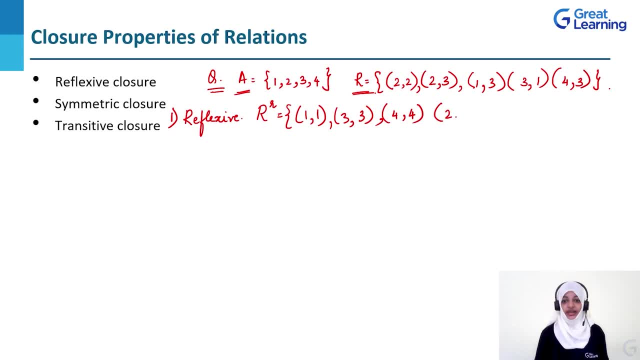 That's pretty simple- is already a part of the original relation. The rest of the relation comes as it is So and will be a part of the relation as they were previously. Thus, our relation has now been converted into a reflexive relation. 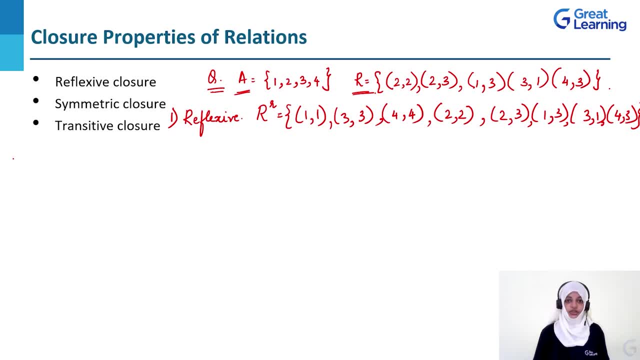 Next, let's look at how we can convert this particular relation into a symmetric relation. In order to have a symmetric relation- let's call it R- we need to ensure that for every ordered pair, there exists a corresponding ordered pair of. Let us see how we can do that. 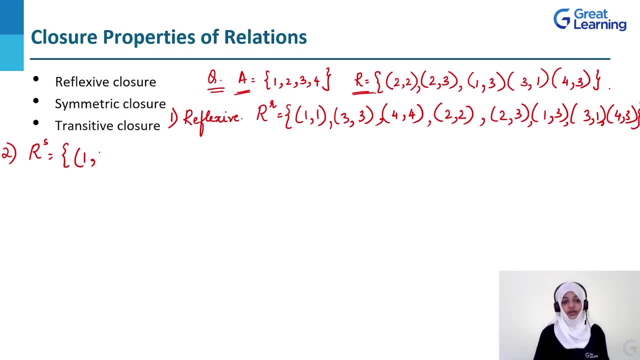 Consider the first ordered pair here. If this is considered, as then would also be, This is true for every reflexive ordered pair. Thus, and will be written as they are. Next, let's look at the ordered pair. 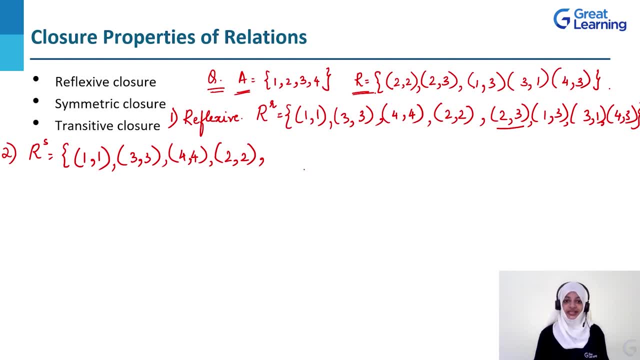 In order to be symmetric in nature, there needs to exist an ordered pair. As it does not already exist in our relation, let's add that. So we've got, as an ordered pair, to correspond to which already exists in our relation. 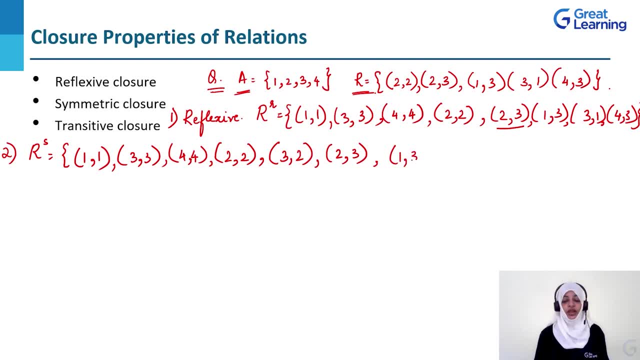 Next, we've got the ordered pair. has its corresponding symmetric pair already existing in the relation. Lastly, we've got the ordered pair as a part of our relation. again, does not have a symmetric ordered pair for it, So we're going to attach it as. 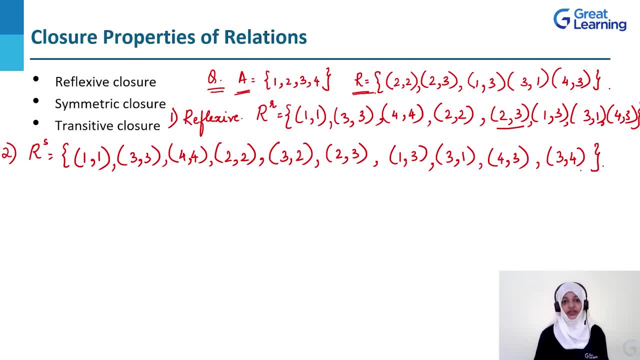 Thus, the relation has now been converted into a symmetric as well as a reflexive relation. Lastly, we're going to look at how we can actually convert a relation into transitive closure. Converting a relation to transitive closure is actually simple. 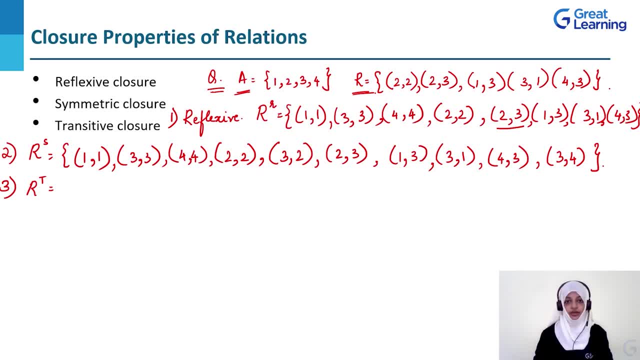 It's just a constantly iterative method. As such, we need to be very careful while attaching transitive ordered pairs into closures. In order to actually understand how transitive ordered pairs work, let us look at the example given here. If we've got the first ordered pair, 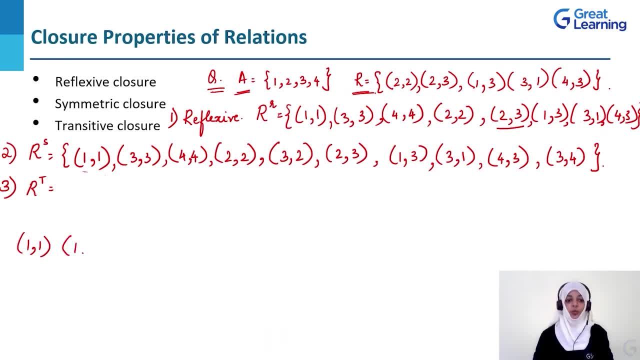 and we've got a corresponding ordered pair. we will then have an ordered pair for transitivity, such that it would be: What we need to understand here is very simple: If this is A and this is B, and this ordered pair has B and C, 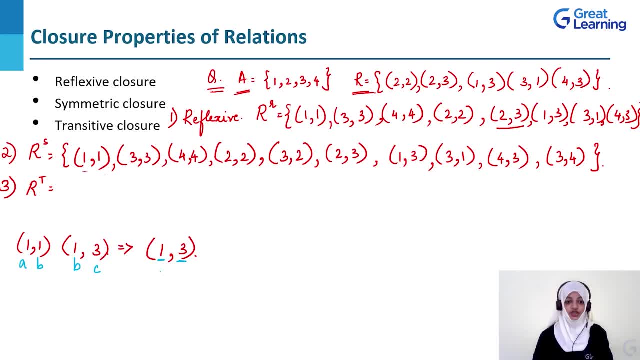 then the final ordered pair for transitivity should have terms A and C. This is how we're supposed to identify all of the elements that may be a part of transitivity. Let's take another example. Let's consider the set and its transitivity match. 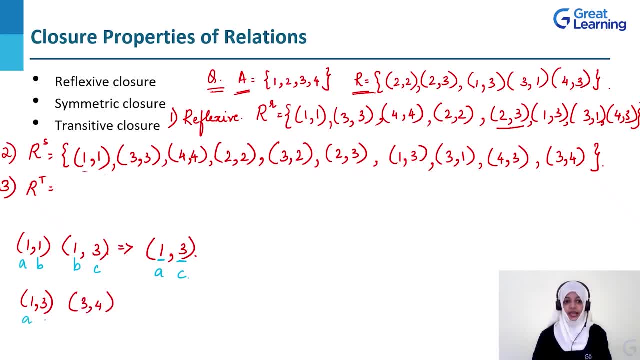 If we consider this as A, this term as B, then this term becomes B and this term becomes C. Thus our transitivity ordered pair ends up becoming: Observe closely does not exist in the given relation here. So what do we need to do? 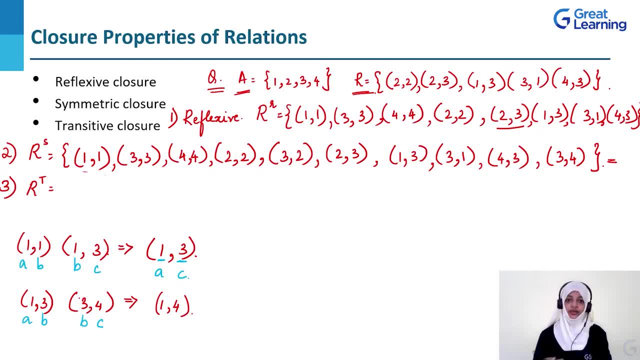 We need to attach this new ordered pair in order to make this whole relation transitive. This particular calculation has to be performed in an iterative manner for each and every ordered pair in our relation. In the end, what we get is the transitive closure. 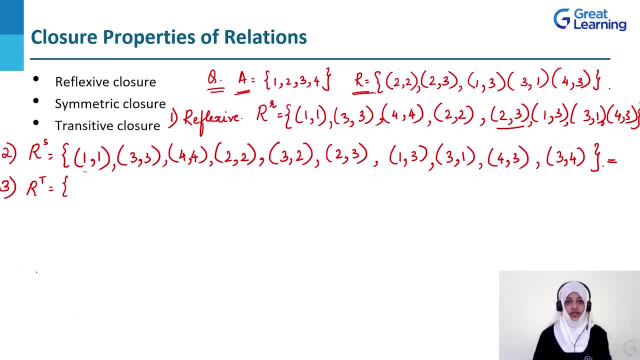 Let us take one last example here to better understand transitivity closure. Let us consider the set with and the set with. Thus, as we can see here, this is the transitive relation after closure. Please note that this is not the only form of transitive relation. 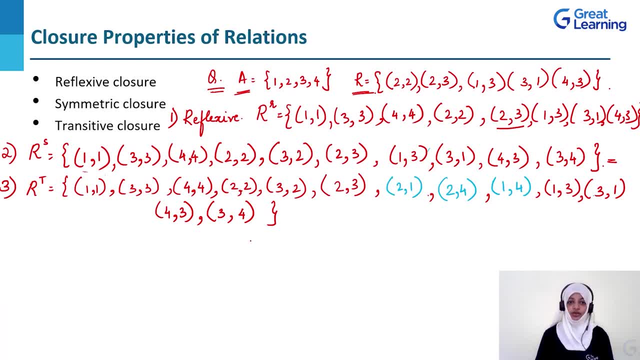 More iterations can be carried out later on in order to see whether this particular transitive relation is really in closure or not. An important point to remember here is that if we achieve reflexive closure, symmetric closure and transitive closure all in any relation, 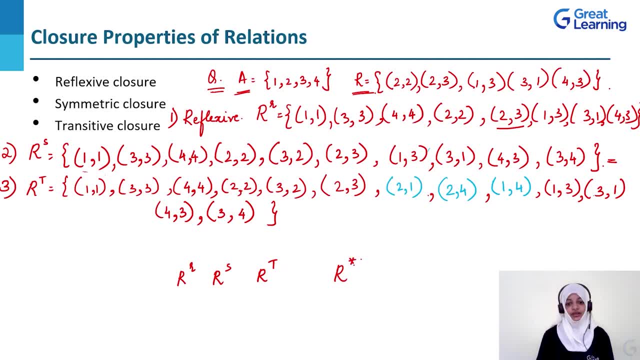 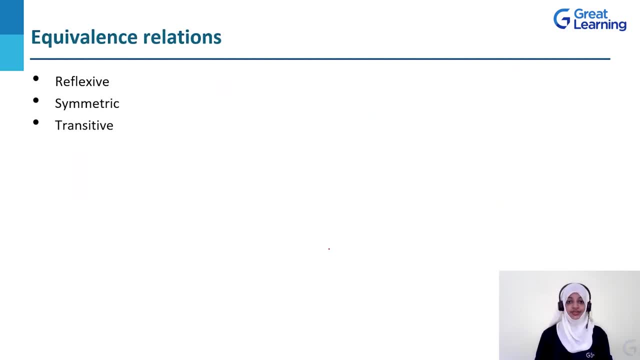 then that relation is said to be in equivalent closure and is denoted by r raised to star. Let us go on to the next topic, which is equivalence relation. Now, as per the definition, we already know that an equivalence relation is one where the relation is reflexive, transitive. 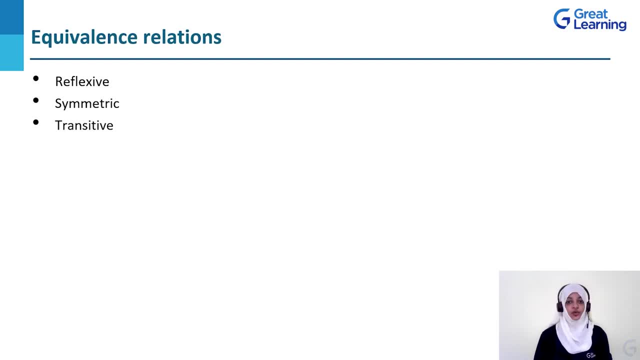 as well as symmetric. If any relation has all of these three different properties within it, then the relation is said to be equivalent in nature. Let us understand this concept with a practical example of a set in a relation and how we can determine whether that relation 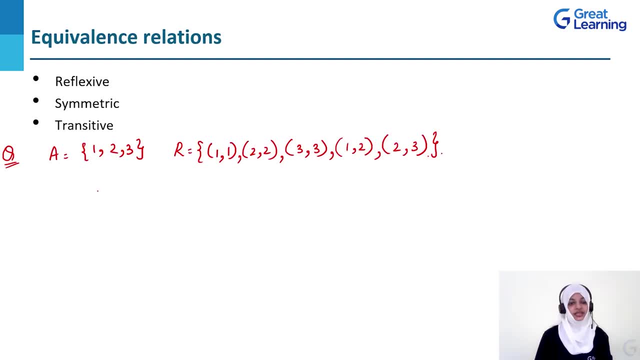 is equivalent relation or not. Let us consider this simple example as our first example. As we can see here, we have a set A such that A consists of elements 1,, 2, and 3.. Next we've got a relation r. 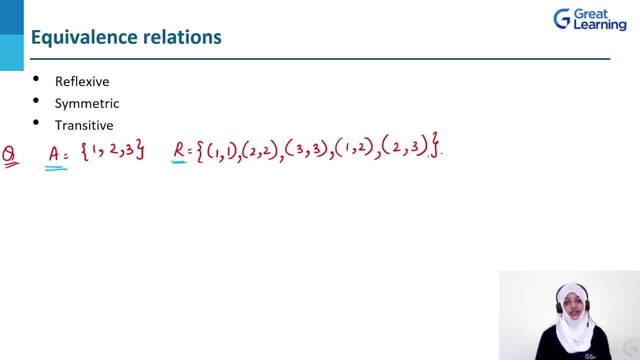 on this set A such that r contains all of these ordered pairs. Let us see whether these elements are reflexive, symmetric or transitive. First let us look at whether these elements are reflexive. A relation would be reflexive if there exists. 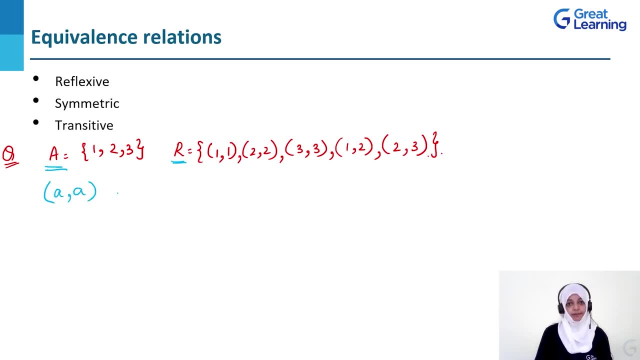 ordered pairs of the type for each and every element that belongs to the set under consideration. This is seen here. As we can see, there are three elements- 1, 2, and 3- in our set For all of these three elements. 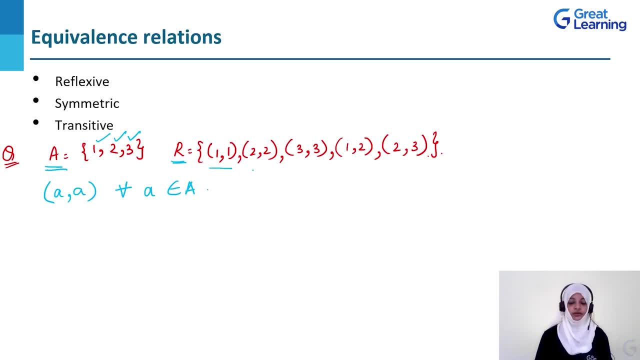 we have ordered pairs of the type 1, 1,, 2,, 2, and 3, 3.. Thus we can say that the relation r is reflexive in nature. Next, let us look at whether this particular relation is symmetric or not. 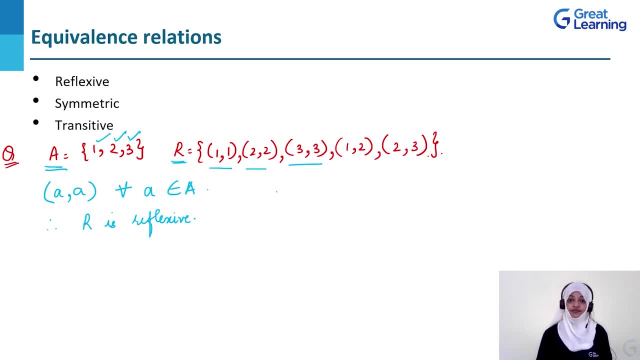 As per symmetricity, we know that for every ordered pair there should exist a such, that A and B both belong to the actual sets that are under consideration in the relation. Let us see if that is satisfied. here We've got an ordered pair. 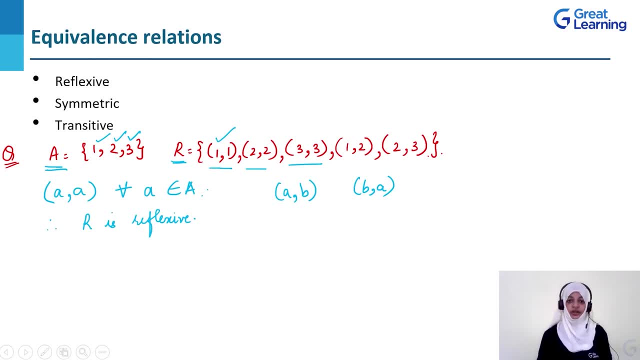 its symmetric would be again. This is true with all of the reflexive ordered pairs. Let us check a non-reflexive ordered pair. On seeing the ordered pair, we should ideally have another ordered pair to make this symmetric. Similarly, if we've got the 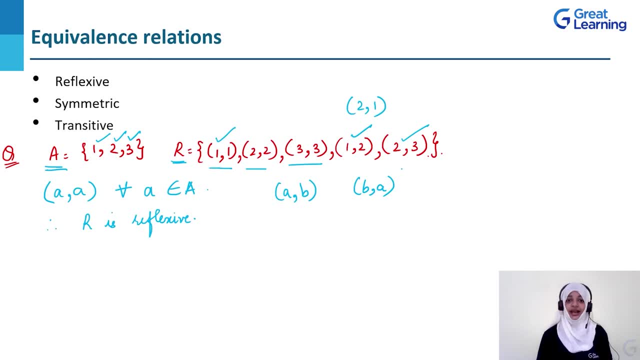 unreflective ordered pair, there should ideally be a corresponding ordered pair to make this a symmetric relation. Thus we can see that, even though this particular relation is reflexive in nature, the relation is not symmetric in nature. Next, let us look at whether this particular 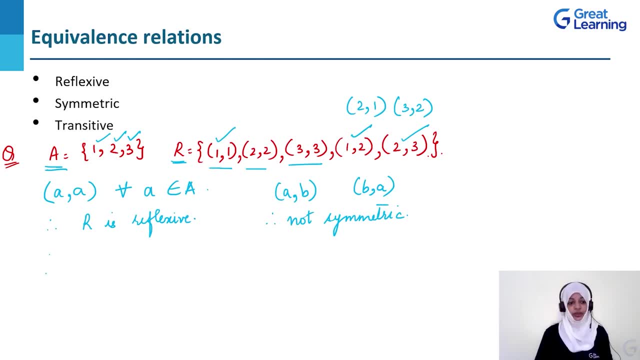 relation is transitive or not. In transitivity, we know that for every ordered pair, if there exists a ordered pair, then there should exist an ordered pair. Let us check whether that is true within our relation. Let us consider the ordered pair. 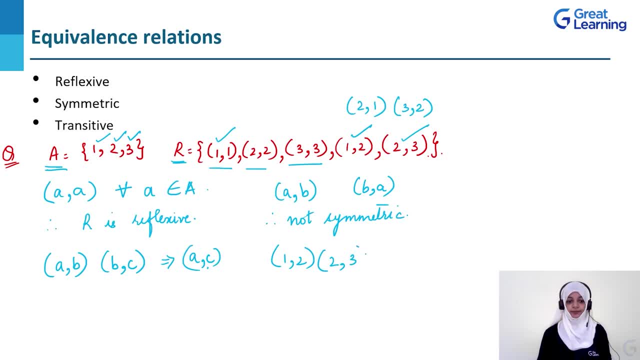 1,2 and 2,3. Considering these two ordered pairs, if this is A and this is B, and this is B and this is C, this implies that there should exist an ordered pair of the type 1,3.. Since this particular 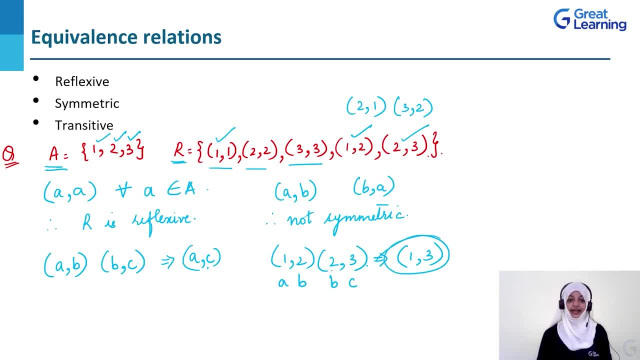 ordered pair does not exist, we can't say that this particular relation is transitive in nature. Therefore, the relation provided here is not transitive either. Thus, since this particular relation is neither symmetric nor transitive, but only reflexive, this relation is not an equivalence. 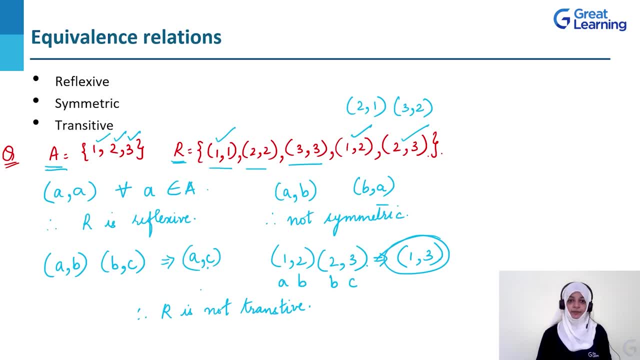 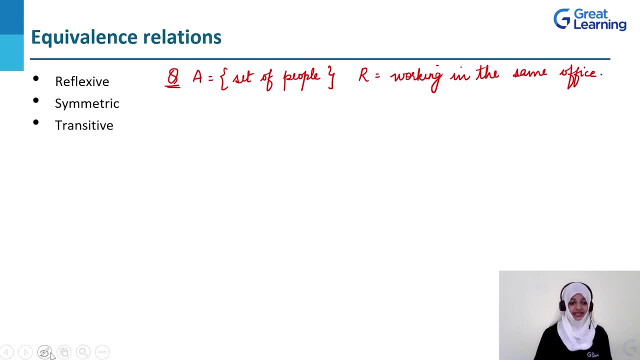 relation. Next, let us look at an example of an equivalence relation. Let us consider this particular example. Let us have a set A, which is the set of a few people, and let the relation on the set be such that it is defined as the ordered pair of people who are: 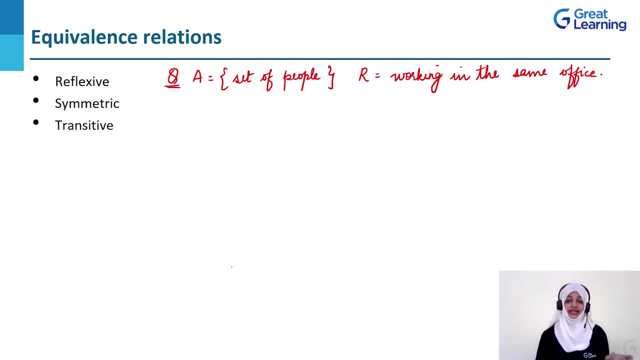 working in the same office. Let us see if this is an equivalence relation or not. Consider the first quantum here, which is reflexivity. If there exists a person A, such that this person belongs to the set of people, then we can say that A. 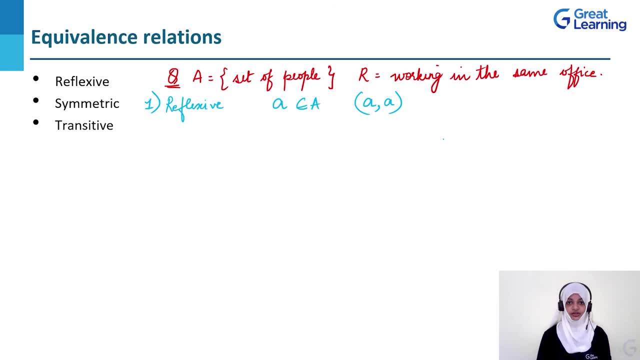 and itself works at the same office. Logically, this does make sense, because one person will work at the same office as themselves, Right? This would be true for each and every value that is contained in the set of people. Every person would be able to work at the exact 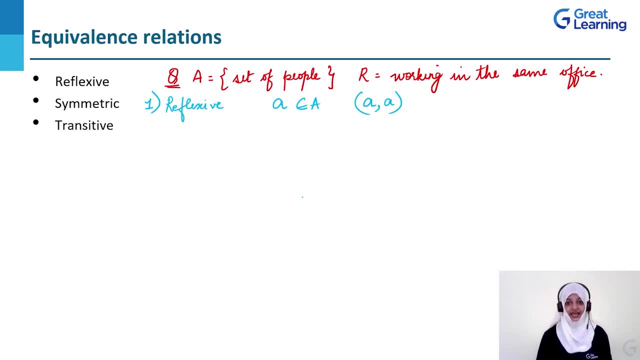 same office that they are working at. Thus, we can say that the relation is reflexive. Next, let us look at the second condition here. Is this particular relation symmetric in nature? In order to be symmetric, we need to have an ordered pair such that, if 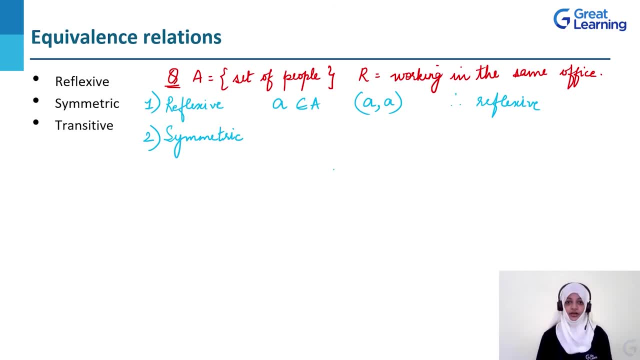 exists, then also exists Here. let there be two people who are working in the same office and belong to the set of people under consideration. If are working in the same office, this implies that would also work in the same office. Thus we can have: 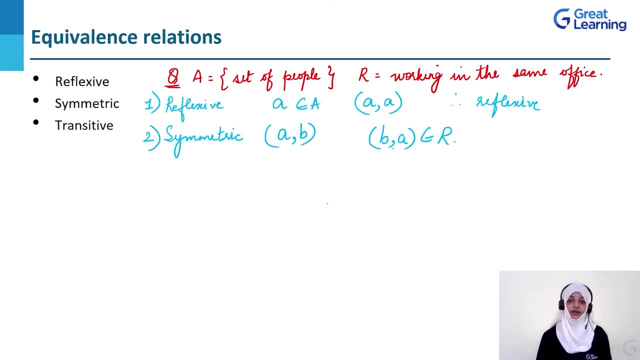 an ordered pair that belongs to our relation R. Thus we can say that this relation is symmetric in nature. Taking any two people in this particular set of people will give us the same result. If two people are working together in the exact same office, then 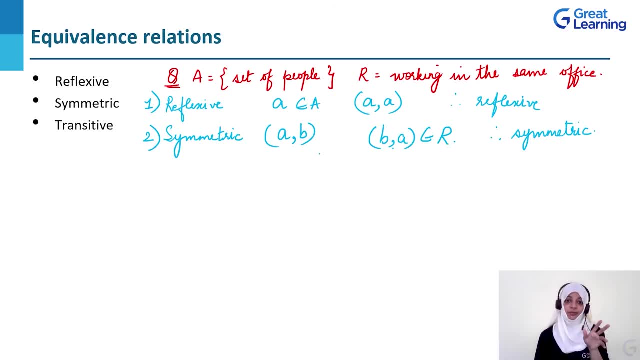 it does not matter how you arrange the ordered pair, they would still be working in the same office. Lastly, let us look at whether this particular relation is transitive or not. If we have two people, A and B, working in an office and 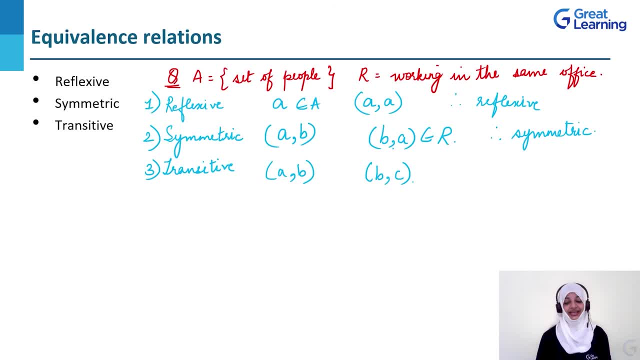 we have another set of people- B and C- working in the exact same office, then both of these sets belong to R. Not only that, if A and B are working in the same office and B and C are also working in the same office, this automatically. 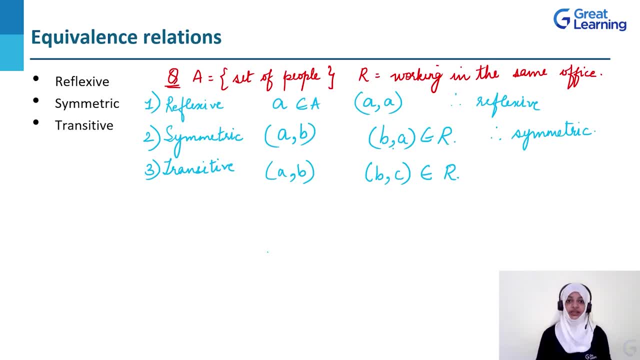 implies that all three people- A, B and C- are working in the same office. As such, we can say that A and C are also working in the same office, and the ordered pair A- C belongs to the relation R. So if A- B, 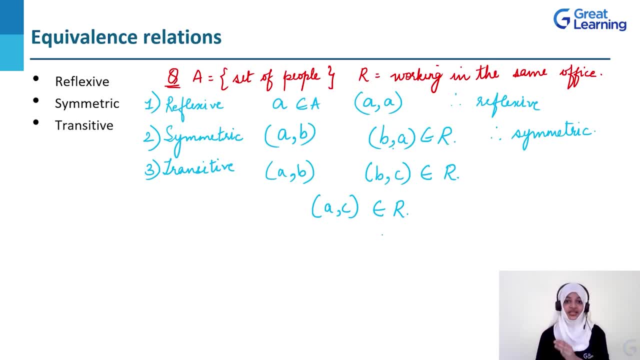 B, C are belonging to R, then A- C is also belonging to R. Therefore, the relation here is transitive in nature. Since we have seen that the relation is reflexive, symmetric as well as transitive, we can finally say that this particular 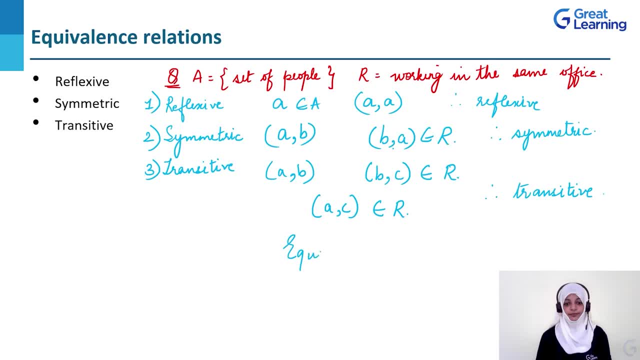 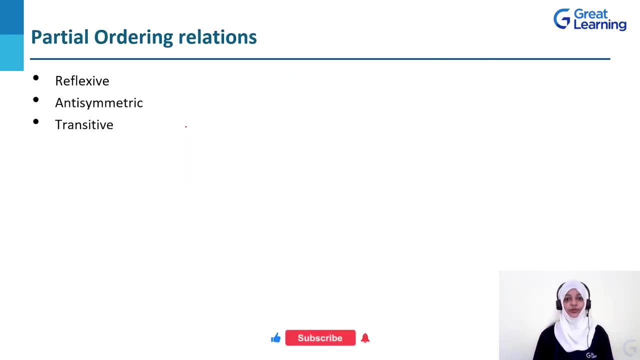 relation is equal or equivalent in nature. So any relation that has all three properties, namely reflexivity, symmetricity and transitivity, in it is known to be an equivalent relation. The last topic that we are going to be seeing in this particular session is the partial order relation. 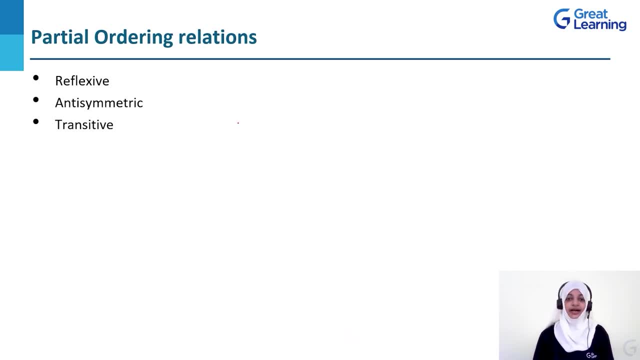 Now, what is a partial order relation? A relation is said to be partial order relation if it is reflexive, anti-symmetric and transitive. We have already seen what all of these three mean when we were looking at the types of relations. Let us now understand. 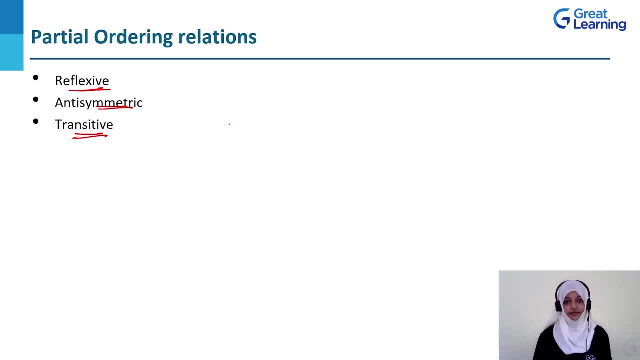 them with an example. A relation is said to be reflexive if it contains ordered pairs of the type where A actually belongs to the set on which the relation is working. On the other hand, a relation is said to be anti-symmetric if for. 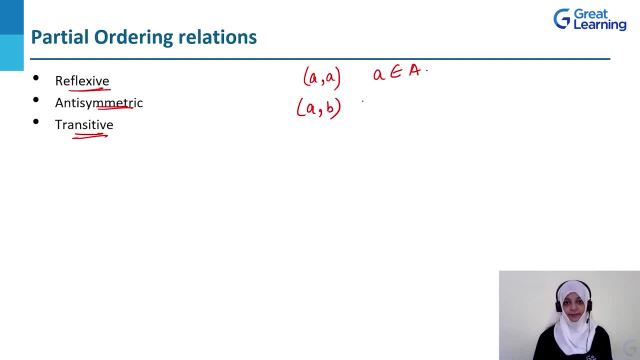 an ordered pair. there exists an ordered pair such that B is equal to A. What happens if this condition is not satisfied? Then this particular relation would no longer be called anti-symmetric in nature. Another important thing we need to remember is the condition that 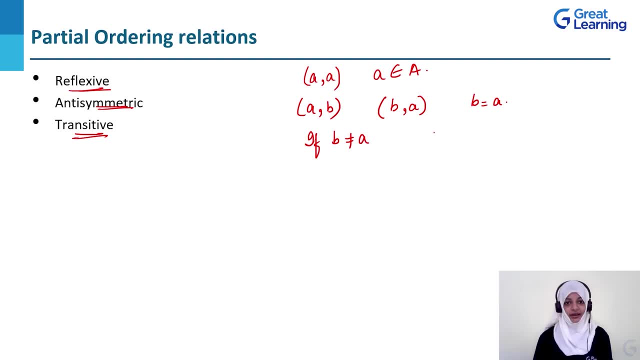 if B is not equal to A, then should not belong to the relation. In either of these cases, the relation will be said to be anti-symmetric. So either the two values should be equal to each other or should just not belong to the relation. 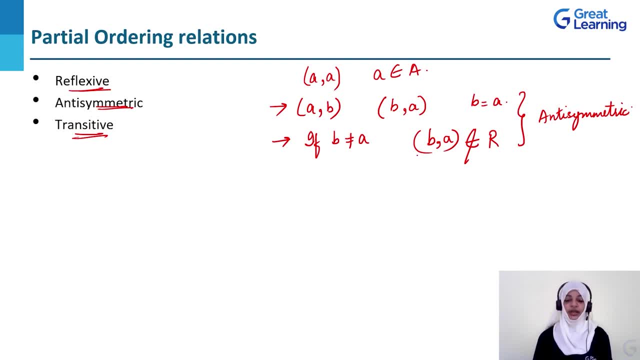 If any of these conditions are satisfied, then the relation is said to be anti-symmetric. Lastly, if we have an ordered pair of the type and another ordered pair of the type, then for the relation to be transitive in nature, we will have to have: 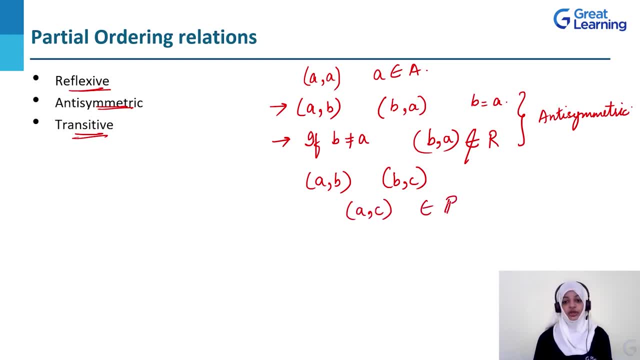 an ordered pair which also belongs to the relation. These are the three conditions for any relation to be a partial ordering relation. Let us now look at this particular concept with an example. Let us now consider these examples given here and check whether these are partial. 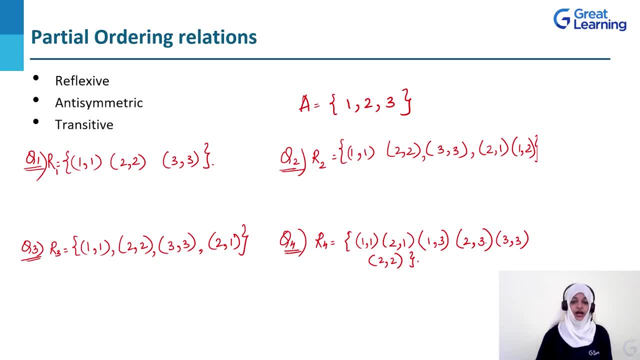 order relations or not. All of these relations are based upon the set A as given on the screen. Let us look at the first relation, R1.. The first relation R1 is obviously reflexive in nature. That is because each and every element has been 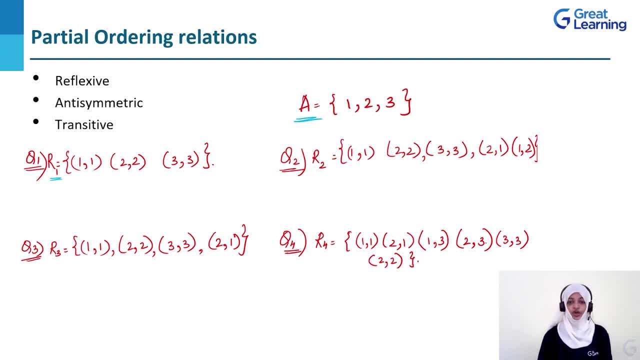 ordered with itself. So 1,1,2,2 and 3,3 are all a part of the relation, So it is obviously reflexive in nature. Let us see whether this relation is anti-symmetric in nature. The ordered pair: 1,1. 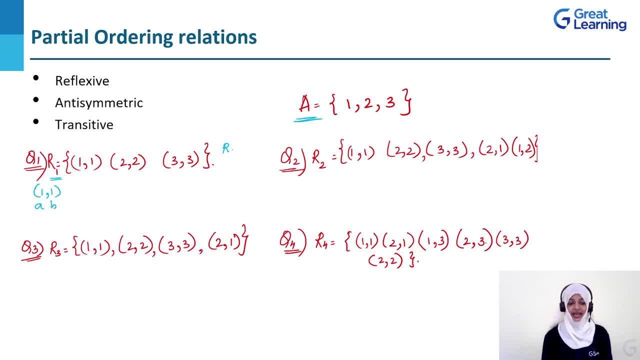 exists. If we consider this as A and B, then BA would be 1,1.. Both of these ordered pairs exist in our relation. Apart from that, we can also see that B is equal to A, because both of the values are, after all, equal to 1.. 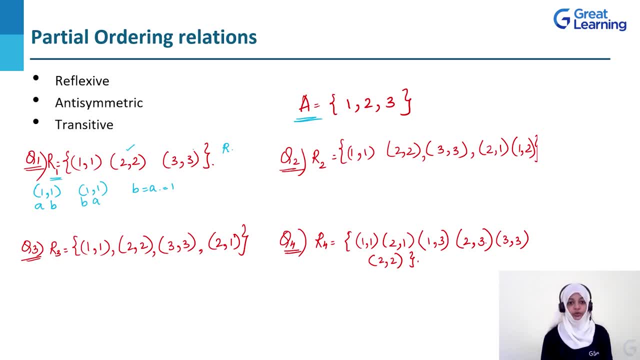 Similarly, if we look at the ordered pair 2,2 and 3,3, we get a similar result. As a result, we can conclude that each and every one of the ordered pairs in this particular relation are anti-symmetric in nature. 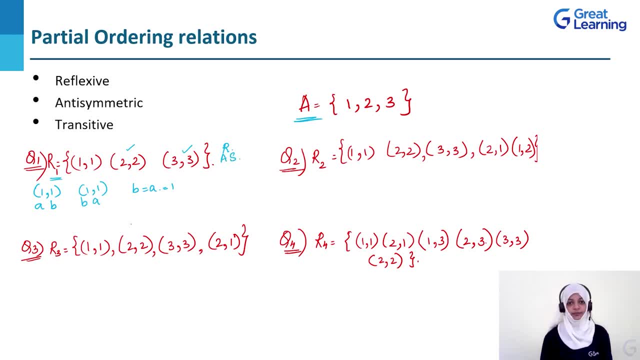 Thus we can say that this relation is anti-symmetric. Lastly, let us look at whether this particular relation is transitive or not. So we have got relation 1,1. let this be A and B. We have got an ordered pair 1,1. 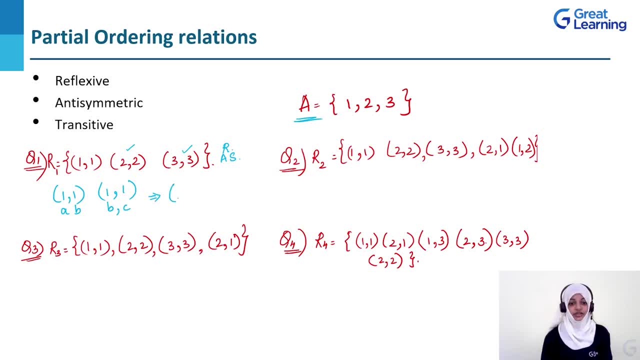 let this be B and C, and this should ideally give rise to 1,1, which is A and C ordered pair. As you can see, if we have the ordered pair AB and BC, we are getting an ordered pair AC, all three of which. 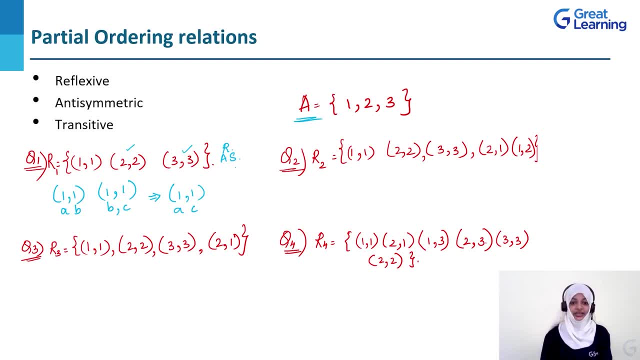 are present in our relation. As a result, we can say that this relation is transitive. also, If a relation is reflexive, anti-symmetric and transitive, we can easily conclude that this particular relation is a partial ordered relation. Next, let us look at the second example given here. 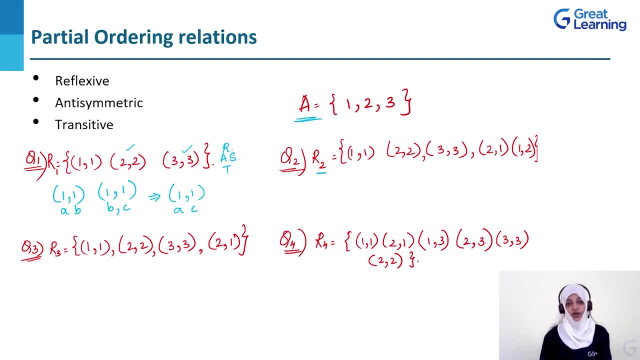 For the relation R2, which is again set on A, we can see that 1,1,, 2,2 and 3,3 exist. As a result, this relation can be said to be reflexive in nature From the previous example. 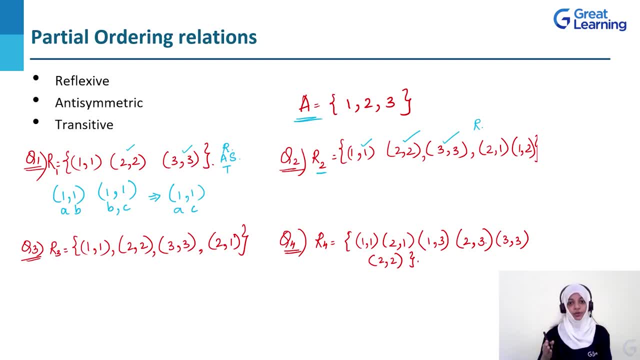 we already know that the ordered pairs 1,1,, 2,2 and 3,3 are always going to be anti-symmetric in nature. Let us look at the other two ordered pairs that are also given here. We've got the ordered pairs. 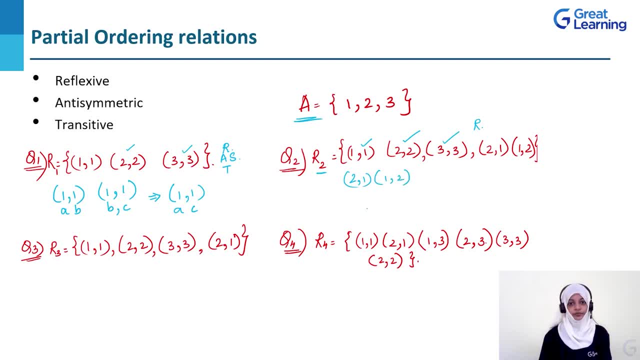 2,1 and 1,2.. If they are of the form AB and BA, then they should ideally be equal to each other. This means that A should be equal to B, But, as we know, 2 is not equal. 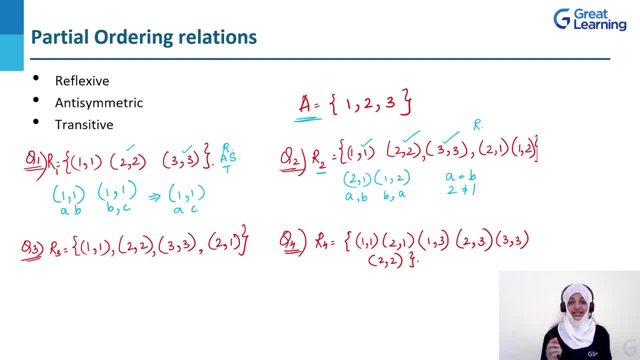 to 1.. Thus this particular relation is symmetric in nature, not anti-symmetric. So if a relation is not anti-symmetric in nature, it can't be a partial ordered relation either. So this particular relation is not a partial ordered relation. 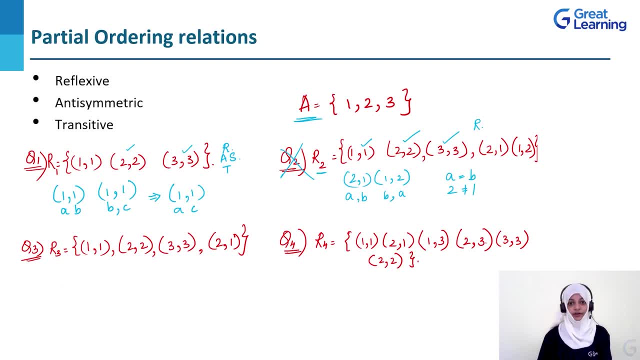 Next, let us look at our third example given. here. We've got the relation R3, which is again set on A. In this particular relation, we can see that we've got ordered pairs 1,1,2,2 and 3,3. 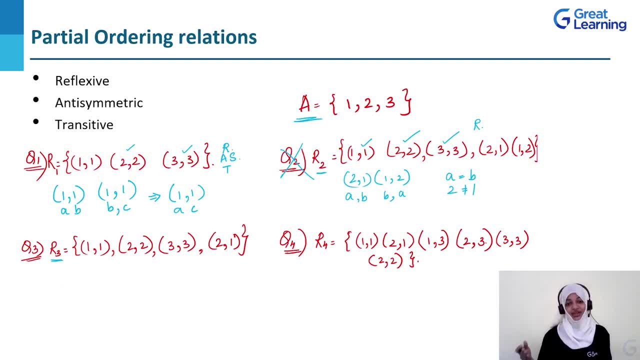 By now we are very confident that 1,1,2,2 and 3,3 are ordered pairs, which make us realize that this particular relation is reflexive in nature. Next, let's see whether we have anti-symmetricity here. 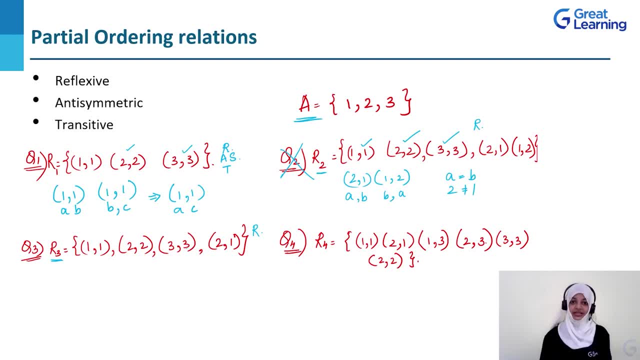 1,1,2,2 and 3,3 will obviously be anti-symmetric, as we've seen from example 1.. What about the next ordered pair? We've got an ordered pair of the type, But there are no types. 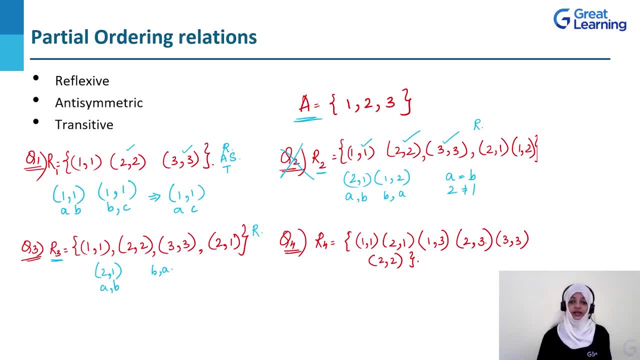 What do we do in this case? We check out our second condition, which is a part of anti-symmetricity. We've seen that B is not equal to A. In such a case, if B is not equal to A, it is better if the ordered set. 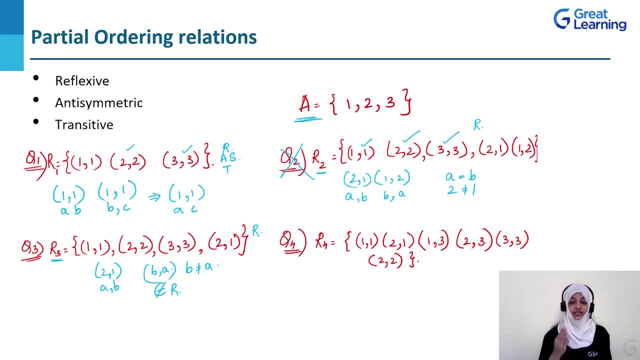 does not belong to the relation. If the ordered set does not belong to the relation, we can say that this particular relation is anti-symmetric in nature. Thus, because the two values given here, namely 2 and 1, are not equal to each other, that is, 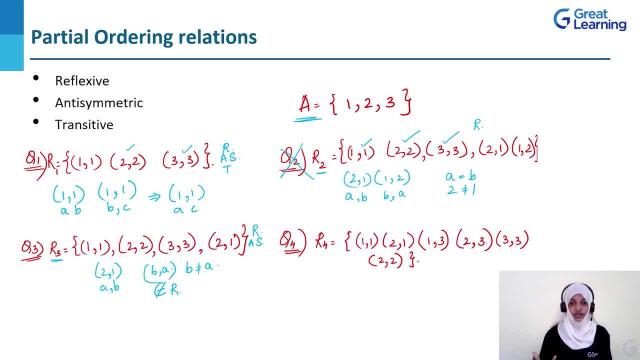 why not? belonging to the relation is actually converting this relation into an anti-symmetric relation. Next, let us look at whether this relation is transitive. Again, if we look at 1,1,, 2,2 and 3,3 from, 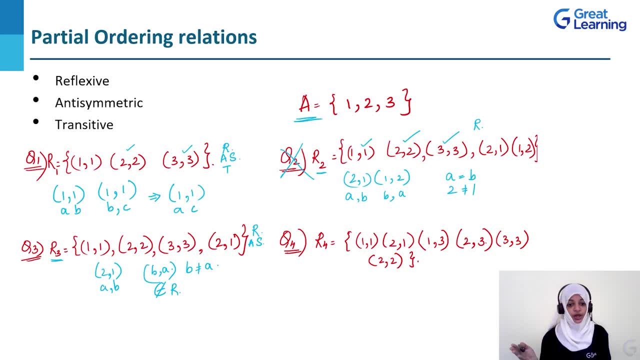 example 1,. we already know that these are transitive in nature. What about 2,1 is an ordered pair which is not continuing anymore. We've only got ordered pair of the type that is: There are no, nor are there any. 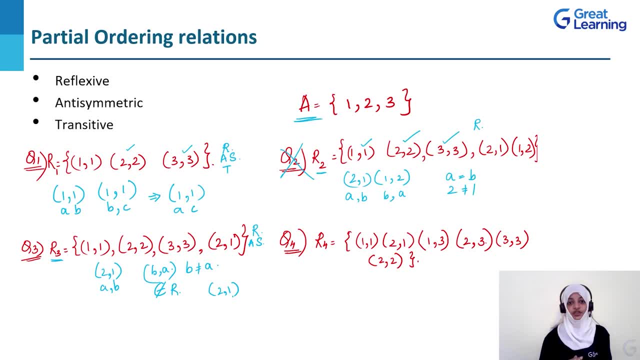 related to this. As a result from our definition, we can say that this particular relation is transitive also. Thus we can identify that relation R3 is a partial ordering relation. Next, let us look at example 4.. We have 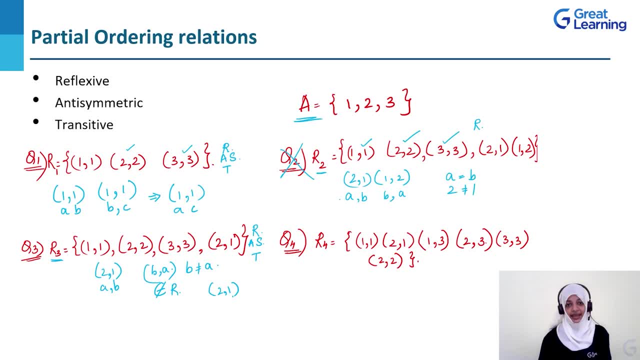 relation 4, again set on the set of values. A Relation 4 consists of 1,1,, 2,1,, 1,3,, 2,3,, 3,3 and 2,2.. From this we can: 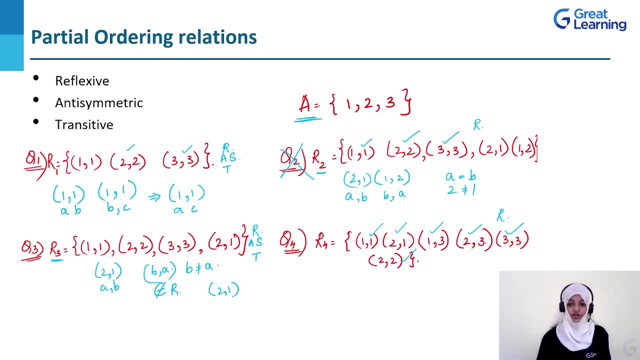 understand that this particular relation is reflexive in nature. Let us see whether this relation is transitive in nature. We've got the set here: 2,1.. Both the values are different and there is no set corresponding to it as 1,2.. 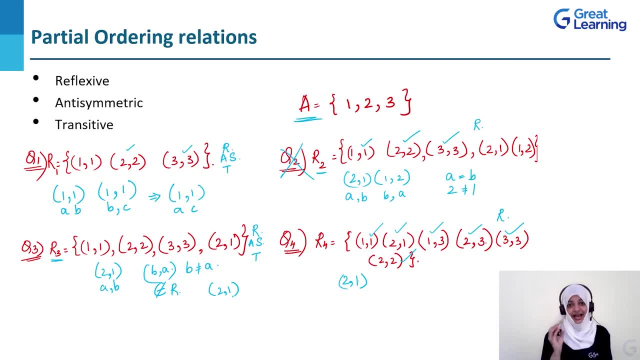 Thus this particular ordered pair is antisymmetric in nature. Next, let us look at 1,3.. We find a similar possibility there. Again, we've got 2,3 having no corresponding 3,2, and both the values are different. 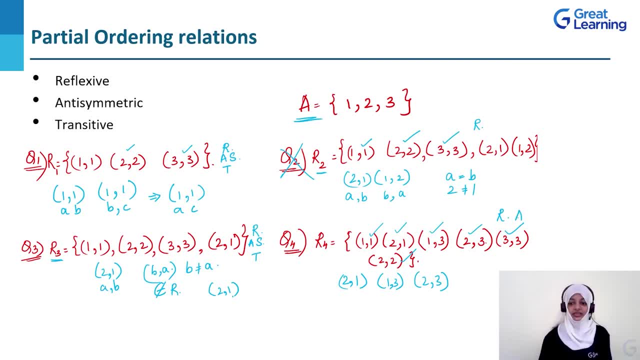 Thus, this particular relation has an antisymmetric property attached to it. Lastly, let us look at transitivity. Looking at the example given here, we already know that 1,1,, 2,2 and 3,3 are all going. 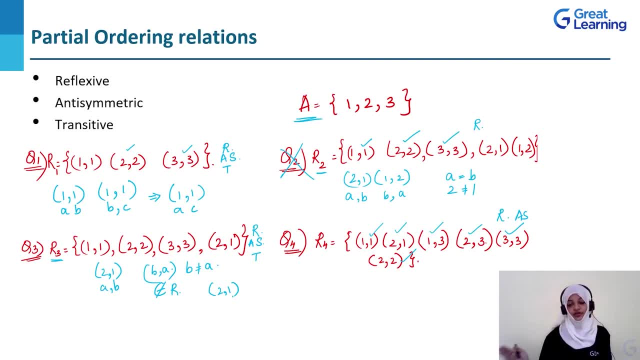 to be transitive in nature. What about the rest of the ordered pairs? We've got the ordered pair 2,1 and 1,3.. These can be considered as AB and BC. Ideally, we should be having 2,3 as an ordered. 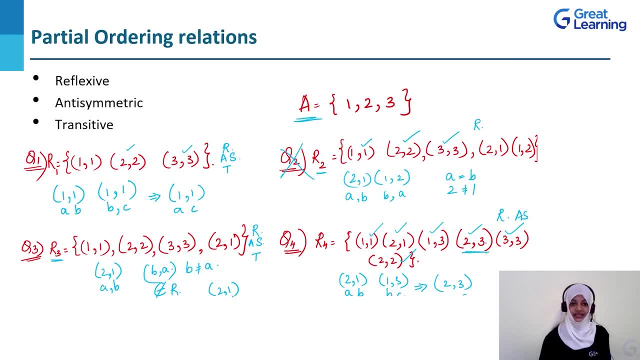 pair of the type AC. Since it exists, we can say that there is a transitivity relation. But this is not enough. We need to check for all of the ordered pairs available here. Checking for 1,3.. 1,3 can be matched up. 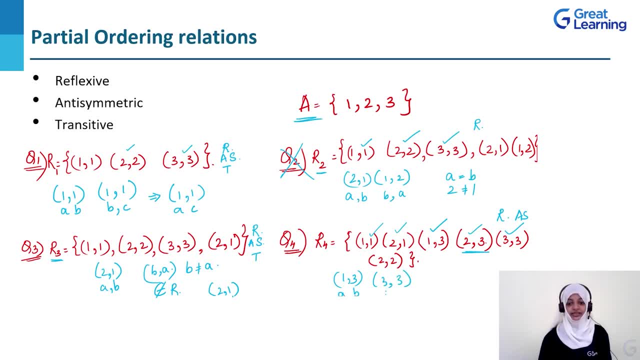 with 3,3.. So this is AB and this is BC. Ideally, we should be getting 1,3 as AC. All of these 3 exist as a part of our relation. Next, let us look at the ordered pair. 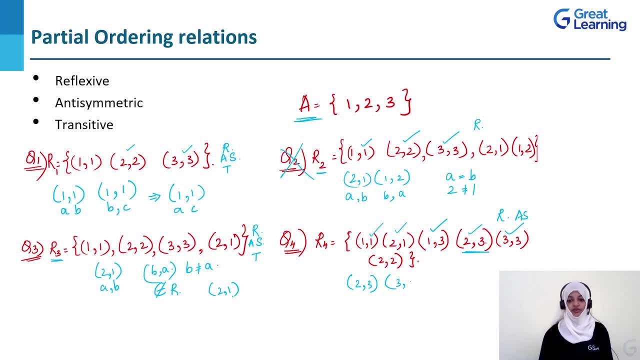 2,3.. 2,3 and 3,3 will exist in a relation here as AB and BC. Ideally we should be having 2,3 as a part of the relation as AC. All of these 3 ordered pairs. 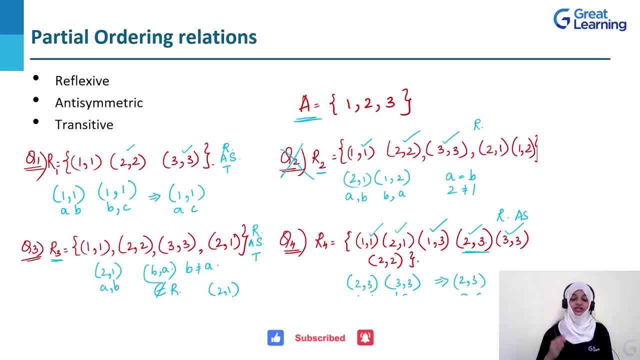 exist in the relation. As a result, we can say that each and every ordered pair here in this relation has a transitive nature. Since all the ordered pairs are reflexive, antisymmetric and transitive in nature, we can say that relation 4 is a partial order. 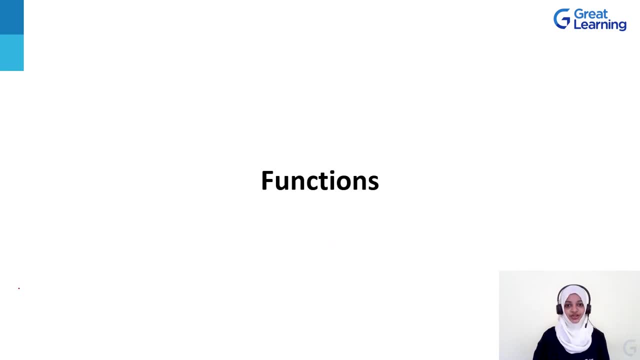 relation. Hello everyone, Welcome to this session on functions. In our early schooling days we have learnt various functions, Some functions such as quadratic functions. We have learnt functions such as polynomial functions. We have also learnt functions like trigonometric or rational. 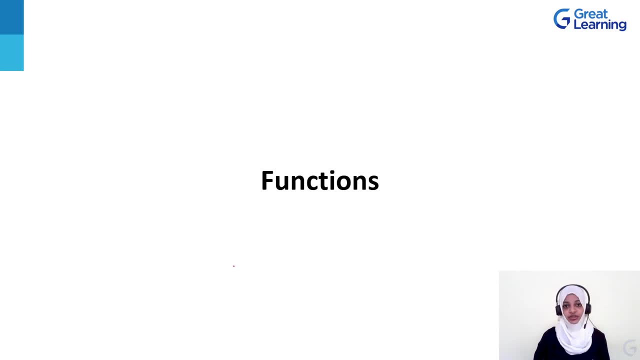 functions. So in this session we are actually going to see what these functions are. Now, functions are a very important part of either normal or discrete maths. This is because functions are generally a formation of calculations that take a certain input and provide. 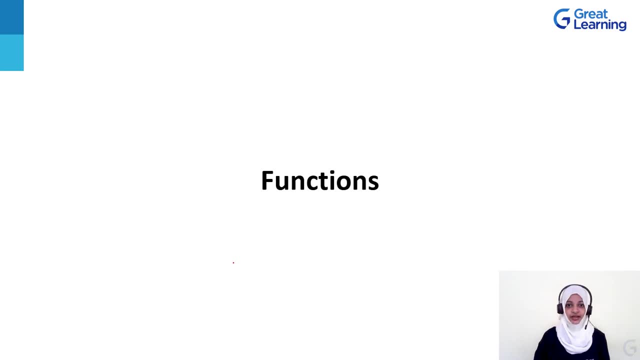 us with an output for it. So let's get started. In this session, we are going to understand exactly what functions are and what are its components. After understanding that, we are going to look at the most commonly used types of functions. 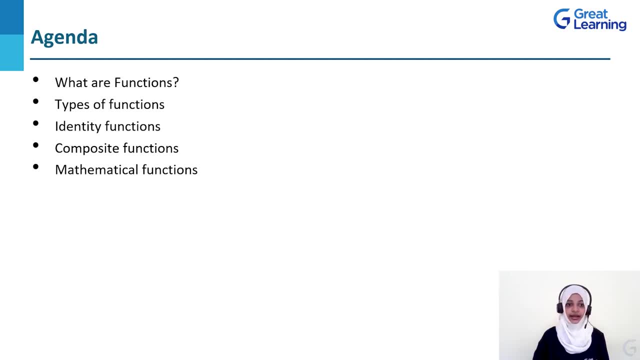 There are five types of functions, as we will be seeing ahead. Next, we are going to look at a specialised type of function known as identity functions. Furthermore, we will then be looking at what a composite function, or it's also known as composition of functions, actually 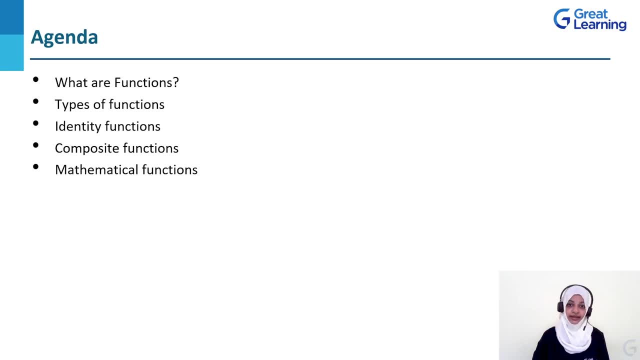 means, How can they be worked through and what are the complexities there? Lastly, we will be looking at some of the most commonly used mathematical functions that are often translated into programming languages. So let's get started. So, as we have already seen, 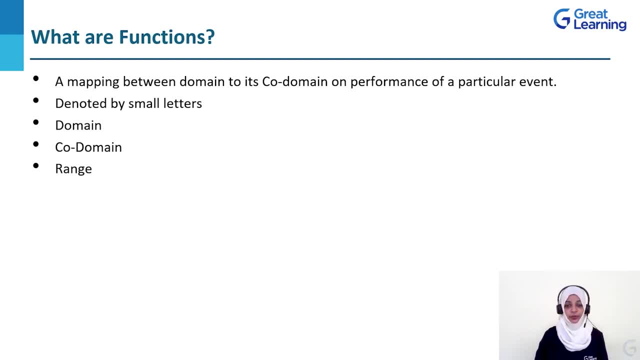 relations are actually the relationship between two different sets that we might have under consideration. Functions are a specialised relation. This means that the function will inherit all of the qualities that were there within relations. This implies that functions would have a certain set of inputs, and these inputs would 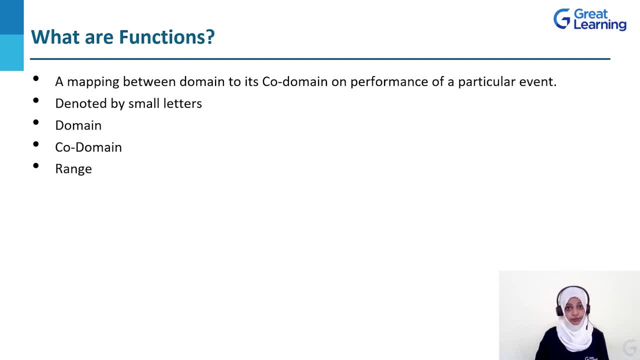 actually help us generate outputs. Furthermore, by looking at relations, we have seen something known as ordered pairs. Functions carry forward these traditions of ordered pairs. Now we will often see functions denoted by small alphabets. These alphabets commonly used. 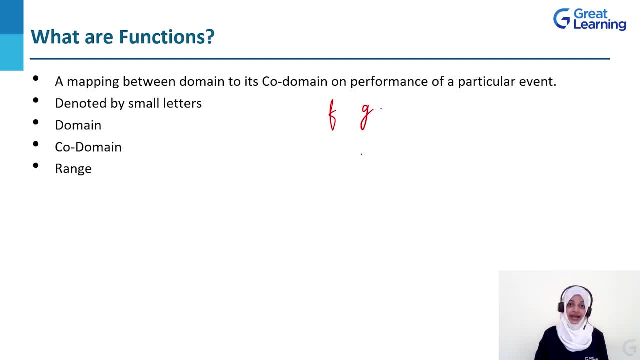 are F and G Again, as we had in relations. we may use other alphabets too, But these are the most commonly used ones. Also, please note that while relations are denoted by capital letters, functions are specifically denoted by small letters. 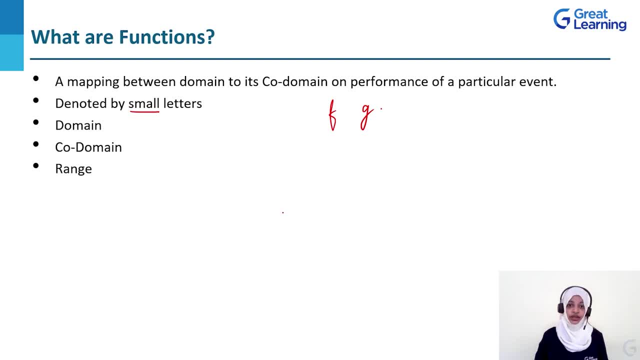 The mapping of function is also created from one set to the other. As a result, you will often see functions defined as the notation of the function under consideration, such that it is on set A going to set B. This notation is often followed by a description. 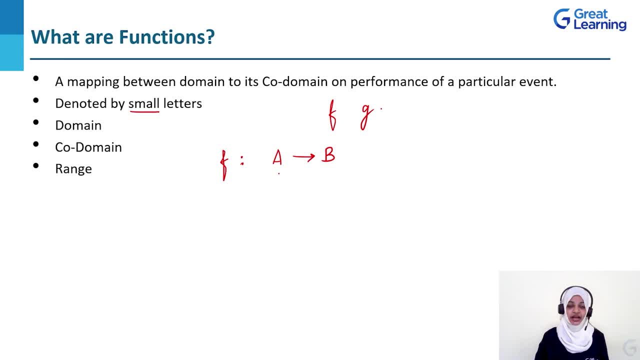 of what the function is trying to perform. Let us understand what these A and B actually stand for. Consider a set A. Since the arrow is pointing from A to B, we can say that the set A acts as the set of inputs and the set B 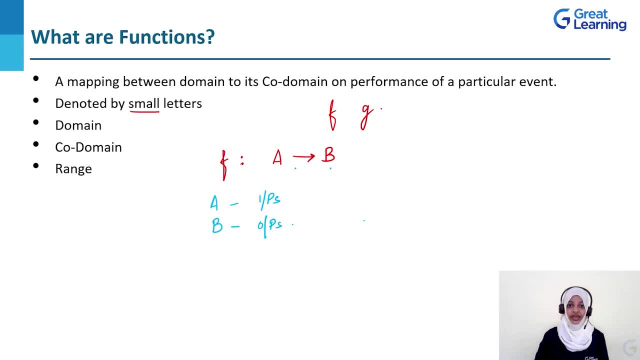 are the set of outputs. As a result, we have three components in functions. Three components, But I just denoted two here. Yes, it's three components. Let us look at the various components here. First, we've got the domain. 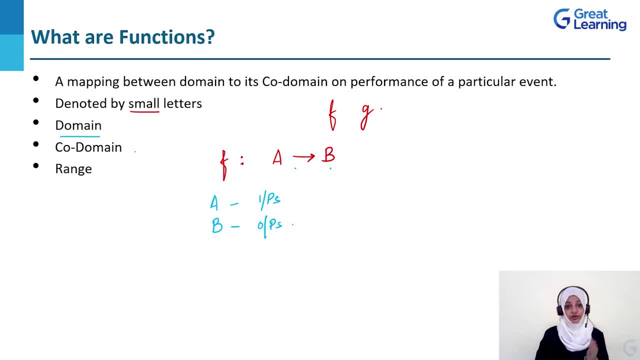 The domain is actually the set of possible inputs that can be provided for the function. It basically means that in this function given here, A is the domain, since it is the set of possible inputs. Next we've got the set of possible outputs. 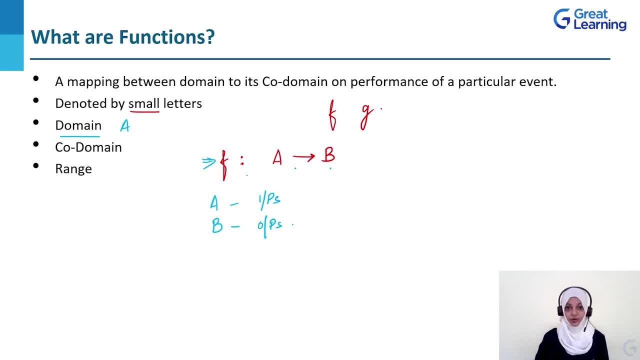 As I said, it's the set of possible outputs. It is not the set of all outputs. So the set of possible outputs are known as co-domain. The object B here actually belongs to the co-domain. Lastly, we've got the 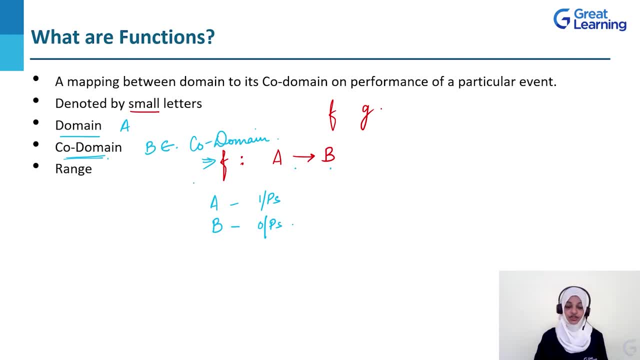 actual set of outputs that will be provided by the functions on processing the input. This is known as range Set B. here is actually the range, As we can see, because of the function going from a set of inputs to a set of outputs. 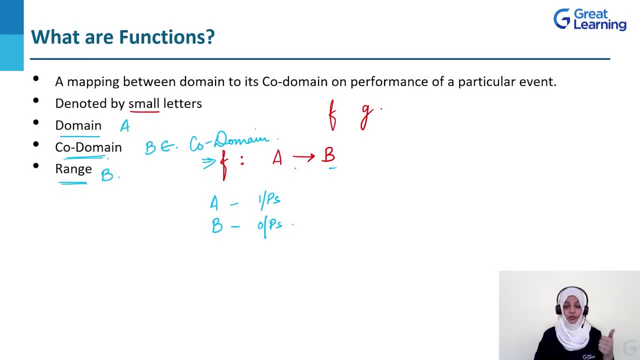 we actually get three different components: The domain, which is the set of inputs, the co-domain, which are the set of possible outputs, and the range, which is the actual set of outputs. Thus, any function that we look at, be it a polynomial function, 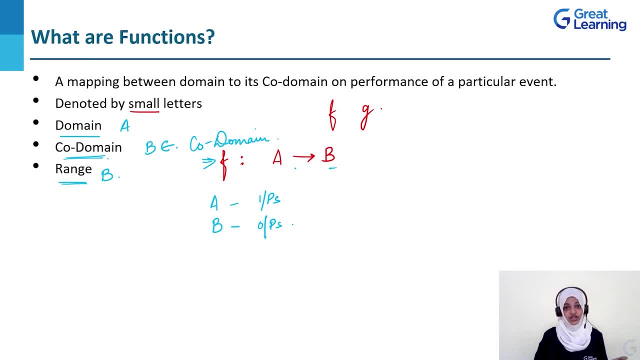 be it a quadratic function, a trigonometric function, a rational or an irrational function or any other type of function, all of them will always have a domain, a co-domain and a range, And the function will work such that it will always move. 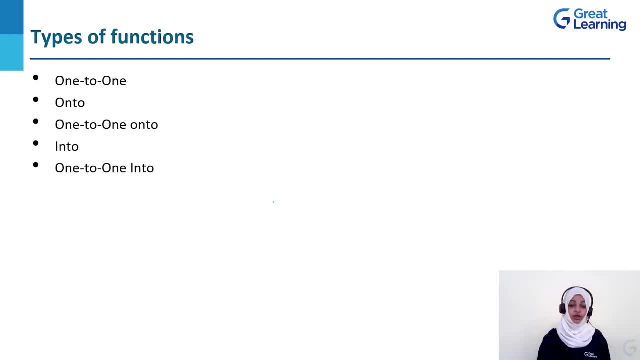 from the domain to the range. Next, we're going to look at what are the type of functions. The first function that we're looking at here is the one-to-one function. The one-to-one function is also known as an injective function. The one-to-one 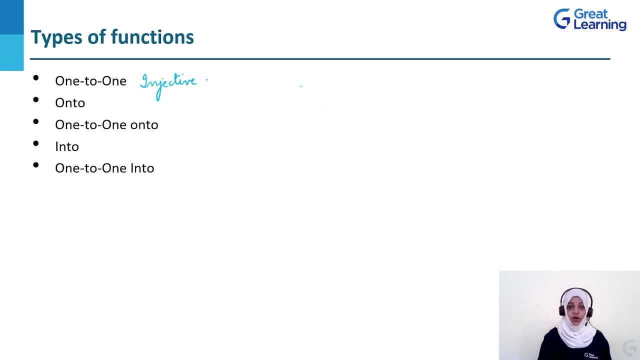 function is defined as a function such that one member in the domain is related to one member in the co-domain or the range. For the purpose of these examples, let us consider co-domains, So every time we've got one element in the domain. 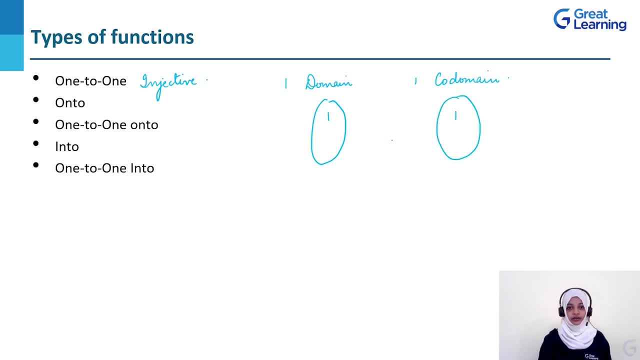 it would be related only to one element in the co-domain. That means there is a one-to-one relation between the two sets. What happens if there is one element in the domain and it is related to two elements in the co-domain, In this case the function? 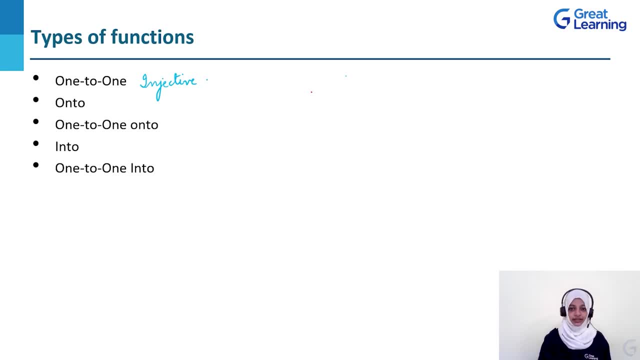 no longer remains one-to-one. To better understand this concept, let us take two examples. Say, our first example is a function going from the set of real numbers to the set of real numbers. In this case, both the domain and the co-domain are a set of real numbers. 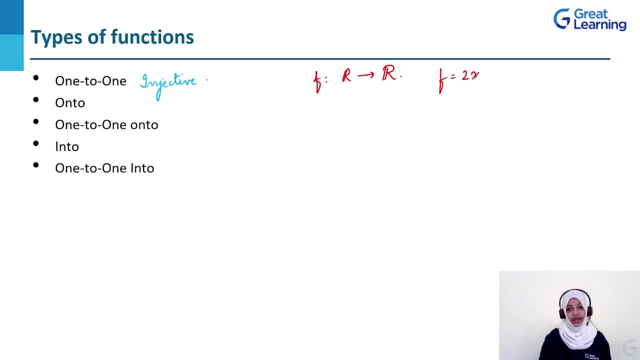 If the function f is defined as 2x, let us see whether this particular function is one-to-one or not. Mathematically, in order to check whether a particular function is one-to-one or not, we use a very simple methodology. A function is: 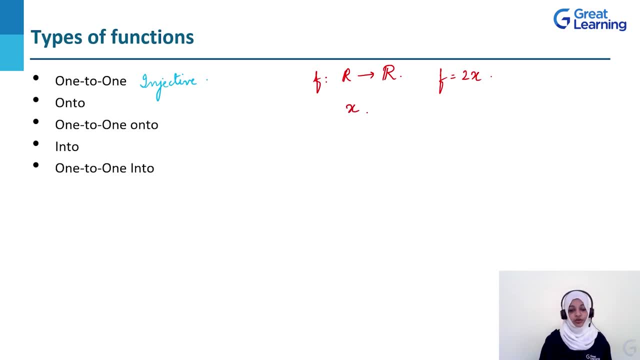 said to be one-to-one if, on taking two inputs from the domain- x1 and x2, we get two outputs, f of x1 and f of x2, such that x1 and x2 are both equal to each other, thereby making f of x1 equal. 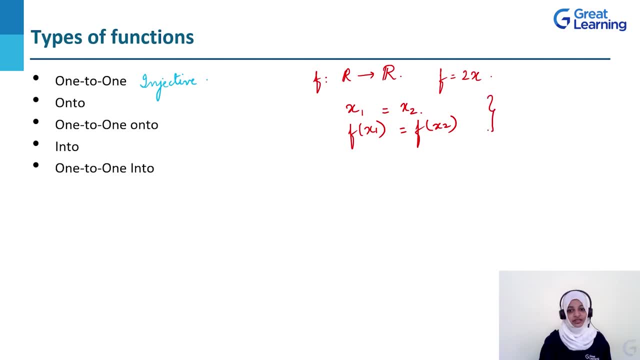 to f of x2.. If we implement this particular concept mathematically, it becomes easy to understand whether a function is injective or not. There are two ways of understanding this. One is by using an example, and the other is by using generic values. 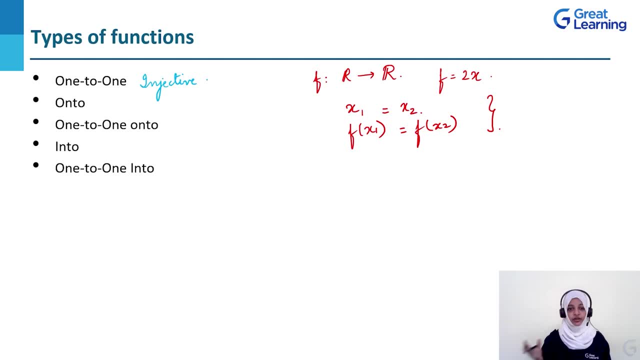 The generic value is the most commonly used method of resolving this. Let us see how it works. Let us take two values: x1 and x2.. We do not know whether these two values are equal to each other, yet Let us take function and assume. 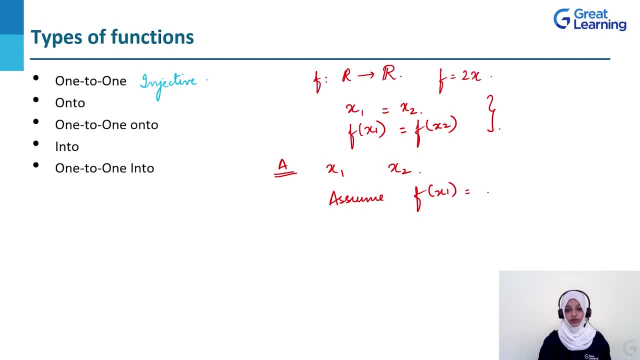 that f of x1 is equal to f of x2.. Substituting our function within f of x1 and f of x2, we get that 2x1 is equal to 2x2.. Deleting 2 from both sides. 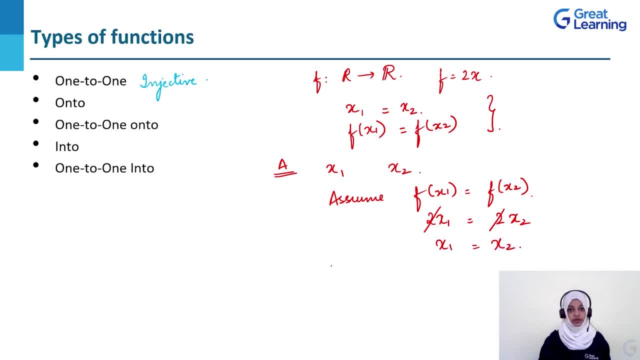 we end up with: x1 is equal to x2.. Thus, using the outputs, we have proven that the inputs were actually equal to each other. So if the outputs are equal to each other and the inputs are equal to each other, that means for one value. 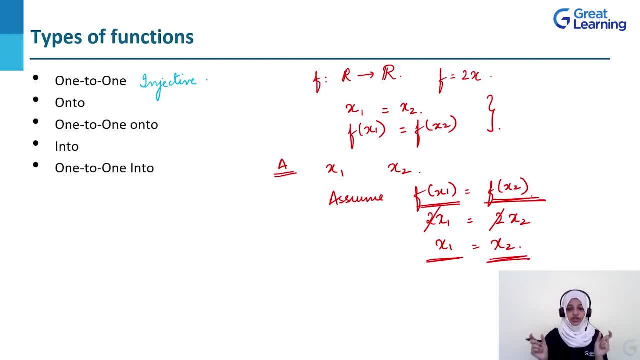 of domain. we have just one value within the range associated with it. This is how a one-to-one element looks like. Next, let us look at how a function which is not one-to-one will react. Let us take a function such that it goes from: 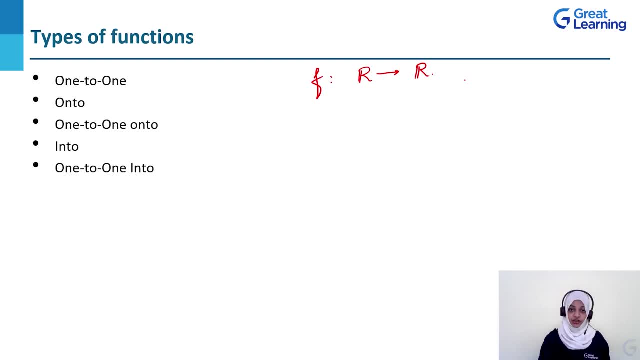 r to r, which is again the set of real numbers, but the function is such that it is defined as modulus of x. Modulus of x actually means that it is the positive value, irrespective of whether x is a positive or a negative value. We are just. 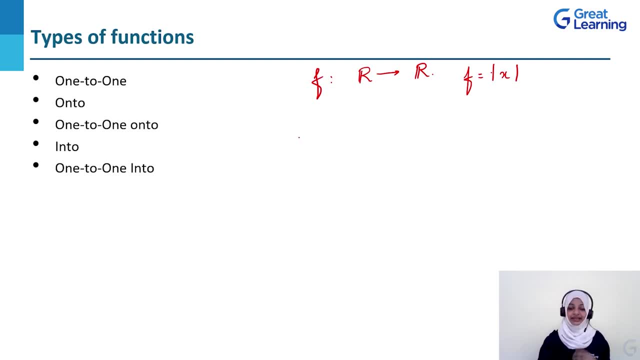 taking the quantity here. That is what this modulus means. Let us apply the same methodology of generic values to this particular question and resolve whether this is one-to-one or not. Firstly, let us assume that we have two values, x1 and x2, which are inputs for. 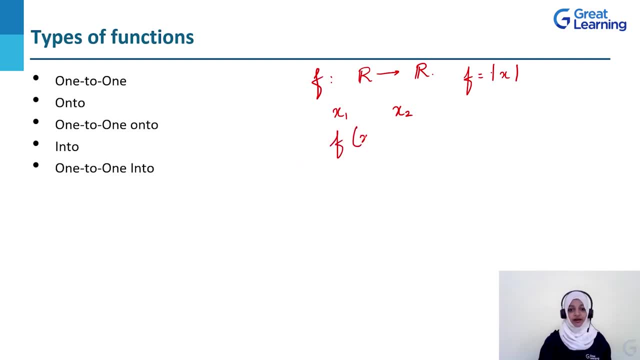 this function. Let us then assume that we have f of x1 is equal to f of x2.. If f of x1 is equal to f of x2, this will mean that modulus of x1 is equal to modulus of x2.. Trying to 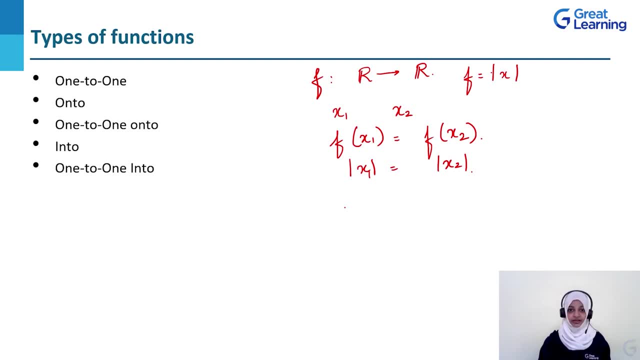 resolve the modulus is very simple, but it is also pretty daunting to some. That is because while resolving the modulus, you will often see answers like this: If resolving the modulus here, we will get, x1 is equal to x2, but this x2 can either be. 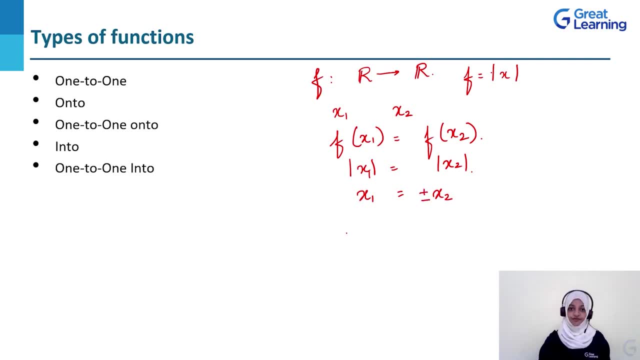 plus x2 or minus x2.. If we consider the values here, this means that x1 can be equal to x2, but on the other hand, x1 can also be equal to minus x2.. If it is x2, we would. 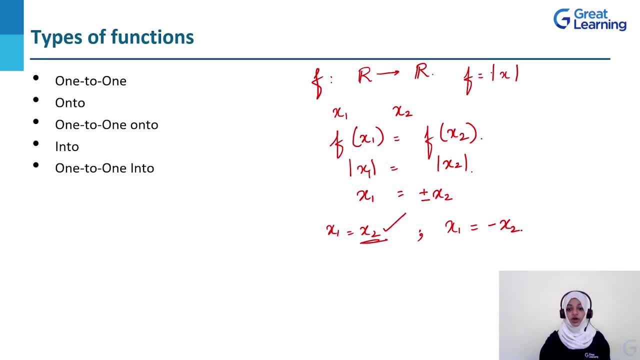 say that it is injective in nature, but because there is also an advent of minus x2, these can't be equal to each other. As a result, there is a contradictory result here On getting f of x1 equal to f of x2,. 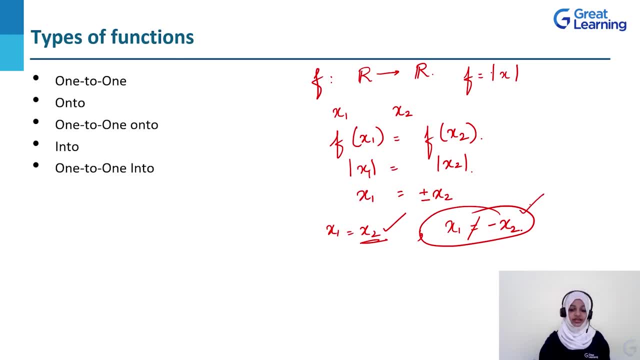 we are not able to get. x1 is equal to x2 unequivocally. As a result, this particular function is not injective. Next, let's look at the onto function. The onto function is also known as the surjective function. 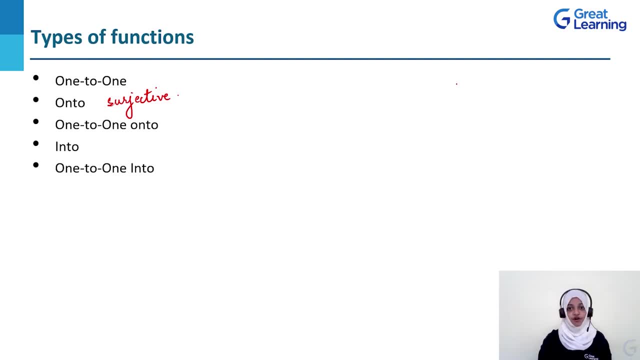 A function is said to be surjective if, for each and every element in the codomain, we have a corresponding preimage or a corresponding related value in the domain. This means that, as in 1 to 1, instead of going from the input to the output. 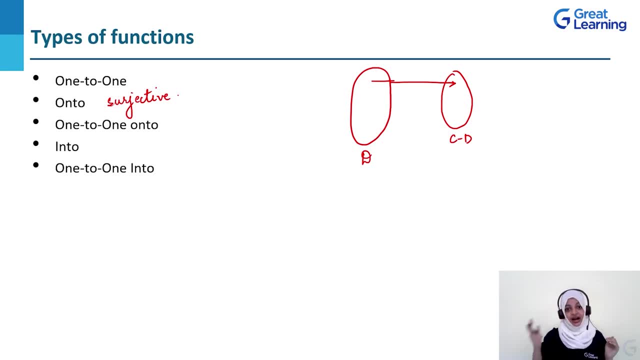 for onto we actually go and check whether outputs have inputs or not. If we have an example, if even a single element in the codomain does not have a related preimage in the domain, then the function is said to be non-surjective, or 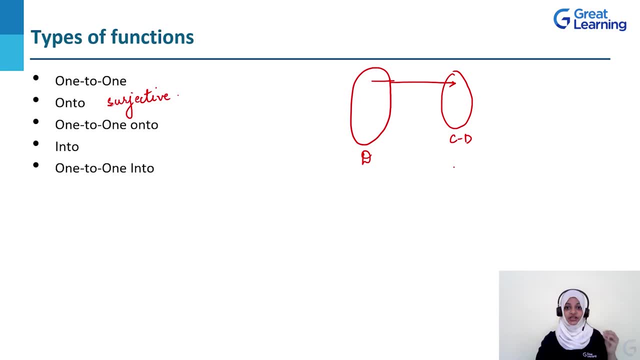 not onto in nature. This means that each and every element that is a part of the codomain has to have its preimage, or it has to have a related input in the domain. Let us understand this with the help of this example. As we can see here, we have 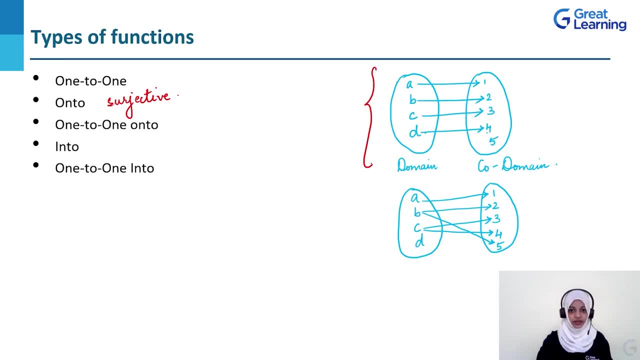 two examples: The first one given here and the second one denoted here. Look at example 1.. We've got a set of 5 elements in the codomain and a set of 4 elements in the domain. If we look at this, we can see that each 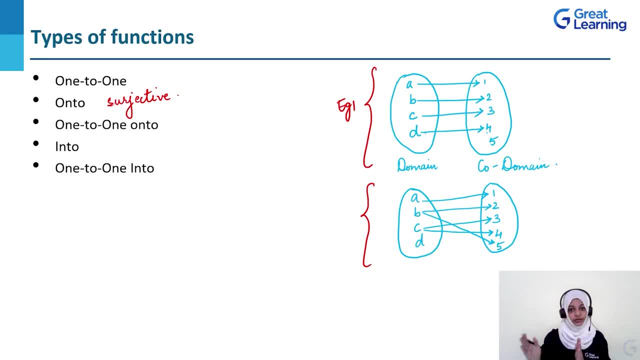 and every element of our domain is related to only one element in the codomain. Looking at this, we may say that this particular function denoted here would be 1 to 1.. On the other hand, look at the codomain, As you can see. 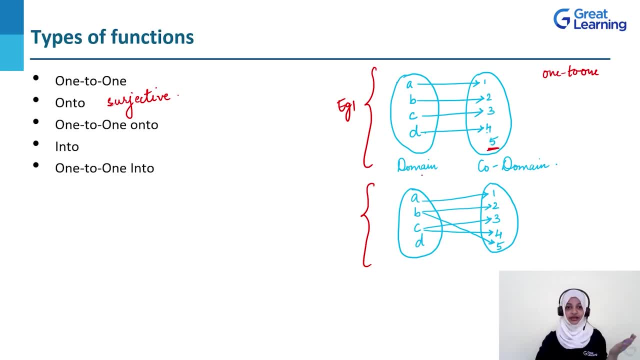 there is one element 5, which does not have any related element in the domain. This is where we can say that this particular function is not onto. That is because we have one element in the codomain which does not have a preimage or a related element. 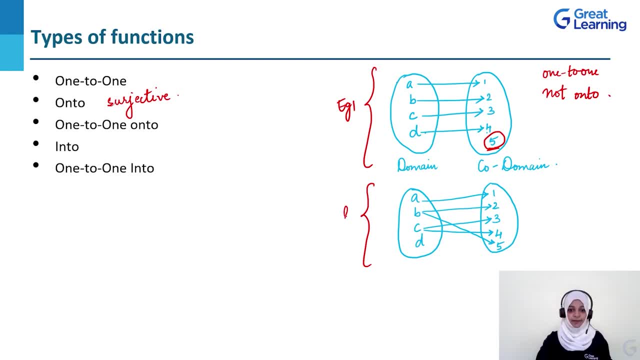 in the domain. Let's look at example 2. on the other hand, Here we've got two elements of the domain b and c, which have two elements related to them in the codomain. As a result, the function here is not a. 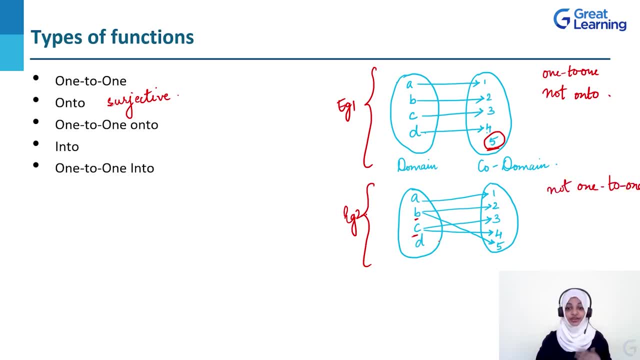 1 to 1 or not an injective function. On the other hand, let's look at the codomain. Each and every element in the codomain is actually related to any one element, at least within the domain. This means that there is no such. 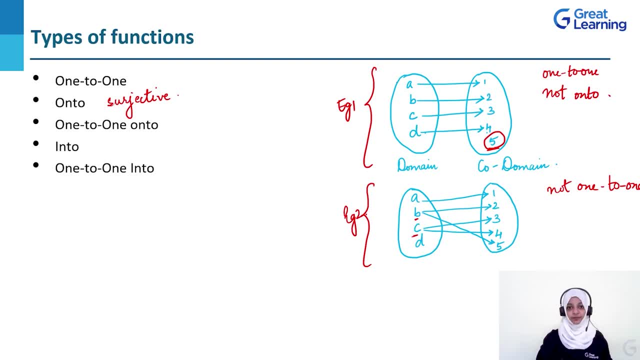 element which does not have a preimage in the domain. Thus this function can be called an onto function. Let us also understand this with an example, a mathematical one, that is. Let's consider a function f such that it moves from set of real 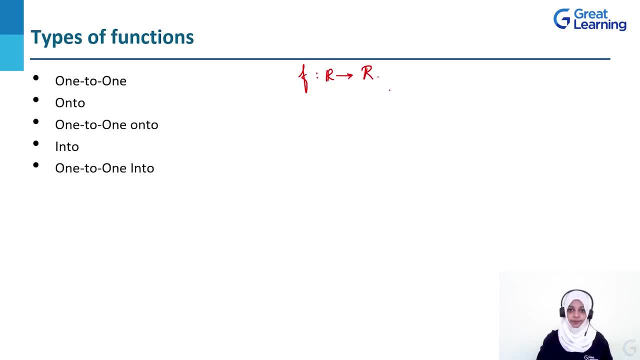 numbers onto another set of real numbers. Here, let the function be defined as modulus of x. As we already have seen in the previous video, modulus of x is not an injective function. Let us now check whether it is a surjective function. 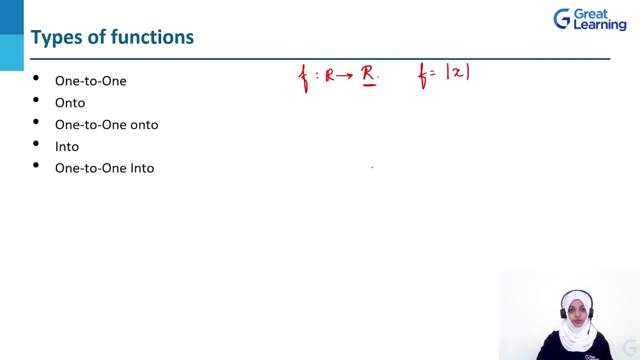 If we look at our codomain, we've got a set of possible values as the set of real numbers. These real numbers would be negative integers, positive integers, decimals, rational numbers, irrational numbers and all the values in between Till they are not. 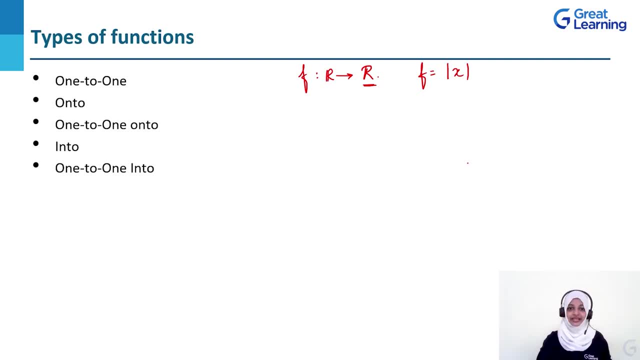 imaginary they would be a part of the set of real numbers. Let us take one single example of a real number that, ideally, is a part of the codomain. For example, let us take minus 2.. Minus 2 is a part. 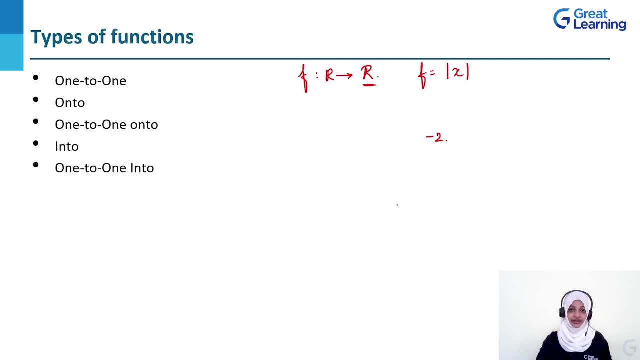 of the codomain. The question here is: can it be an output of any function? As we know, modulus of x is such that it will always give us a positive answer. That is exactly how the operator works, Irrespective of whether the value 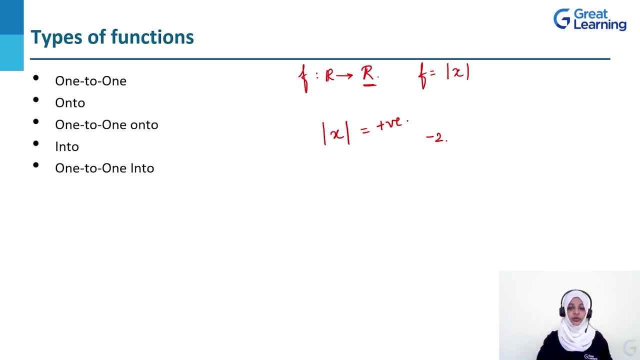 given to it is positive or negative, it will provide us with a positive answer. Minus 2 being an answer is not possible, since it's a negative number. As a result, all the set of negative integers, whether whole or decimal based, will never be. 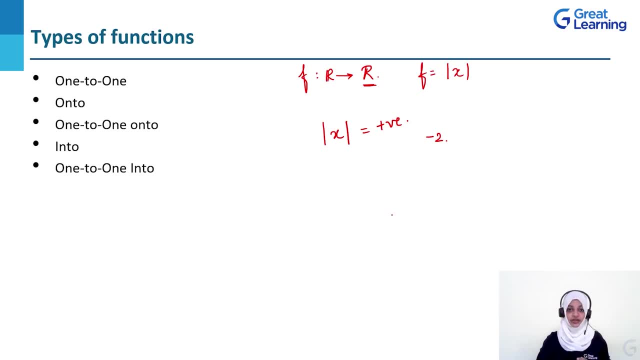 considered as a part of output. As a result, all of these values will be the values which do not have a pre-image in the domain or do not have any related inputs, even though they are contained within the set of possible outputs. Thus, this particular 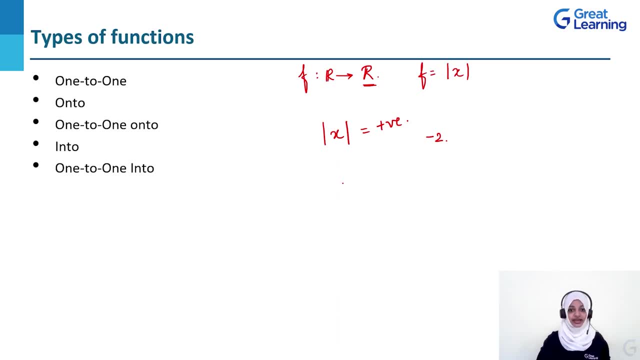 function here. modulus x actually is not surjective in nature or is not onto in nature, because all the negative values that are there as a part of the core domain will never have a related input in the domain. Let us look at another example here. 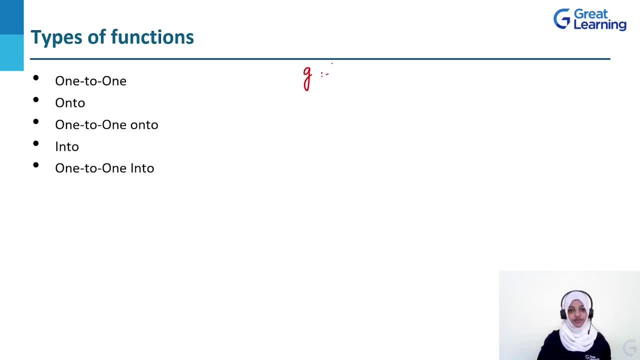 Say, we have a function g such that it goes from set a to b where set a is defined as r minus 2 and set b is defined as r minus 1. So that means our domain cannot contain 2 and our range can't contain. 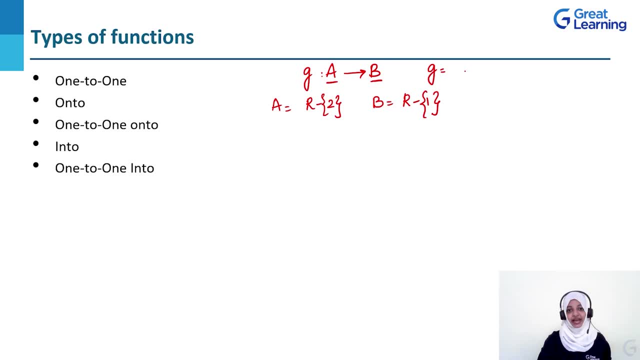 1. And let g be defined as the function. say like this: wherein f of g is equal to x minus 1 upon x minus 2.. Let's see if this is a surjective function or not. Let's consider g of x as a value y. 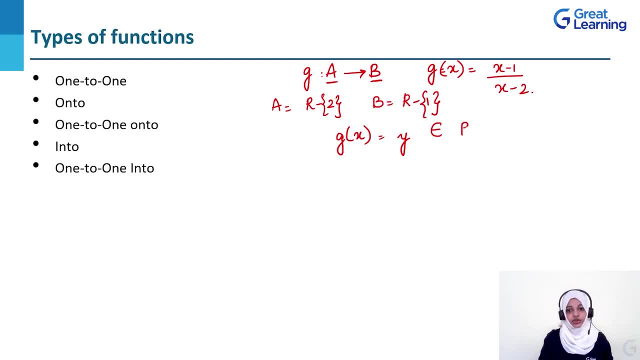 such that this particular value belongs to our core domain. Thus, looking at this particular function, we can say that y is equal to x minus 1 upon x minus 2.. Next, let us rearrange this a bit, So we get y into x. 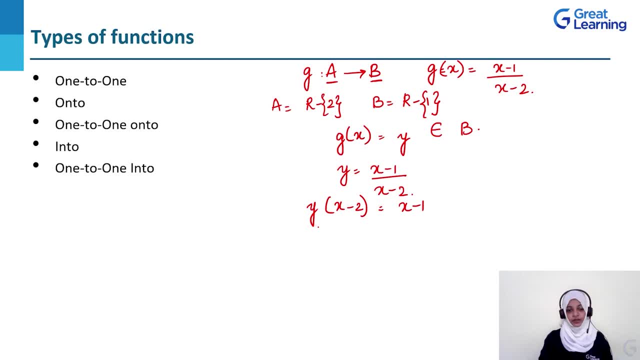 minus 2 is equal to x minus 1.. Opening up the bracket, we get xy minus 2y is equal to x minus 1.. Club together all the terms containing x and all the terms containing y, We'll get xy minus x is equal to. 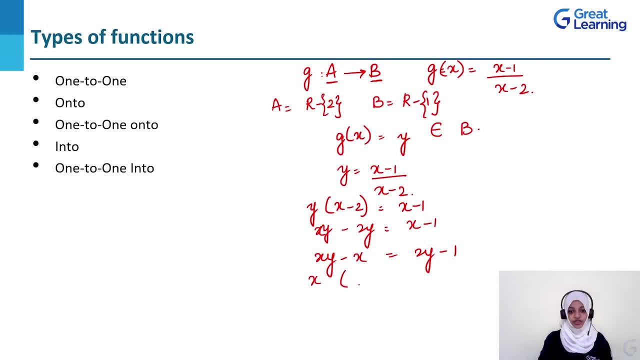 2y minus 1.. Take x out as common and we get something like this: This means that x is essentially equal to 2y minus 1 upon y minus 1.. From this particular equation we can state that it's possible to get any. 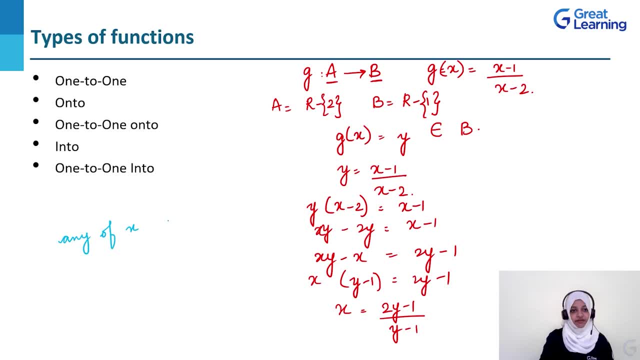 value of x as long as we have a value of y wherein y belongs to b. Now, why is this possible for us? What happens if the denominator becomes 0? Well, fortunately, the denominator will never become equal to 0. That is. 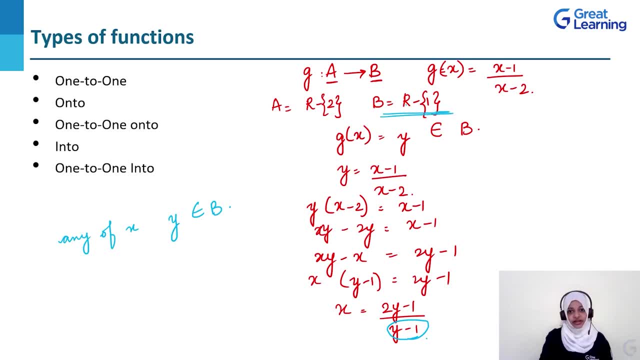 because b is defined such that it contains all the elements of the set of real numbers but excludes element 1. So it's possible that for every element of y we'll have a relation related element of x which will be a part of the input. 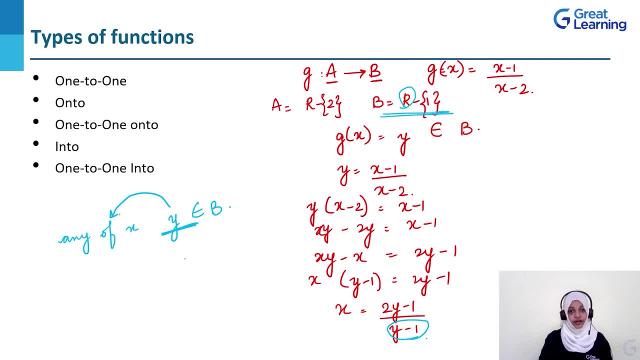 This actually implies that for every element belonging to the codomain, we have a related element that will belong to the domain. This means that the function given here is surjective in nature. Next we're going to look at another kind of function known. 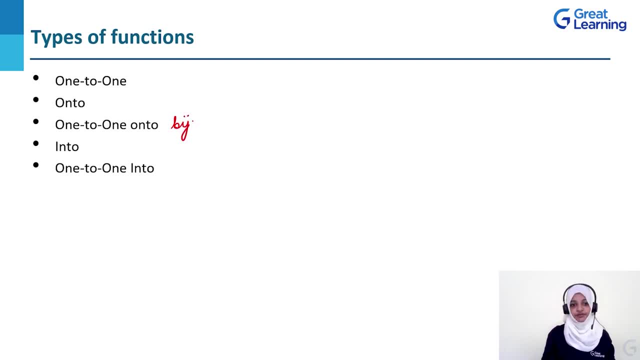 as the one-to-one, onto or the bijective function. Most of you might have already understood what it entails. If any function is both one-to-one as well as onto, or injective as well as surjective, then the function is automatically known to be bijective. 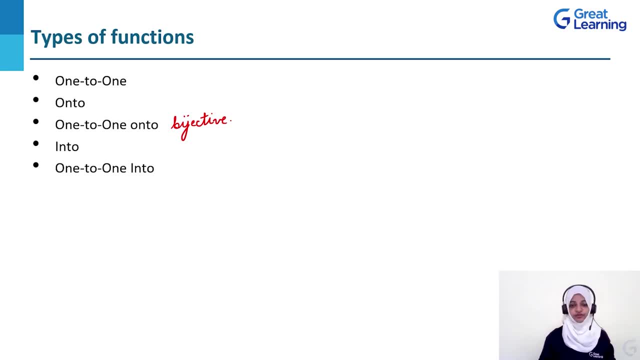 in nature. It is also known as the one-to-one onto function. You can use any of these terms. Let's look at an example of the same Say we have a function f such that it is drawn on the set of real numbers to the set of real numbers. 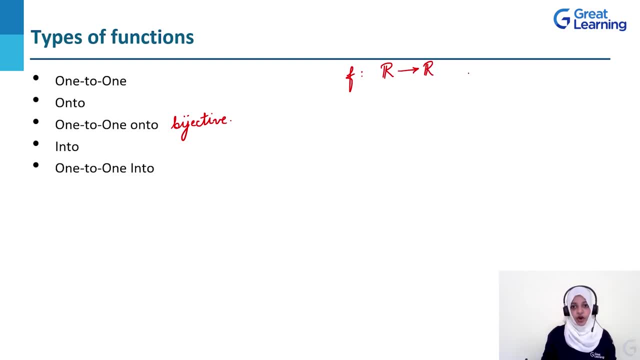 Let the function f be such that we've got the function f defined as 3x. Let us check if this particular function is injective in nature. Let us consider two input values, for example x1 and x2, such that f is: 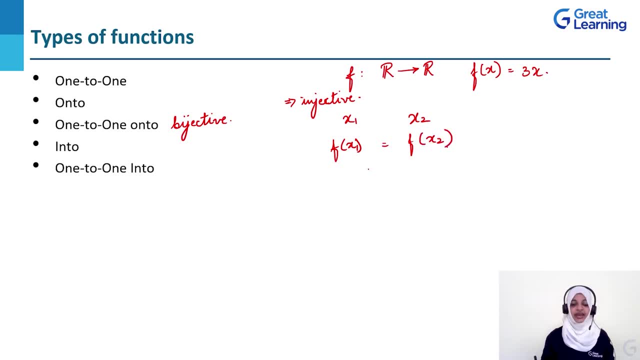 equal to f. If f is equal to f, we can say that 3x1 is equal to 3x2.. Canceling out the 3s on each side of the equal to, we get that x1 is equal to x2.. 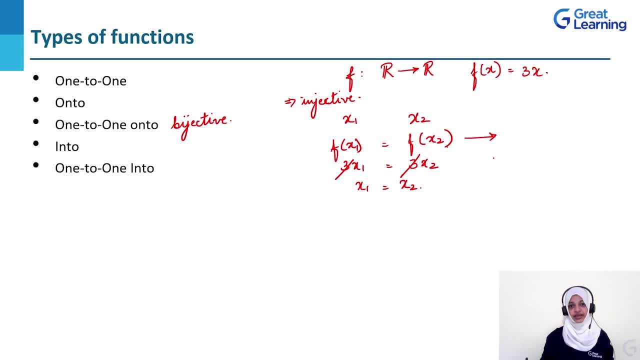 This means that if the final answer of the function is the same, then even the initial values considered as inputs for the function would be the same as each other. That means that this particular function is injective in nature. Next, let us consider whether 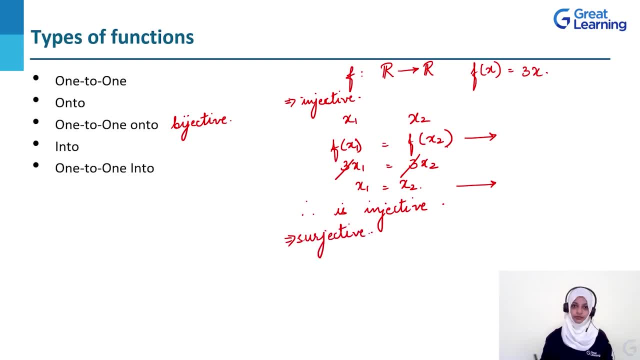 this is surjective in nature or not. Let us consider a function such that f is equal to some y, where y belongs to the set of real numbers which is a part of the codomain. From the function we can now say y is equal. 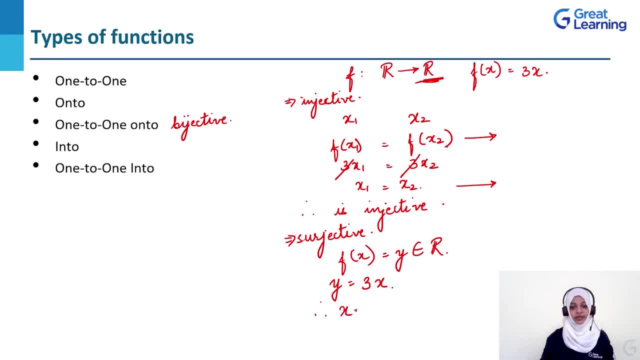 to 3x. Therefore, x will be equal to y upon 3.. This means that for any value of y belonging to the codomain, there will be a preceding input value of x, which actually belongs to the domain. Thus this particular 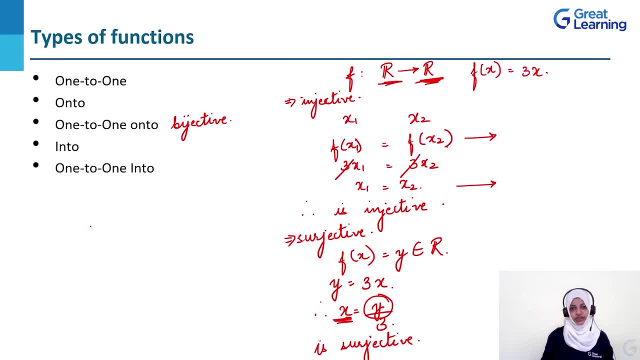 function is surjective in nature. A point to be noted here is that if we take the exact same function and try to build that function on the set of natural numbers, this particular function would not be surjective in nature. The reason behind that is very simple. If we 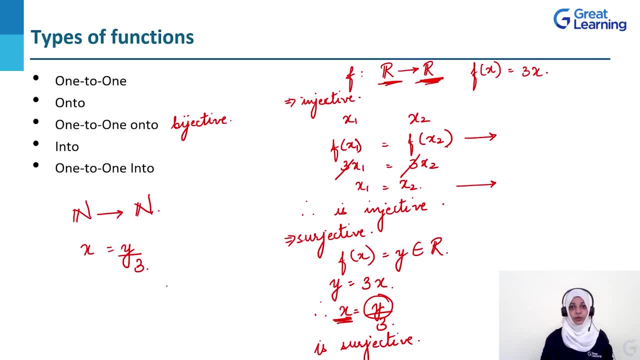 take x is equal to y upon 3, we will see that we could either have x as integer values or whole numbers. There is no guarantee of what you might have If it is a set of real numbers that is acting as the domain. 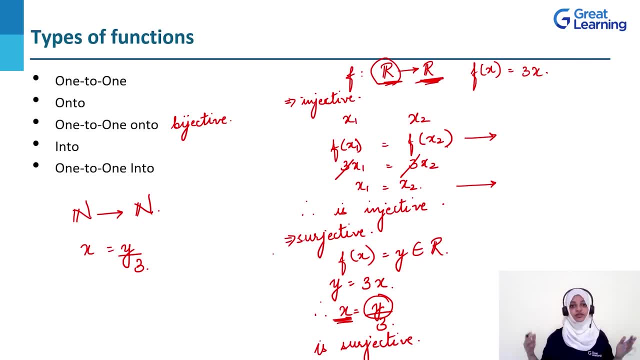 this set would contain all the decimals as well as whole values, thereby giving us no issue to claim that every codomain element will have a preimage in its domain. On the other hand, looking at natural numbers, natural numbers contain all the values except 0.. 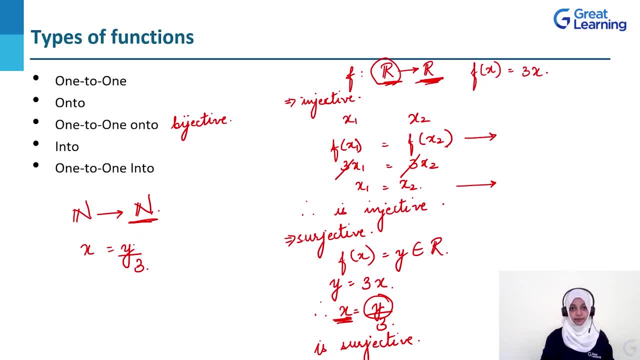 There is no space for decimals here. A value of y divided by 3 might give an equivalent value of x, which is actually a decimal. This decimal will not exist in the domain, since even the domain is a set of natural numbers. This actually goes to show that. 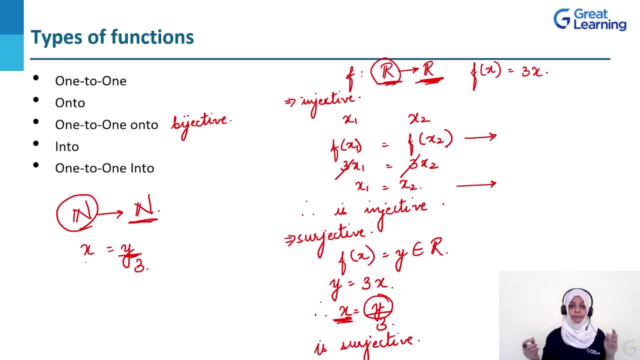 function is not only based upon the equation, but also upon the domain and the range of that particular function. Next, let's look at the into function. After I've explained the into function, you might feel that it's the opposite of the subjective function, and you won't. 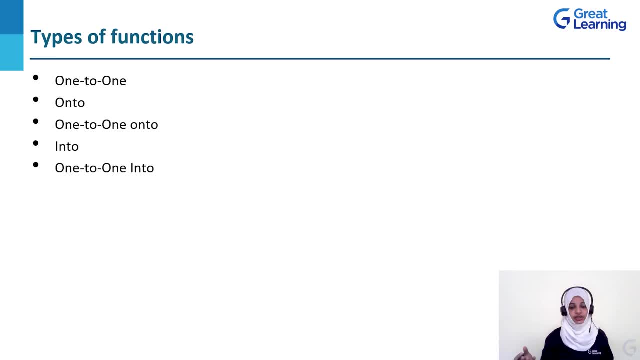 really be wrong. As we've seen in the onto function, there is a compulsion that each and every element of the codomain should have a related element within the domain. In into functions it's the exact opposite. The into function actually states. 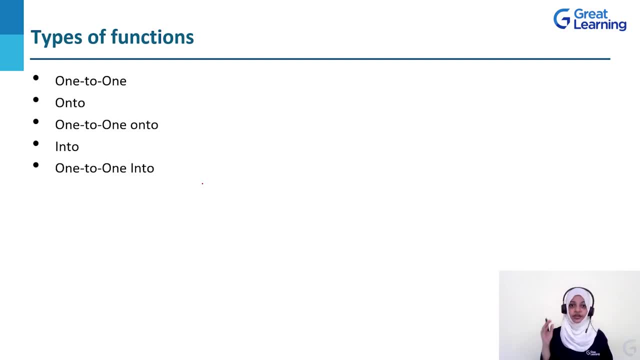 that there needs to exist at least one element in the codomain that does not have a related preimage in the domain. This means that each and every function that is not subjective in nature often becomes into in nature, So this means that each and every question that we've 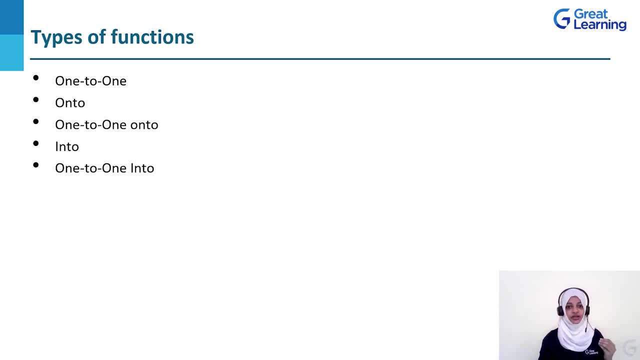 seen till now, which is not subjective, becomes a part of the into functions. Let's look at the next topic here, which is one to one into. This means that any function which is one to one that is injective in nature but not subjective in nature. 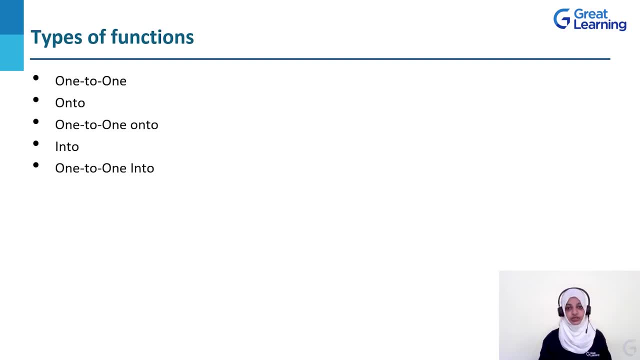 would be a part of one to one into functions. Let's look at into functions with an example and let's look at one to one into also. Firstly, going to the into function example, if we've got two sets such that we have set A is 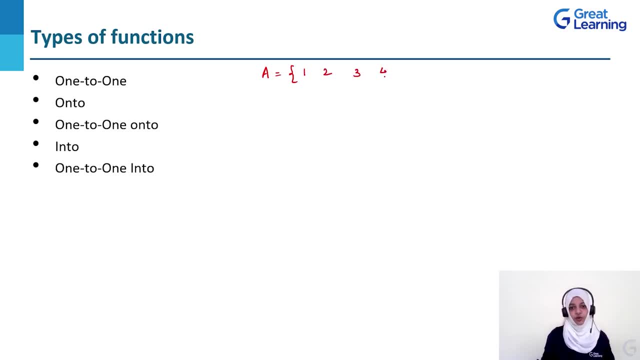 equal to one, two, three and four, And we have set B equal to A, B and C. Let's take two more elements, D and E. Let there be a function F, such that at the end, after carrying out all of the calculations, 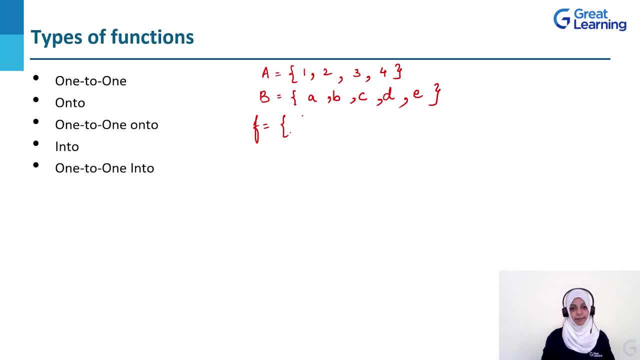 we get an input output ordered pair of this type: 1A, 2B, 3C and 4D. As we can see, the function is going from A to B. Also, as evident here, there is one element E that has not come. 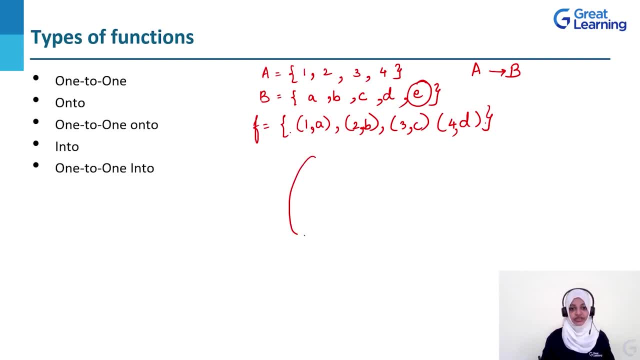 up as a part of the output, If we show this as a diagram so that we better understand this. we've got the domain here as one, two, three and four and we've got the co-domain here as A, B, C. 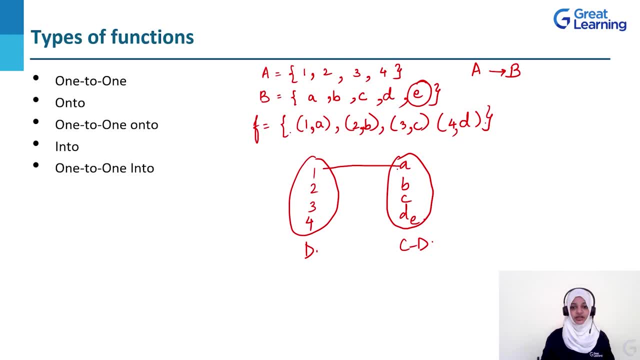 D and E. Each and every element here has a pre-image on the domain, all except the element E. As a result, E is one such element not having a pre-image in the domain, and thus it makes this whole function into in nature. Let's take an example of: 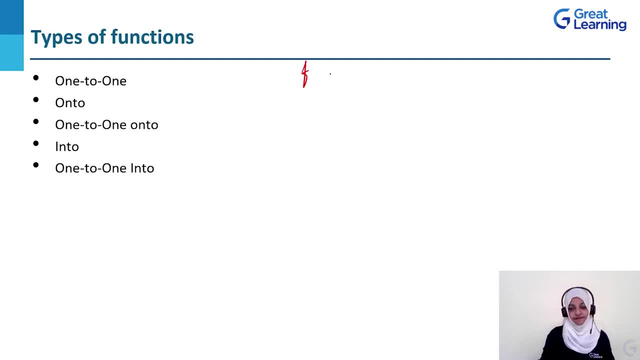 one-to-one into function. Let's consider a function F such that it is based upon the set of natural numbers. and going on to the set of natural numbers, Let the function be defined as 2x. This means that if we have F, it would. 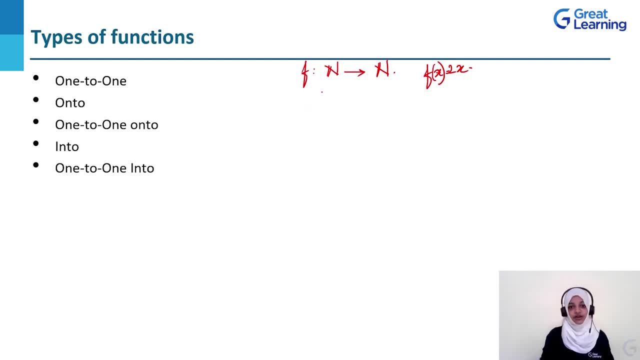 equate to 2x. Let us check if this particular function is injective in nature. Let's consider two values, such that we have x1 and x2,, both of them belonging to the domain of natural numbers. Let us assume that F is equal. 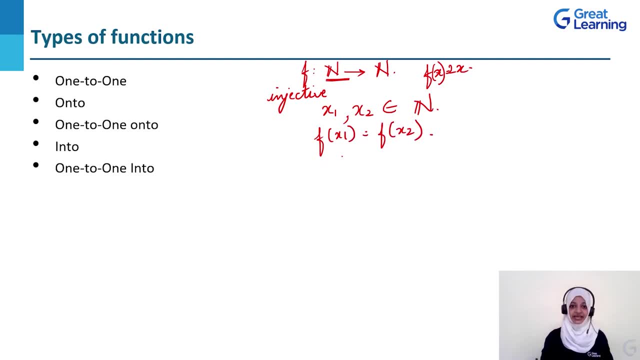 to F. This implies that 2x1 is equal to 2x2.. Canceling out 2 from both sides, we are able to obtain the result that x1 is equal to x2.. Therefore, for the same image in the co-domain. 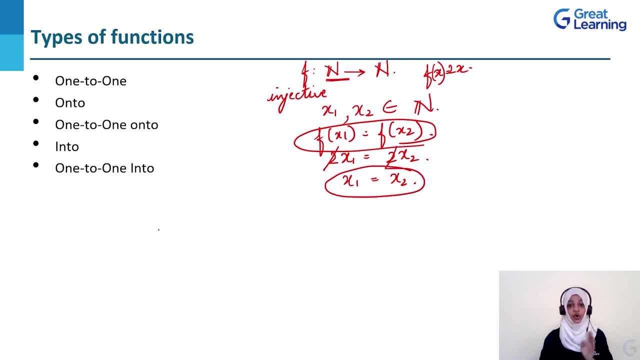 we have a prior input within the domain, which is also the same as each other. This means that the function is injective in nature or is one-to-one in nature. Next, let's look at whether this particular function is subjective or into Or onto, and. 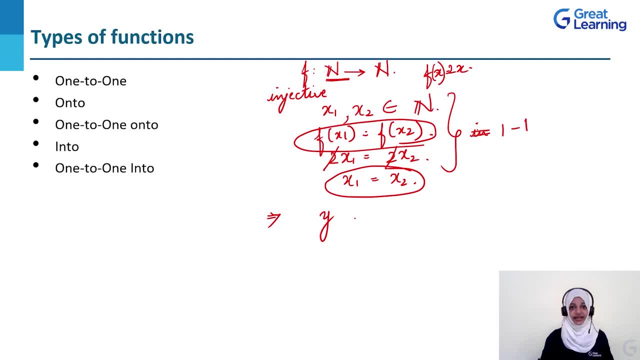 into. Let's consider a value y such that value y belongs to the co-domain of natural numbers, as given here. This implies that if we take F equal to y, then y is equal to 2x. It further goes to imply that x is equal to. 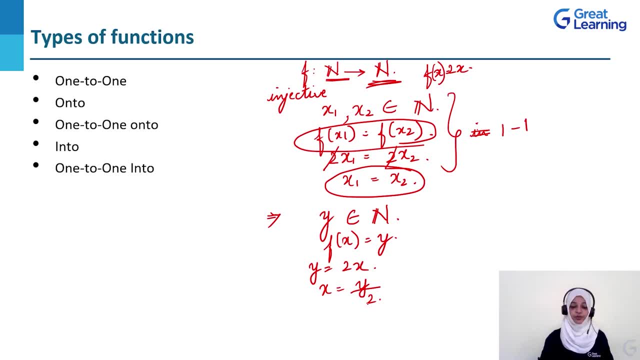 y upon 2.. y upon 2 could possibly give a decimal. This means that it's possible that x would be equal to a decimal value, But decimal values are not a part of the domain, which is a set of natural numbers. This means that there would be 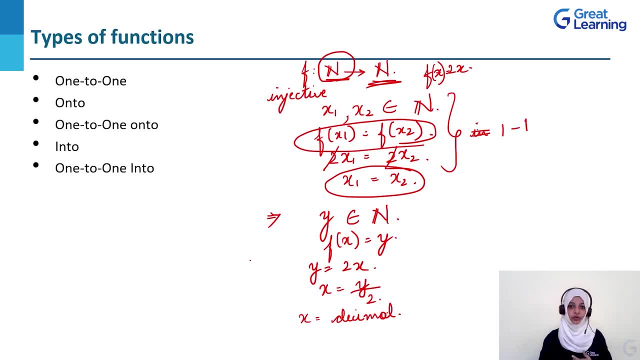 some natural numbers which, when divided by 2, will give you a decimal value which is not there as a part of your domain. This means that there would be some elements which are a part of the co-domain, for example, 13,, 11,, 15,. 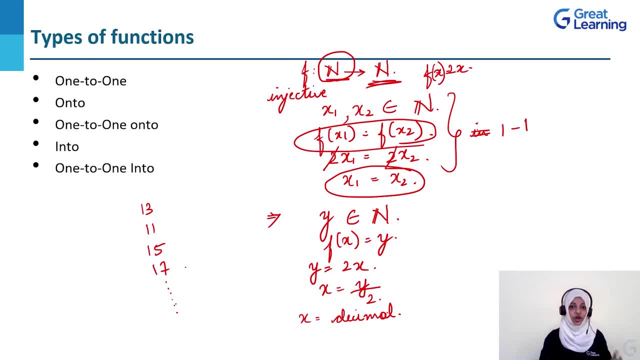 17, and so on and so forth, which will not have a pre-image in the domain. As per the definition of into functions, we already know that if even one element in the co-domain does not have a corresponding pre-image in the domain, then the function is said to be. 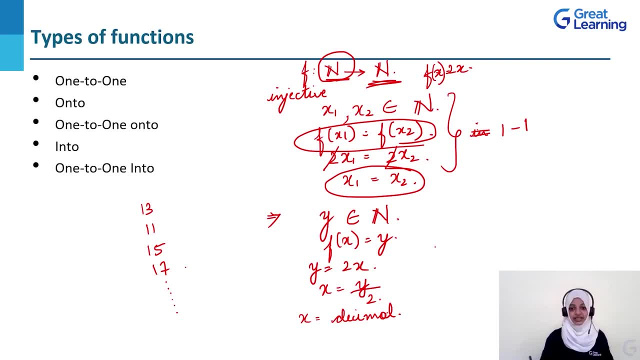 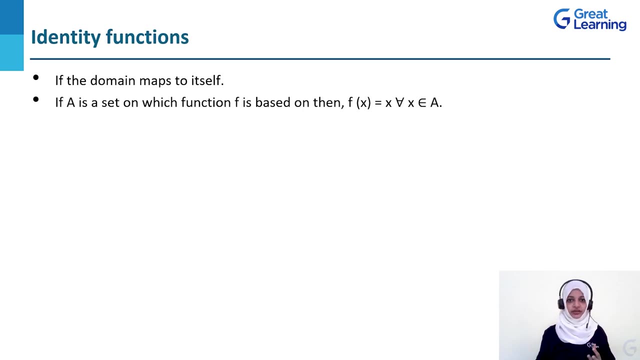 into function. As it turns out, we can say that this particular function is an into function. So this is an example of one-to-one into functions. Next, let's look at identity functions. We already know that identities are values that either. 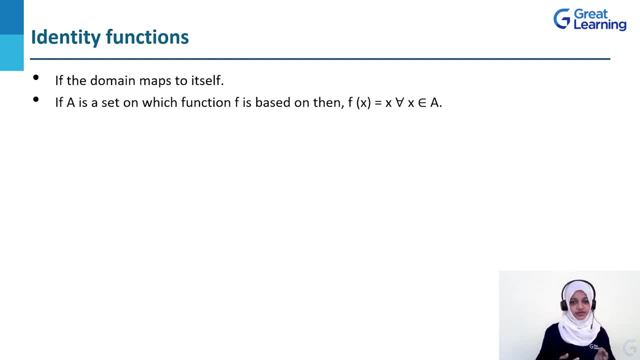 preserve themselves or preserve others right. This is what these functions also do. Now, identity functions are actually functions in which the domain maps exactly to itself. This means that the domain is actually equal to the range. Please remember that the range means the actual values of. 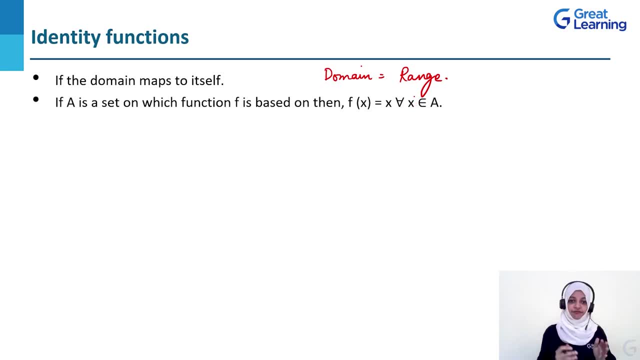 outputs, not the possible. So this means that for every value in the domain we would always get the exact same value in the range. So if we take x as a possible input in the domain, we will get x as the output. 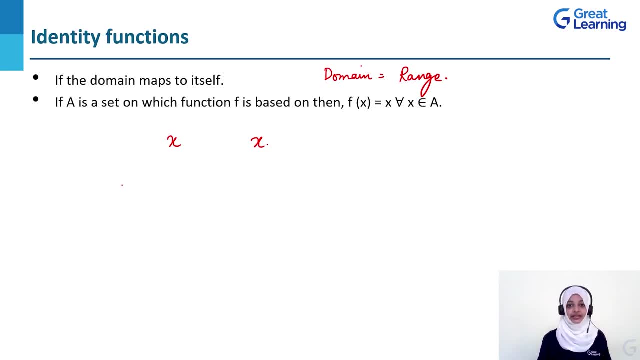 in the range too. These are known as identity functions. As a result, identity functions are defined as functions that are based on any set, such that for any f of x, we get back the value of x as the result, And this happens for. 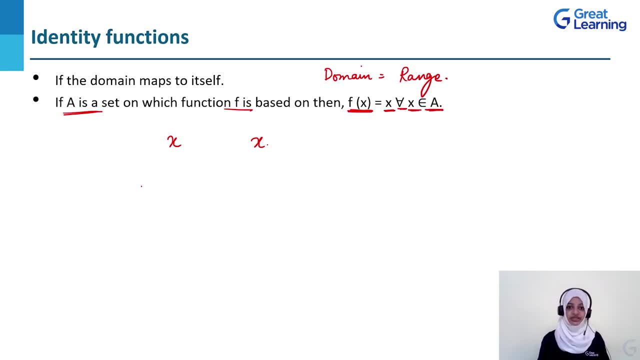 each and every value of x that belongs to the set. Let us understand this with an example. If we have the function f of x is equal to x. if we take the x value as 1, we get y value also as 1.. If we 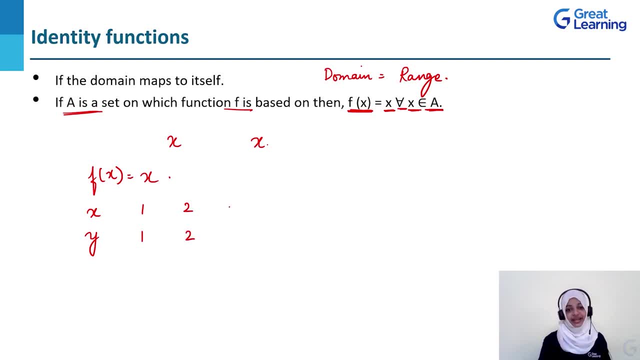 take x value as 2, y would be 2.. If we take x value as minus 116, we will get y value also as minus 116.. This means that for each and every value of x, the value of f of x is equal. 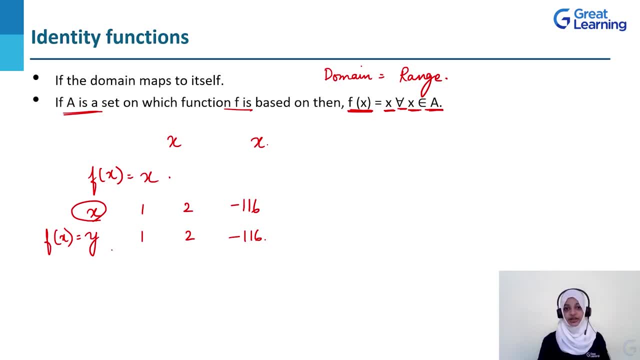 to itself. This is what an identity function does. When we try to plot the identity function on a graph, the identity function's graph would look something like this, where each and every value of x is actually equal to the value of y. So much so. 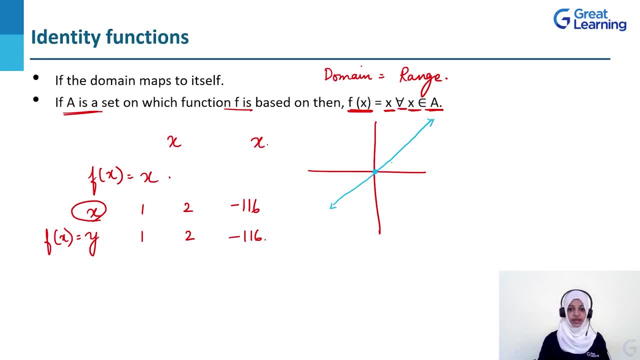 that this particular graph will pass through the origin. All of these points would be points like, and so on, and so forth, And these points would be similar on a negative scale though. So and so on and so forth. This is an 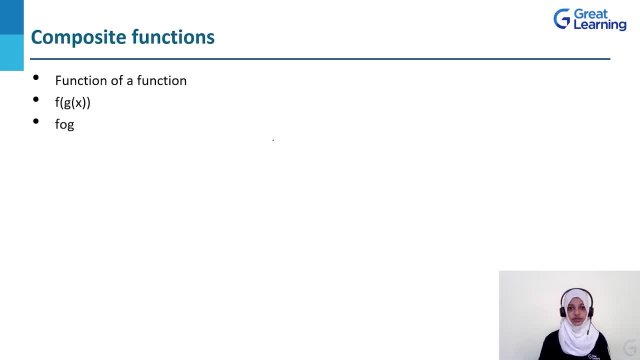 identity function. Next, let's look at composite functions. Composite functions or, as they're also called, composition of functions. Now, what are these? These are actually functions that behave as values for functions, Or functions placed inside functions, so that 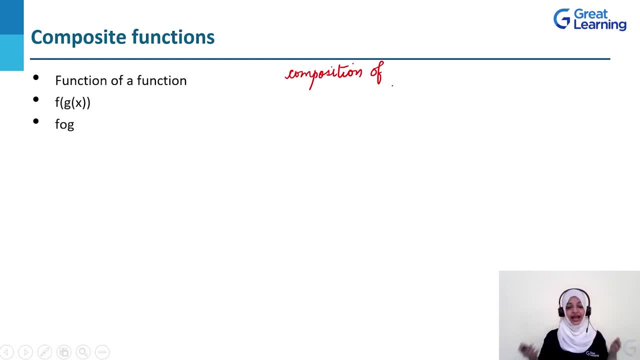 more complex calculations can be performed and more complex values can be obtained as outputs by giving inputs. Composition of functions has various applications seen in real life. In most cases, we've got multiple small functions such that all of these functions generate outputs of their own. 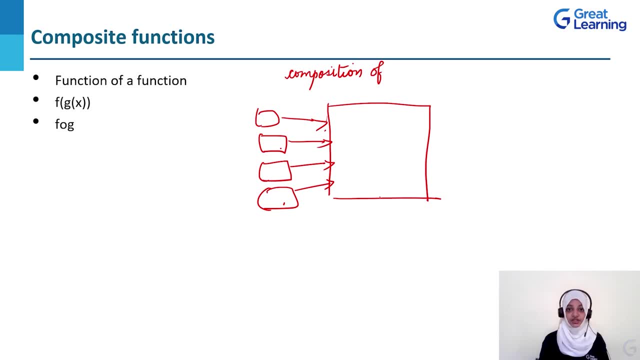 These outputs are then considered as inputs by a larger function, and then complex calculations are performed on them in order to provide a single final output. This implementation actually has its base on this particular function component, So let's see how it actually works. 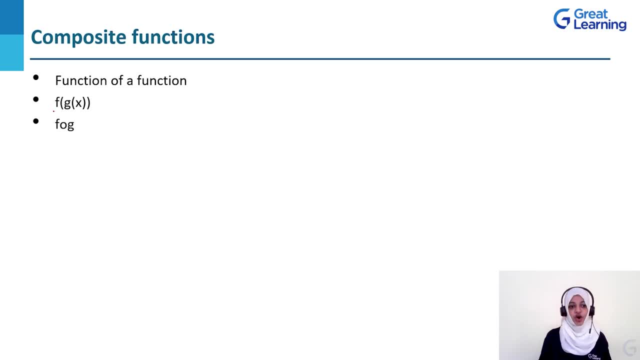 If we've got a function which is a composition of function, it's often denoted as outer function with inner function, Or it's also called FOG. Please don't read it as fog. It's just denoting that we've got. 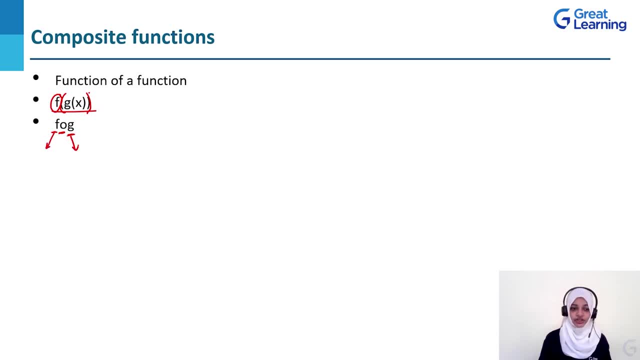 an outer function and we've got the inner function and they're both related to each other in a composition which is denoted by the O here. Now we can have any number or any complexity of compositions. Suppose we have three functions, namely 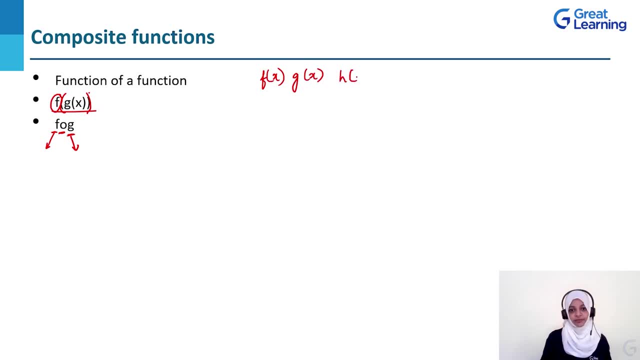 f, g and h. We can have simple function compositions such as f encompassed by g, which is also denoted as gof, or we could have g of h, of x, which is denoted by goh, or we could have a bit. 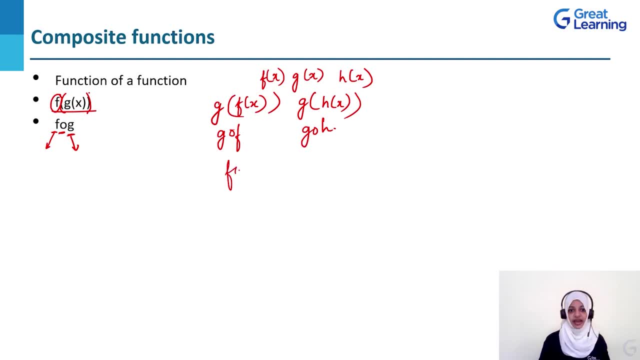 more complex compositions such as fogoh, which is h of x, encompassed by g, encompassed by f, and then we can increase the level of complexity as per our requirements. So we could also have something like this: og og. 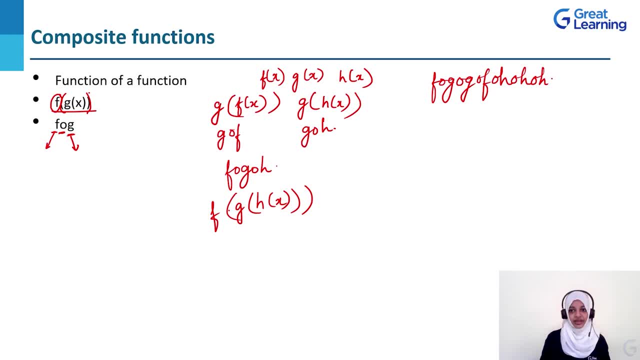 of oh, oh, oh, of of. How do we resolve this? It's simple: Start with the last, which is the innermost function. Outside that, we would have the one beside it, Outside that, the one beside. 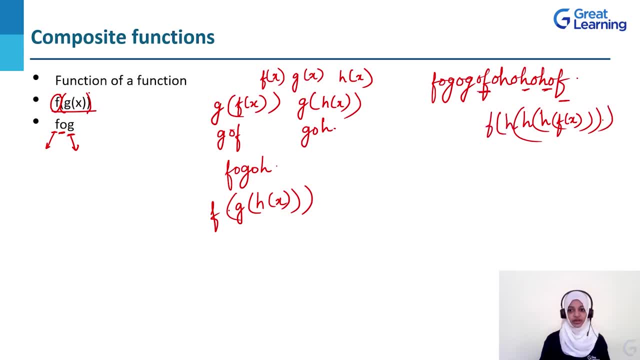 the one beside, and so on and so forth till we don't complete. So this is what the composition looks like in the end: f of g, of f, of h, of h, of f of x. So the value of x will actually first be computed. 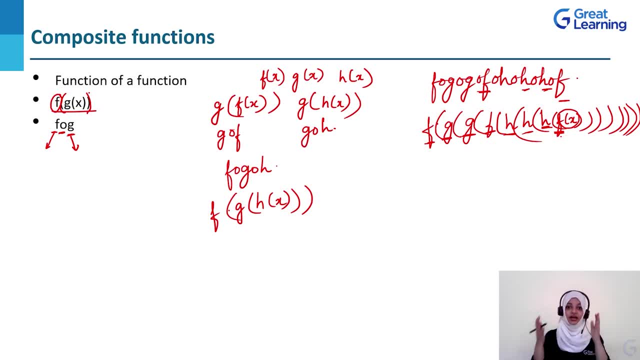 by the innermost f of x, and then the output of that innermost f of x will act as the input for the h of x, the output of which will act as the input for h of x, the output of which will act as: 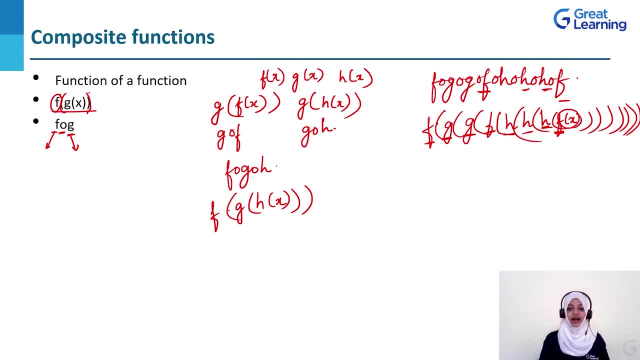 the input for h of x and so on and so forth till the outermost f is not resolved. Let us also explain this with an example. Let's say we've got a function- f of x is equal to 7 x, and we've got another. 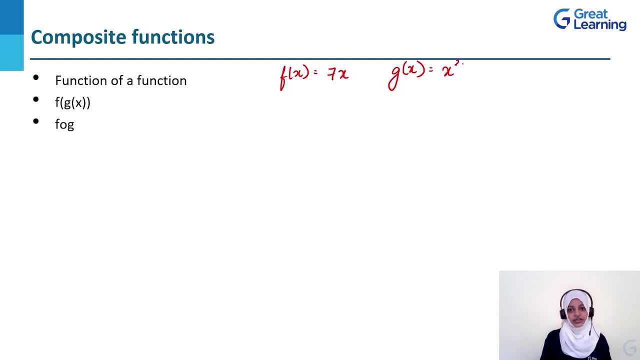 function g of x, such that is equal to x square plus 1.. If we take a composition of function g of f and another composition of function f of g, let us see how they resolve. Consider g of f, which actually means g. 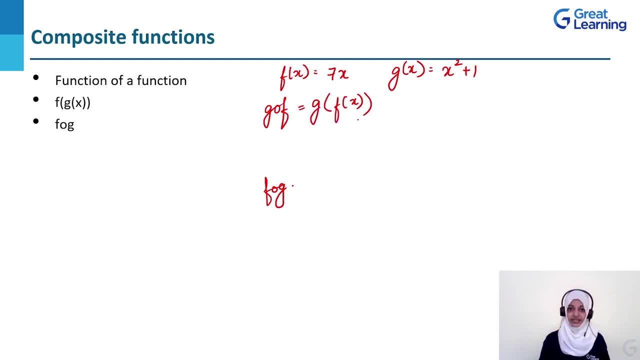 of f of x. This means that we first need to resolve the value within which is f of x, and the output of f of x would then act as the input for g function. Similarly, taking f of g would be equal to f of. 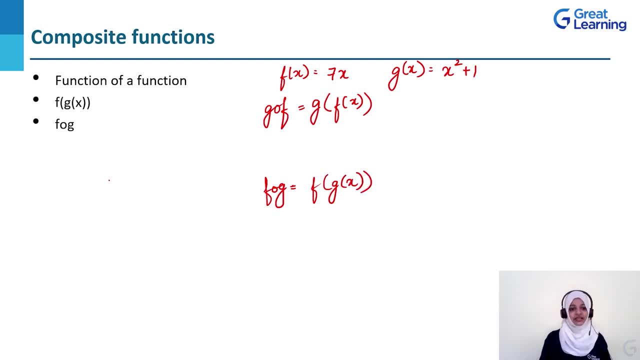 g of x. Let's consider an x value which is equal to say 4.. If we consider g of f of x, we're actually going to consider this as g of f of 4. This means that we'll first take the f function. 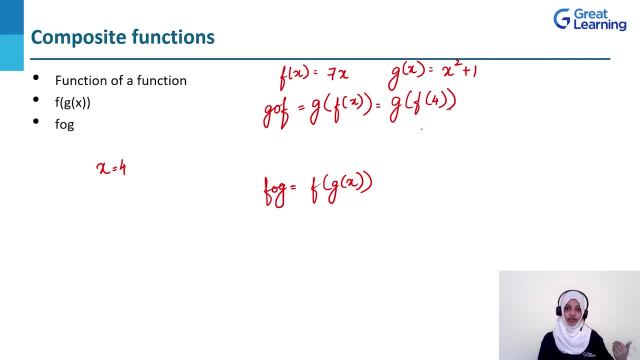 substitute the value of 4 into it, get an output, and whatever the output would then act as the input for the g function. Let's start. Let us consider 7 x here. This means that we've got 7 x, which acts as: 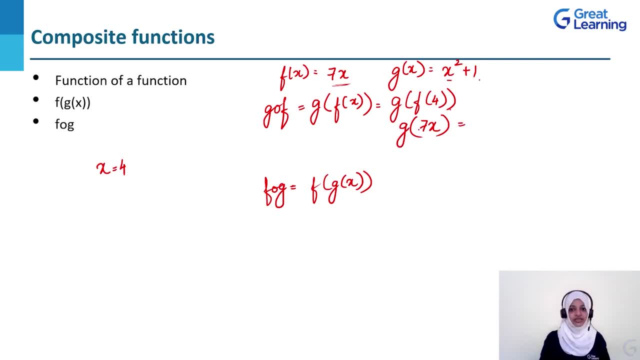 the input for g. This converts this particular function into 7 x the whole, square plus 1.. This means that we're essentially getting 7 x 4, the whole square plus 1. This would be equal to 28, the whole square plus 1.. 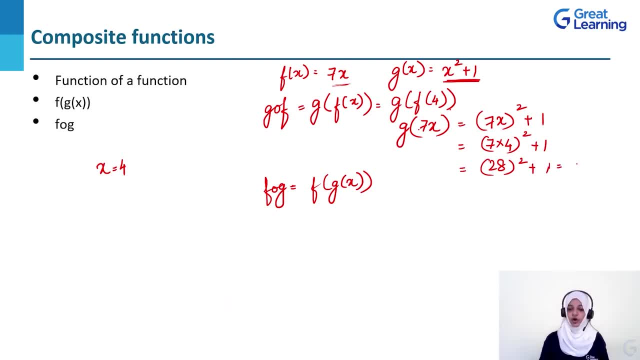 After calculation, we can see that we've got the value here as 784 plus 1, which is 785.. Next let's try to calculate f of g also. As we've already seen, f of g can be simplified as f of g. 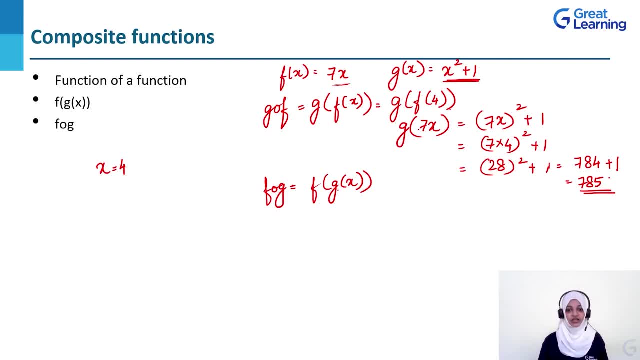 of x. As a result, let us first consider g of x, which is x square plus 1.. This is going to act as the input for f. This means that our function essentially transforms into 7, into x square plus 1.. 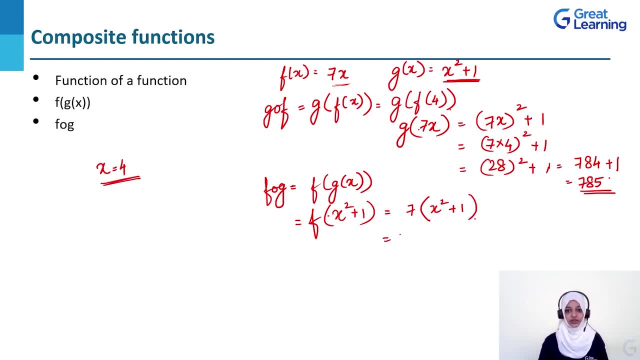 Considering that our value of x is 4, this can be written as 7 into 4 square plus 1, which is equal to 7 into 16 plus 1,, which is 7 into 17.. Now, 7 into. 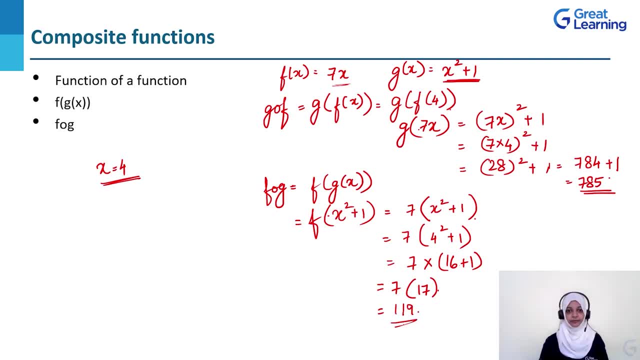 17 is actually 119.. Thus we've seen that we get a value for gof and fog. An important point to note here is that gof is not equal to f of g. This means that the composition of function is non-commutative in nature. 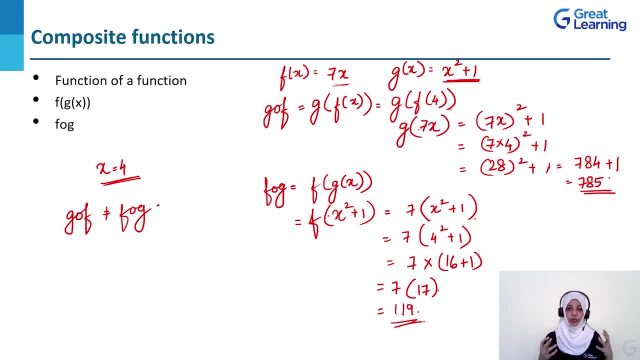 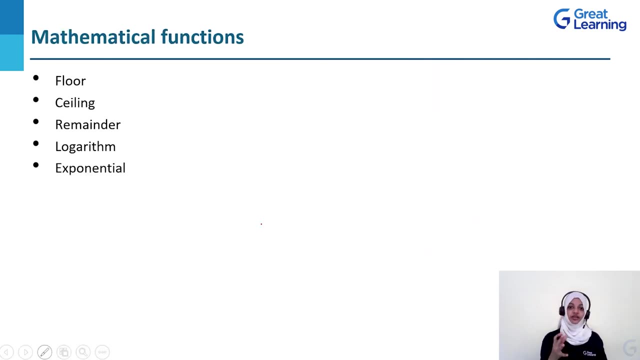 There might be some cases and some function combinations wherein gof would be equal to f of g, but this is not the norm. So please note that this particular composition of function is almost never commutative in nature. Lastly, let us look at the most. 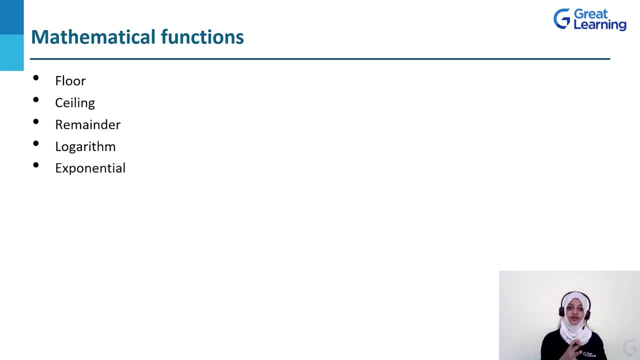 commonly utilized mathematical functions. Now, these functions are not the only mathematical functions, but these are those functions that are present in maths and are also present in most of the programming languages in one way or another. Most programming languages, such as C, C++ and Java, 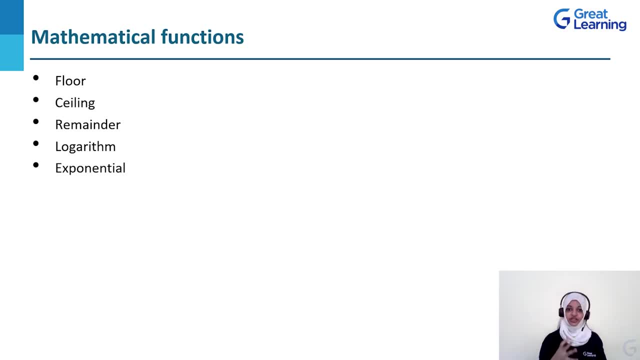 either have header files or have packages that actually contain these mathematical functions. They help us with various mathematical calculations that might be a part of any kind of computation. As a result, these are important to note. The first is the floor function. A floor function is very simple. 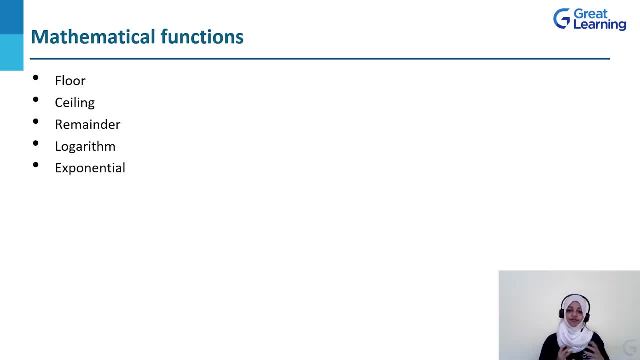 Let's look at these functions in a bit more detail. First, we've got the floor function. The floor function is defined as the function that actually allows us to get the greatest integer, which is less than the value currently under observation. On the other hand, the ceiling- 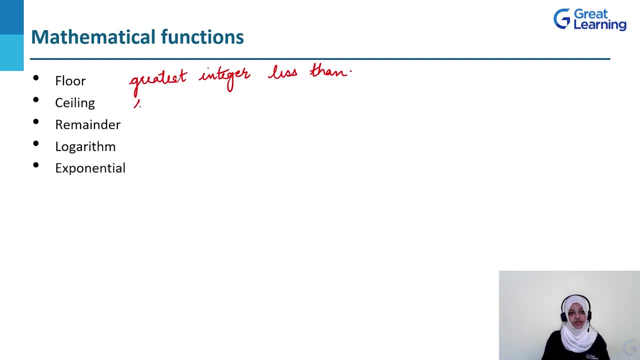 function is the function that provides us with the smallest integer, which is greater than the actual value under consideration. Let's look at an example of these two to actually understand why they are so confusingly stated. Now let's take the first example, which is seal. 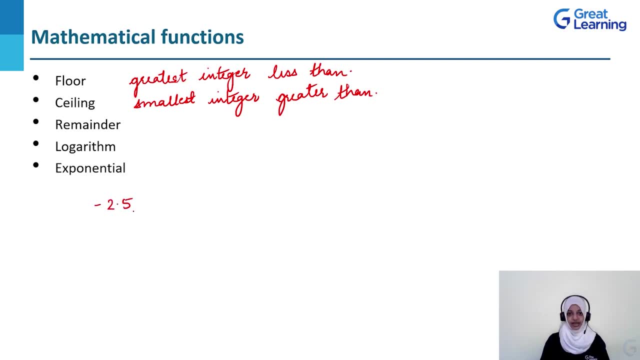 of minus 2.5.. Now the ceiling, or the seal as it's called in various programming languages, is actually denoted by this type of an open-ended bracket. So the first thing is actually analyzing what is written there. We need to select the smallest. 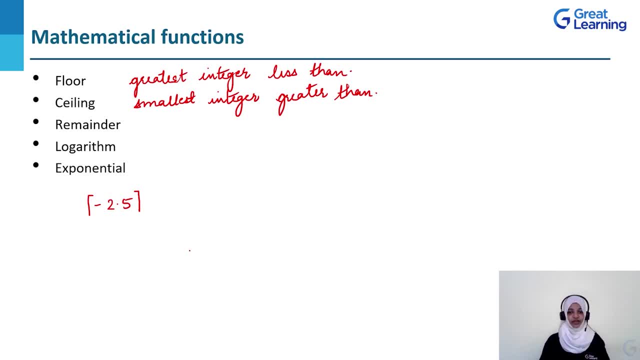 integer which is greater than the value that we currently have. What is the value here? The value is minus 2.5.. The integers closest to minus 2.5 on any number line are actually minus 3 and minus 2.. Which of these is? 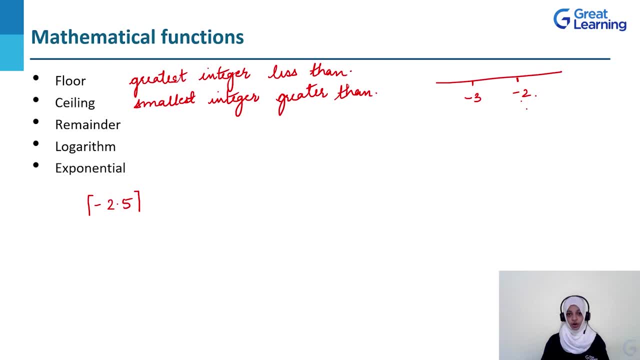 greater than minus 2.5?? Obviously, the value is minus 2.. So the seal value of minus 2.5 is minus 2, since it is the smallest integer which can be greater than minus 2.5.. Other integers can also be greater. 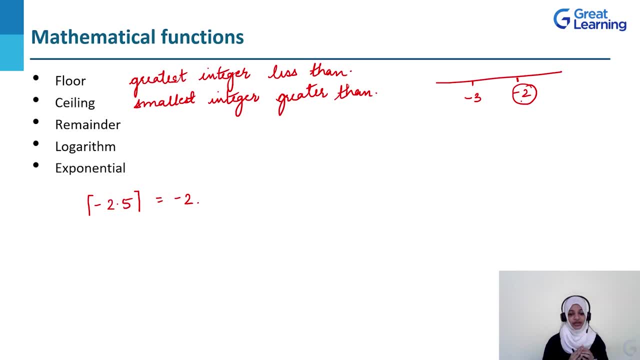 than minus 2.5, but minus 2 is the closest to it and the smallest value out of all of those. Similarly, let us consider another value, Say for example 3.25.. On the number line, what is the value? 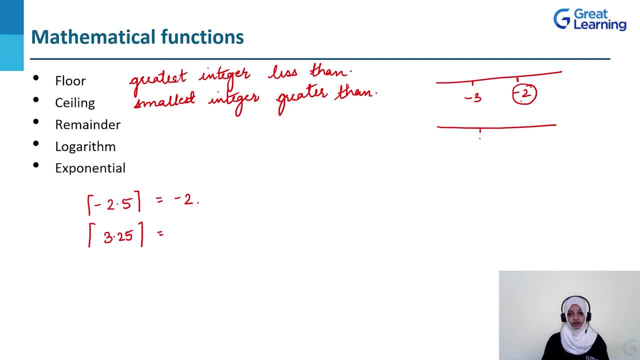 which is closest to 3.25?? We've got the value plus 3 and the value plus 4.. Which of these is greater than the value under consideration? That would be 4.. As a result, the seal here of 3.25. 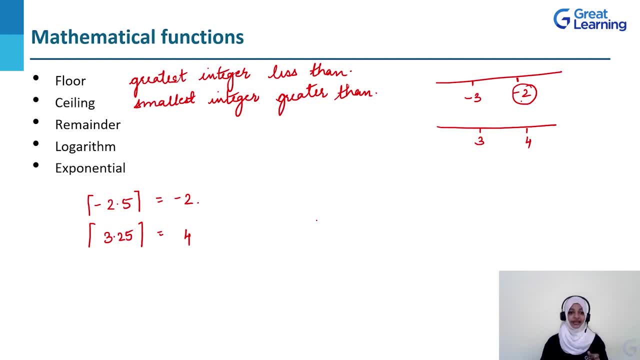 would be 4.. Similarly, let us look at the floors or the floor function values of these particular values. Floor function values are denoted by these open-ended brackets. If we are considering minus 2.5 again, then we are supposed to take the integer. 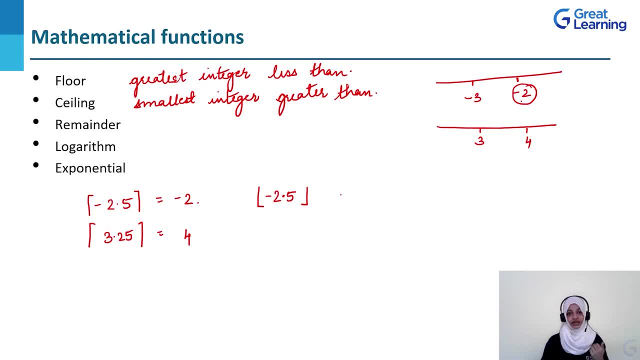 which is less than the value under consideration, but it should be the greatest from all of these. So the value which is closest to minus 2.5 are again minus 3 and minus 2.. Which of these is smaller than minus 2.5?? The answer. 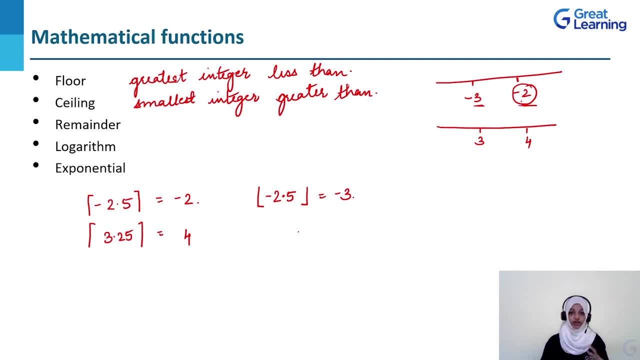 is minus 3.. Thus the floor here or the floor function value will be minus 3.. Similarly, if we consider 3.25,, then the floor function will provide us with a value of 3.. This is how we can differentiate. 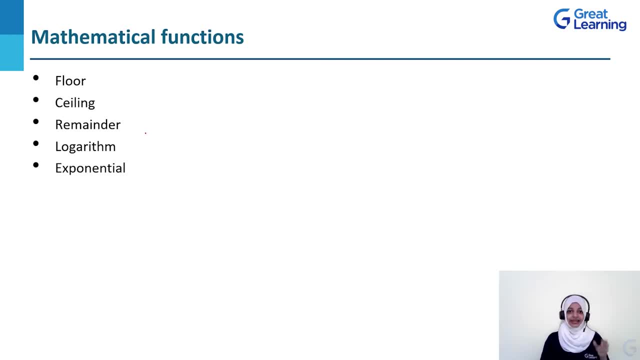 between the floor and the ceiling functions. Next, let's look at the remainder function. In most of the programming languages or pseudocodes, or even algorithms, for that matter, we often look at the remainder function. The remainder function is very helpful in understanding. 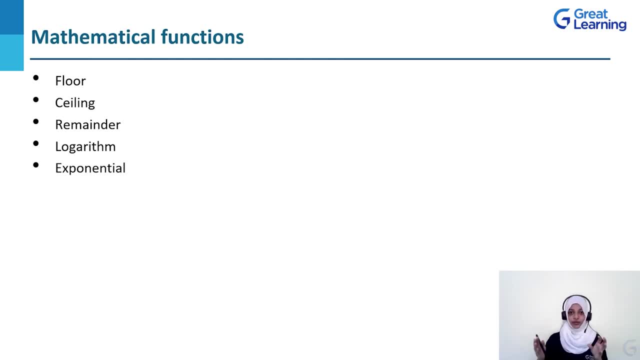 whether or not a value is divisible by another value. If one value is divisible by another value, the remainder function will provide us with an answer of 0. Otherwise, other values will be taken up as answers based upon how much the remainder is. 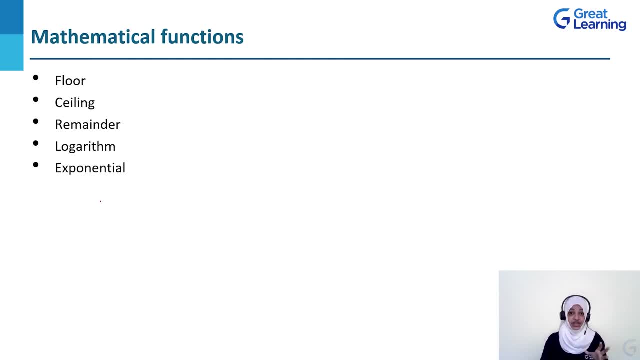 The remainder function is often denoted generically as the mod function. So if we have a function written as 7 mod 4, it actually means that we are dividing 7 by 4 and we are trying to find out what the remainder. 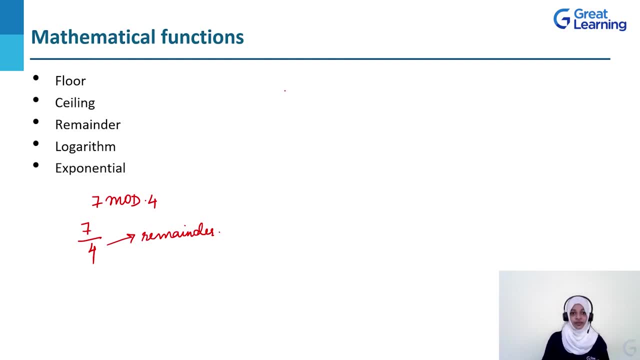 of this particular calculation is going to be Carrying out. this division will actually give us a quotient of 1 and a remainder of 3.. Similarly, we can have other values also taken up as a part of this particular function. Say, for example: we've got: 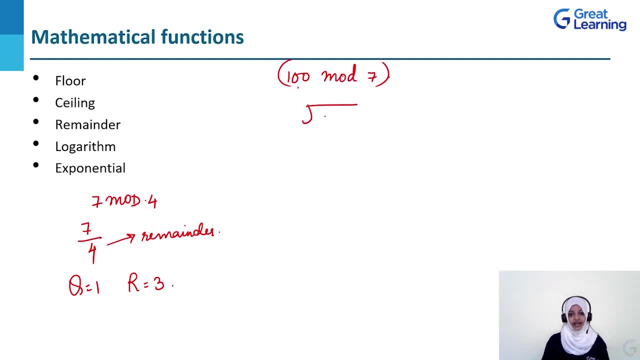 100 mod 7.. Let's divide 100 mod 7 and see what the quotient and the remainder are. So, as we can see here, we've got the division all done. We've got a quotient of 14 and a remainder. 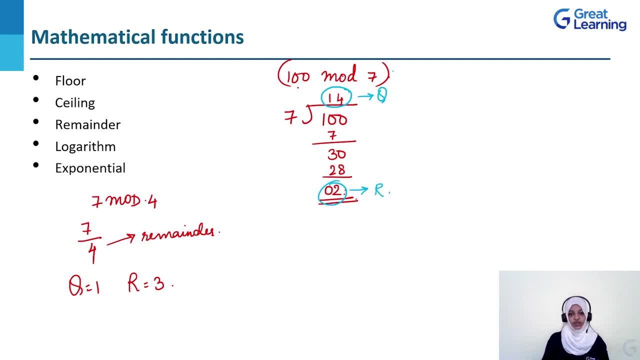 of 2.. This means that this particular operation, 100 mod 7, will provide us with an answer of 2.. This is how the remainder function works. The logarithm function, on the other hand, actually allows us to find out the value of any 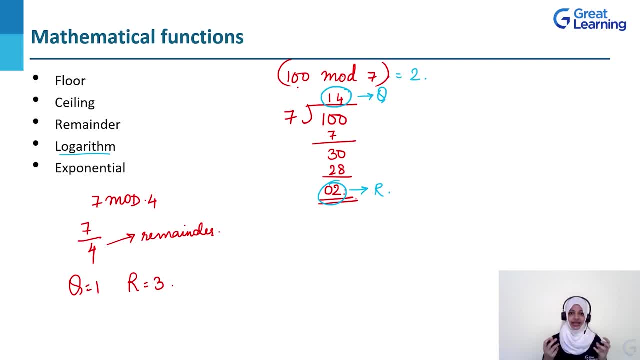 two values given to it. What it does is it takes the actual value of which the logarithm has to be computed and it also takes the base to which this particular logarithm has been computed. So we can have base 10,. we can have base 2,. 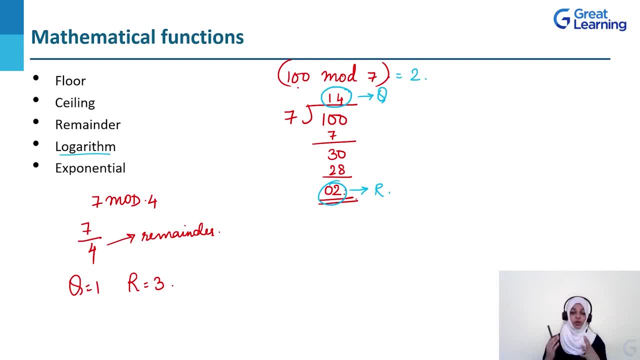 we can have base 5,, we can have base 8, and, depending upon what base has been chosen, we'll get different answers for the values that we're trying to compute the logarithm for. Lastly, we've got the exponential function that actually 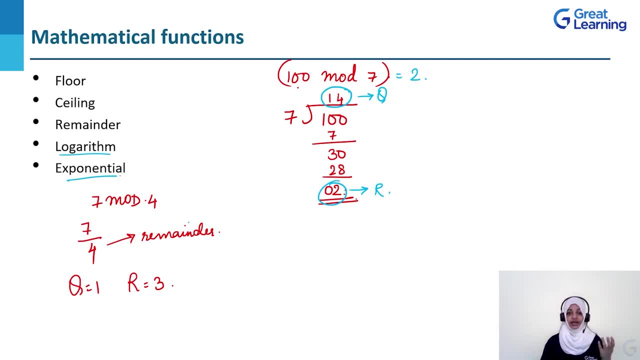 helps us find the various powers of any value. Again, exponential functions are extremely helpful while we're trying to find out the values of any number raised to another number. An application of exponential is when you're trying to find out the powers of 2. 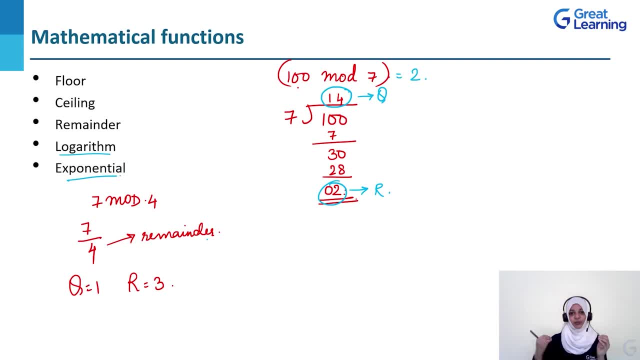 while trying to convert from hexadecimal values into binary values, or binary values into decimal values or octa values into decimal values, etc. So number system conversions is where exponents actually have a practical application. Thus we've seen some of the most. 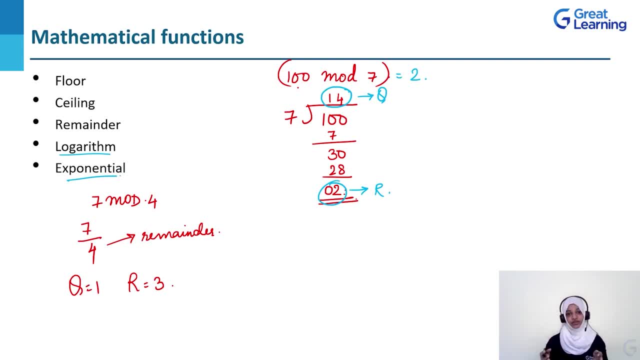 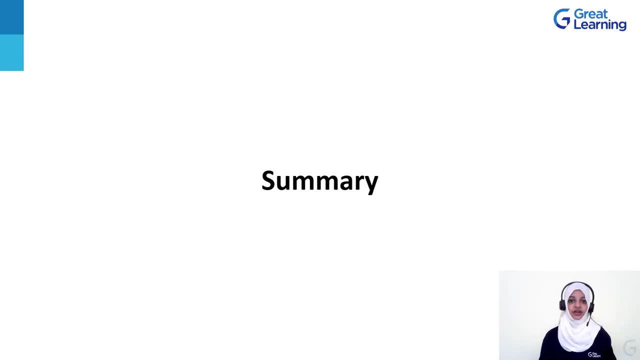 commonly used mathematical functions that often get translated into some of the other kind of programming language in one way or the other. So that ends our very first course of basics of discrete mathematics. Let us have a quick look at what we've learned till now First, 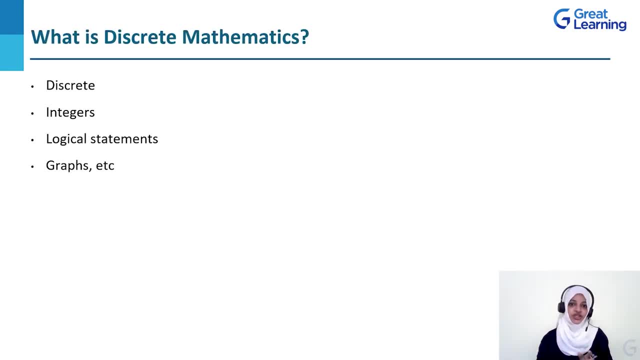 we looked at an introduction to discrete mathematics. We understood that discrete mathematics is actually related to non-continuous numbers, such as integers, logical statements or graphs for that matter. We were able to understand what the basic applications or the most commonly used real-life applications of discrete 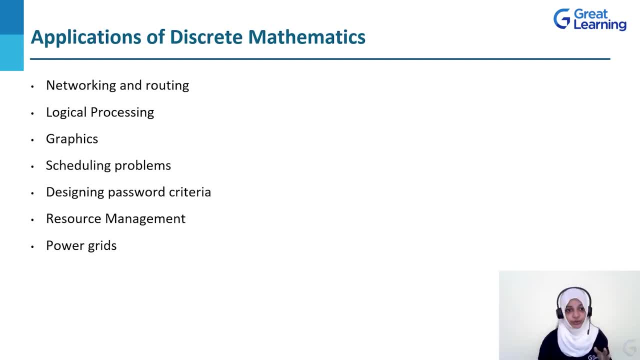 mathematics were, For example, in logical processing. when we've got any kind of computing device, when we've got graphics in order to actually perform the transformations, we can apply various linear algebra properties there. If we require resource management, then we've got counting problems. So all. 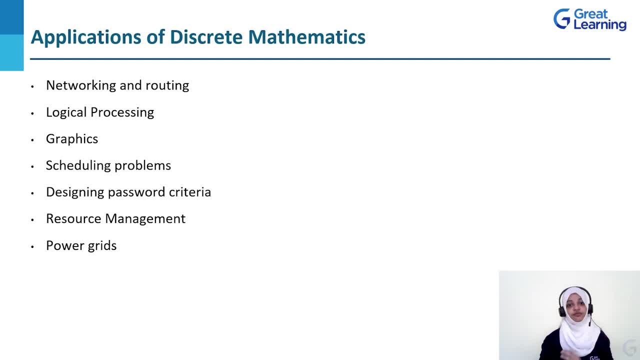 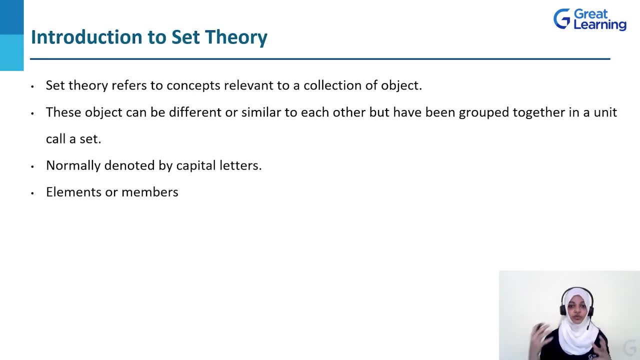 of these problems could actually be resolved with the help of discrete mathematics. Next we looked into set theory. We saw exactly what set theory was. We understood that we've got a collection of objects and they're grouped together to form one cohesive unit. 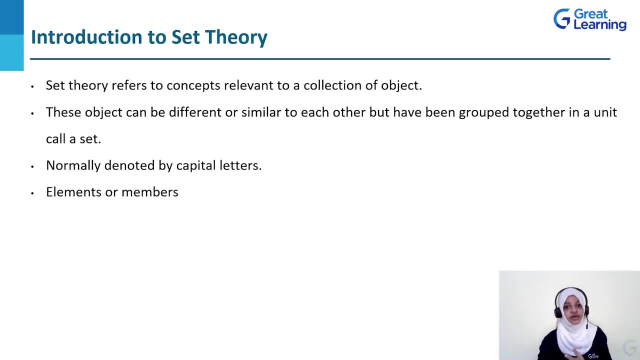 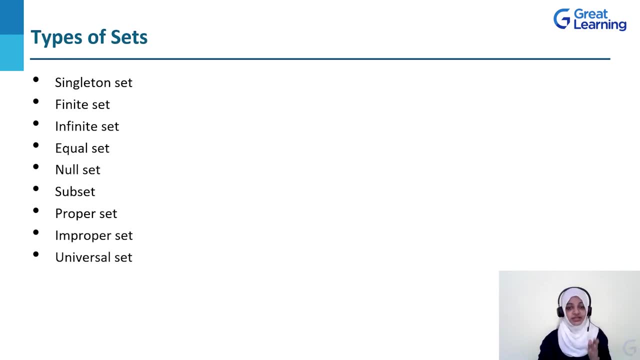 These objects would be known as elements or members, and they would normally be denoted by capital letters. Next, we understood what are the various types of sets that we have while we're actually using set in real life, So there could be sets which do not. 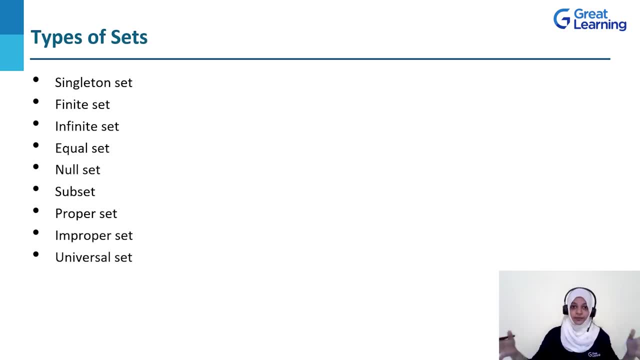 have any elements. There could be sets that are actually considering all the elements that we're currently working with, For example, universal set. We also understood that each and every set that we're using will have a power set, which is basically the parent set of each and every set. 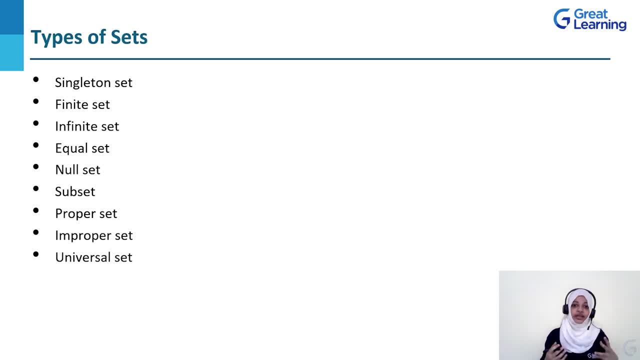 whether we're using it or not, Right? We also saw that there are different kinds of sets, like infinite set or finite set. We also saw that, based upon the concept of subsets, we have two other sets, such as proper and improper set, where we often 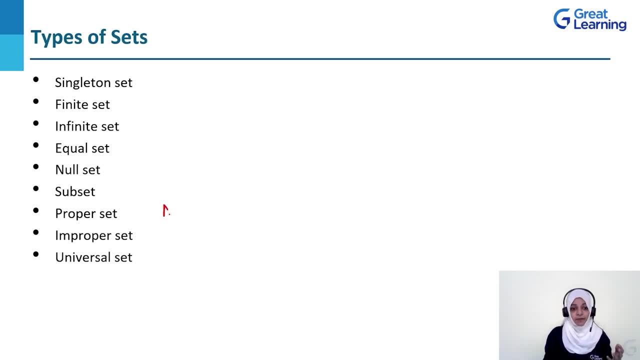 try to say, or we try to understand, whether the subset can be equal to the parent set or whether the subset should not be equal to the parent set. So if the subset was not equal, or never equal, to the parent set, we would call it a proper. 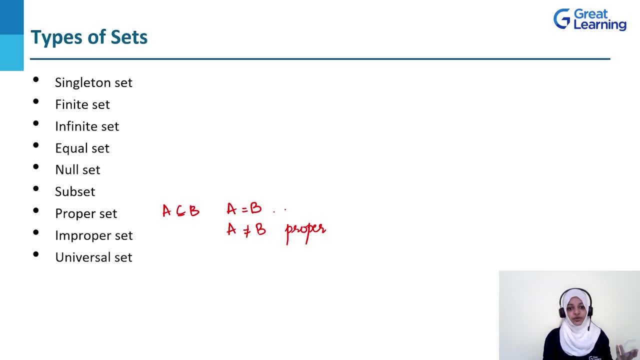 set, And if it was sometimes equal to the parent, we would call it an improper set. So in this manner, we saw various types of set that we often used. Next, we also saw the various operations that we could perform on set. 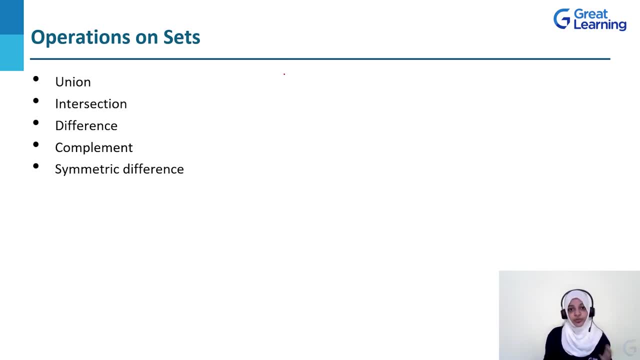 We also saw how these particular operations could be shown or could be depicted with the use of Venn diagrams, Right. So this actually helped us in visualizing the operation that is currently ongoing and in understanding exactly what is going on. So it was no longer. 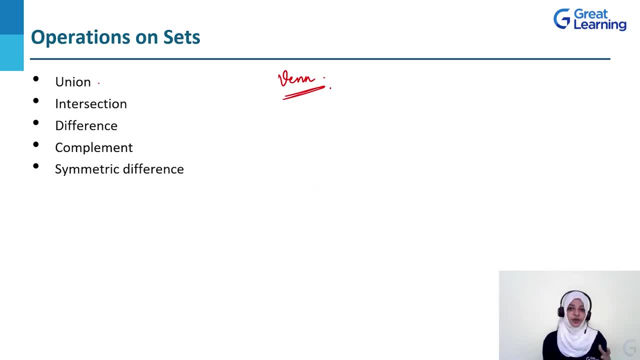 abstract. It now became concrete in nature. So first we've got union, which actually helps us find out all of the elements or group together all of the elements in two given set. Next we've got intersection, which actually helps us find out the commonalities. 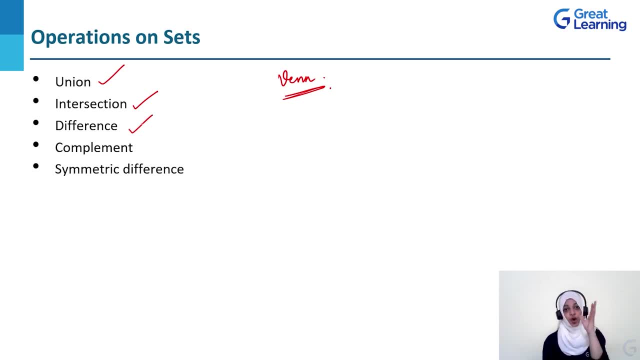 between any two sets. We've got difference that helps us include all the elements in one set while excluding all of the elements of the other set. Or another way to frame this would be include all the elements in one set and exclude all of the elements of the other set. 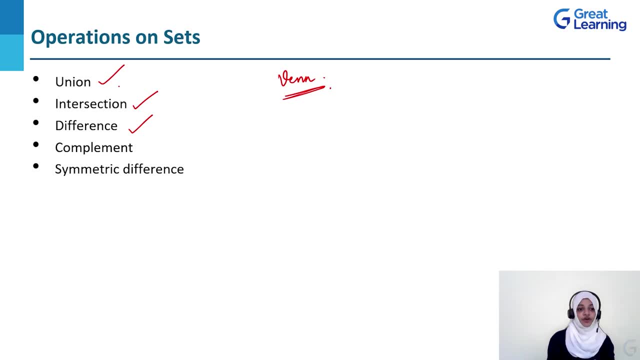 Right. So here we've got union, intersection and difference. Please note: union and intersection are commutative in nature, whereas difference is non-commutative in nature. Next, we saw the complement, which is often denoted by the. 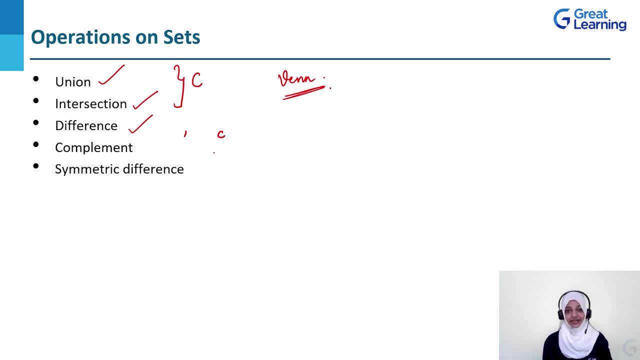 apostrophe or a superscript of C Right. This actually means negation. So if we have a set, say, for example A, then complement of A would be all the elements that are not a part of A. Lastly, we have the symmetric difference. 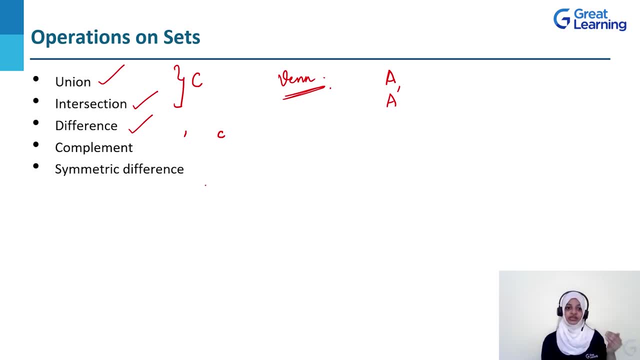 which, as we saw, was a combination of union, intersection and difference, such that A and B, if they are two sets under symmetric difference, we would have symmetric difference defined as A union B minus A intersection B. Also, set difference was denoted by three different. 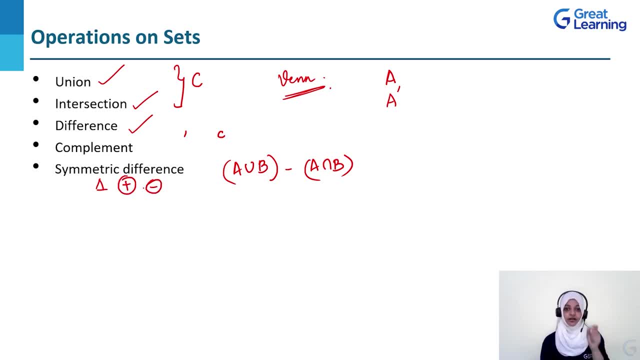 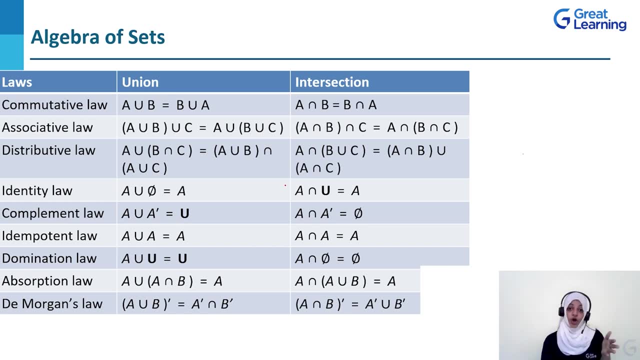 denotations, all of which are right, which is delta. The other one was plus inside a circle and minus inside a circle. Next, we looked into the various laws that were present as a part of the algebra of set, and we also saw how we could. 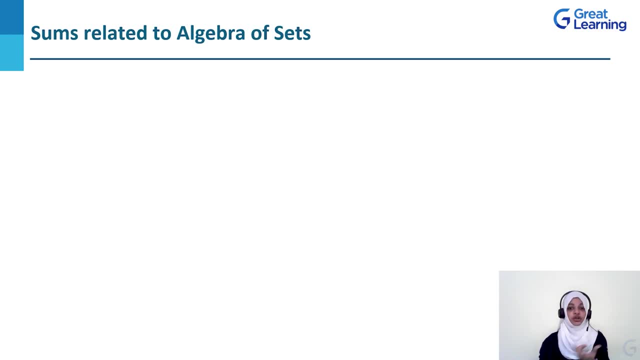 resolve our problems, word problems or sums- on the basis of these laws. The next topic that we looked into were the relations. We understood what were the various applications of relations, namely for functional analysis. We understood that a relation is actually the connectivity that exists between: 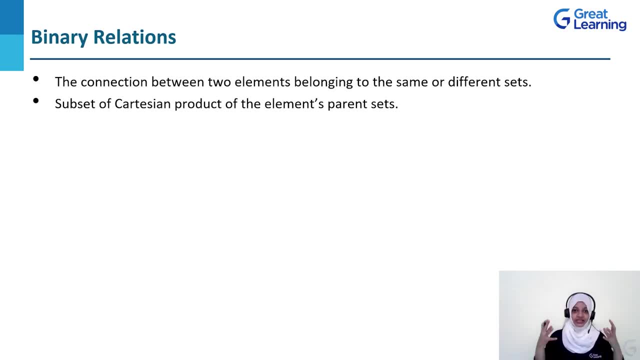 any two sets and that the final answer that we get as a relation is going to be in the form of a set of ordered pairs that are actually going to be a subset of the Cartesian product, of whichever two sets are interacting with each other. Next, we saw the various types of 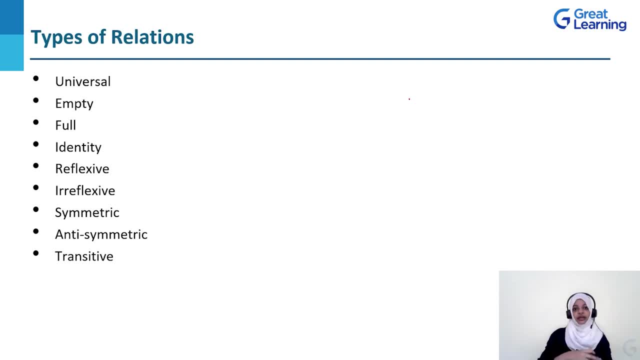 relations that we would have, whether it is the universal relation, the set containing all of the relations, whether it is an empty relation, wherein there are no ordered pairs that are a part of the relation, or it is a full relation or an identity relation, a reflexive. 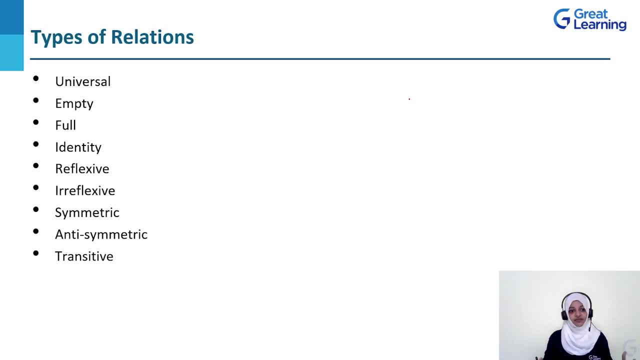 symmetric, irreflexive, anti-symmetric or transitive relation. We've also seen the closure properties, meaning how are we actually supposed to make a non-reflexive or non-symmetric or non-transitive relation into a reflexive, symmetric or a transitive relation? 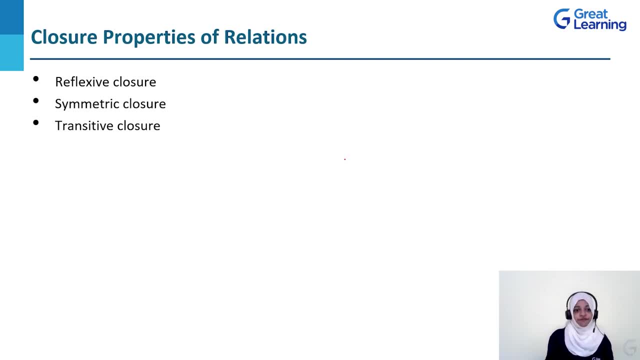 So doing that, as we've seen, is very simple. If a particular relation was not reflexive, we added the symmetric ordered pair, such that it becomes symmetric. If a particular relation was not symmetric, then for every ordered pair we added another ordered pair. 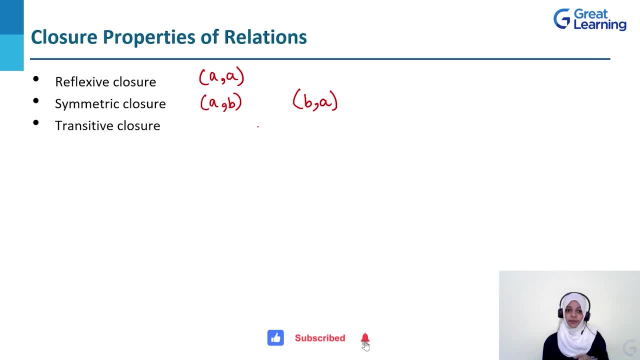 till the relation did not become symmetric. Lastly, for every relation that was not transitive, we converted it into transitive. The method of doing so was very simple: For each and every ordered pair that had, if it had, a related, we would. 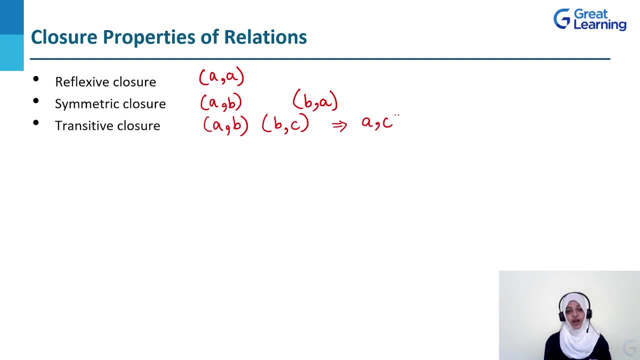 actually be able to attach a ordered pair, which would help us make the relation into a transitive relation. So this is how we were able to actually convert non-reflexive, non-symmetric or non-transitive relations into reflexive, symmetric or transitive relations. 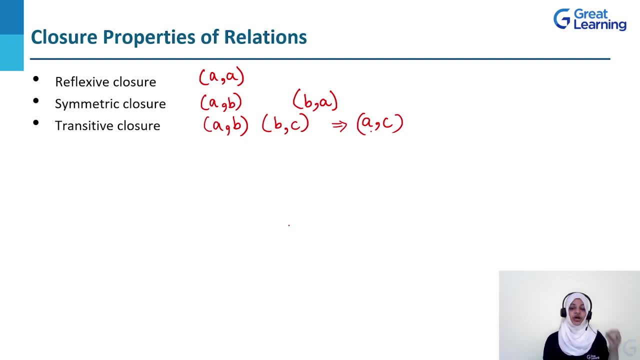 We also saw that if any relation would be converted into reflexive, symmetric and transitive, we would also have something known as equivalence closure Right. Next, we had a look at what equivalence relation actually is. So in a relation, if a relation 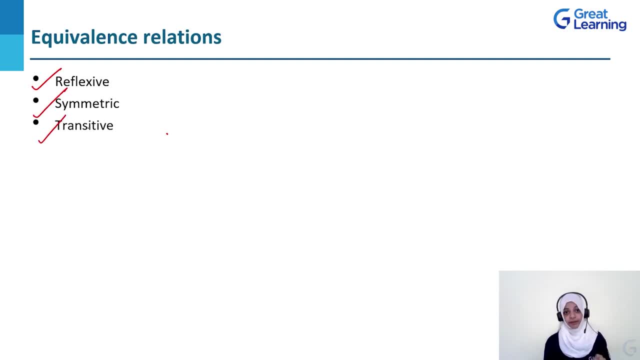 is going to be reflexive, symmetric and transitive at the same time, then that particular relationship is known as an equivalence relation, If a relation is either not reflexive or not symmetric or not transitive. that means that in a relation, if even one of these 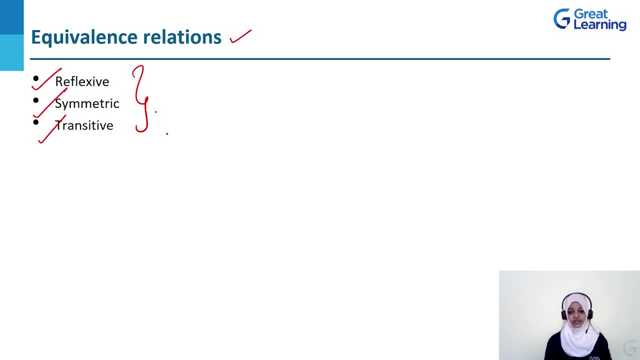 components is missing, then it will no longer be known as an equivalence relation. Lastly, we saw that we've got a partial ordering relation, which actually states that the relation must be reflexive, anti-symmetric and transitive. The difference between symmetric and anti-symmetric was very 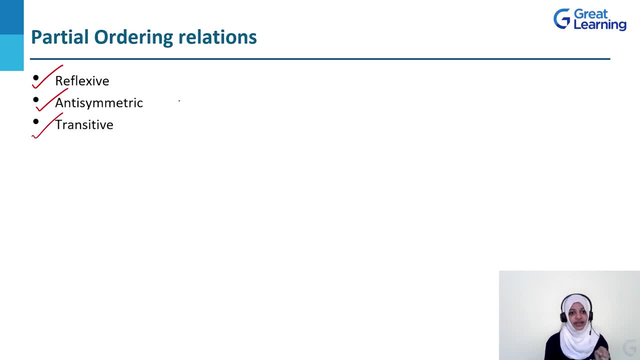 slight but very important. So, as for anti-symmetric, if we had an order pair, then we could have two possible options. Either we have a, such that b is equal to a, or if b can't be equal to a, then we have. 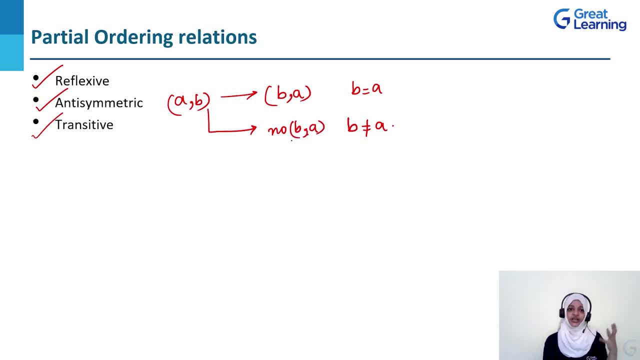 no ordered pair at all. This is what anti-symmetric was. So if a particular relation has even one of these components missing, this means that if it is not reflexive, or maybe not anti-symmetric or not transitive, it will no longer be a partial. 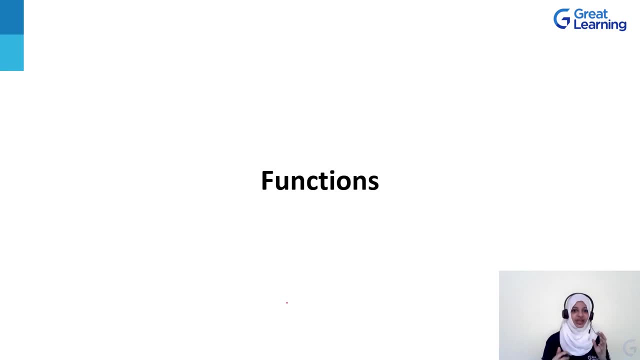 ordered relation. Lastly, we looked at functions. We discussed why we were using functions. To some extent we understood that large calculations had to be carried out by functions and we've already seen various functions in our lower classes, So we understood that. 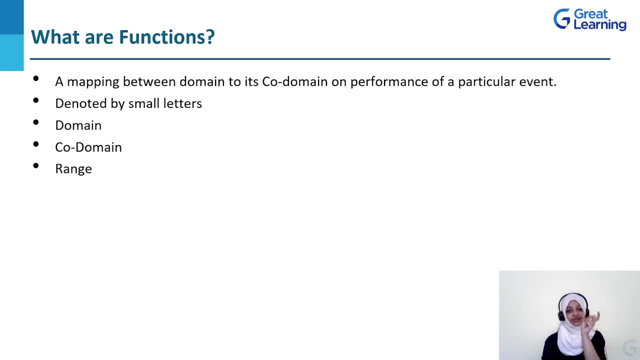 each and every function was actually contained of three separate sets, namely the domain, the co-domain and the range. We also realized that functions are just a specialized form of relation. So, again, these two work with the sets, as we've seen with relations. 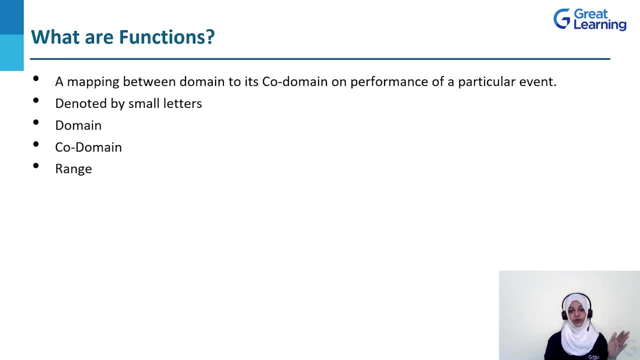 We also saw that each and every function has an input and an output. Next, we saw that the domain acts as the input. the co-domain actually acts as the possible outputs and the range is the actual set of outputs. Next, we've seen the type of 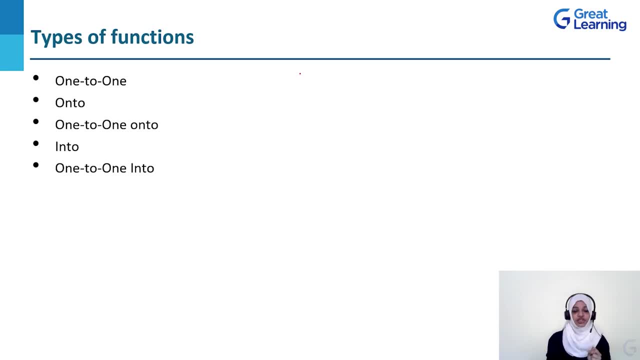 functions that we can commonly see. We've got one-to-one functions, which actually define that each and every element in the domain has to have only one related element in the co-domain. Next we've got the onto function that states that each and every element in 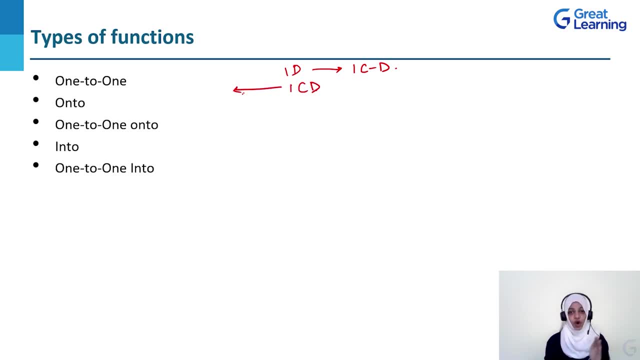 the co-domain has to have a prior image or a related input within the domain. It is not a one-to-one relation here. You can have multiple elements linked from the co-domain onto the domain, but the thing to remember is that such a linking 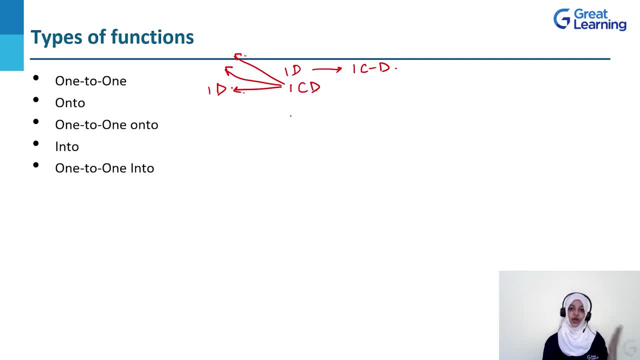 should exist. If it does, then the function is said to be onto. If a function is both one-to-one and onto, then it is known as a one-to-one onto relation or a bijective relation. Next we've got the into function, which is actually: 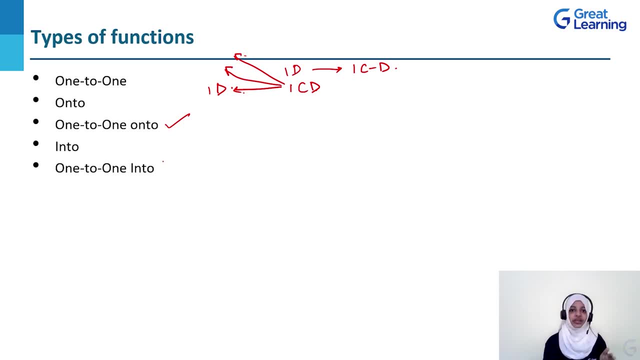 the opposite of the surjective function or the onto function as given here. So our surjective function said that each and every element of the co-domain had to have a related image in the domain. Here the into function says that there should be at: 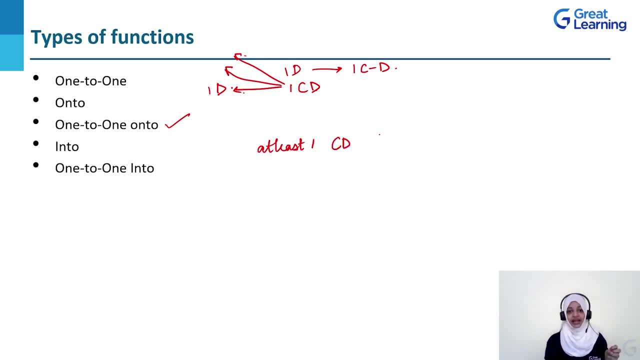 least one element in the co-domain that does not have a related image in its domain. That is what into function means. Again, if a function is both one-to-one and into, then it is known as a one-to-one into function. We've also seen illustrations of 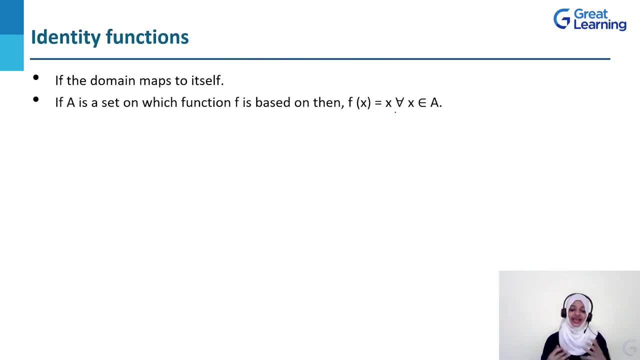 all of these types of functions with their own examples. Next, we had a look at identity functions, wherein if a function is based on a set, then the function is defined in such a manner that taking an input from our domain is going to give us an output. 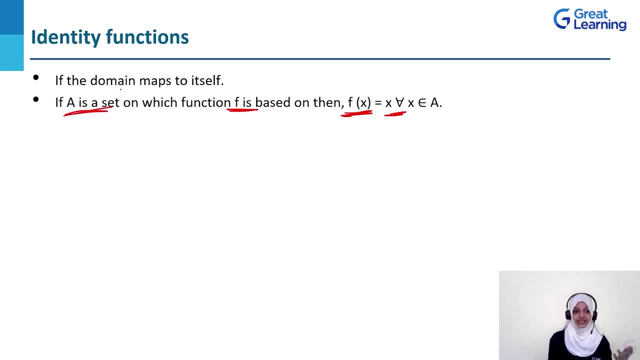 which is again a part of the domain. That means that the function is such that the domain is mapped from itself to its own self, And this happens for each and every element that would be a part of the domain. We've also seen that the 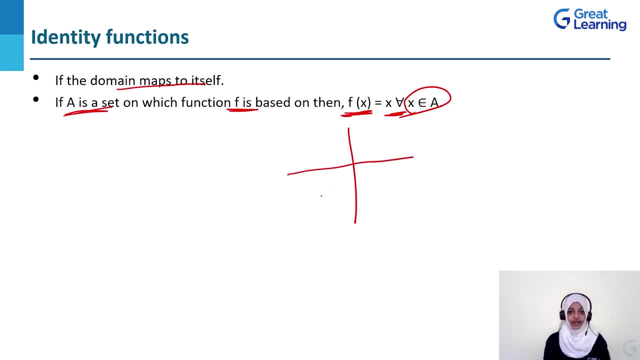 graph that often comes out of the identity function is like this, wherein every value of x is equal to the value of y, such that the graph passes through the origin at and it passes through each and every diagonal point that is present on the graph. So the values of x and y. 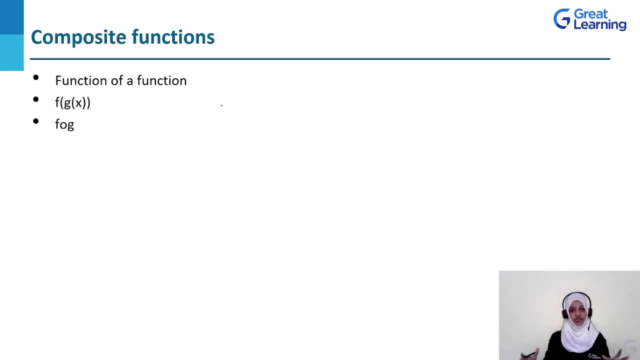 would always be the same. Next, we saw the composition of function and how the composition of function actually helps us club together various functions to perform more complex operations. This is also practically implemented in various scenarios where the outputs of some functions are going to act as the input of 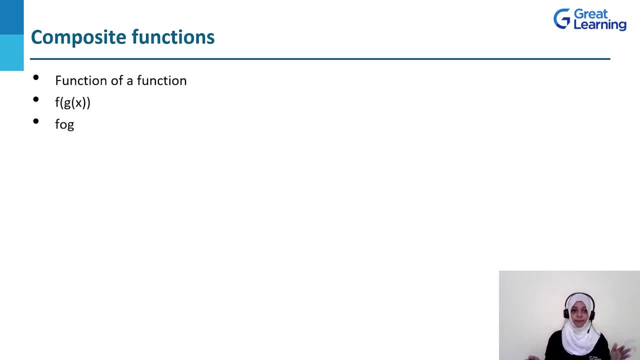 another function. That is where the composition of function comes into play. Composition of functions can be denoted using both of these denotations, either f of g or f of g of x. Either of these denotations are the right way to denote. 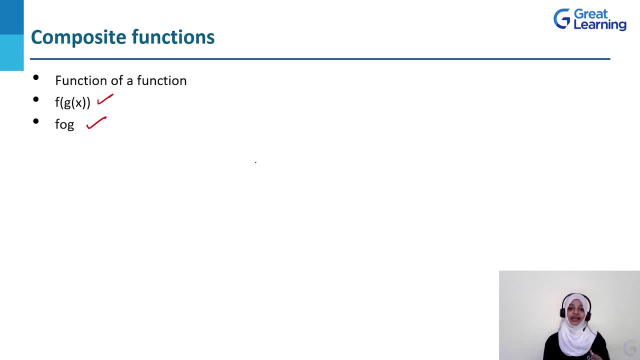 them. It's up to you which denotation you use. There can be n number of complexities. we can have n number of functions clubbed together in complex ways, such that the outputs of one function are feeding into the other function as inputs. Next we saw a series of mathematical 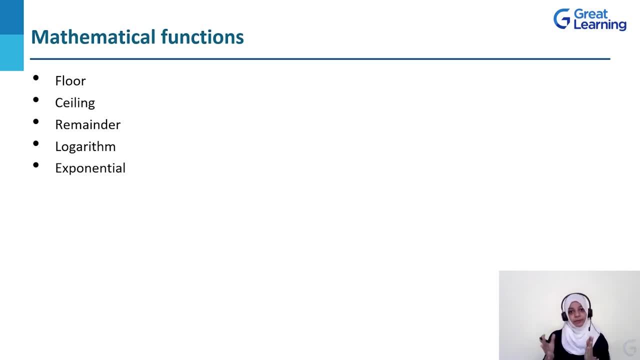 functions that are often seen or implemented in programming languages. We saw the floor function, we saw the seal function, we saw the remainder function, we saw the logarithmic function and the exponential function. We also discussed that the exponential function is often used while we are converting. 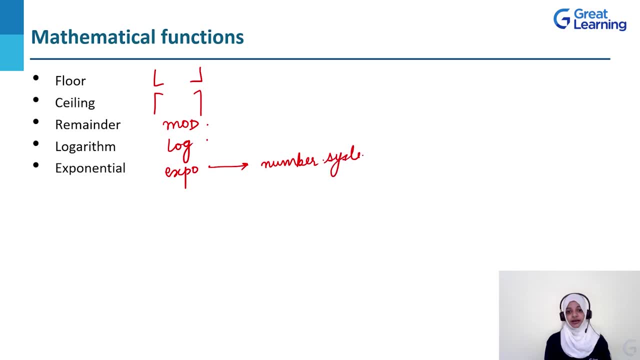 from one number system to another. So this is how we can actually implement the various functions, relations and sets that we have. Thus we've seen at the end that a set is actually just a collection of elements, whereas relations help us define a connectivity between 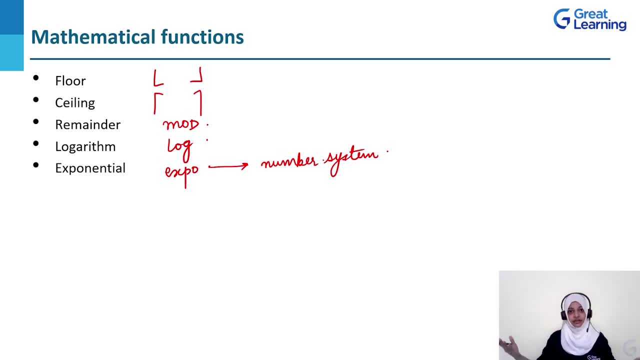 various sets that may be a part of our environment. Functions, on the other hand, are a specialized form of relations that provide equations which can help us in calculating based upon the input from the set, and they also help us determine what would be the possible output in the form of set. 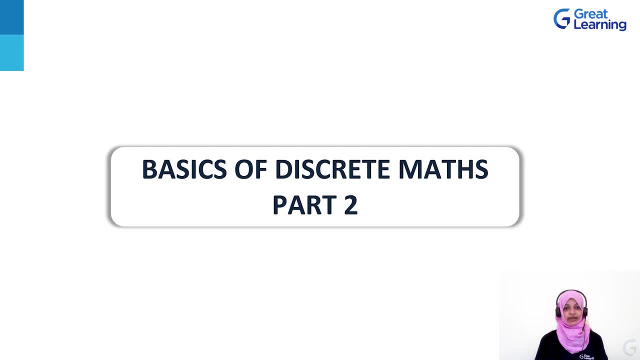 Hello everyone and welcome to the second part, in which we'll be looking at some basic concepts of discrete maths. Now, in the first part, we've already seen what set theory, relation theory and function theory were. We've also seen the relation between all of these three theories. 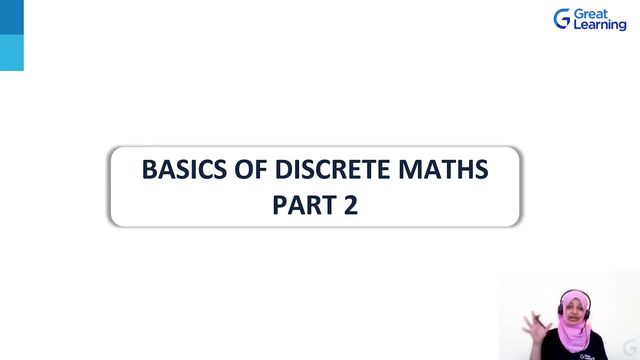 Now these theories actually form the parent set of all of the other concepts that are a part of discrete mathematics. In this particular course, we'll be looking at some of the more advanced topics that are a part of discrete mathematics. Again, these particular topics that 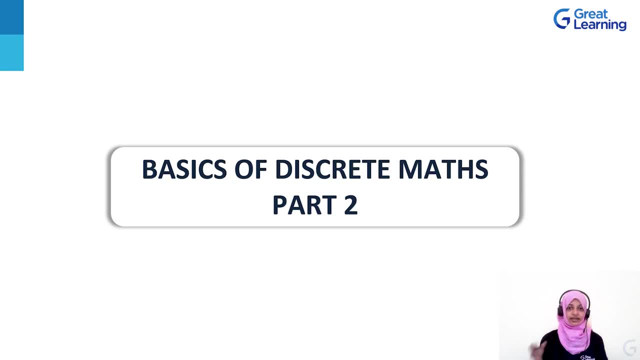 we'll be looking through might or might not use set theory at its base, So let's quickly get started. So in this particular course, we'll be learning about some of the most commonly seen counting principles. We'll be looking at what sum and product rules are. 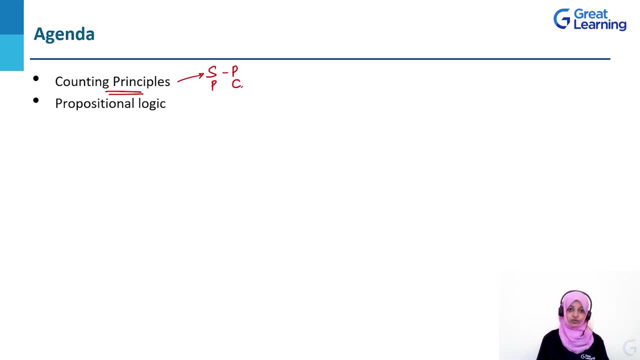 We'll be looking at some of the permutations and combination rules. We'll also be looking at a very specialized counting rule, known as the pigeonhole principle. Now, one of the most basic uses of these counting principles is selections, arrangements and apportionments. 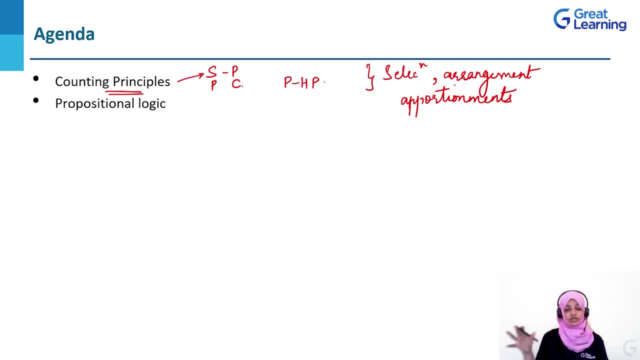 This means that if we need to select or arrange a certain set of objects in a certain manner, we'll be requiring counting principles for that. Next we'll be looking at the propositional logic section, wherein we're actually going to see how logic works and some of the most basic. 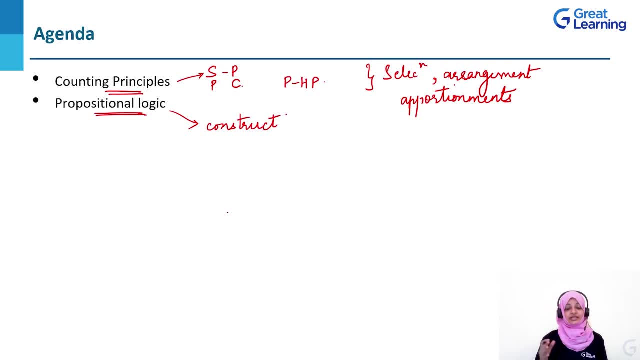 constructs of propositional logic. These constructs will actually help us understand how logic can be manipulated in one way or the other to provide us with the required output. Everything that we do in propositional logic is always going to be based upon the laws of Boolean algebra. This means: 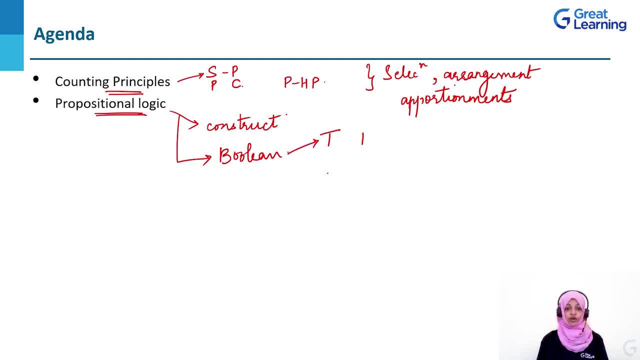 that either the outputs will be true or one in nature, or the outputs obtained here will be false or zero in nature. So let's quickly get started and dive into the concepts here. Let us first look at the counting techniques that we will be looking at in this. 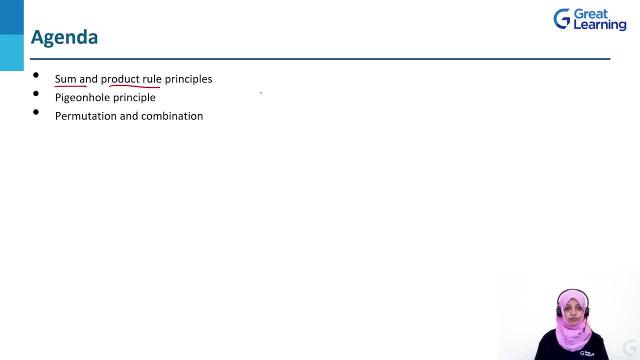 course. First we'll be looking at the sum and product rule. This particular sum and product rule actually has seen various applications when it comes to union and intersection operations in set and has also been adapted to actually fit probability. Next we'll be looking at pigeonhole. 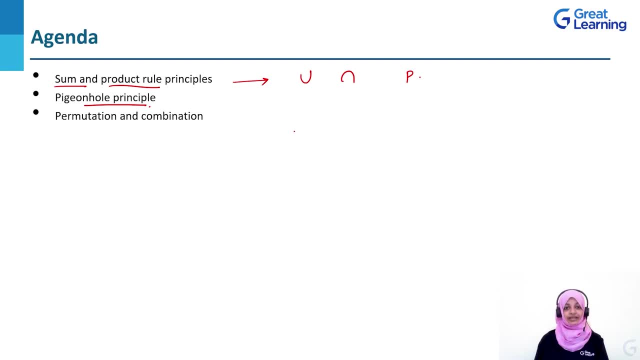 principles, which is actually a very basic principle that helps us ascertain exactly how a particular set of objects have to be arranged in a particular manner. Lastly, we'll be looking at permutation and combination techniques, with a few examples for the same. So let us first look. 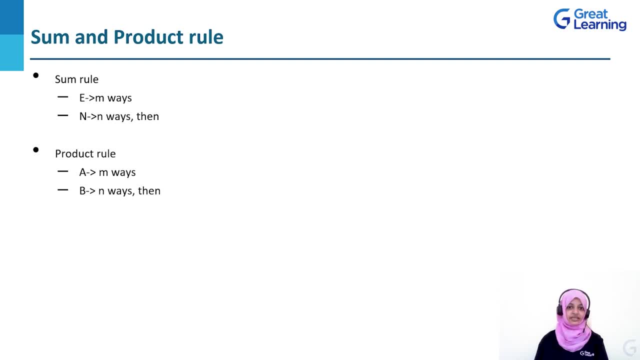 at the sum and product rule. So what is the sum and product rule? The sum rule says that if we have an event E which can be carried out in M ways and we have an event N which can be carried out in N ways, then the number of ways 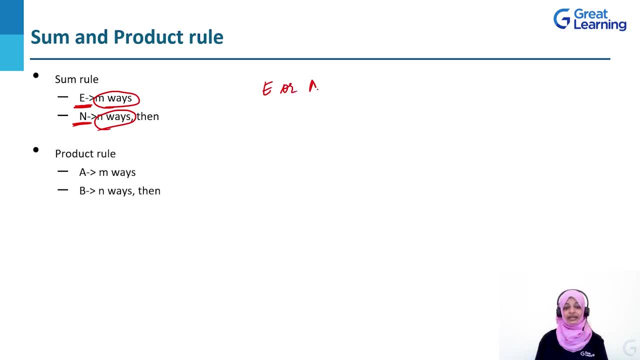 in which E or N can be carried out is actually number of ways of carrying out E plus number of ways of carrying out N. This means that if we do not have a preference over which one of these events need to occur or which of these events need to be completed, 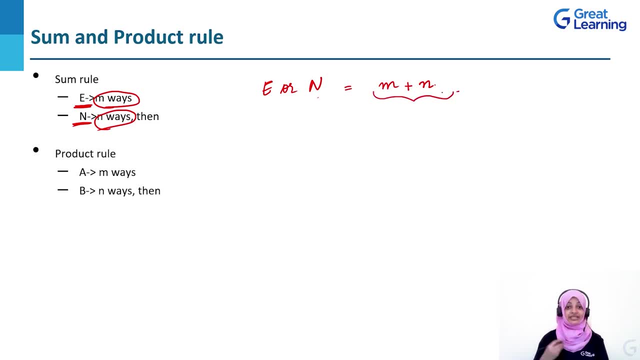 then the total number of ways will be the sum of their individual number of ways. On the other hand, the product rule states that if we have an event A that can be completed in M ways and a product B that can be completed in N ways, then the number of ways 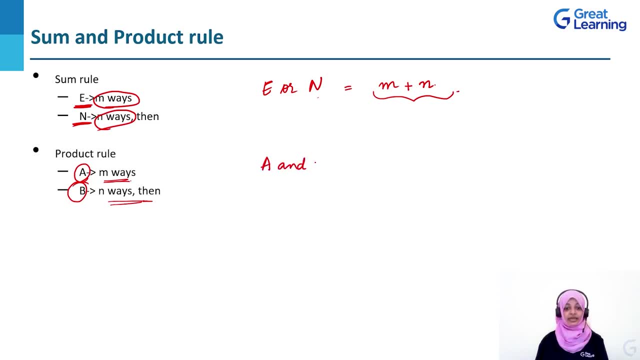 in which both A and B can be completed will be the product of their individual number of ways. One of the things to note here is that these particular events are supposed to be independent of each other. This means that A and B are not really dependent. 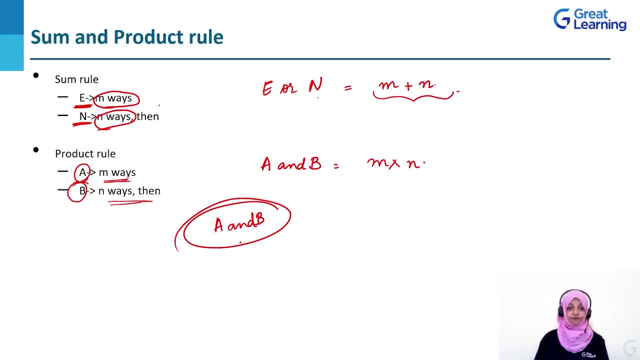 upon each other for their completion. Similarly, for the sum rule, E and N are not really dependent upon each other for their completion. Since they are independent events, the number of ways in which they can be completed are also independent in nature. As a result, 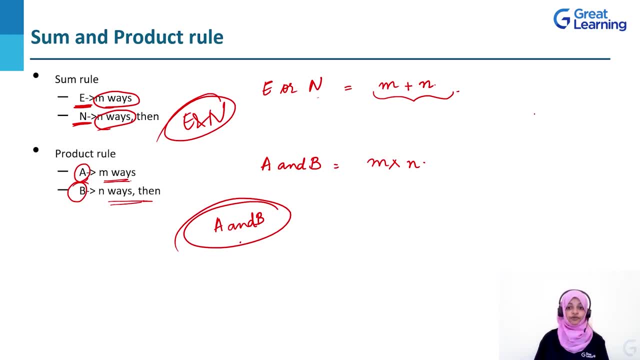 the sum and product rule are always true for all independent events that might be a part of any environment. Let us understand this with an example. Say we have 10 apples and we have 10 oranges. The number of ways in which we can pick up an apple is. 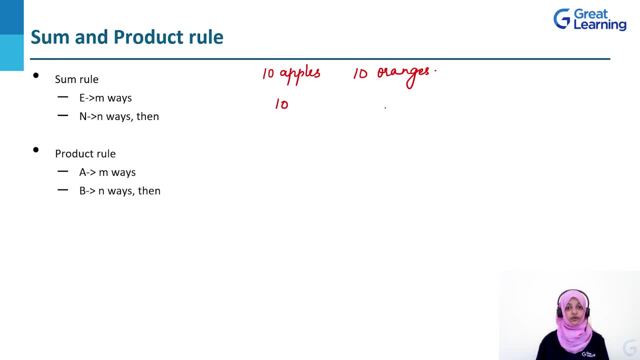 10, and the number of ways in which we can pick up an orange is also 10 ways. So, since these two events are not dependent on each other, we can say that the number of ways in which we can pick one fruit is if we pick either apples. 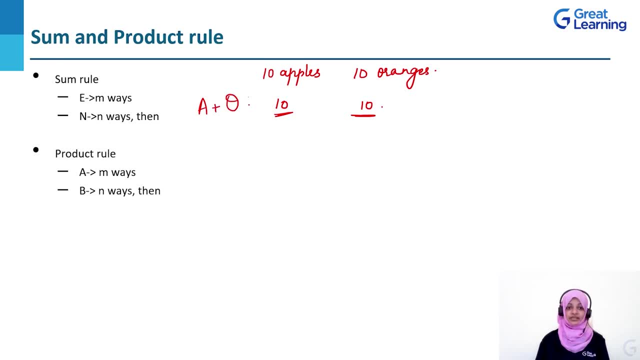 or we pick oranges. This means that we are utilizing the sum rule here. As a result, the number of ways in which apples or oranges can be picked are actually 20 ways, Which is the individual sum of the two ways in which the events can be completed. 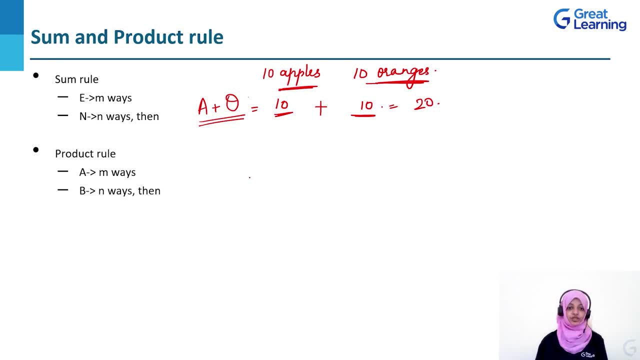 Next, if we are picking out a bunch of fruits, we can say that the probability of picking apples and oranges- Now, please note, here we are saying a bunch of fruits, not one of them, So number of ways in which apples and oranges can be picked are actually. 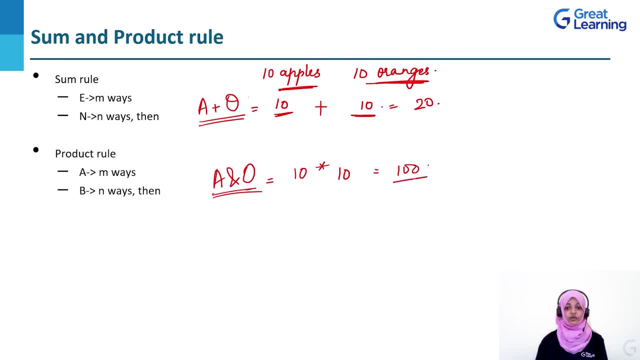 10 x 10. Which is 100 ways. Now, what are these 100 ways? We could either pick a bunch of 10 apples, or we could pick a bunch of 10 oranges, or we could pick a combination of 5 apples and 5 oranges. 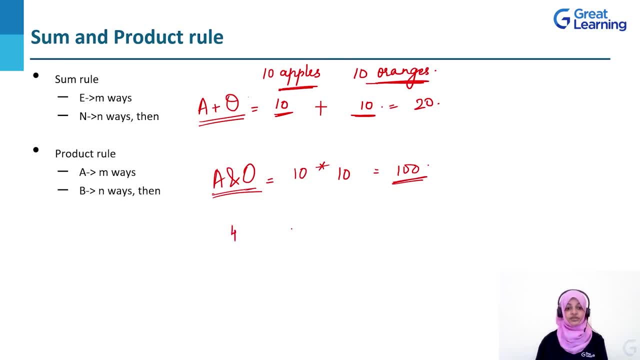 or we can pick a combination of 4 apples and 6 oranges, or we can pick up a combination of 3 apples and 7 oranges, and so on and so forth. In any case, at the end we can pick 10 of any fruit, and at the start 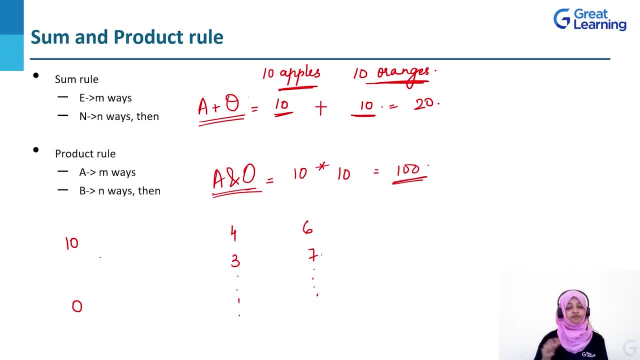 we can pick 0 of any fruit. As a result, the number of combinations in which a bunch of fruits can be picked up are multiple in nature and can be found out by using the multiplication rule or the product rule. Next, we are going to look into 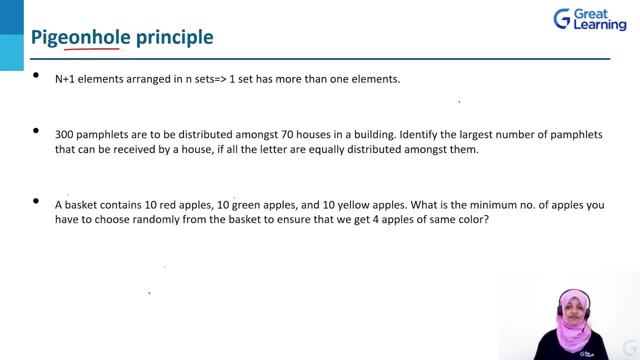 the pigeon hole principle. The pigeon hole principle is a very important apportionment technique. Now, what is apportionment? Apportionment is actually the technique by which you are able to distribute a given set of resources between a given set of people. 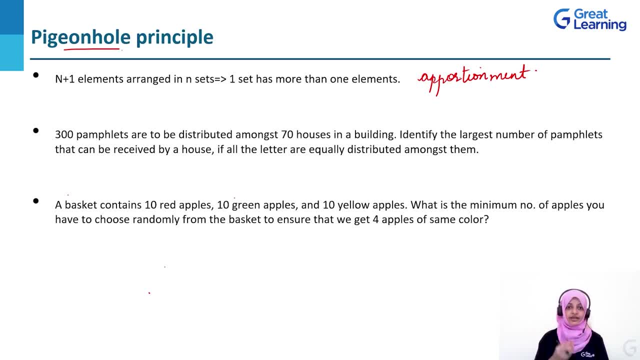 It can always be thought of as arranging a certain number of objects into some given containers. So the pigeon hole principle is one that states that if you have n plus 1 elements and you arrange it in n sets or n containers, then there has to be 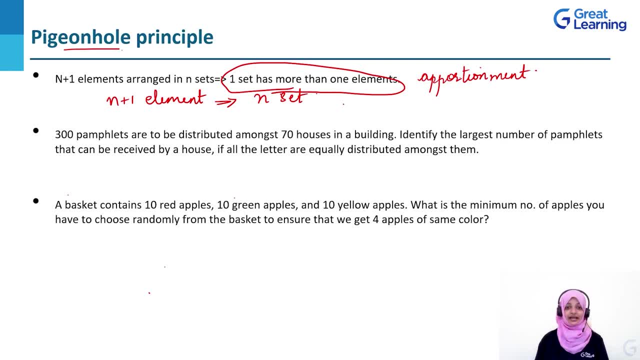 one particular container at least that has one more element than the others. Think about it in this manner: If we have 21 pencils but we have only 20 slots, then there would be one slot that would have to contain two pencils in them. The rest, 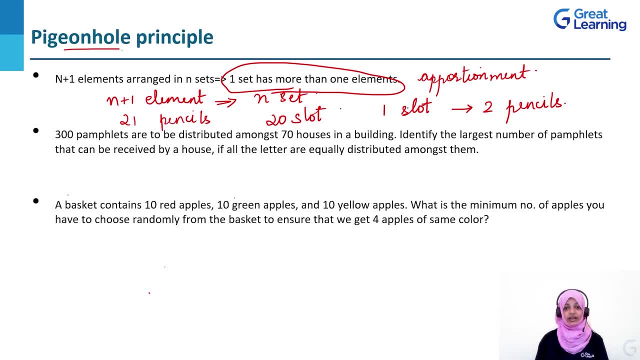 of the slot would all contain one pencil each, while one unique slot will contain two within itself. This is what the pigeon hole principle says. Now, there are two ways of implementing the pigeon hole principle. One is using the formula, and the other one is using 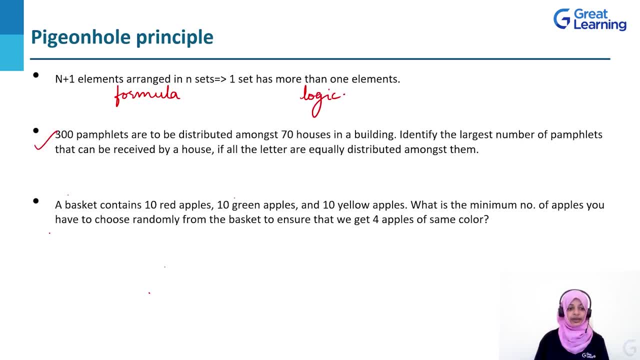 logic. Given below are two examples: one in which we will be using the formula and the second one in which we will be using logic to determine exactly what the answer is. Let us first understand what the formula is. As per pigeon hole principle, if we have 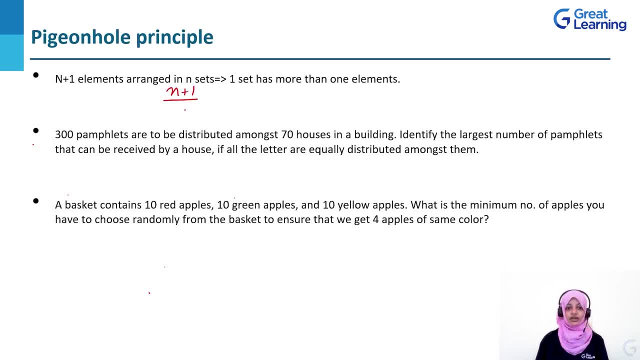 got n plus 1 elements and they need to be arranged in n ways or, for that matter, in any kind of arbitrary n ways. then we are supposed to divide the two values and take the seal function of the values. Now, what is the seal function? 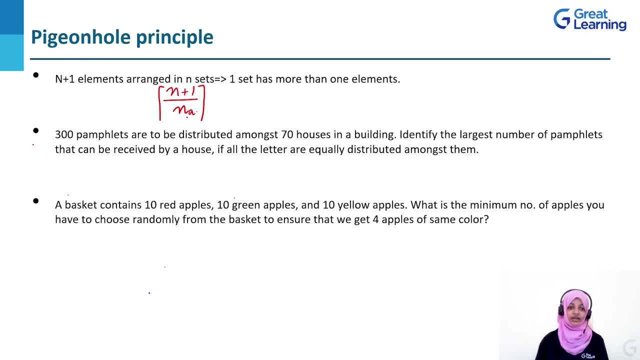 The seal function is actually the smallest value that is greater than whatever value is under consideration. For example, if we have got 8.23, then the value just greater than this would be 9.. That value will be known as the seal value for 8.23.. 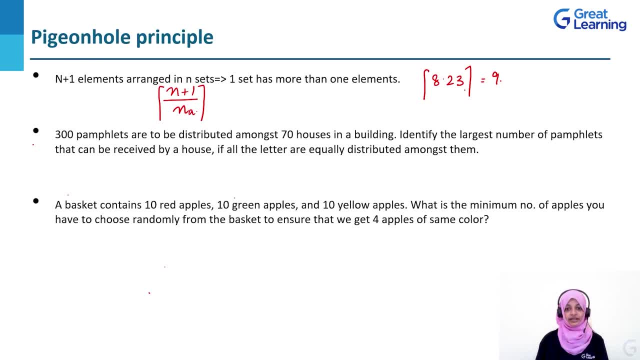 The integer, which is larger than the value under consideration, but the smallest value when you look at it in comparison to the other large values. Now, what does this formula actually give us? the answer: This provides us with the largest number of elements that have to be put. 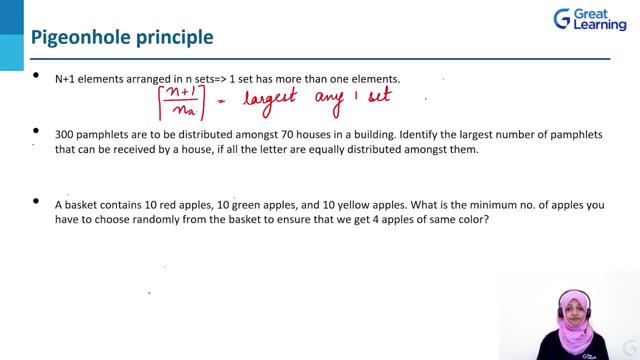 in any one set if there is a fair distribution of all of the elements that are actually available to us as resources. So what it is actually doing is it is fairly distributing all of our resources into various containers and then looking at what is the largest value, that any. 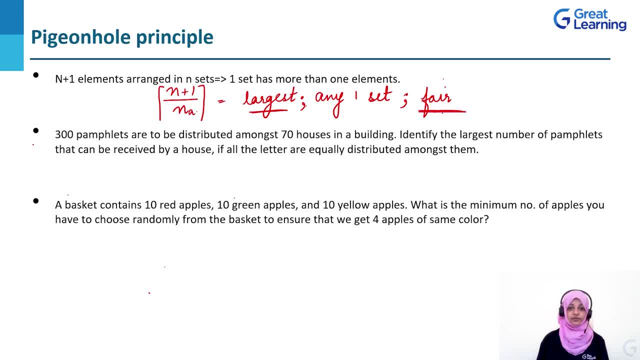 container would contain if there is a fair distribution Right. So let us understand this with an example. Now suppose we have our first question as given. here We have got a building in which there are 70 houses. We have 300 pamphlets. 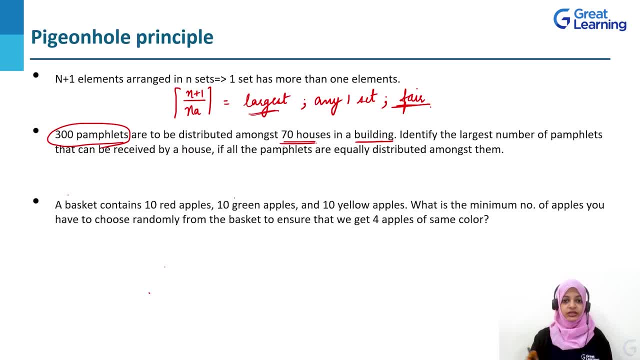 in total, which need to be distributed fairly amongst these 70 houses. What we need to identify is what is the largest number of pamphlets that any one house can receive, if all of them are equivalently or fairly distributed amongst all of the 70 houses? So how? 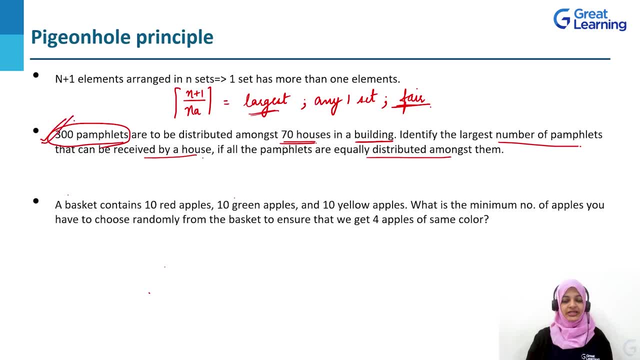 do we actually do this? Think about the 300 pamphlets as the objects that need to be distributed and the 70 houses as the containers where these objects need to be distributed. Therefore, using our formula as given here, we can say that we have got a maximum of. 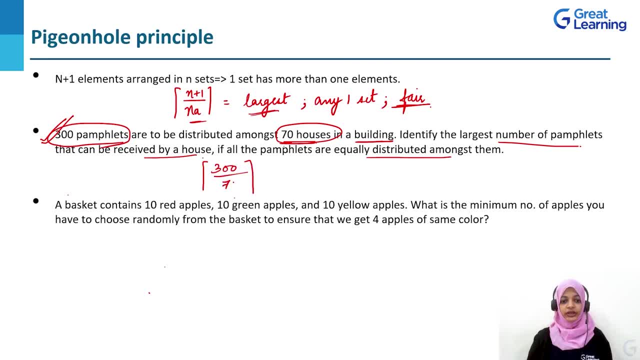 ceiling of 300 upon 70.. On calculating this value, you will find out that the value actually comes to 4.8 and a few more decimals after that. This is a non-terminating decimal and the seal value of this decimal will actually equate to. 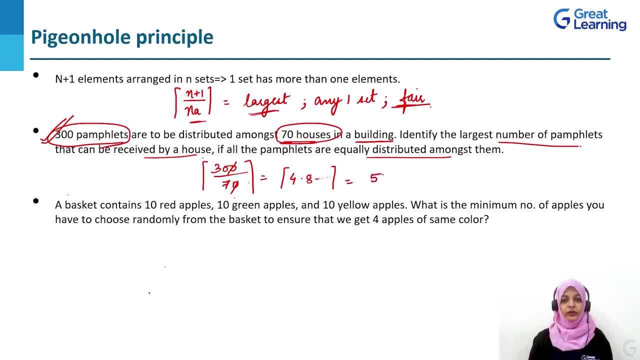 5. Therefore, from this particular example we can say that in these 70 houses, one house, or more than one house, can receive a maximum of 5 pamphlets, whereas in other cases people might receive 4 or less than 4 pamphlets. also, 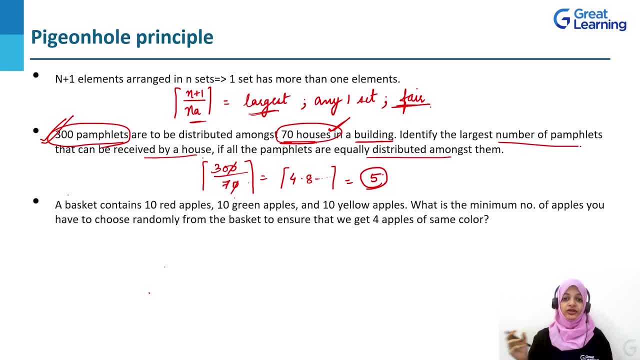 So if the pamphlets are equally or equivalently distributed or fairly distributed amongst the various houses, then we can say that 5 pamphlets are the maximum number of pamphlets that can be received by any one house. Next let us look at the second example. 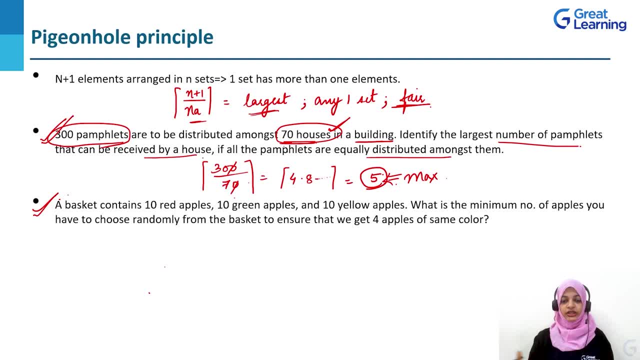 In order to solve the second example. we will be doing this both using the formula method as well as the logical method. Let us first understand how we can solve this using our formula method. If we read this question carefully, we will see that we have got 30. 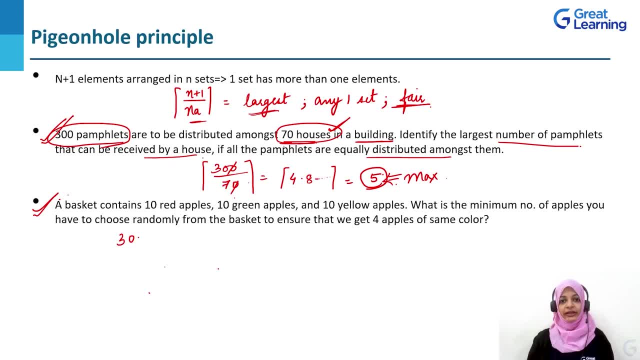 objects that have been distributed in a particular manner, such that 10 of them are green apples. that is, We have got 10 of them which are red apples and we have got 10 of them which are yellow apples. So the distribution has already been done. 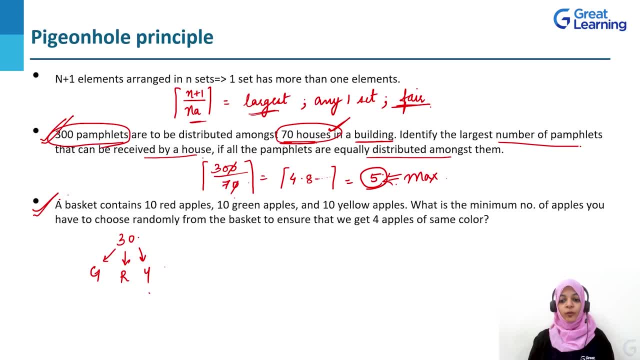 What do we have to find out here? We need to find out how many apples do we need to pick in order to obtain 4 apples of exactly the same colour. So what we need to do here is very simple. We have been told that. 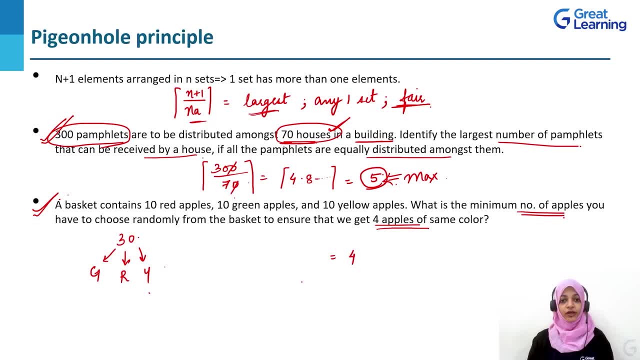 we have got to pick 4 apples of the same colour. So that is our end result: 4 apples of the same colour. Where do we have to pick these apples from? We need to pick it from our basket. How many do we need to pick? 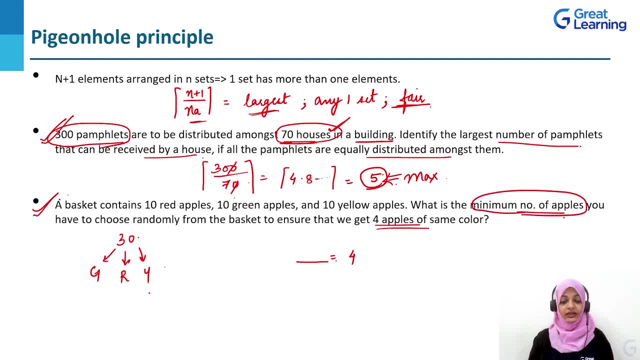 That is what we need: to determine The minimum number of apples that we need to pick And how many baskets or how many containers do we have? Logically, since we have got apples of green, apples of red and apples of yellow colour, we can say we have a logical. 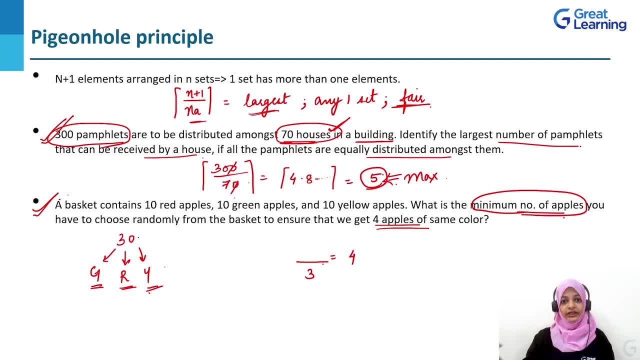 container ship of 3.. 3 different container pertaining to 3 different colours. Now we need to find out what is the missing value here. Now, how do we solve this? Solving this is very simple. If we take 9 upon 3. 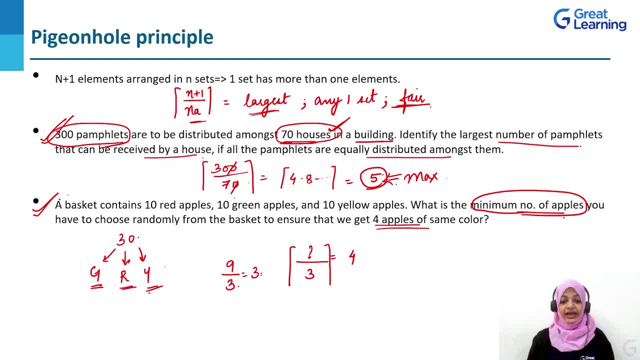 it would give us a perfect answer of 3.. This particular answer can never give us a seal value of 4.. So what do we do? We add one value here. As soon as we add one value here, this would give us 10 upon 3. 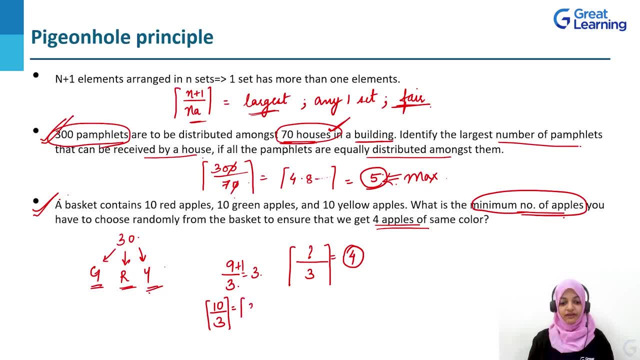 and 10 upon 3 actually will give us a division value of 3.333, and so on and so forth. When we take the seal value of this, we will actually get a perfect 4.. So the minimum number of apples that we need to select in order to get 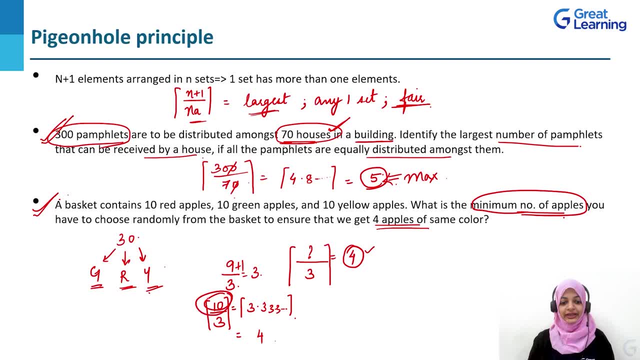 4 apples of the exact same type becomes 10.. So our value here would be 10 apples. We need to pick out minimum 10 apples. Next, let us understand this in a more logical manner. This is our situation currently. We have got: 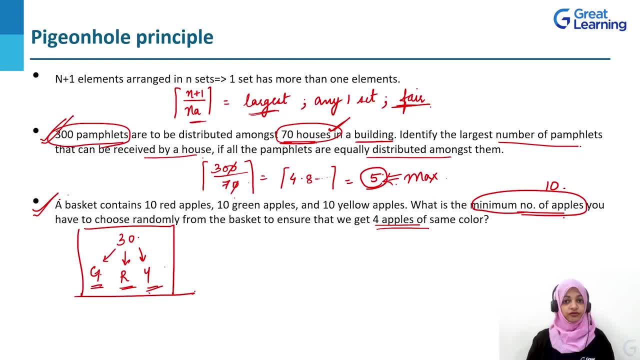 30 apples in total, such that we have 10 of green, we have 10 of red and we have 10 of yellow. We need to pick out apples in such a manner that we have got 4 apples of the exact same colour. 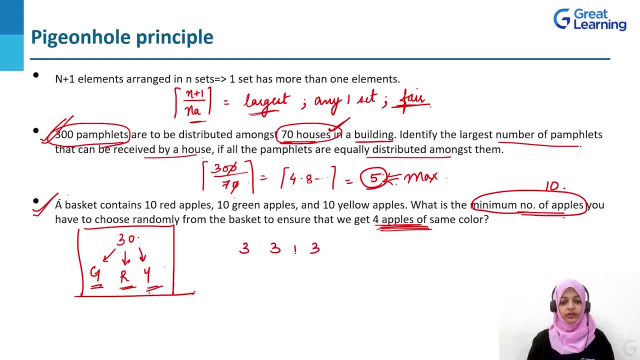 Let us say we pick out 3 apples of each colour, Right? So we have got 3 apples of green, we have got 3 apples of red and we have got 3 apples of yellow. On picking out just one more apple, what do we obtain? 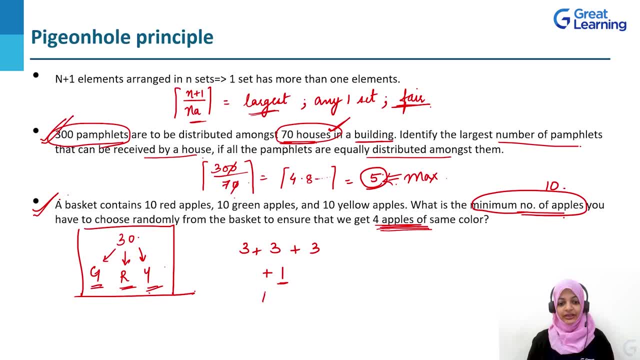 Now, this one apple that we are picking out here can either be red, or it can be green, or it can be yellow. In any case, with our green, red and yellow apples previously chosen, we will get at least one apple which is going to be of another colour here. 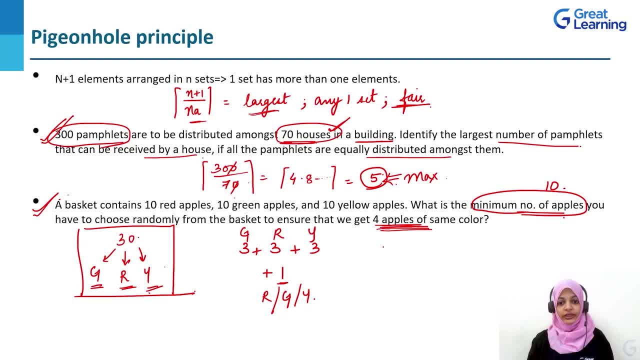 So what does this do? This actually means we will get a combination of 4 greens, 3 reds and 3 yellows, or 3 greens, 4 reds and 3 yellows, or 3 greens, 3 reds and 4. 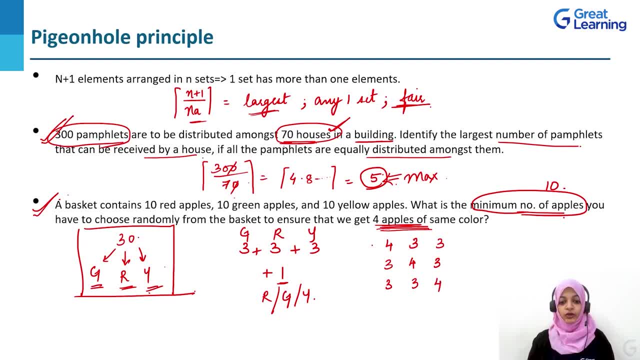 yellows. In each of these cases, you can see that the total number of apples that have been picked up is actually equal to 10.. So this means that even if we are logically picking out the various items in such a manner that we get 4 apples, 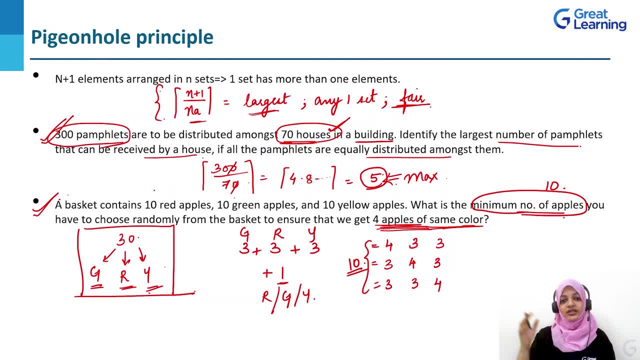 of the same colour or if we use the formula given here. irrespective of the method that we are selecting, the pigeonhole principle will give us a minimum value of 10.. This means that 10 minimum apples have to be picked up in order to ensure that we have got at. 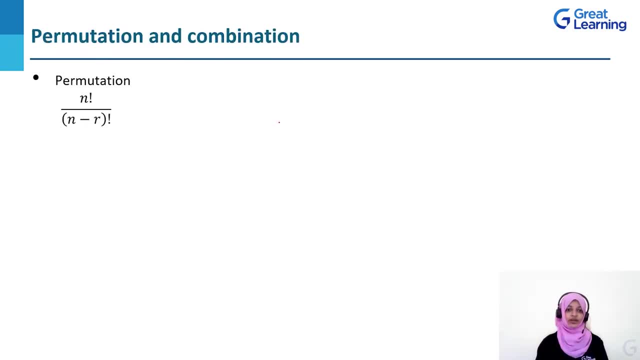 least 4 apples of the exact same colour. Next, let us look at the next concept, which is permutation and combination. The first thing we need to understand is that permutation, or NPR as it is often portrayed, is a way in which we may arrange objects in a certain 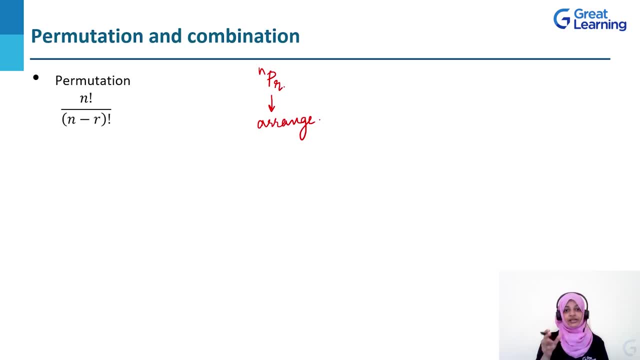 given order. So if we know exactly how a set of objects have to be arranged, or if we actually require to arrange objects in a certain manner, then we use permutations. On the other hand, combinations or NCR are a way in which we may select a certain set of objects. 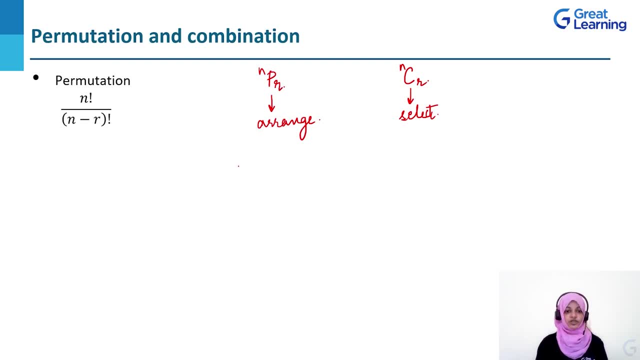 Let us understand this with an example. Suppose we have got a list of hobbies. If we need to arrange the given hobbies into a certain set of likes, then we would require permutation for that. On the other hand, if we simply have to select our favourite, 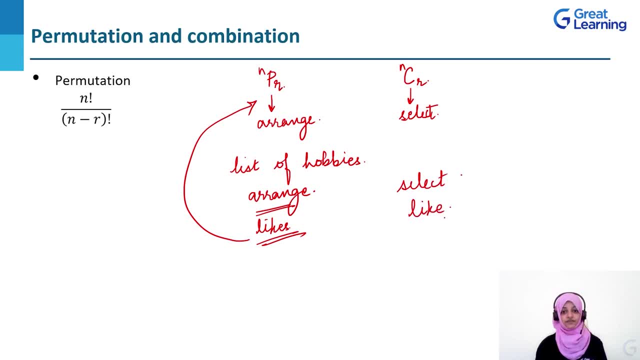 hobbies or likes from the list of hobbies given to us, then we are simply supposed to use combination. So this is how we can differentiate between permutations and combinations. So any permutation given by NPR can actually be set up using this particular mathematical formula. It is 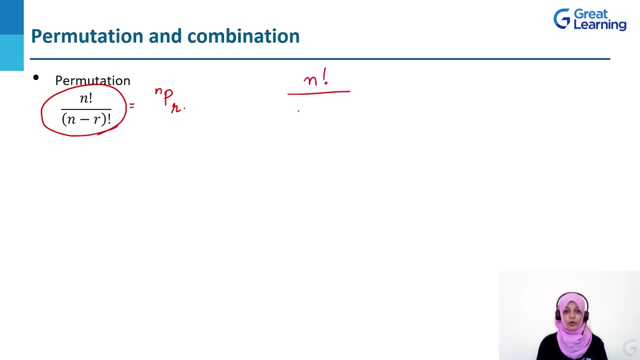 actually read as N factorial upon N minus R factorial. So given two numbers, for example 3 as R and 7 as N, 7 P 3 will actually be equal to 7 factorial upon 7 minus 3 factorial. What this gives us is a. 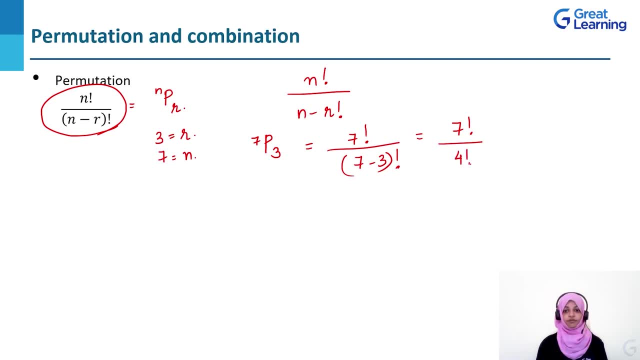 simple answer of 7 factorial upon 4 factorial. Now we know that factorial is actually 7 into 6, into 5, into 4, into 3, into 2 into 1.. Similarly, factorial of 4 would be equal to 4 into 3 into 2 into. 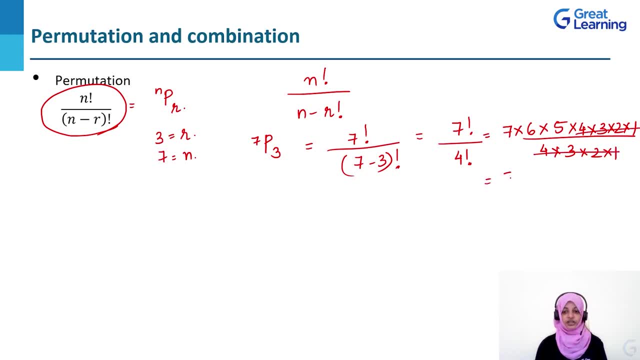 1. All of these values, after cancelling each other out, would give us 7 into 6, into 5.. Right Now, observe closely: If you have a set of 7 vehicles and you need to arrange them in 3 ways, such that you are actually. 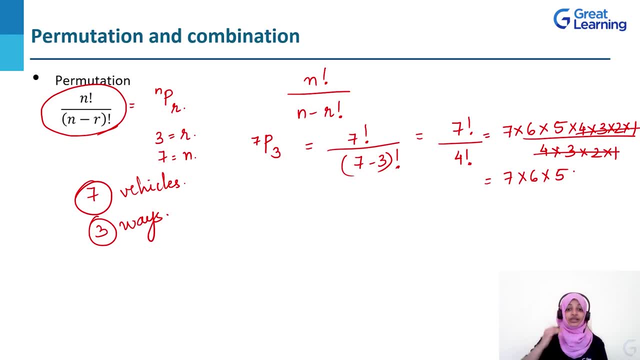 trying to arrange them from the most commonly used to the least commonly used. In the first position you are going to have the 7 vehicles as an option. You might choose one from them, but you have an option to choose from 7.. Next for. 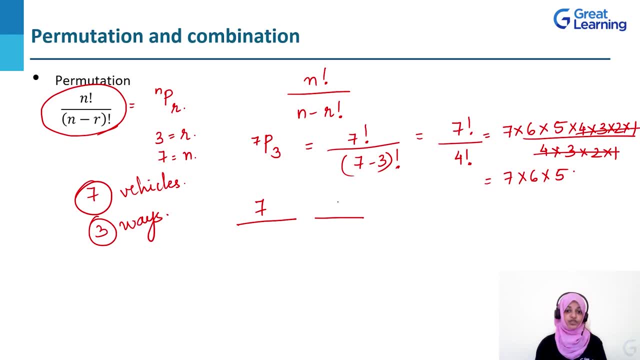 the second position, you will only have an option of using 6 of these vehicles. That is because one of them has already been selected for the first position. Next, you will have an option of 5 vehicles to choose from, since the first and second positions are. 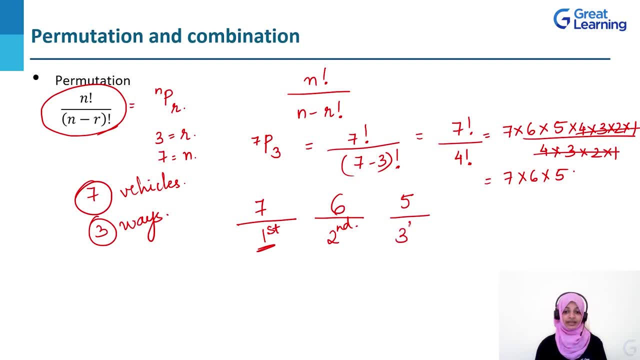 already filled up by 2 of those vehicles. Thus, if we've got 7 vehicles and they need to be arranged in 3 ways, the ways in which we can do that is selecting one from 7 vehicles and then going and selecting one from 6. 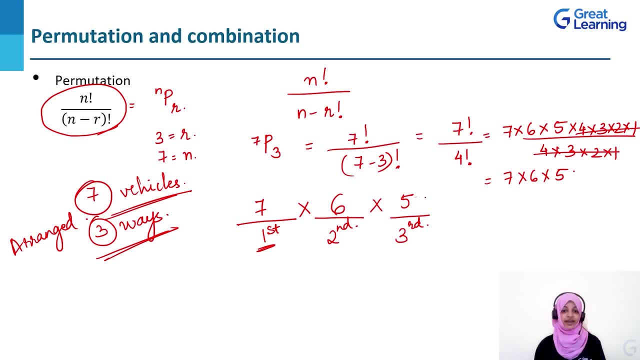 vehicles and then going and selecting one from 5 vehicles. That is exactly what we are getting as an answer here when we find out the value of NPR. This is why permutation is actually important, while we are arranging a given number of objects in a certain manner. 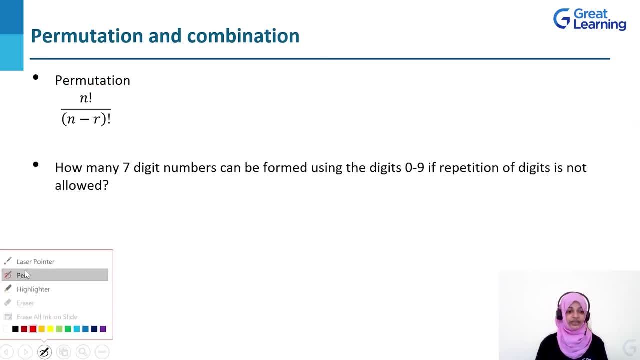 Let us now understand this concept better with the help of a mathematical example. Suppose we have digits from 0 to 9. These digits are never to be repeated. Right, That is what is given here, that the repetition of digits is not allowed. 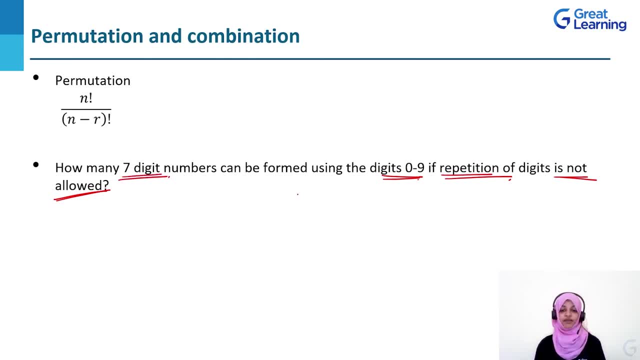 If this is the case, how many 7 digit numbers can be formed using all of these digits? Now we know for a fact that we've got 0 to 9.. If we utilize 7 of these numbers, let us see in which manner. 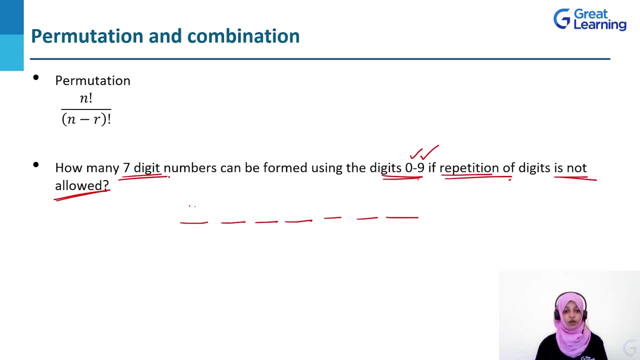 they can be arranged First. we've got 9 numbers that can be selected here. Why 9 numbers? Why not 10?? Because the moment we actually utilize 0 here there will be a problem, Right? Why would there be a problem? Because 0. 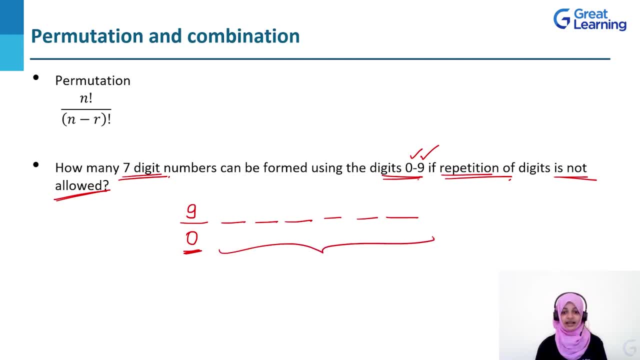 as the first number implies that the succeeding value is actually only a 6 digit number. So we will not consider 0 and we will consider the rest of the 9 values, namely 1 to 9.. Next we will then have the second position In. 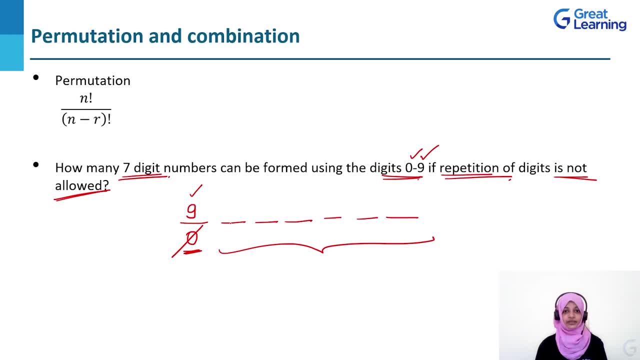 the second position, one value has already been selected from here, So we will now have another 9 values that can be attached here, Because the 9 values that we considered for the first position did not have a 0. That particular element can now be included. 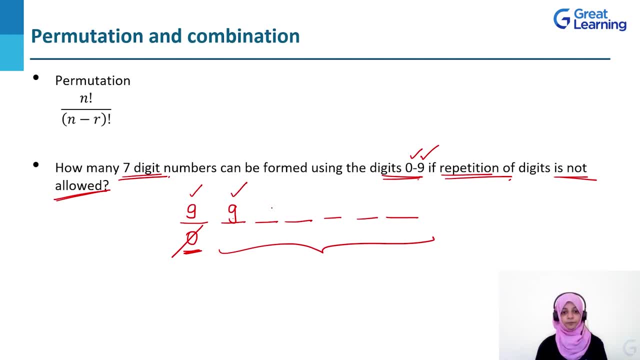 on the second position, Thus giving us a value of 9.. Next position would have 8 options, The next would have 7 options, The next would have 6 options, The next would have 5 options And, lastly, 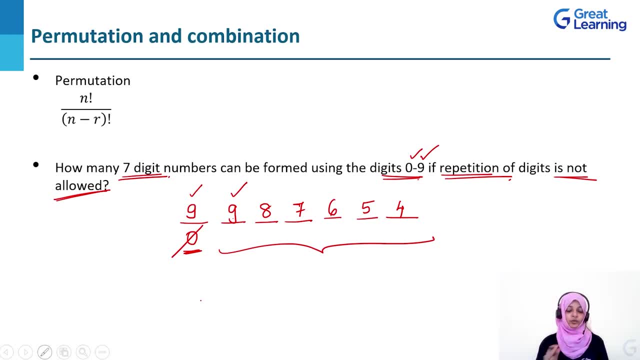 we would have 4 options. So now, how many ways are these actually, Or how many numbers have actually been created here? So we've got our first place, which gives us 9 values, And we've got our second place, which gives us 9 values. 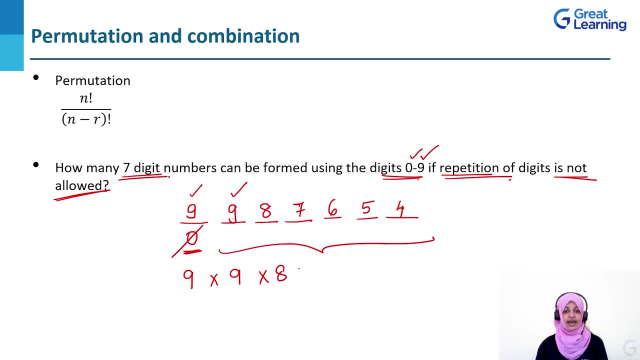 And we've got our third place, which gives us 8 values, And we've got our fourth place, that gives us 7 values, And so on and so forth. Right Now, calculating this number becomes slightly difficult. So what we do is we actually use 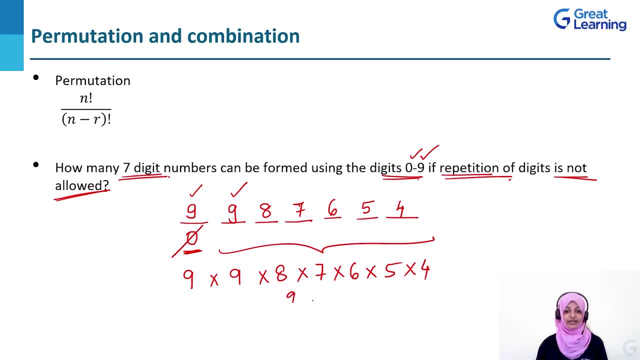 permutations. As we can see, we've got 9 values which have been arranged into 6 positions, And apart from these we've got 9 other values here. So this is what our final formula will look like: 9 into 9 factorial. 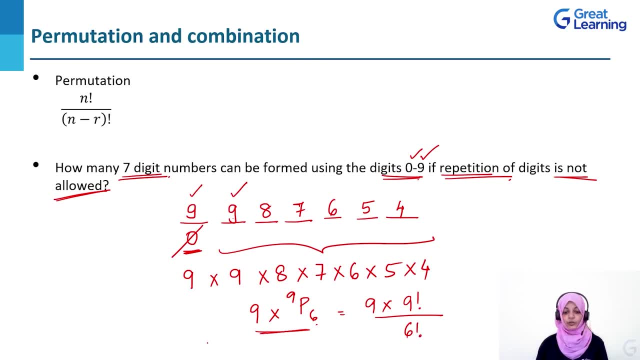 upon 6 factorial, This would actually give us 9 into 9, into 8, into 7.. The final answer of this can be found out by a simple calculation. This is the manner in which we're actually supposed to use permutations, to understand exactly. 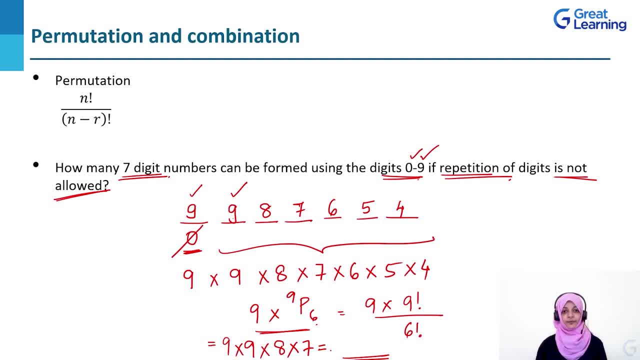 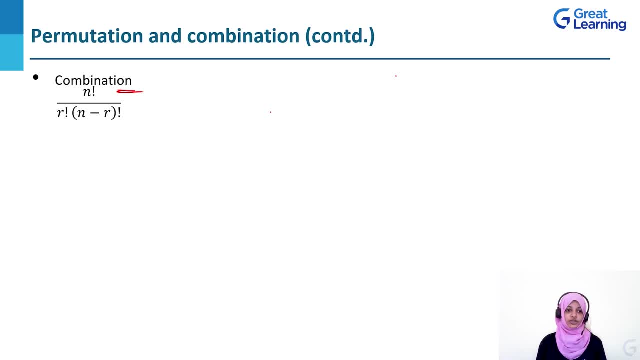 how the objects have to be arranged in a particular manner. Next, let's look at the other concept here, which is combination. Now, what exactly is combination? So, combination was actually the manner in which a certain set of objects could be selected from a parent set of objects. 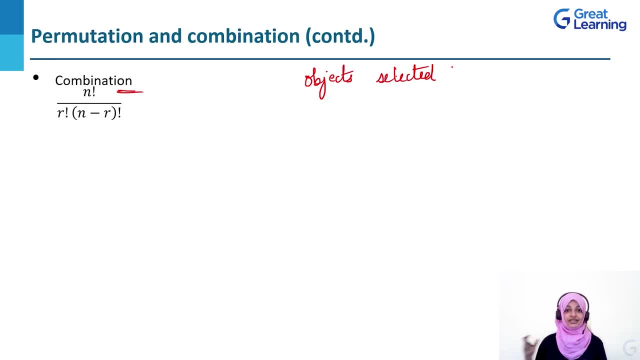 Now, one of the ways in which we can use this is to actually select a certain set of objects. Right, Let us understand how that can be done. Suppose I want to select a set of 3 objects from a set of 7 objects. 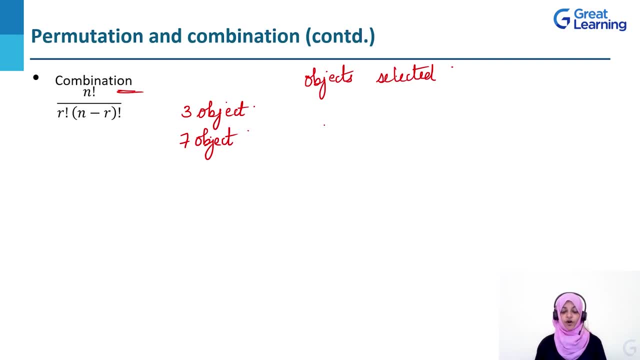 Please note that I just want to select a set of objects, Right? So let us see how this can actually be carried out. Let us take the 3 objects that have to be selected as the value r, and let us take the 7th value, which. 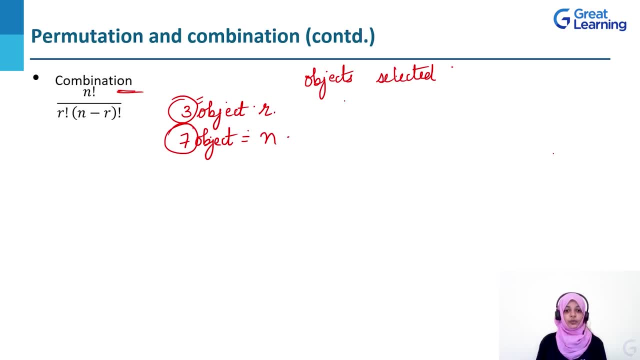 form our parent set as the value n, So we've got ncr defined as 7c3.. Right, So, as per the formula, we've got 7 factorial upon 3 factorial into 7 minus 3 factorial. This is actually equal. 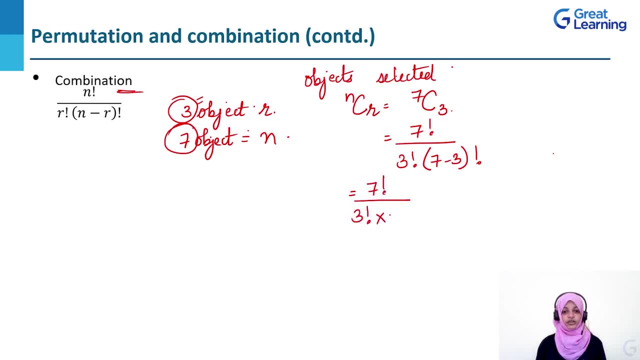 to 7 factorial upon 3 factorial into 4 factorial. This gives us 7 into 6, into 5, into 4, into 3, into 2, into 1 upon 1, into 2, into 3, which is for 3 factorial. 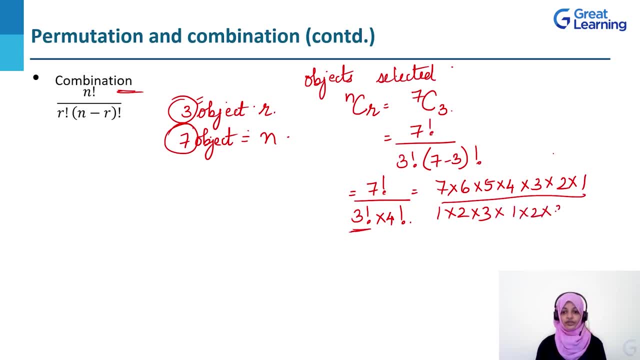 into 1, into 2, into 3, into 4, which is a part of the 4th factorial. Dividing all of the common values, gives us a final answer of 7 into 5, which is actually equal to 35. Thus we can say that. 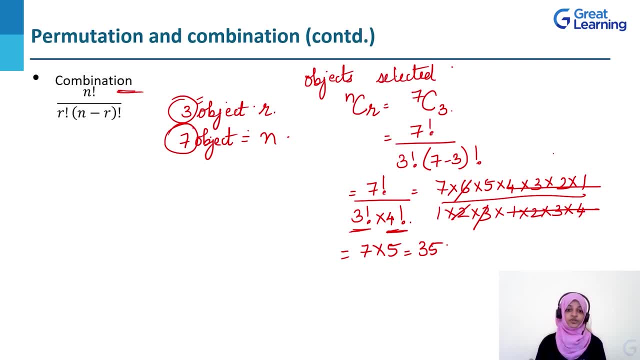 there are 35 ways in which a particular object, or 3 objects, can be selected from a set of 7 objects. Here, as you can see, we are not discriminating on any of the objects. We are just selecting 3 objects. This means that there 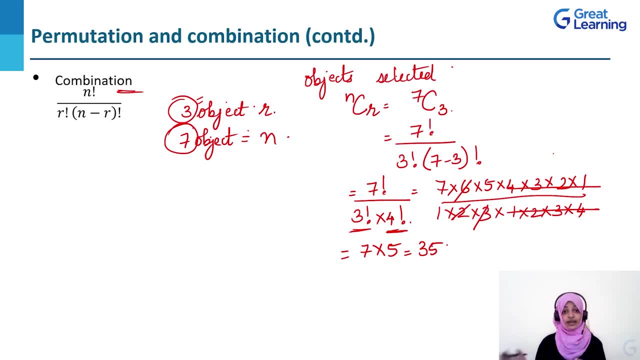 is a chance that the same object might be selected 3 times. There is also a chance that we might select one object twice and one object just once. There is also a possibility that one object just will keep getting selected 3 times, or 3 objects will keep getting. 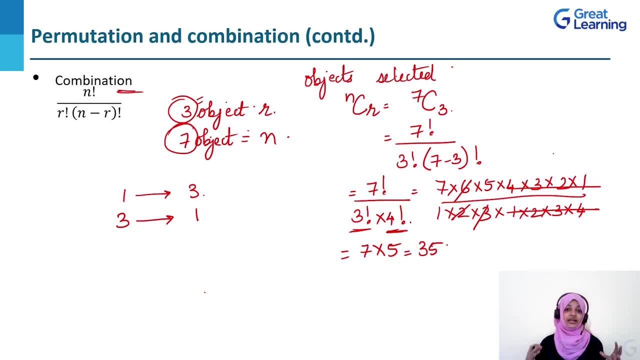 selected just once. This means that there are n number of ways in which the selection can be carried out, with no discrimination of repetitiveness or non-repetitiveness. That is how combination works. It is only concerned with selection of objects, One of the most commonly seen. 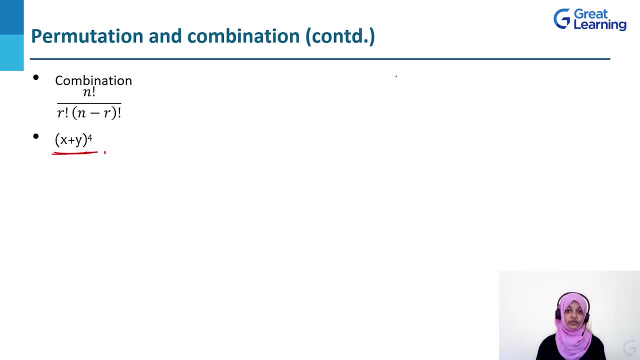 applications of combination is in binomial theorem. This is something that is often done in lower classes, and we see that for any equation given in the binomial format, the answer for this equation can actually be given by the summative identity of summations r going from 0. 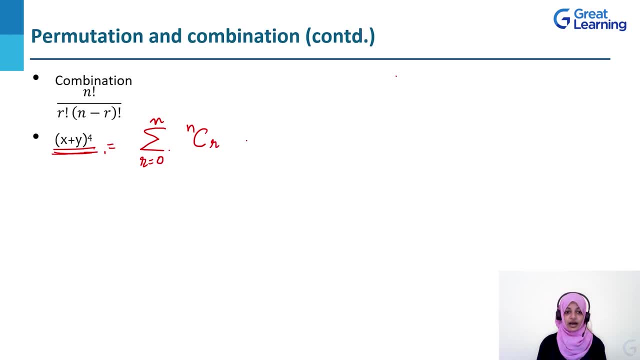 to n, ncr. x raised to n-r, y raised to r. Let us apply this in this example and see exactly what this means. As you can see, we've got a summation symbol here. This means that for values of r that are going from 0 to n, we will. 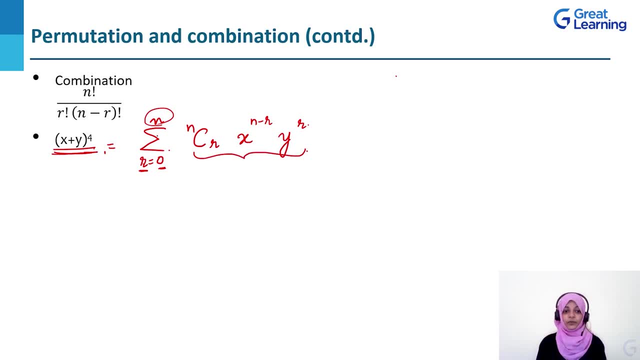 have various components that will look like this and we need to form a summation or an addition of all of these objects. Applying this formula into the example given here, we can see that we've got 4c 0 into x, raised to 4-0. 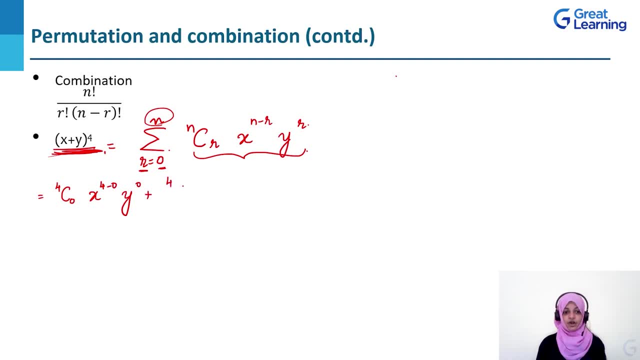 into y, raised to 0 plus 4c, 1.. Now why has this become 1?? Because the value of r will keep changing from 0 to one increment of it till it doesn't reach n. So after r was initially 0, now r. 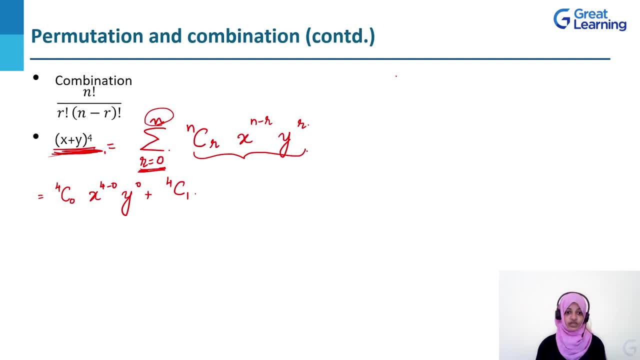 becomes 1.. Right, So we've got 4c1 x raised to 4-1, y raised to 1, plus 4c2 x raised to 4-2, y raised to 2, plus 4c3 x raised to 4-3. 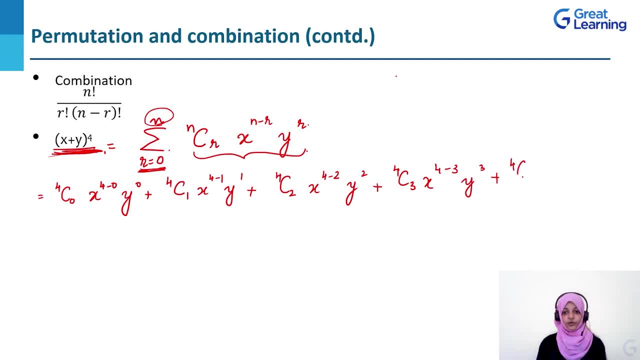 y raised to 3 plus 4c4, x raised to 4-4, y raised to 4.. Why can't we go any further here? That is because r has gone from 0, which was its minimum value, to 4, which is actually the maximum value. 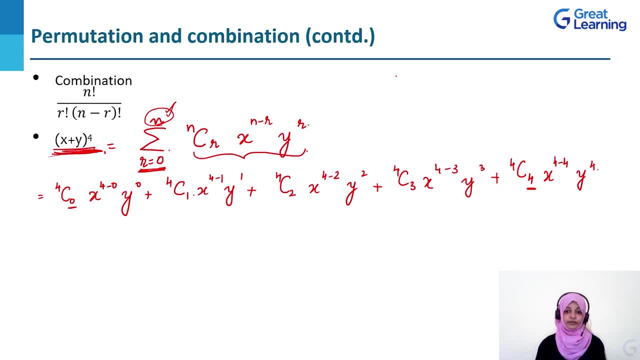 since this is the value of n in this particular example, Right? So let's see what this equates to. We've got 4c0.. 4c0 means that it's 4 factorial upon 0 factorial into 4-0. 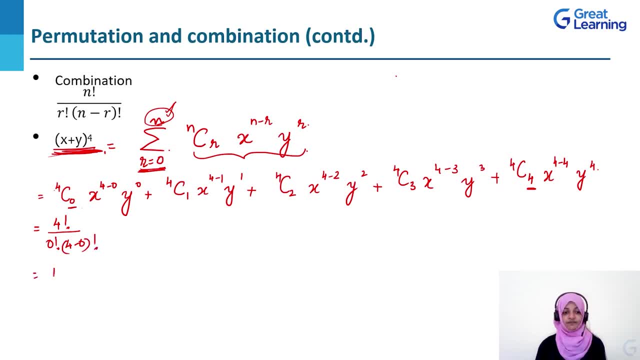 factorial. This would actually give us 4 factorial upon 1 into 4 factorial. Canceling out the numerator and denominator, we get a simple 1.. This means that the 4c0 value will actually give us a value of 1.. Next, 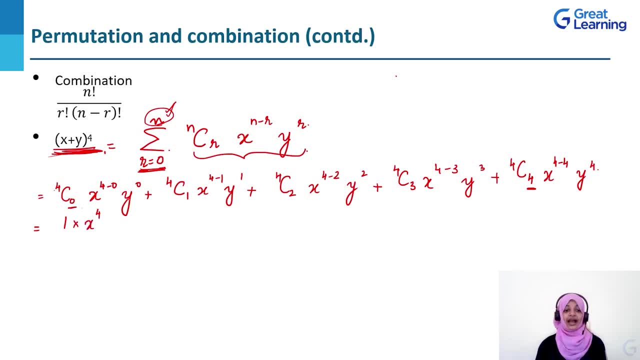 we've got x raised to 4-0, which is 4, and y raised to 0, which is actually 1, because any y raised to 0 gives us 1.. Next, let's look at this second entity given. here We've got: 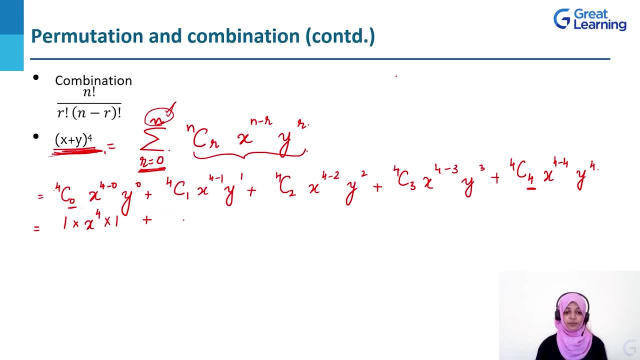 4c1.. Calculating 4c1 in a similar manner, we'll get that 4c1 actually is equal to 4.. x raised to 4-1 gives us x raised to 3 and y raised to 1 will give. 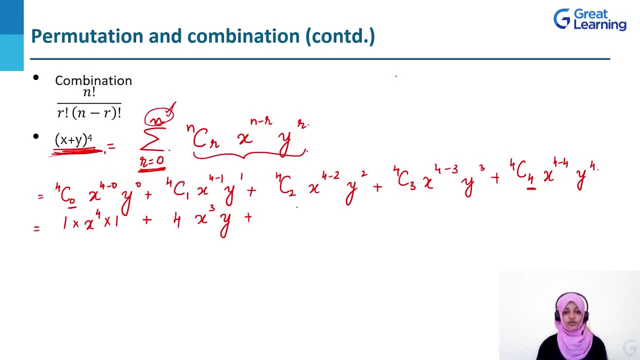 us y Next, if we take 4c2, we get the value 6.. Right, Let us see how we can get the value 6.. We've got 4 factorial upon 2 factorial into 4-2 factorial. This would give us: 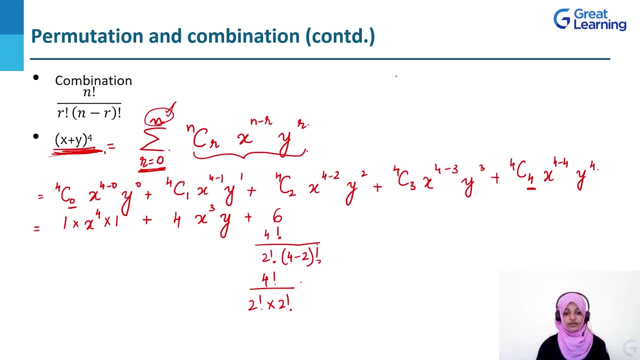 4 factorial upon 2 factorial into 2. factorial, which is equal to 4 into 3 into 2, into 1 upon 1 into 2 into 1 into 2.. The common values will easily cancel each other out and you get 2 into. 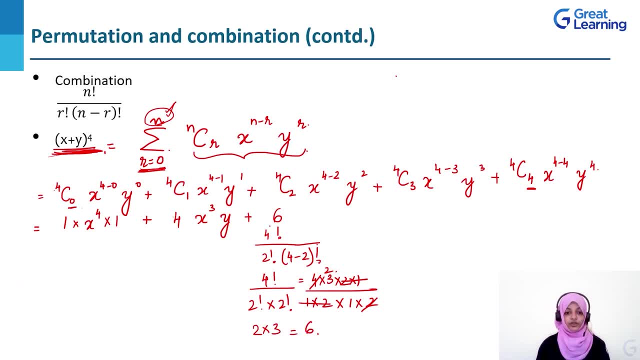 3 left out, which is actually equal to 6.. That is how you get the value of 6 here. Next, x raised to 2, y raised to 2 will be the next two values. Next we've got 4c3.. 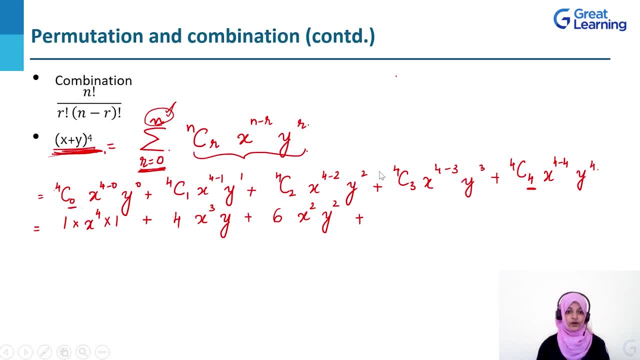 One of the best parts about combination is that here 4c3 will exactly be equal to 4c- 4-3.. Now, if we look closely, here 4c4-3 is actually equal to 4c1.. So whatever the value of, 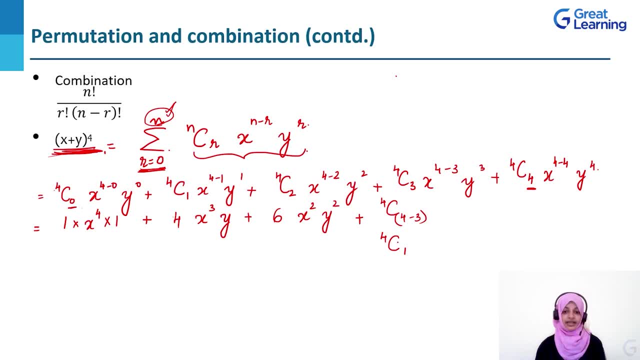 4c1 will actually be substituted here. Thus 4c3 will be written as 4.. Thus the value of 4c3 will be the same as 4c1, which is 4.. Next we've got x, which is x. 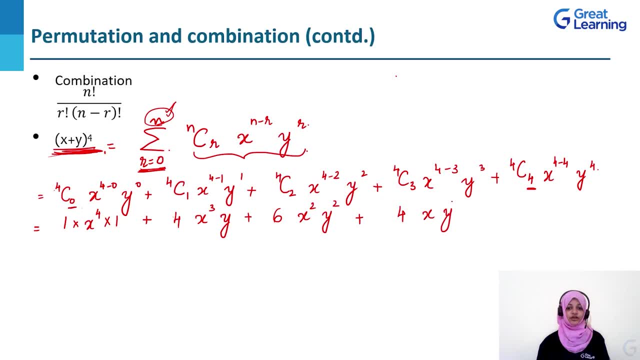 because it is x raised to 4-3 and we've got y raised to 3.. Lastly, the last term, again using the same formula, would be equal to 4c4-4, such that it becomes 4c0.. So, whatever the value of 4c0. 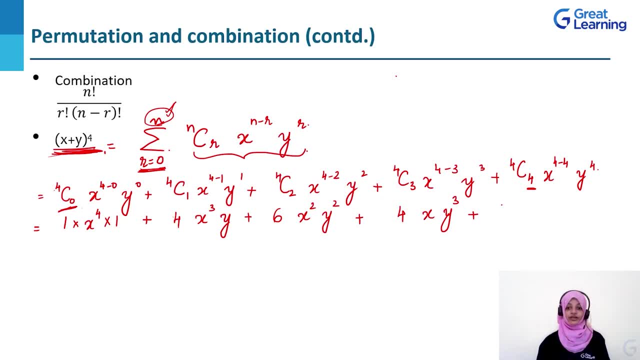 would also be the value here. Thus, the value here is 1 into x raised to 4-4, which would obviously be 0 into y raised to 4.. In the end, what our equation becomes is x raised to 4 plus 4x3y. 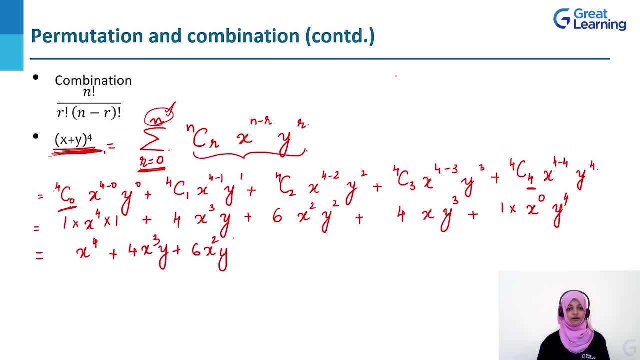 plus 6x2y2 plus 4xy3 plus y raised to 4, because again x raised to 0 would give us 1.. So, as you can see, this is how permutations and combinations can actually help solve various mathematical and real life issues. 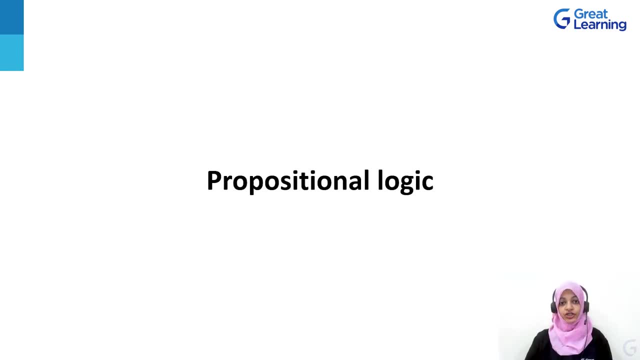 So the next topic in this particular course is propositional logic. So propositional logic, while we go through it will look like a combination of set, query and Boolean logic, which is not really wrong if you look at it. Propositional logic actually has various applications. 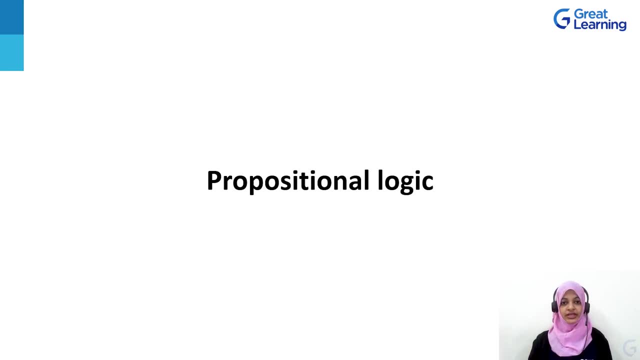 when we look at machine learning as well as compiler designing. So if we want to actually make any machine understand, or any machine learn on its own, we first need to program it in order to be able to learn. This kind of programming is actually carried. 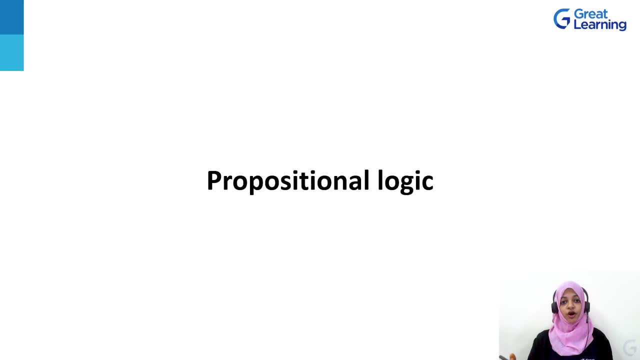 out using propositional logic. Propositional logic forms the basis for logic and knowledge development of any and all compilers and machines. So let's look at its components first. So first we are going to look at an introduction To propositional logic. next we 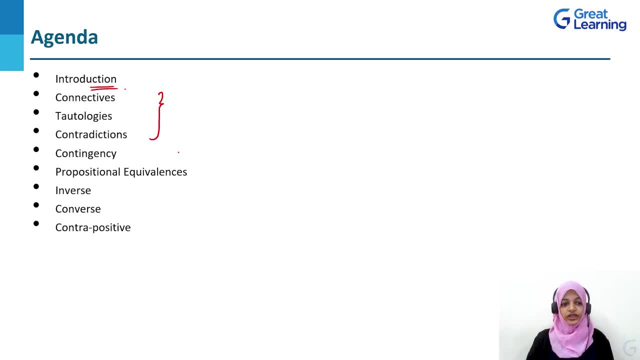 are going to go into the connectives, the tautologies, the contradictions and the contingencies. Now, what are these? how are these related to one another will be seen later on. One thing to remember here is that connectives often act as: 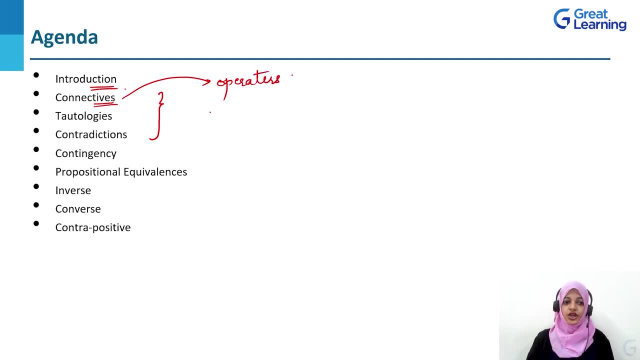 operators do in other programming languages. So please make a note that you have all of your connectives in mind while you go into the more advanced levels of propositional logic. Next we are going to look at the concept of propositional equivalence, how it can be proved and 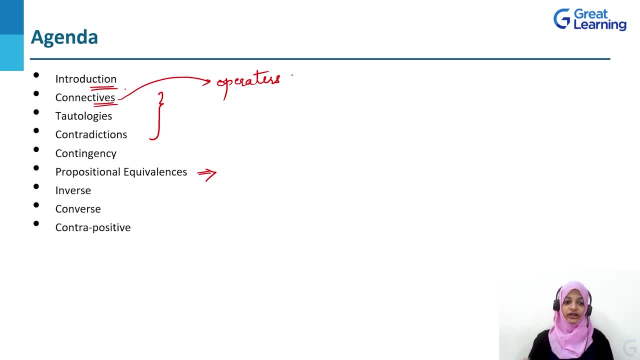 which are the two clauses which have to be, or do not have to be proved here. Lastly, we are going to look at inverse, converse and contrapositives and look at the relation between all of them. So let's quickly dive into this course. 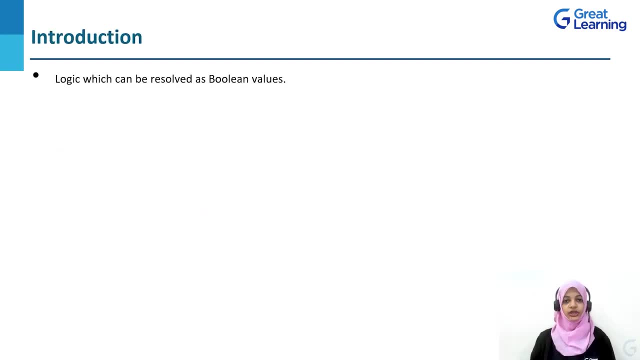 So let us first understand what propositional logic actually is in detail. Now. propositional logic is actually that logic which uses various sets or variables and then combines Boolean values with it. It's one of the simplest ways to understand what it actually is. Now, in any propositional logic, we 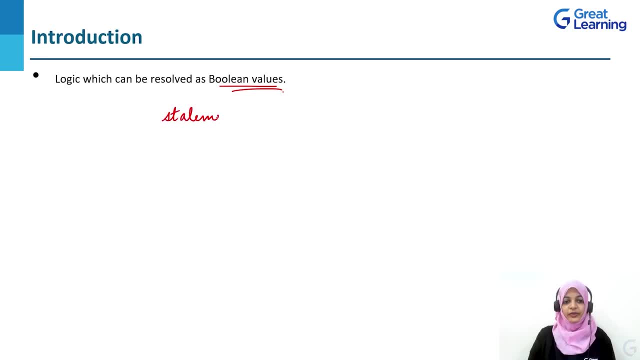 have something known as a statement. A statement is actually an equation of sorts which is always split up into three parts: We've got the variables, we've got the connectives and we've lastly got the result. So the variables are actually capital letters. 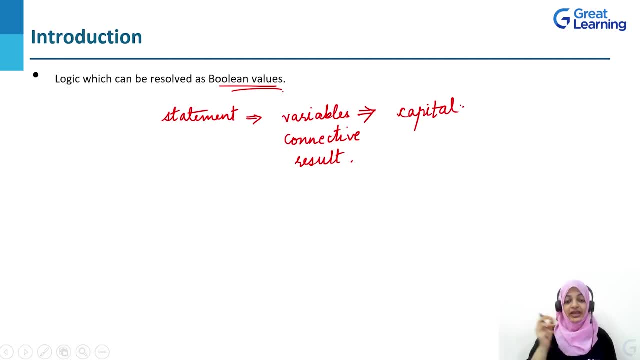 that actually represent the various components that might be a part of the statement. Next, we've got connectives, which act as the operators within this particular statement And, lastly, we've got the result, which can be provided in Boolean values. Now, as soon as we say Boolean values, it 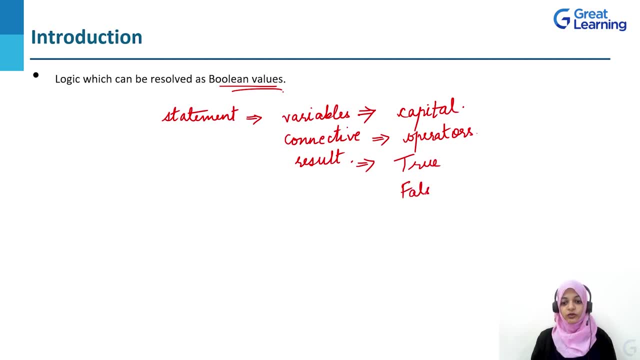 actually means that we've got true and false values, which we get as results here. So any statement that is a part of propositional logic is actually going to have some variables, connectives and a related result with it. Right Now, what are these variables? Variables- 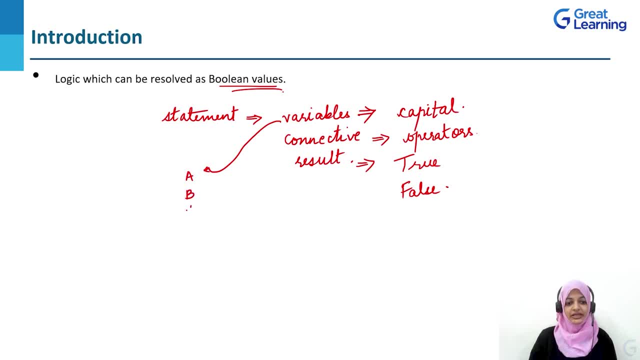 can be any capital letters, say A, B, C, D, etc. They might be statements in and of themselves, or they might just be true or false value. In any case, if they are actually connected to each other with the help of connectives, they will. 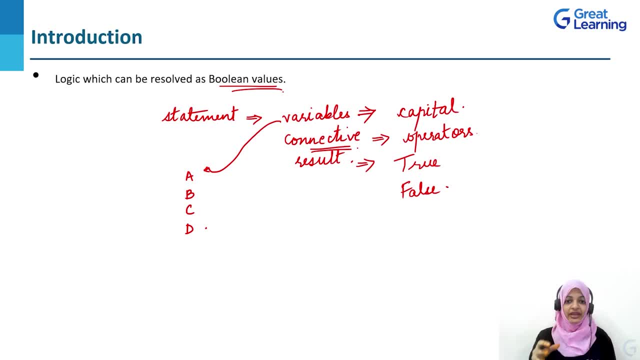 be known as variables. Sometimes, variables are actually complete statements in and of themselves. We'll be looking at examples of the same later on. The results that we receive will often be in the form of true and false, Since we are actually using propositional logic to 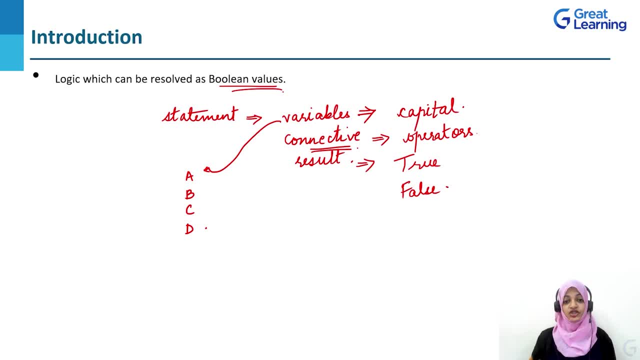 program machines. true and false are string values or words that may not be understood by them. So what we do is we change them into true Booleans, which means that true will be depicted by one and false will be depicted by zero. Thus, using this kind of a logic and this kind of a 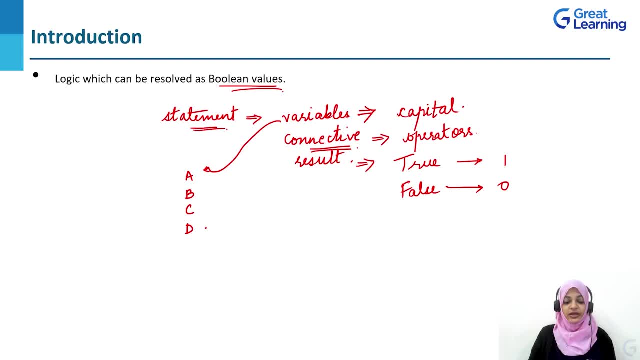 format. we are then able to create various statements, which might be a combination of various statements connected by some connective, and thereby program a given compiler or a machine to complete a certain task. Let us look at some examples of how propositional logic statements actually look like. 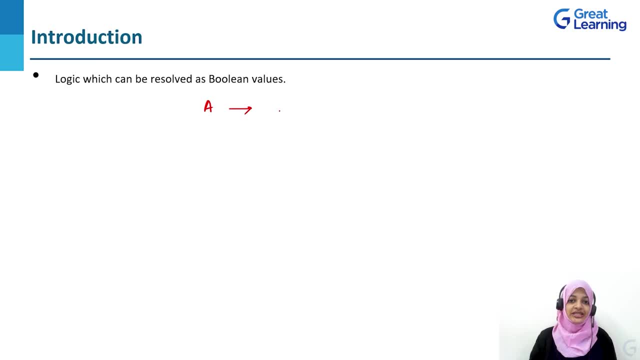 Say, we have a various table A, which actually stands for a statement: man is human. Now, if we think about it, man is a human because a male human is the only species or the only creature on earth who is called a man. Right, We don't call. 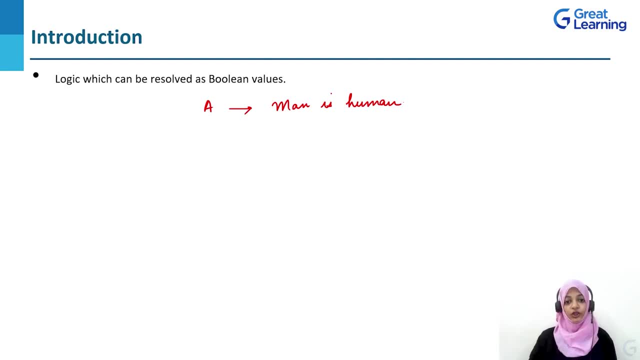 male animals or male plants as man. It's only human who is called a man if they are male. Right, So man is human- will give us a true value Here. I'll be writing one in order to denote that it is true. Let us take another. 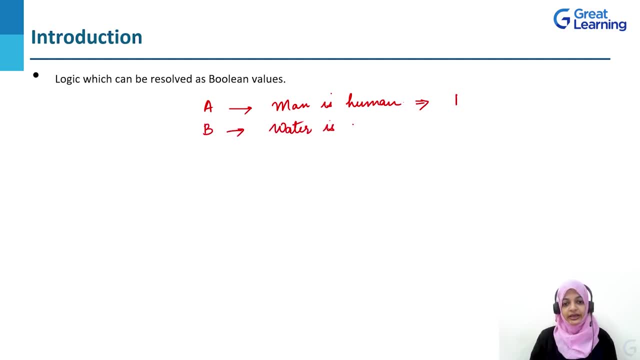 example, Water is chemical. This is also a true statement, right? Some of you might be confused. How is this true? Well, water is actually composed of two hydrogens and one oxygen, both of which are actually chemicals. So, yes, water is also a chemical. 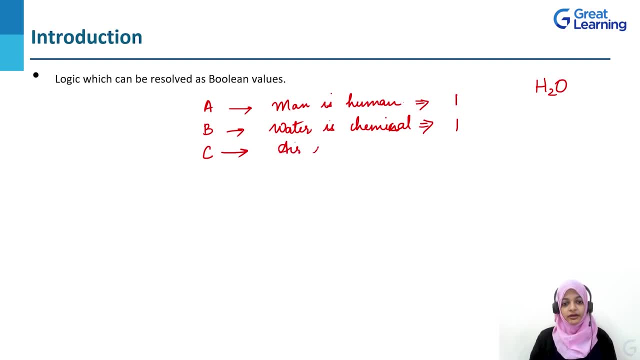 Let's take a third example: Air is fire. Is this particular statement true or false? Obviously this particular statement is false. Why is that? Because air does aid in fire burning, but air is not fire, Right? So this particular statement is actually false. So 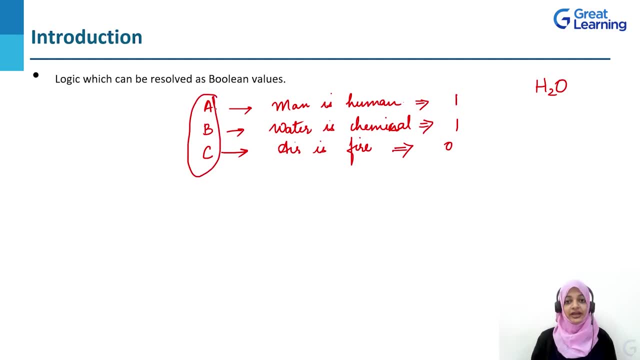 this is how our variables are actually created, and these variables can be combined with each other and utilized in combination with certain connectives. So let us quickly jump into seeing what connectives actually are. Next, let's look at connectives. As I've already stated, 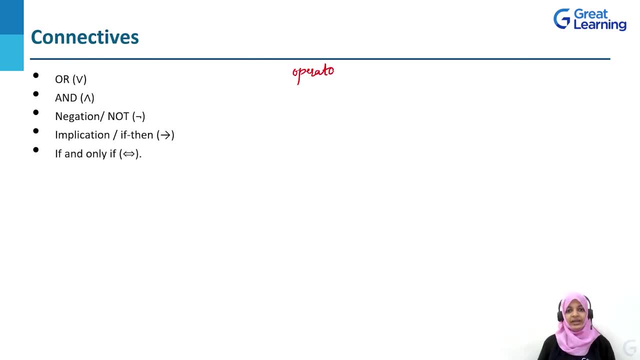 connectives work like operators. Now, as we already know, we've got various kinds of operators, namely addition, subtraction, multiplication. So what do these operators do? They basically take any two operators, such as, for example, 3 and 5, and perform an operation between them. 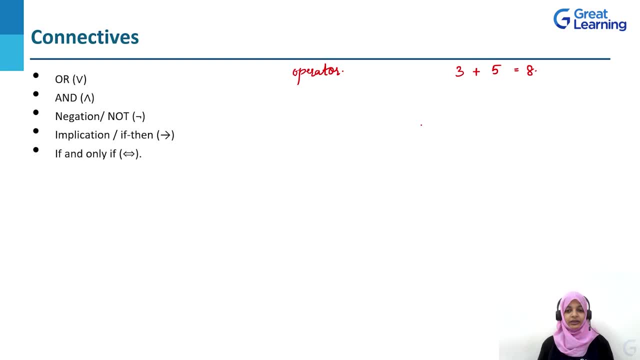 which then gives a result. In a similar manner, the connectives here also work with variables, So various variables are actually put in combination with one another and there is an operand or a connective between these various operations that actually gives us an equivalent result. 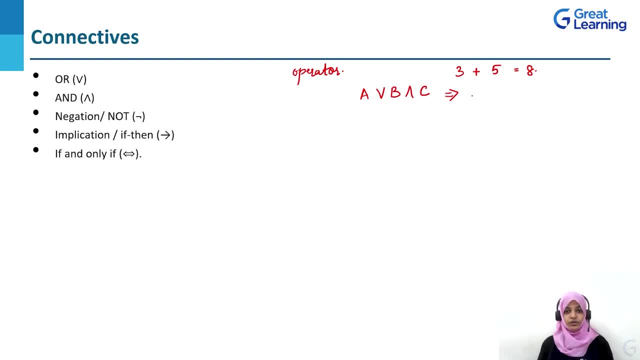 The result, as we already know, of this propositional logic will either be true or false, depending upon the variables and the connectives that we've combined them with. Let us first look at the OR operator or the OR connective. The OR connective has a truth table assigned. 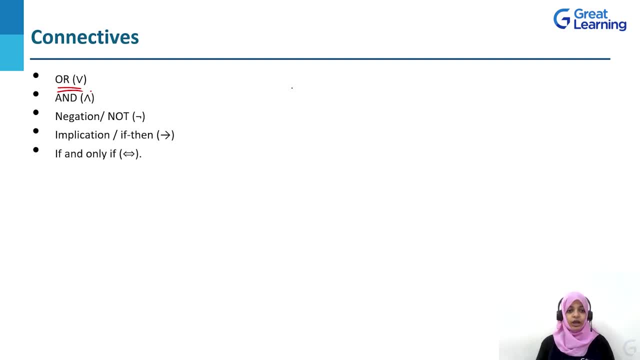 to it. A lot of you, after looking at the truth table, will actually connect this particular OR connective to the OR gate you might or might not have seen in Boolean logic. Now how does this OR work? Suppose we have two variables, A and B, The values. 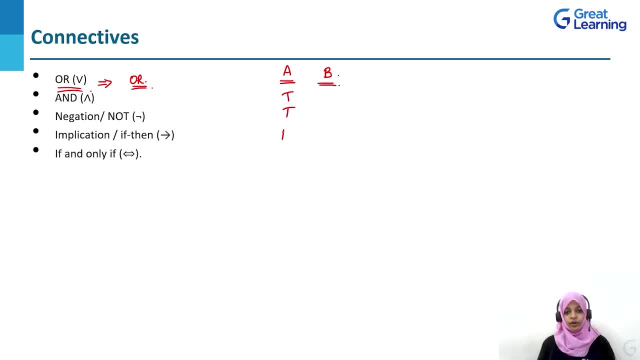 of these two variables can be true or false. Similarly, the value of variable B may be true or false In either cases. if we apply an OR connective between A and B, we end up getting true if both the values are true. true if any one of the value is true. 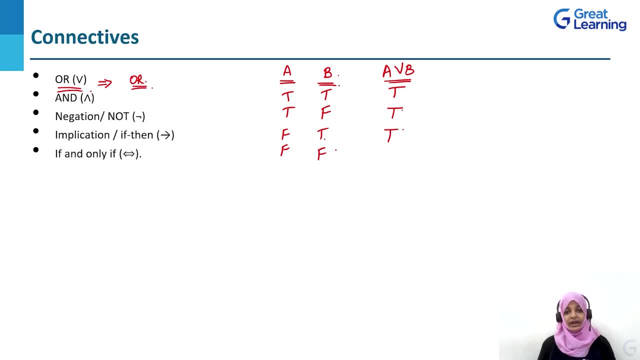 again: true if any one of the value given is true, and false if both the values are given as false. So from this we can assume that the OR gate is always going to give us a true value if any one variable is set to true. So if even 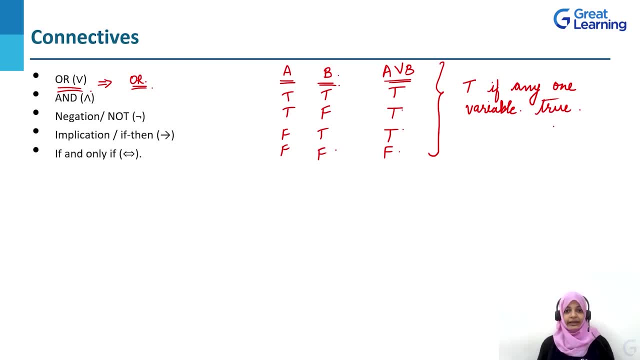 one variable is set to true, then our OR connective is going to give a true value at the end. What happens if none of the variables are set to true? then, as in the last case, we will get a false value. Let us take the exact same. 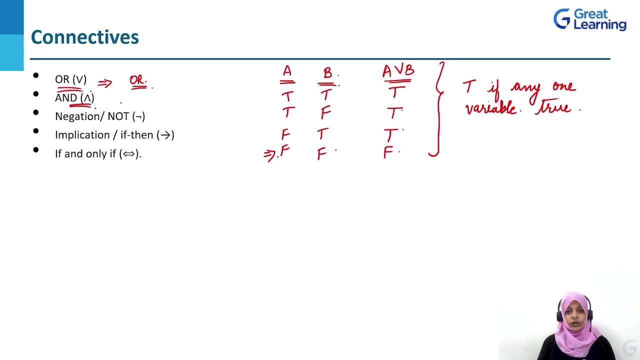 example and understand how the AND connective works. Again, the operation of the AND connective is similar to the Boolean AND gate. So if we have two variables, A and B, such that the values of A are true and false and similarly the values of B may also be true, 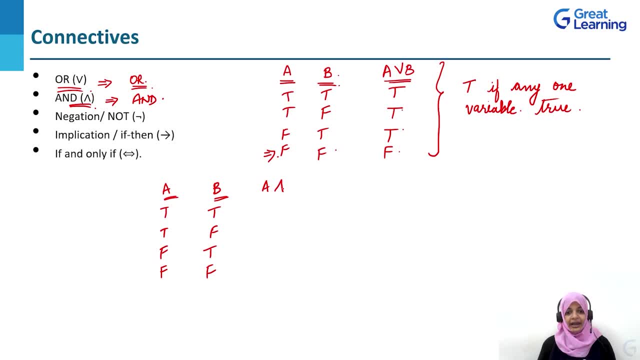 and false, then A and B will give us answers such that it will only give true if all the values are true or all the variables are set to true. So that means, since all the variables in the first case are set to true, we will get a true here for A and B. 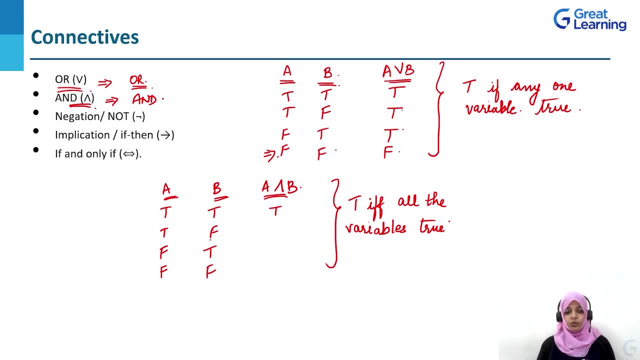 What happens for the rest of the values? since one of these or both of these are false, all of these will give a final result of false on actually utilizing the AND connective. So, as you can see, there is a difference between the OR and the AND connective. 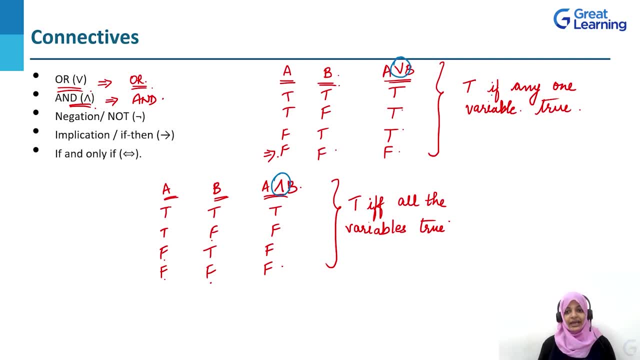 When it comes to the OR connective, we will say that if any one of the variables is true, then the final value will be true, whereas in the AND connective it will only be true if, and only if, all of the variables are set to true initially. 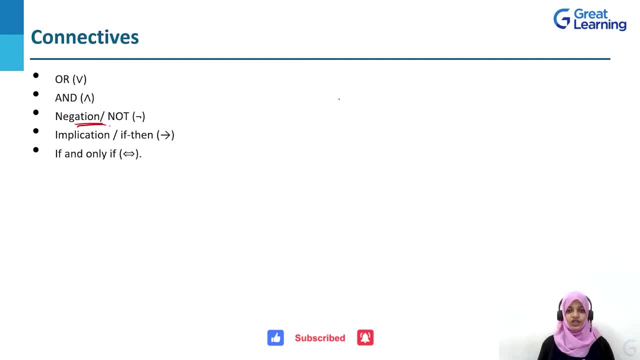 Next, let's look at the negation connective. So the negation connective is a unary operator. this means that instead of utilizing two or more variables, the negation connective only requires one variable. So if we have a variable whose possible values may be true, 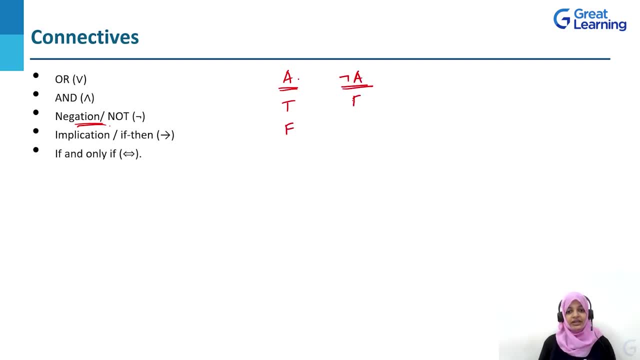 or false, then negation of this variable will give us the opposite answer. So if initially the value was true, then negation of A would give us false, and if initially the variable's value was false, then negation of that variable would give us true. Next we will look at: 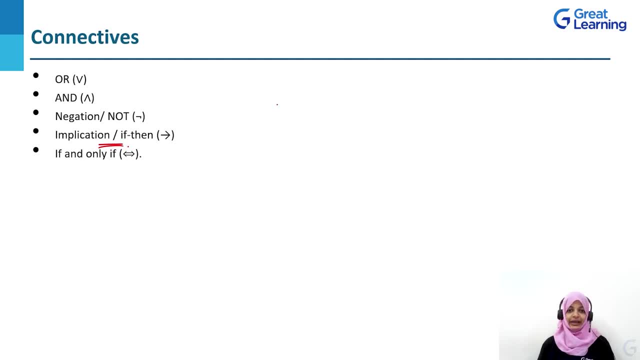 the IF, THEN or the implication connective. The implication connective actually says that if A variable is exactly existing, then we have a B variable. Let us look at the truth table, or the table as we were looking at. for the same, If we've got two variables, 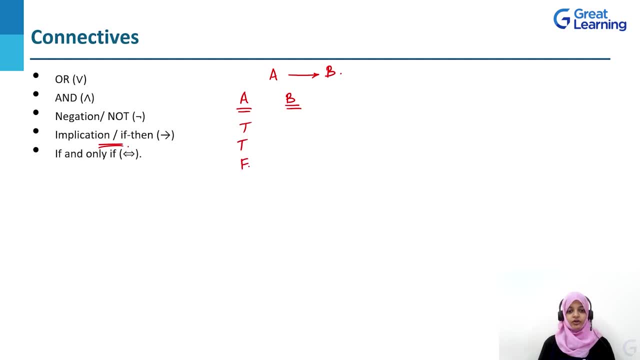 A and B, such that the values of A are true and false and the values of B may also be true and false. then A giving B will give us a true for the first condition, because if A exists, then B also exists. So here we'll get a true condition. 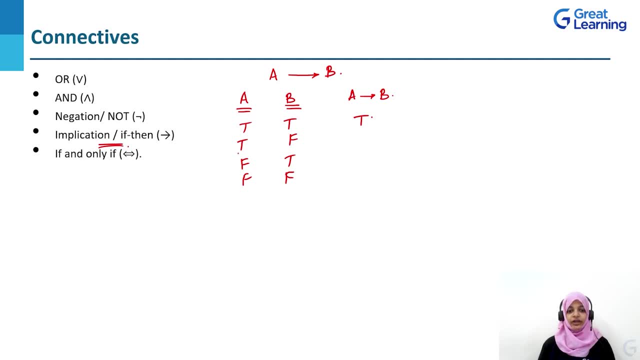 next, what if we've got: if A, then false. this doesn't really make any sense. if one condition exists, then the other should exist. this is the condition in the truth table that will not make any logical sense and hence will get a final value of false. next, if A is false. 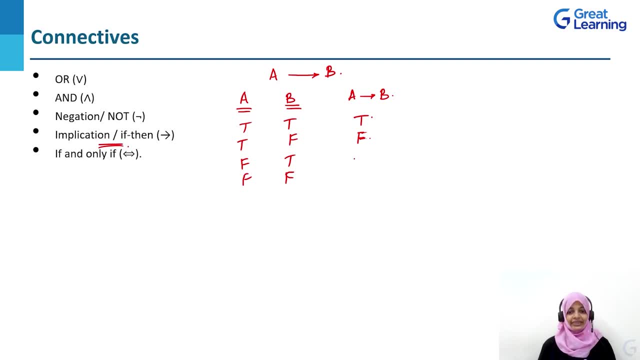 then there is a possibility that B will be true, and that is how, here too, we get A then B as true. lastly, if A is false, then B is false would be like a negation of the first condition given here. so again, this would be true. 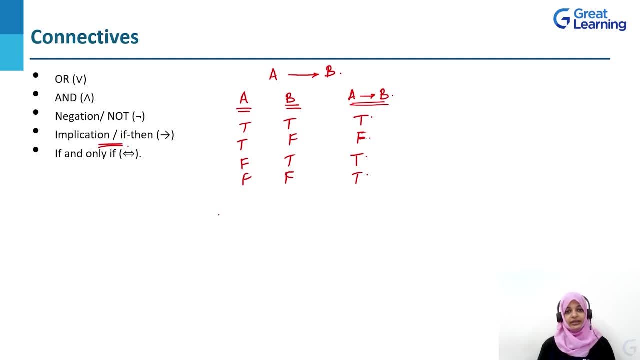 maybe this might confuse some of you. so let us look at this with an example. for example, if we've got variable A as sunny and variable B as not rainy, so if we're looking at the first condition here, then it is sunny and not rainy, so that would give us a true 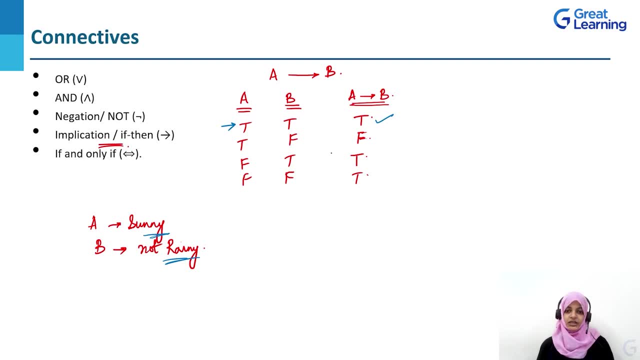 why do we consider a true here? let us consider true as a good day, right? so if it is sunny and not rainy, then we would consider it a good day, so we get a true value there. what if it is sunny and rainy? can you see that B is actually not rainy? 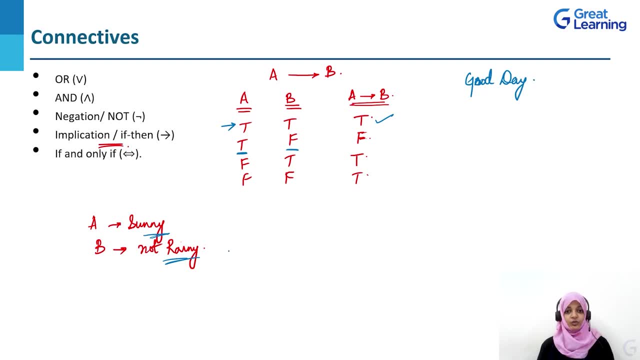 so true would mean that it is not rainy and false would mean that it is rainy. how could we have both sunny and rainy weather together? since this does not make any sense, we get our final value as false. let us look at the next pointer. here we've got. 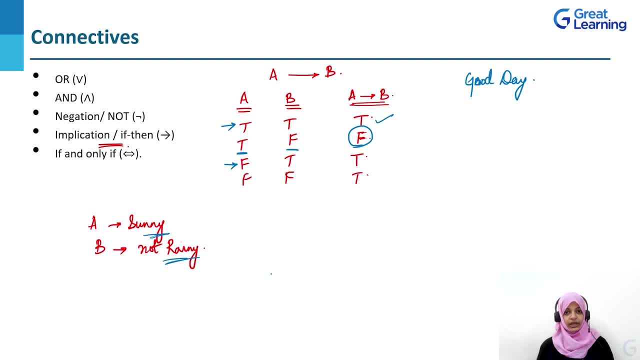 not sunny, and we've got true as not rainy. it might not be sunny and not rainy either, because it could just be a foggy day. was it a good day? yes, it's possible that it could be a good day. lastly, it is not sunny, but it is rainy. 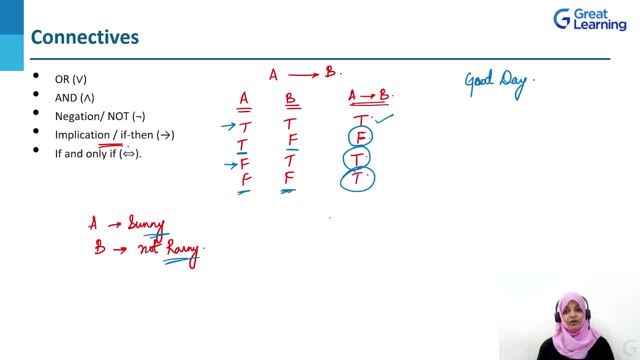 it might still be a good day if you are one to like rainy days. so, as you can see, logically, this is how the truth table will work. the truth table is going to give false only in one condition: if the hypothesis is true, but the condition that you get. 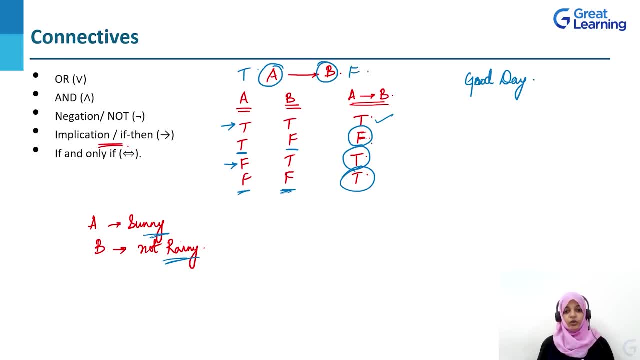 is false. only in this condition are you going to get a false value. in all other conditions, the implication connective is going to give us a true value. lastly, let's look at the if and only if connective. the if and only if connective is also. 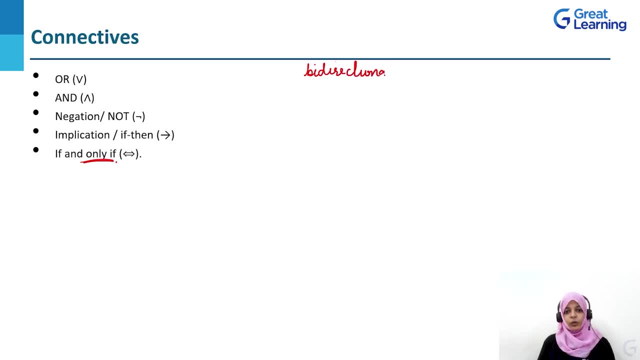 known as a bidirectional connective. now, what is this bidirectional connective mean? it means that it actually consists of two implications. so if we write a, if, and only if, b, it actually means that a implies b and also that b implies a. this means that a will exist. 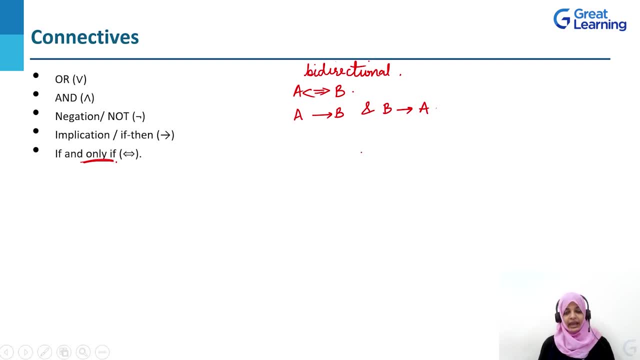 if b does, and b will be if a does. right. this is what it means. so when we look at the bidirectional connective, it actually gives us a scenario wherein the final answer will be true if, and only if, all the variables have the same value. this means: 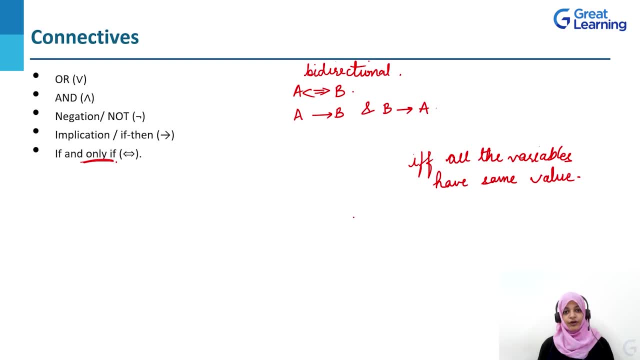 that, in actuality, you will only get true if all of the values of the variables involved in the equation are true or if all of the values of the variables involved in the equation is false. let us look at the truth table for the same say. we have a variable a. 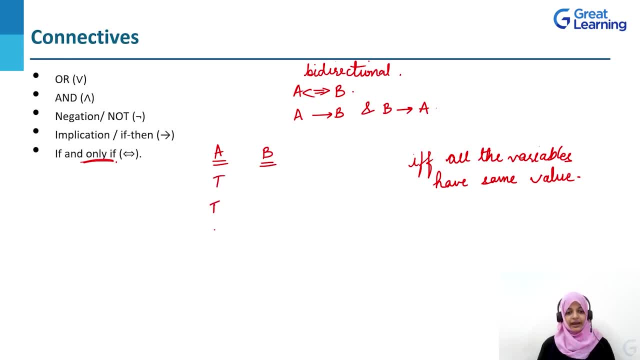 and a variable b, such that a may have values true and false and b may have values true and false, then a if, and only if, b will give true. if all of the values are same, that means for the first and the last case we would have true values. 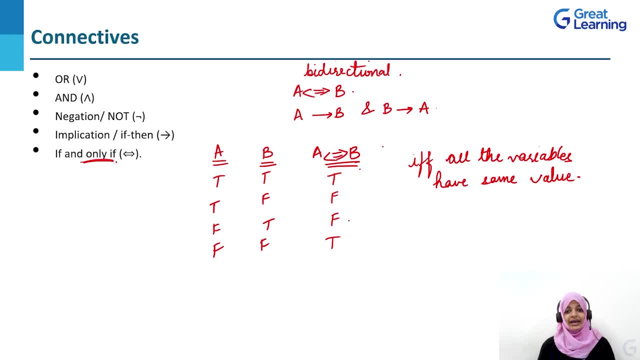 all the other cases would actually give us false. this is how our bidirectional connective, or the if and only if connective, works. next let us look at tautologies. so what is a tautology? a tautology is actually a special property of a propositional formula or propositional. 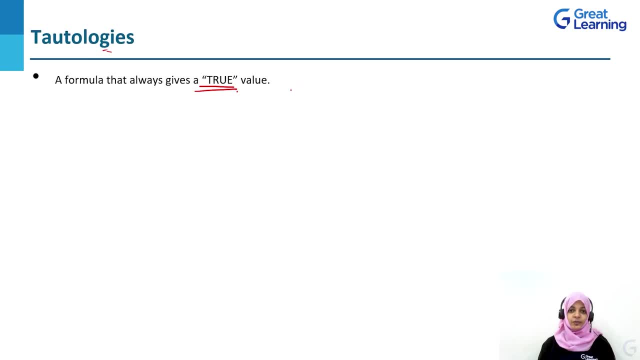 equation that gives us true, irrespective of what the values of the variables may be. keep in mind that it is the whole formula and not the values of the individual variables that we are talking about. let us look at an example of the same. suppose we have an example in such: 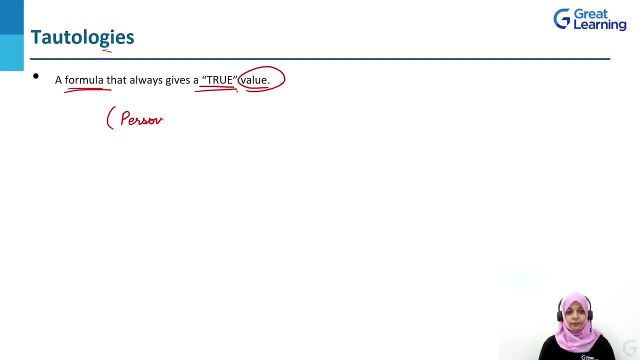 a manner such that a person and human has a good day, and good day implies happy. so what is this particular formula telling you here? this particular formula is just a way in which we can actually show a given tautology, if there is a person and this person. 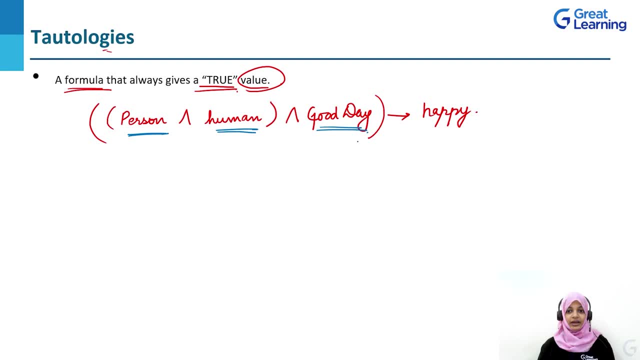 is human and this human has had a good day, there is a chance that this person would be happy. so, if it is a person and it is a human, can you see there is an and. so if it is true and this person has had a good day, then this person. 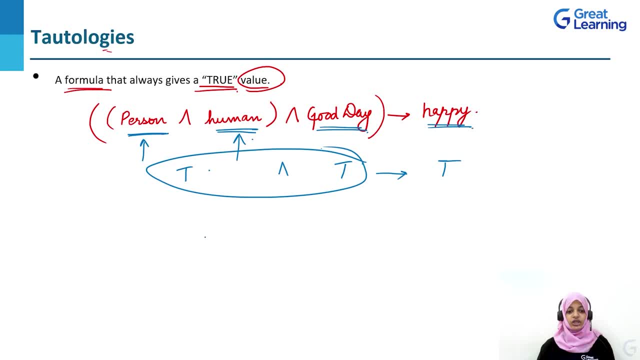 would be happy. so, as you can see, this tautology is always going to be true, or this particular formula is always going to give you a true value at the end. let us look at another example to actually understand this completely, because here there might be some lacuna. 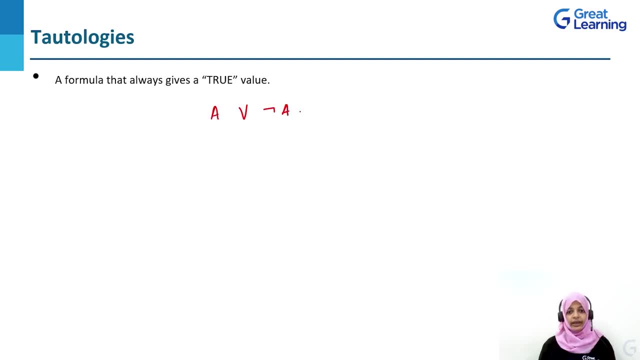 let us look at the formula a or not a in order to better understand what these values are. let us draw the truth table for the same: a and not a. so a can have values, true and false, and not a will have the opposite values, which are negations of. 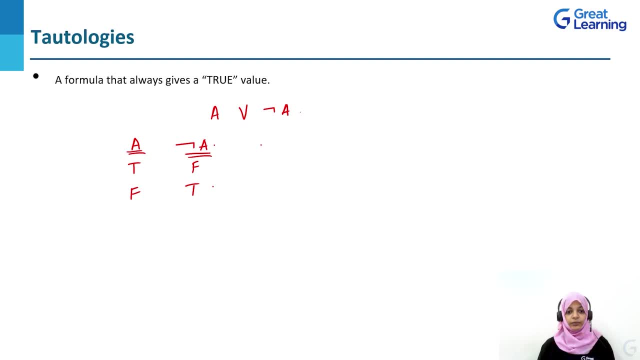 the original values. so we would get false and true here. if we take the or operation of true with false, we get a true, and if we take the or operation or or connective with false and true, we again get true. so this means that irrespective of what the 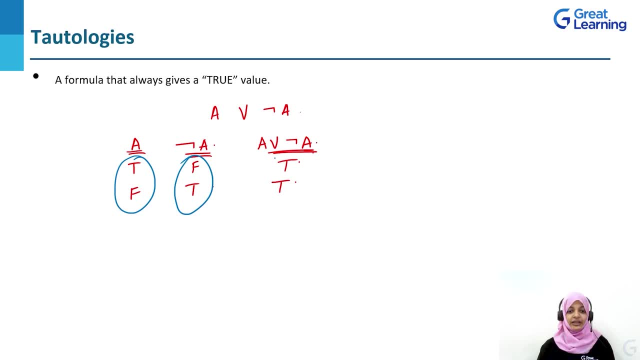 initial values of the variables were the final values that we have received are always true. this is what a tautology is: any value or any propositional equation that in the end, irrespective of the variables, always gives a true value, is known as a tautology. 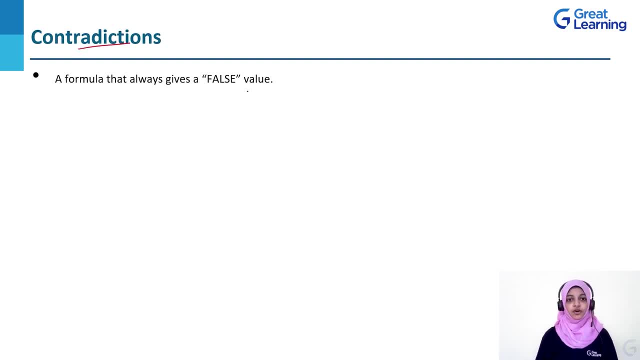 next, let us look into the other concept that is a part of propositional logic, namely contradiction. now, contradiction is something that contains a combination of variables, that is, propositional variables- and connectives, in such a manner that this particular equation is always going to give us a value of false. 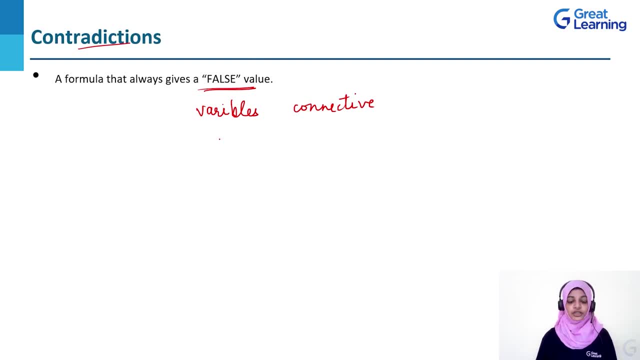 one of the simplest methods of understanding a contradiction is actually carrying out a formula of this type. say, for example, we have an event, a, such that it forms a formula a and not a. let us try to understand this particular formula. what does this mean? so, if a, 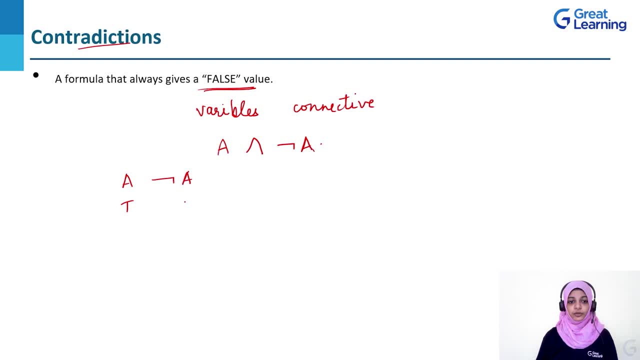 is true, then not a would be false, right, whereas if a were false, not a would be true in any case. a with not a occurring in an and connective will actually give us false in both cases. so it does not matter what the values of the variables are. the final. 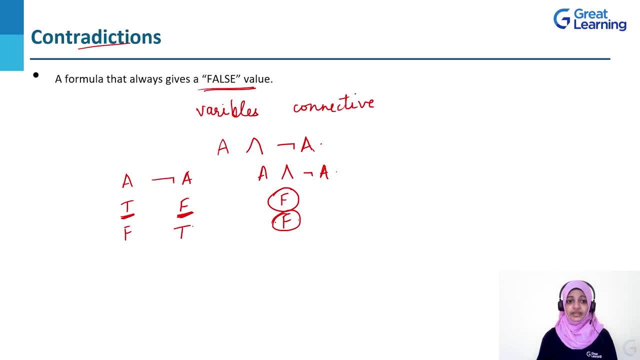 answer will always give us a false value. this is what a contradiction is. let us look at this with an example. say, a is an event such that a person is happy. thus, a dash or negation of a will be an event where the person is not happy. 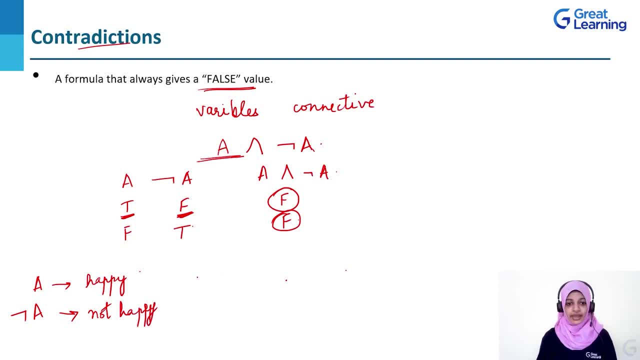 when we take an example of a and not a, it actually means that the person is supposed to be happy as well as not happy at the exact same time, because that is how the and connective is defined. now, this is not possible. a person can't be both happy. 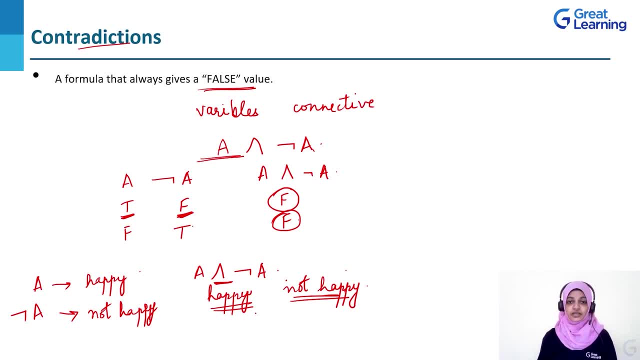 and not happy at the same time. this means that this is a contradiction and the value of this particular formula will always be false. this is what a contradiction states. next, let us look at what a contingency is. a contingency is such a formula that can give us a combination. 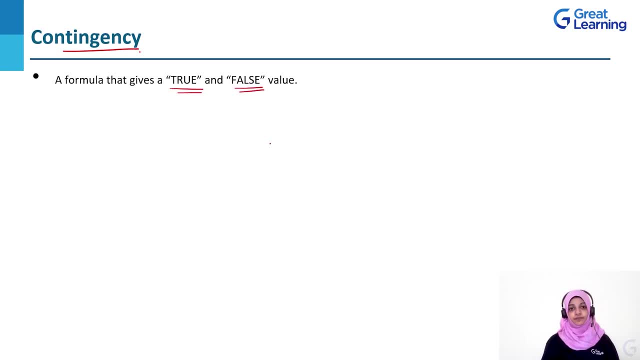 of true and false values as its results. let us take a quick example to understand exactly how this works. suppose we have a formula such that b and a or not b. let us create a truth table in order to understand exactly how this executes. say we have b and a. 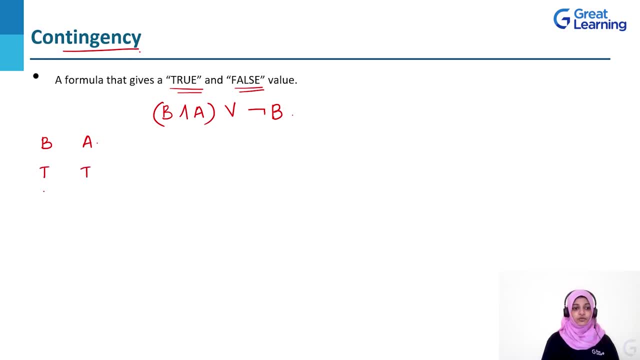 two variables which may have true values, true and false values, false and true values and false and false values. if we carry out the formation of b and a, we end up getting true, false, false and false. next, let us look at what not b will be every time their b value. 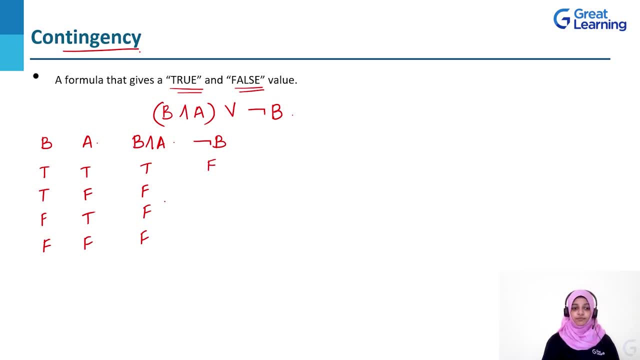 is true, the not b value will be false. every time the b value is false, the not b value will be true. thus, not b will have values: false, false and true, true. next, creating an or operation of b and a with not b. what we get is true. 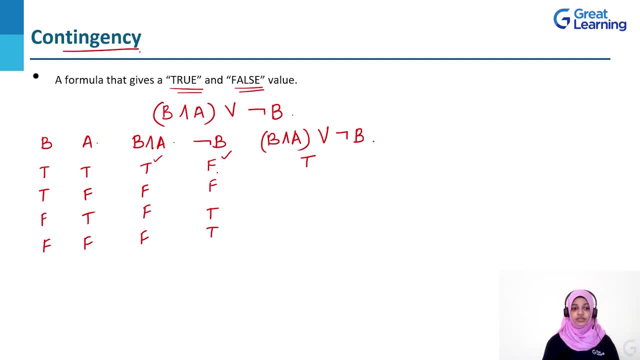 because these two values are as true and false. next, false and false will give us a false, false and true will give us a true, and false and true will give us another true. thus we have seen that the values may either be true in nature or they may be. 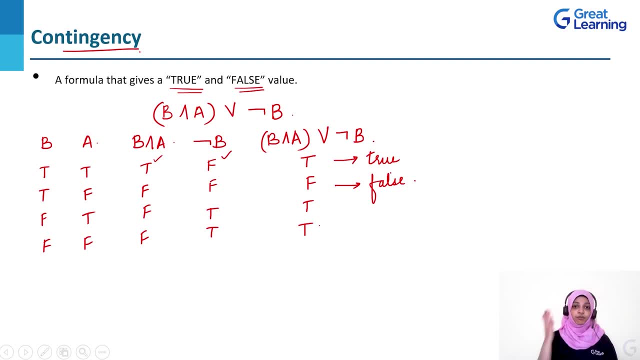 false in nature. thus, there is a combination of both true and false values. this is different from both tautologies and contradictions, because tautologies were where each and every one of the values were true and contradiction had all values as false. contingency is one where some values would be true and others. 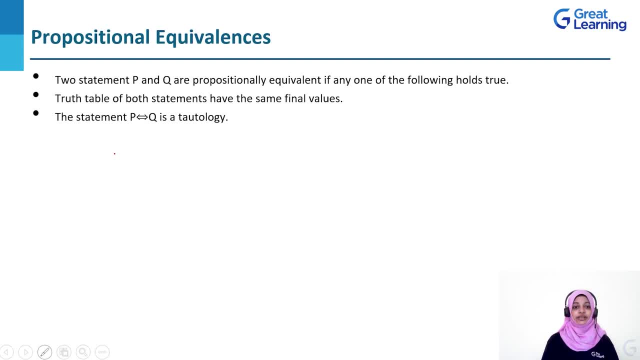 would be false. next, let us look at propositional equivalence. propositional equivalence is actually a statement that helps us define when two propositional statements are equal to each other. these formulae can actually be shown to be equal to each other in two cases. first, if the truth table of both, 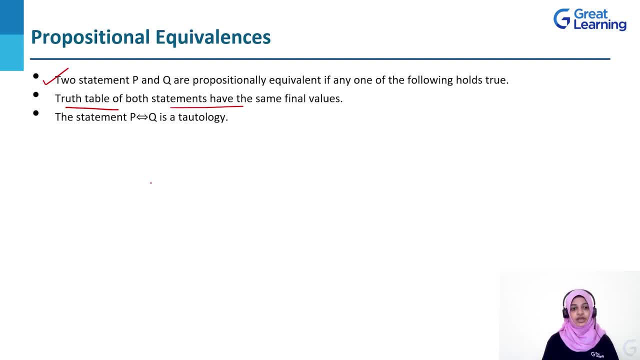 of the statements have the exact same final values and secondly, if the two statements p and q are a tautology, when the bidirectional operation is performed on them. let us take an example to better understand how this can actually be done for the purpose of this particular example. 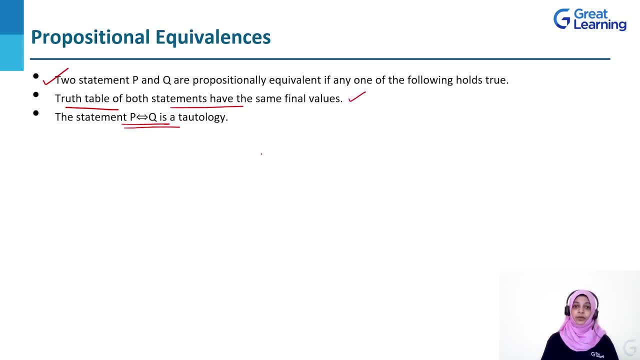 we will actually be proving both the truth table method as well as the bidirectional connective method. consider two statements, namely p and q, such that they are defined as a and b whole under negation, and a negation or b negation. so these are our two statements. 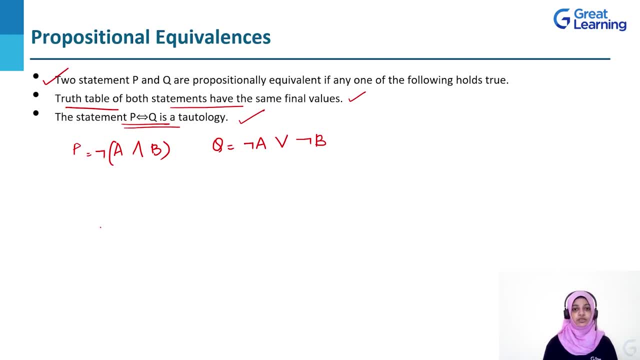 we need to prove that these two statements are equivalent to each other. let us try the first case wherein we are actually going to prove that these two statements are equal to each other using a truth table. say, we take a and b, such that a is equal to. 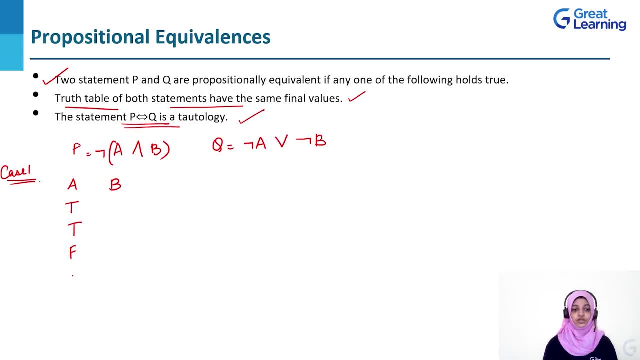 true or true, or false or false. similarly, let b have possible values of true, false, true and false. if we take the operation a and b, we would ideally get the result true, false, false and false. let us preserve this result for some time. next let us see what not. 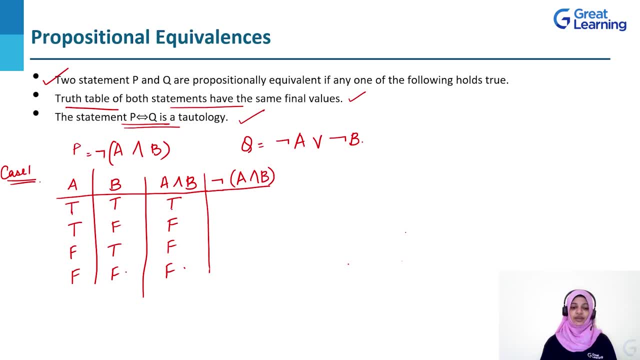 of this particular column would be so wherever there was initially true, we would now get false. so we've got false, true, true and true. next let us look at the truth table. for the statement q, we've got not a and not b initially. since a was t, we will now consider not. 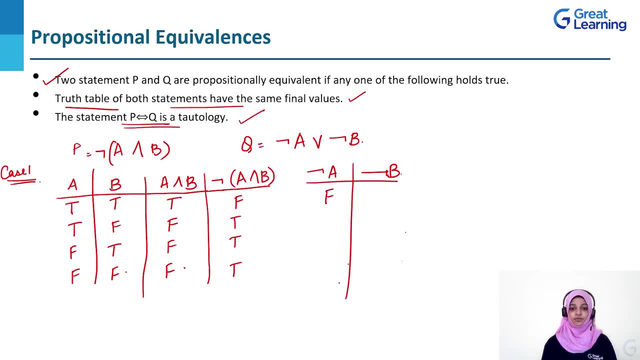 a to be false. thus, a will have possible values of false, false, true and true. on the other hand, not b will similarly have values of false, true, false and true. taking the last operation, which is not a or not b, we get a final answer of false, true, true. 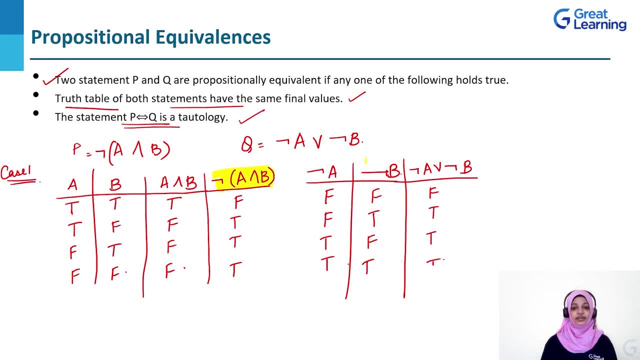 and true. observe the final values in the columns given here. as you can see, all of the final values are the same. this means that we've got false with three trues for both of these final values. this implies that these two statements, p and q, are equivalent to each other. 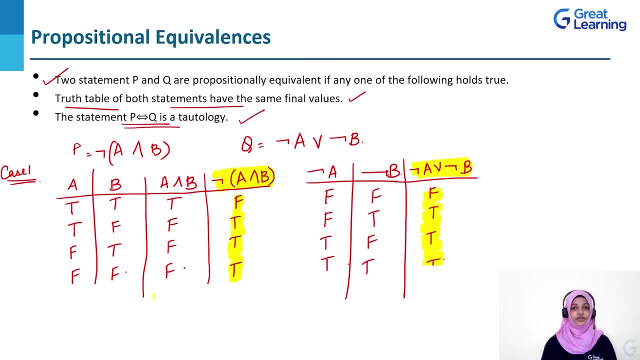 since their truth tables are both equivalent to each other. next, let us try to prove the second part of this particular propositional equivalence. we can also say that two statements are equivalent to each other if the two statements in the biconditional connective are actually. 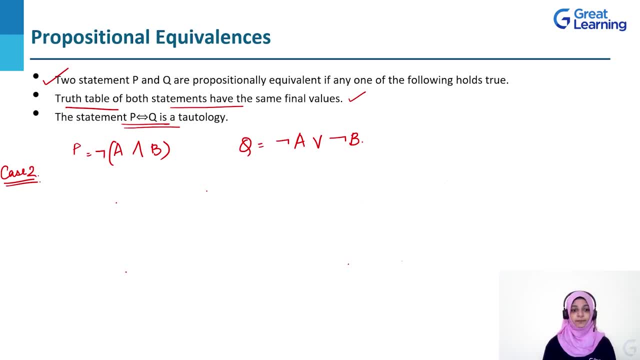 forming a tautology. so let us look into how it happens. if we've got a and b such that a has a possible value of true, true, false and false, and b has a possible value of true, false, true, false, then, as we've already seen in the truth table earlier, 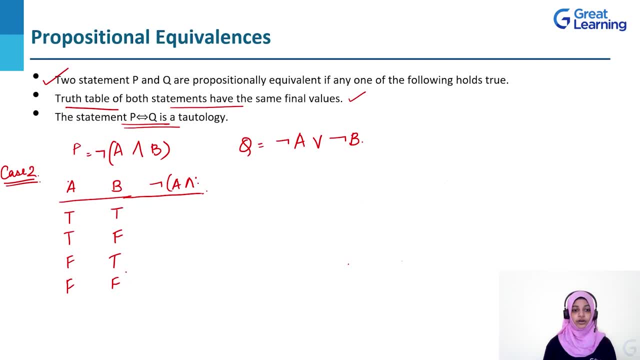 not of a or b will actually provide us with false, true, true, true. similarly, as we've already seen in the initial truth table, not a or not b will provide us with a truth table of false, true, true, true. let us take the bidirectional connective, that is, if and only 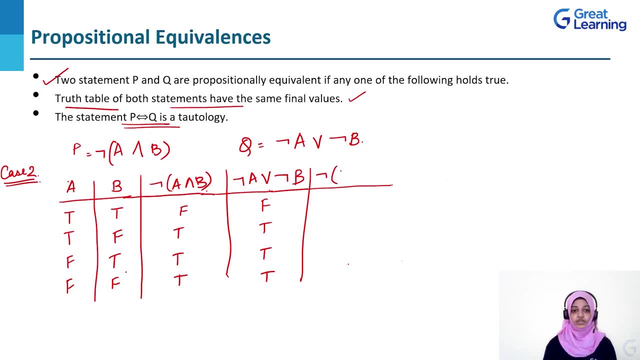 if, here of the two given columns, not of a or b, with if and only if connective, along with not a or not b. now, as per the if and only if, connective, if and only if, gives true if the two values that are interacting with each other. 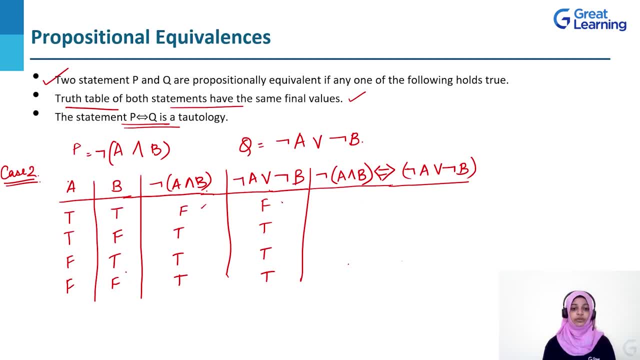 are of the same type. so here we've got false with false. these two values are of the same type. as a result, our bidirectional connective will give a value of true. next we've got true with true. again: two values interacting with each other and of the same type. 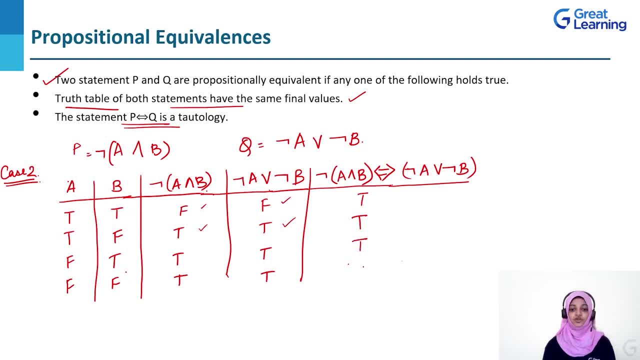 so we'll have the value true, similarly, true and true. as we can see, all of the values here are giving a true, irrespective of what the initial values of the operators were. this is what a tautology is, as we've already seen previously: a tautology. 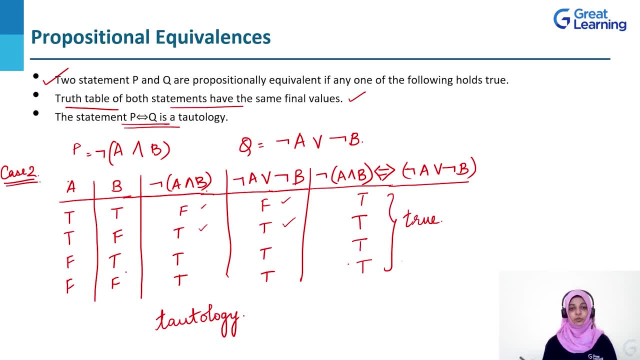 is that particular formula which actually provides us with true, irrespective of what the inputs might be. so here we've proven, using both the tautology or the bidirectional method, as well as the truth table method, that the two statements given in the example are actually equivalent to each other. 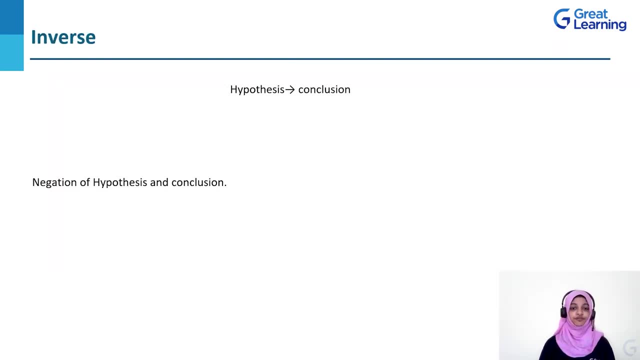 next, let's come on to the first of three connected topics, namely inverse. inverse is actually based upon our conditional connective, which is the arrow connective, or it's also known as the if- then connective. now, the if- then connective is actually one which is split up into two separate. 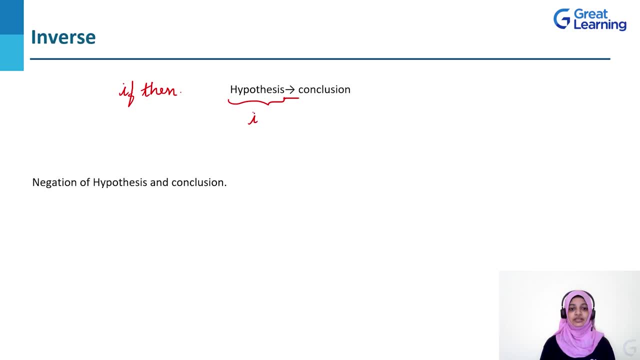 portions. we've got the hypothesis, that is the if statement, and the conclusion, which is the then part. if the hypothesis is true, then the conclusion also holds. that is what is the explanation of this. now, what is inverse? inverse is the negation of both the hypothesis and the conclusion. 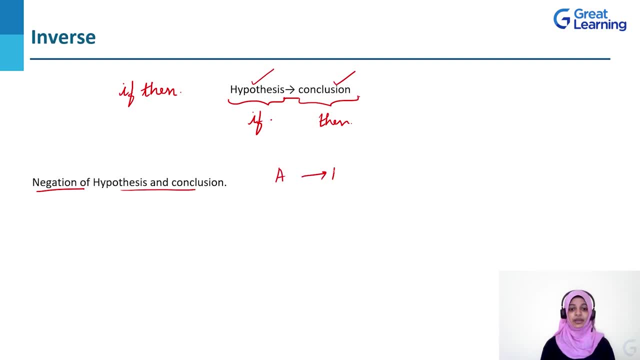 thus we have a statement such that a gives b, then inverse of a gives b will be not a gives not b. let us understand this with a practical example. suppose a is a statement stating sleep well and b is a statement fresh. this means that a gives b actually means. 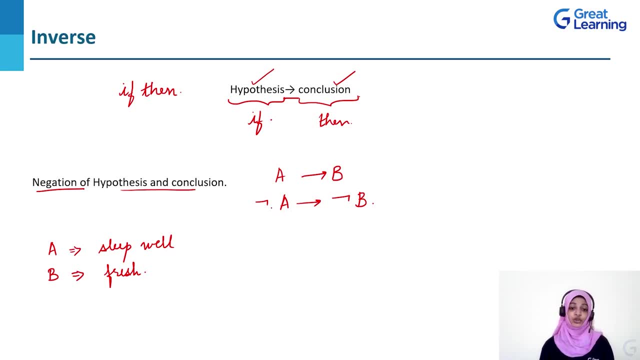 if you sleep well, you will be fresh. so not a gives, not b implies that if you don't sleep well, then you will not be fresh. this is how an inverse works. next let's look at converse. converse, again, is actually dependent upon the if, then connective. 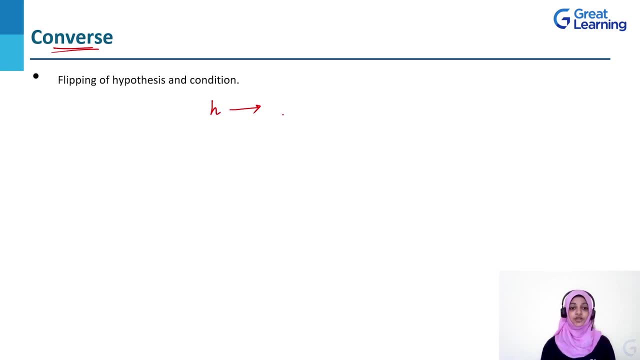 we already know that the if then connective has to two parts to it: the hypothesis which i am denoting by the h and the conclusion which i am denoting here by a, c. what is the converse of this particular if then conditions? here the converse would be: 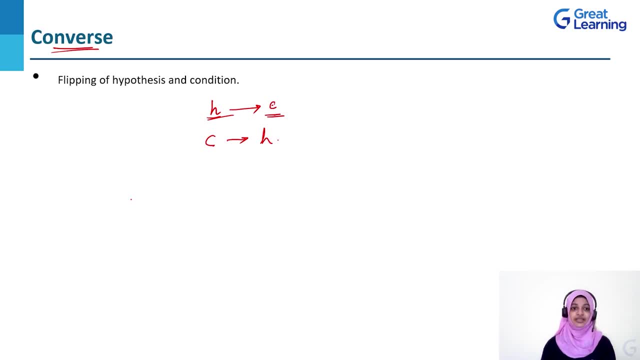 c, then h. this means that the converse flips the position of the hypothesis and the condition. what the converse helps with is actually in proving the bi-directional connective. so if in any given statement the actual hypothesis and its condition is true as well as the converse of that hypothesis, 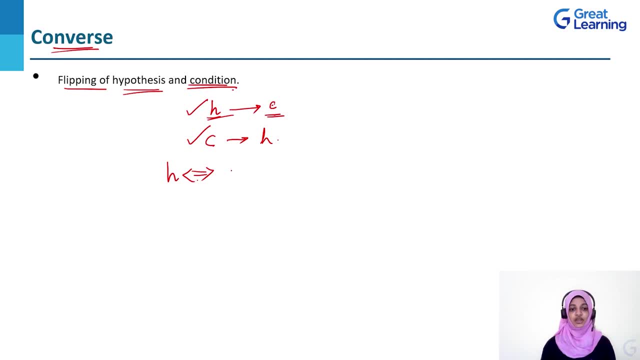 and condition is true, then we can say that h if, and only if, c. let us understand this with an example. let a be an event such that we are sleeping well. let b be an event of being fresh. if we take a gives b. this means that if we sleep well, 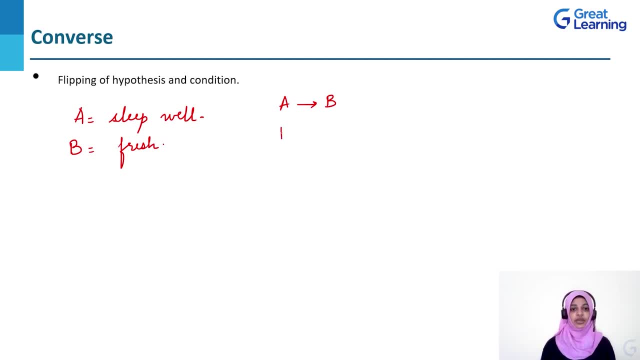 we will be fresh. the converse of this would be b giving a meaning: if we are fresh, we have slept well. so this means that we are actually flipping our hypothesis and condition in order to get a completely new, if then statement. lastly, let us look at the 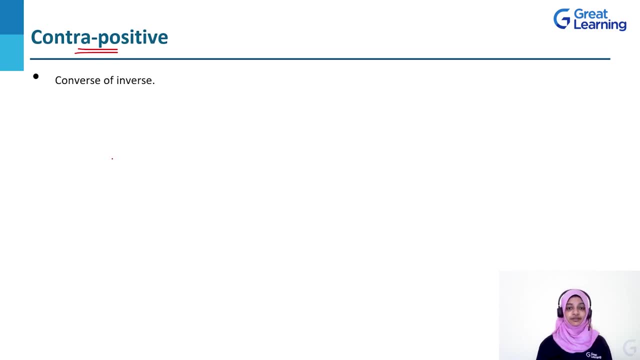 contrapositive. the contrapositive is actually defined as the converse of the inverse of any of the if then statements. so this means if we have an if then statement of the form, if a then b, then the first thing we have to do is take the negation of this, namely 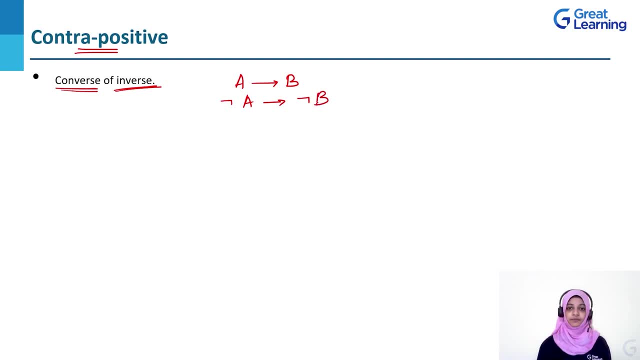 not a, then not b, and next we need to create the converse of it. that means we will be taking not b, then not a, so a giving b is actually converted into not b giving not a as per contrapositive. let us understand this further with a concrete example. let us 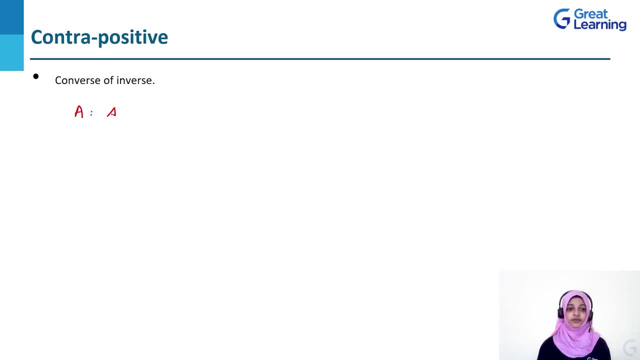 consider an event a such that we have slept well. let b be the event of being fresh. if we consider a giving b, then this means that we have slept well and because of that we are fresh. let us take the inverse of this, not a giving, not b. 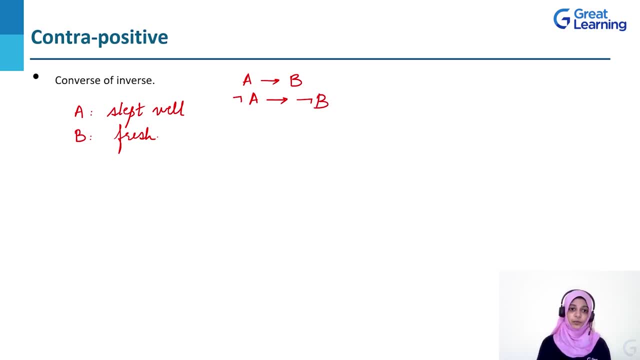 this implies that if we have not slept well, then we will not be fresh. lastly, let us create the converse of this: not b giving, not a. this means that if we are not fresh, we must not have slept well. this is how, in any case, we are able to convert. 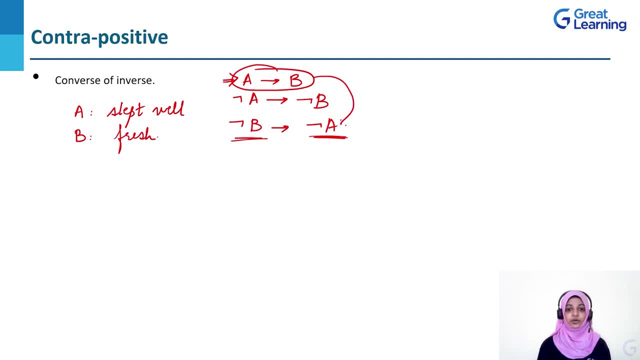 a given hypothesis and condition statement into its contrapositive. so let us quickly summarize what we have studied till now in this course. so first we looked at the various types of counting techniques. we saw that we had a sum and product rule, a pigeon hole principle and some forms of permutations and 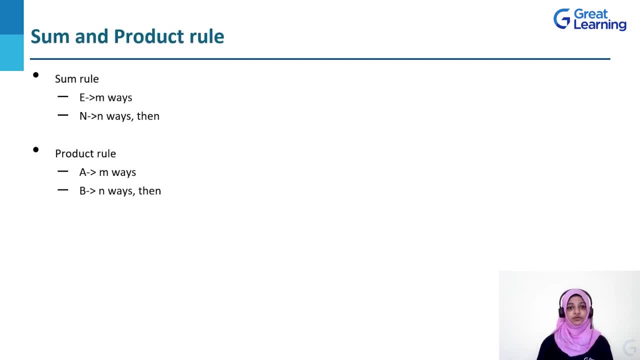 combinations. so the sum and product rule helped us identify how to convert. two non connected events could actually be carried out in tandem with each other. now, when i say in tandem with each other, we didn't actually mean that they were related to one another, we just meant 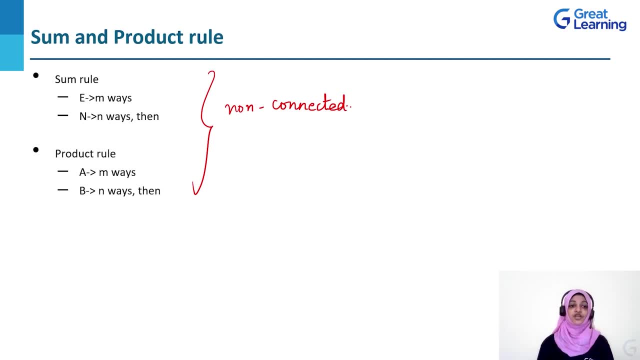 that there were ways in which they could be done right. so the sum rule stated that if we have an event e and an event n that can actually be independently run in m and n ways respectively, then the sum rule states the number of ways in which we can carry out. 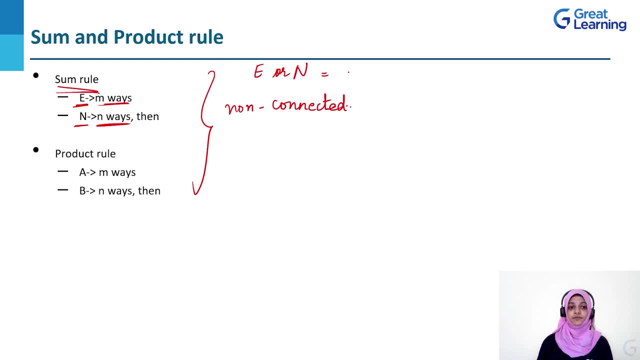 event e or event n then becomes a sum of both the number of ways which are there. similarly, the product rule stated that if we have two events not connected with each other, a and b, then the number of ways in which a and b can actually be executed. 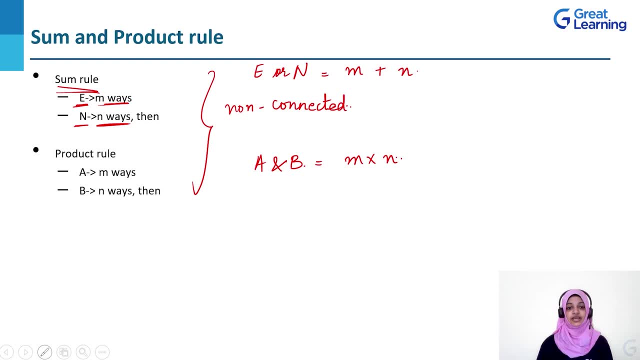 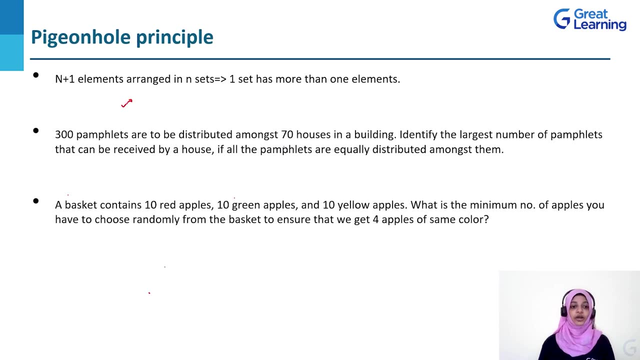 is a product of the individual number of ways in which the event can actually be executed. next we saw the pigeon hole principle, where we actually understood how apportionment can be carried out. we also saw that these particular examples can be solved in a logical as well as. 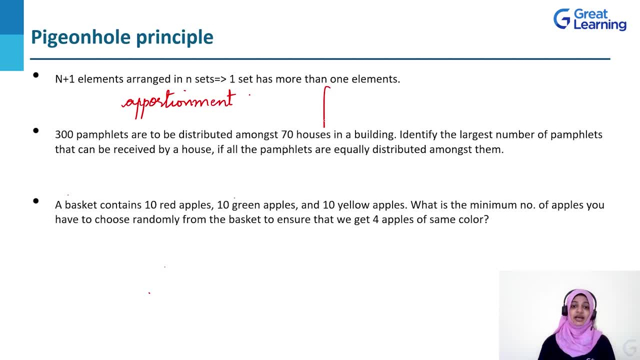 a formula, wise manner. the formula is that we take all of the number of elements or the resources that we actually require to apportion and we divide them by the number of containers that we need to apportion them in. whatever we get as the value here, a seal will have to be taken. 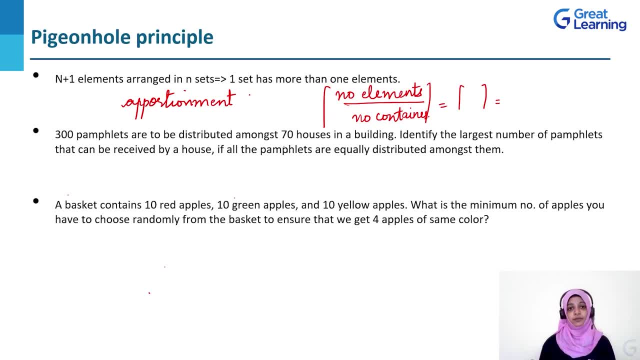 of the same, the seal value will be the smallest number, which is larger than the value that comes up within this open ended bracket. that value will be the largest number that can be contained within any given container if a fair distribution has been carried out within the apportionment. we saw two. 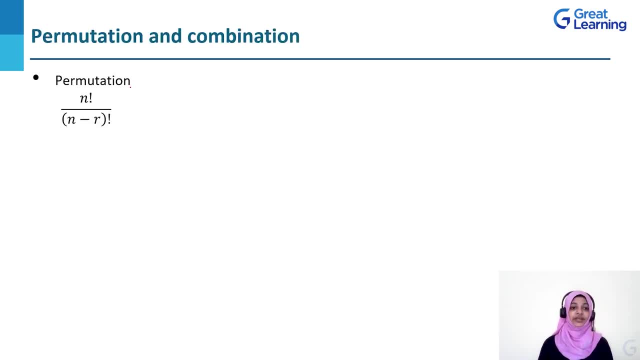 examples of the same. next, we went on to see how we can carry out arrangement of any set of values within a given set of range. so if we have a certain set of resources and we need to pick out a certain set of those resources and arrange them in a particular manner, that 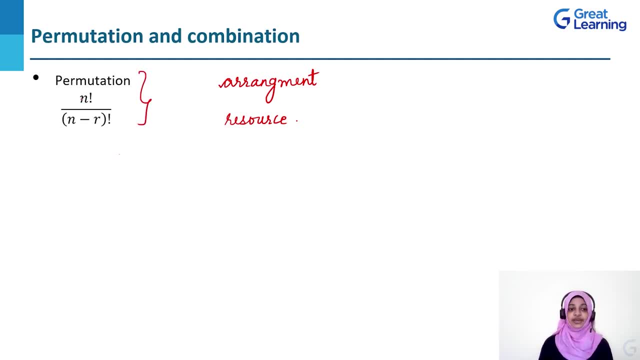 could be done via permutation. the formula of permutation is n factorial upon n minus r factorial, and permutation is often denoted by npr. we also saw an example of how permutation could be used to determine the exact number of possible arrangements in a given scenario. next, we also saw combination. 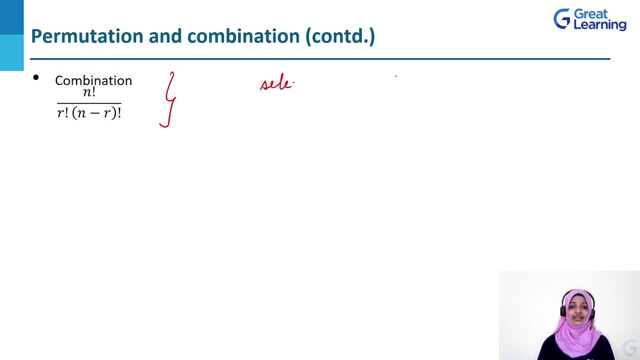 wherein combination is a method by which we can select a particular number of resources from a given set of resources. the way in which combination works is that it only allows us to select elements. we are not allowed to arrange them as we did in permutations. the formula for combination is: 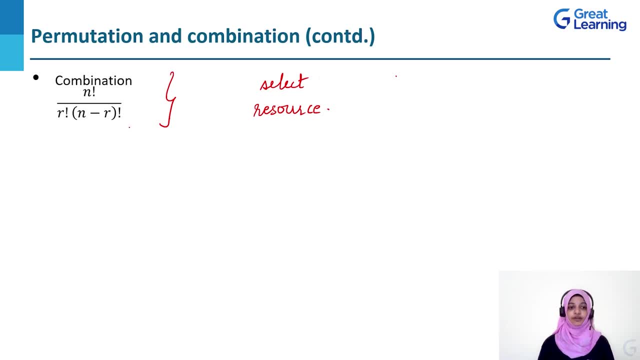 n factorial upon r factorial into n minus r. factorial combination is also denoted by ncr. we also saw a practical implementation of combination in binomial theorem, where we were actually able to find out what x plus y raised to 4 would look like. next we went on to propositional. 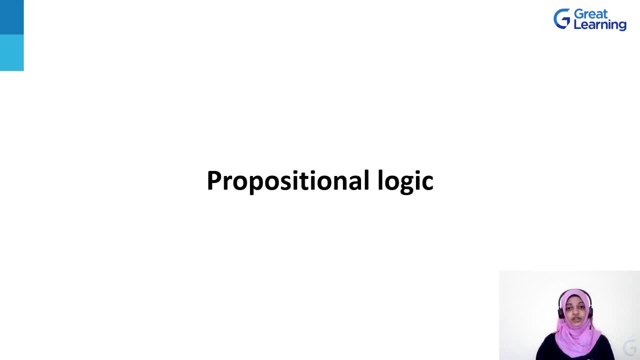 logic which, as we know, is a very large part of how machines are taught to learn themselves. propositional logic is actually a combination of set theory and boolean algebra, wherein it helps us exactly understand how statements interact with each other and provide values in boolean forms we understood. 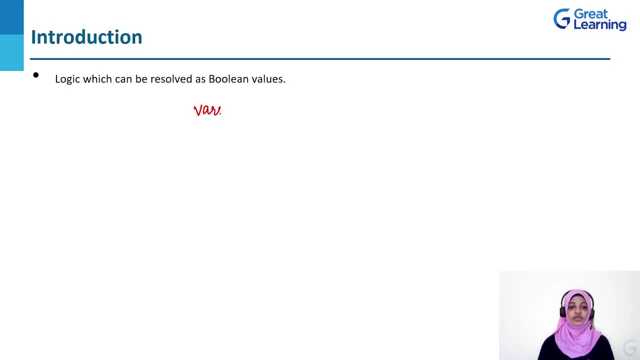 what propositional logic was. we understood what the components of propositional logic were, namely the propositional variable, the connectives and the actual boolean results. next we saw various types of connectives, namely or and not if, then and if and only if. we also saw how they could be used. 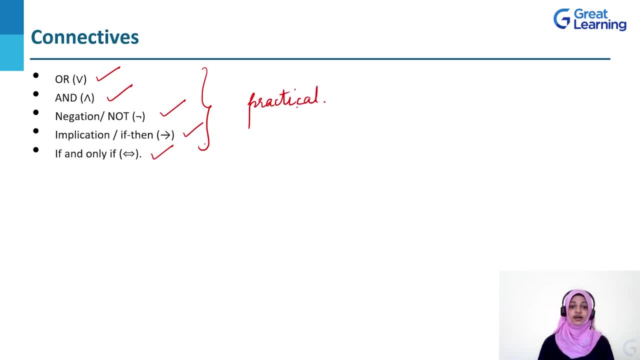 in various practical scenarios or using various practical statements. next, we understood the three types of formulae that we have within propositional logic. the first was tautology, which says that the formula is always going to give you a true value. next, we saw contradictions, which are formulae. 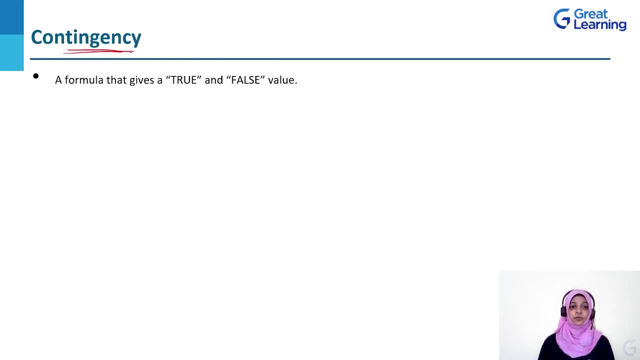 that always give a false value. next and lastly, we saw contingency, which were formulas that might give both true as well as false values. we have seen examples of each of these, with their respective truth tables. next, we saw an example of propositional equivalence here. in propositional equivalence, 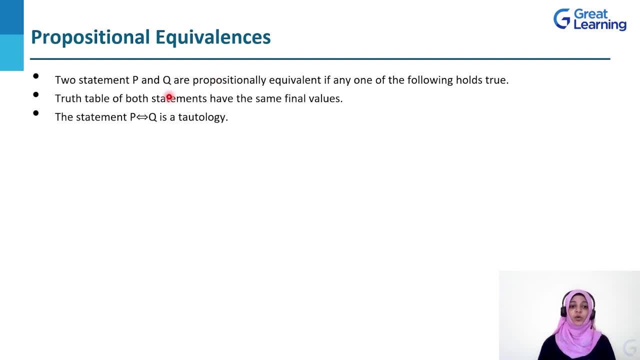 we were able to exactly understand under what condition are two statements going to be equal to each other. thus, we understood that two statements would be equal to each other if either their truth tables were equal to each other or if putting the two statements into a bidirectional 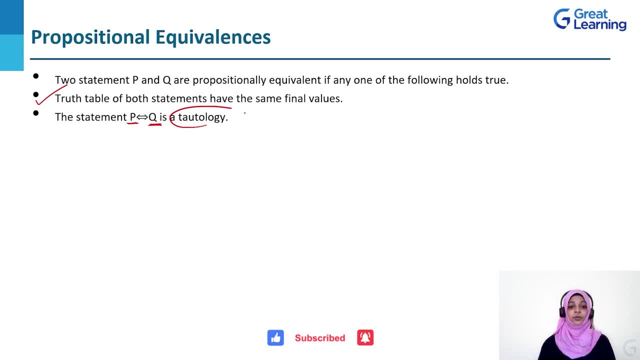 connective, or an if, and only if. connective, we would be provided by a tautology. if any one of these two conditions were true, then the statements were supposed to be equivalent to each other. we also have seen an illustration of the same, with an example we saw.